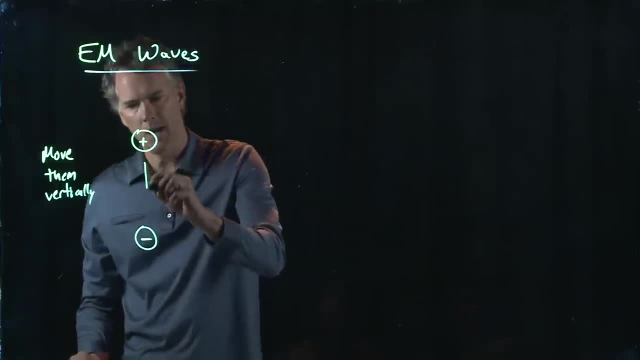 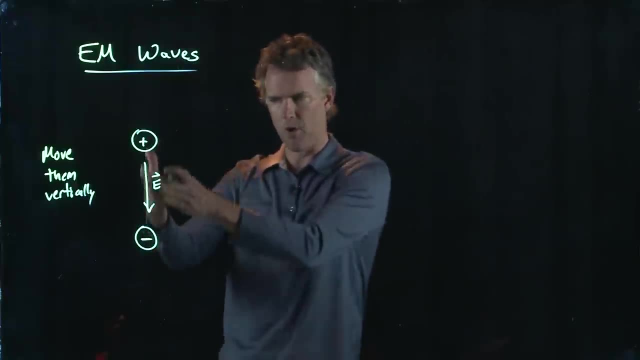 And if I think about the electric field in between these two, I know what the electric field looks like. It's pointing from the positive to the negative. Okay, I'm just going to draw one line for simplicity, But now let's move them vertically. 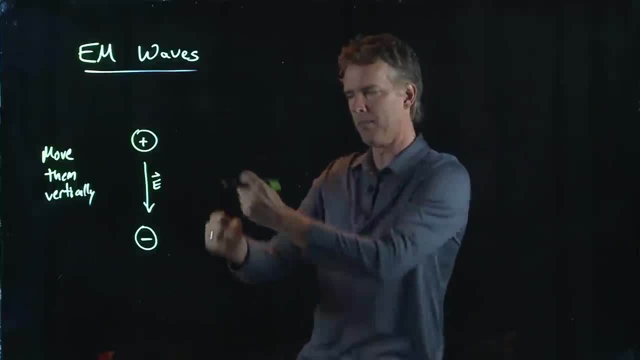 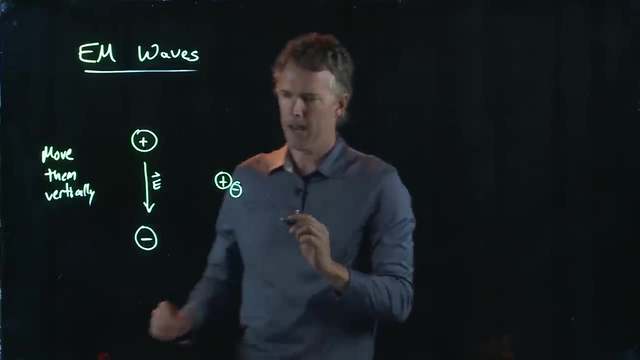 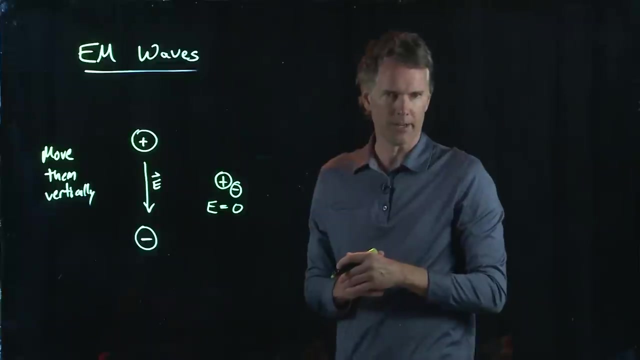 So the plus is going to come down, the negative is going to come up, And so at some later time They're nearly right on top of each other, And at that time the E field is essentially zero. Okay, There's nowhere I can draw an E field very cleanly. 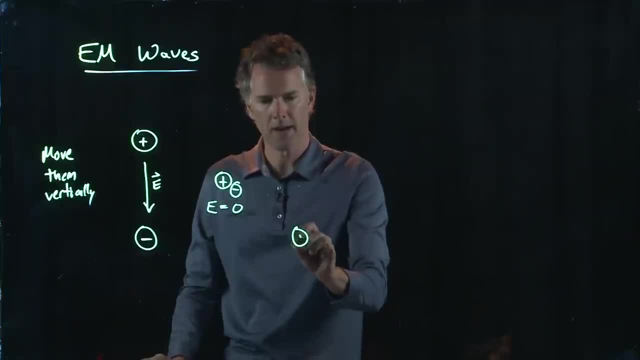 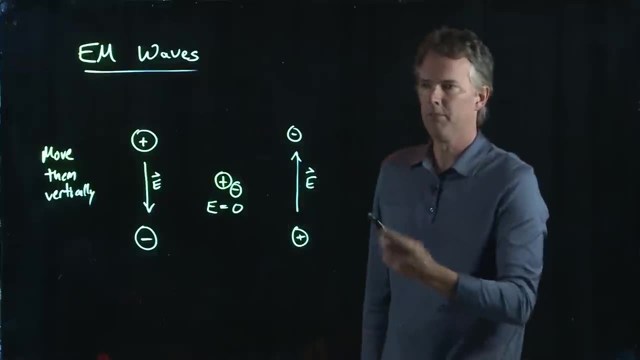 But now let's keep moving them. We're going to put the positive charge all the way down on the bottom and put the negative charge up on the top, And now the E field is pointing up. Okay, So all we're doing is we're taking these positive charges and negative charges, we're putting 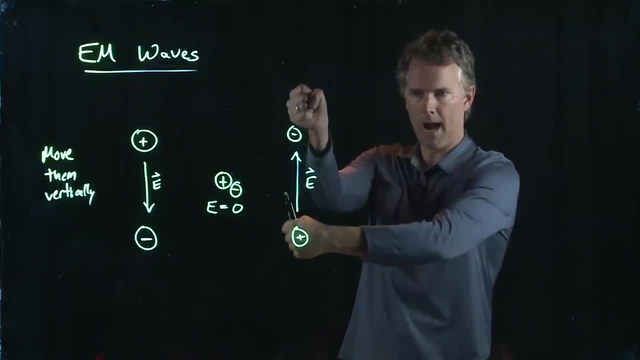 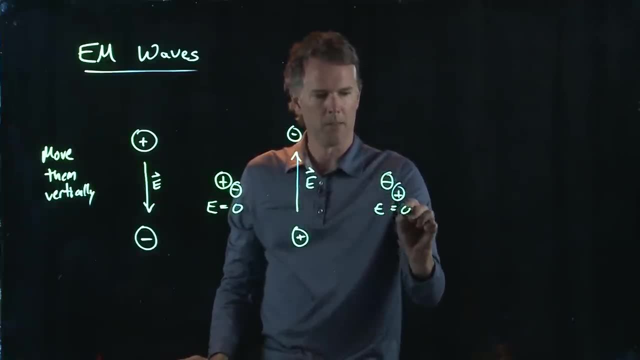 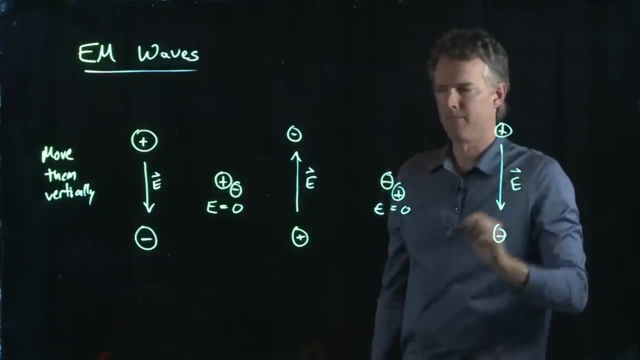 them together and then we're going to keep moving them. So now they're the opposite way, And then we're going to come back together again. So now the minus is heading back down and the positive is heading back up, And eventually they're back to where they started. 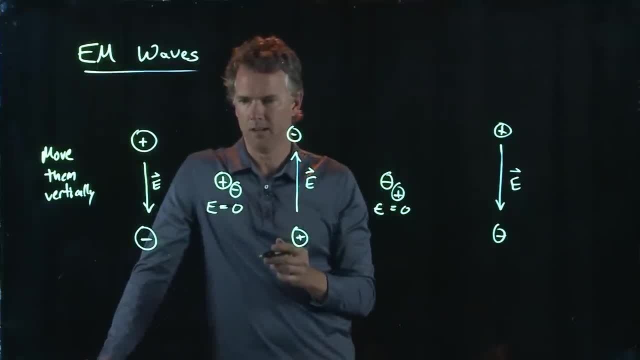 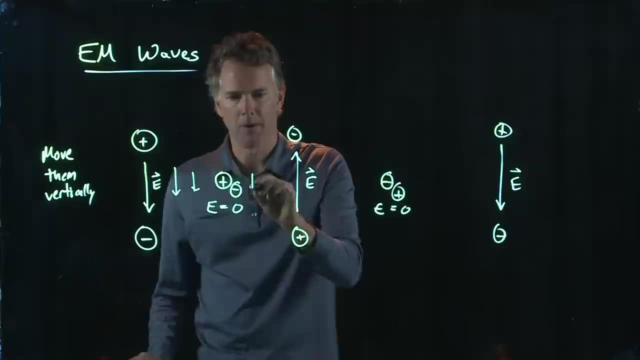 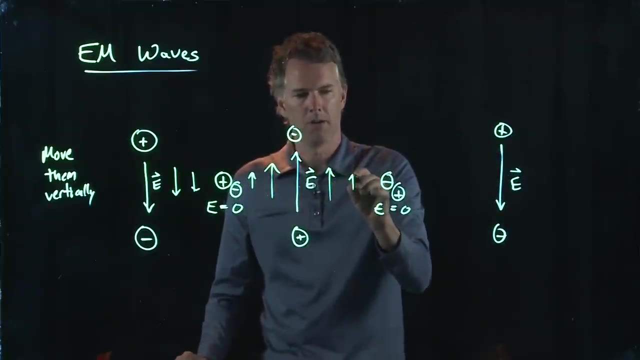 So if I think about what this E field looks like, it is getting smaller and smaller and eventually zero. Okay. And then it flips direction and starts getting bigger and bigger, And now it's a positive. And then it gets smaller and smaller until it's zero. 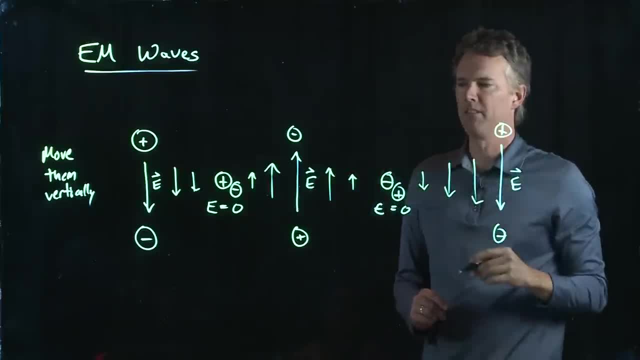 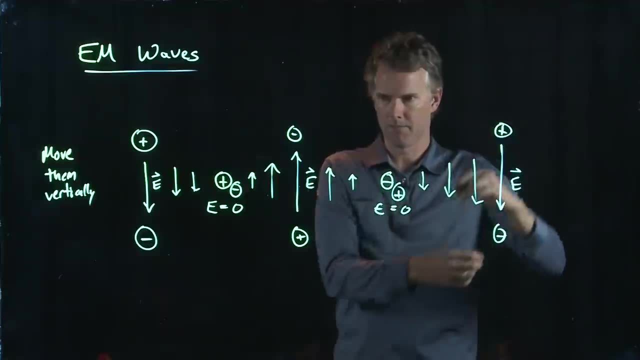 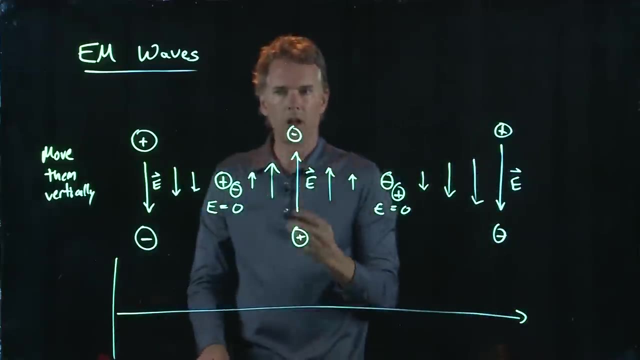 And then it flips direction and gets bigger and bigger until it's again pointing in the negative direction. It sort of oscillates up and down, Okay, And that hopefully looks familiar to you. All right, We like things that oscillate, Okay. 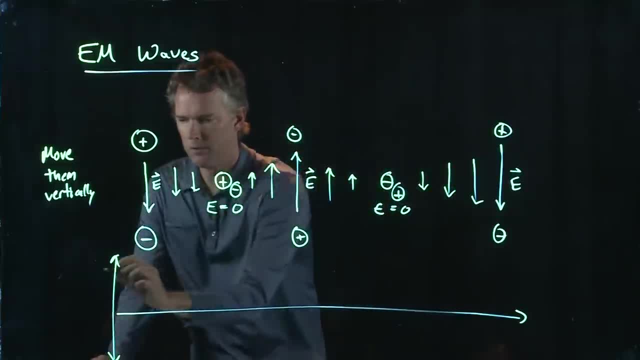 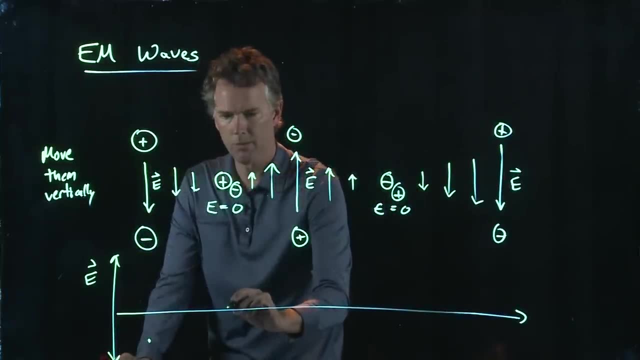 And if I think about drawing the electric field as a function of time, now what can I say? Well, here it was negative, So it's some negative value. Here it was zero. Here it was positive. Here it was zero, Here it was negative. 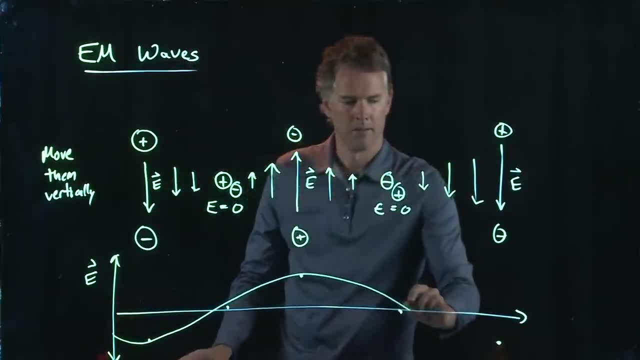 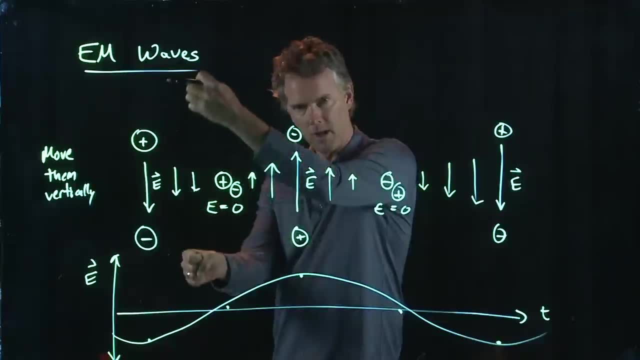 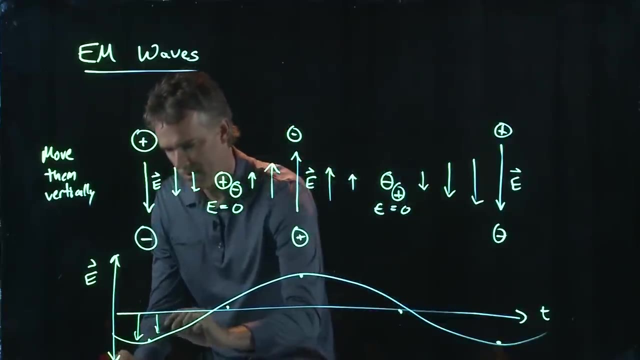 And so it's going to look something like this: Okay, It oscillates up and down as a function of time As I move these charges up and down. Okay, Okay, The electric field is going to oscillate up and down. It's pointing down here. 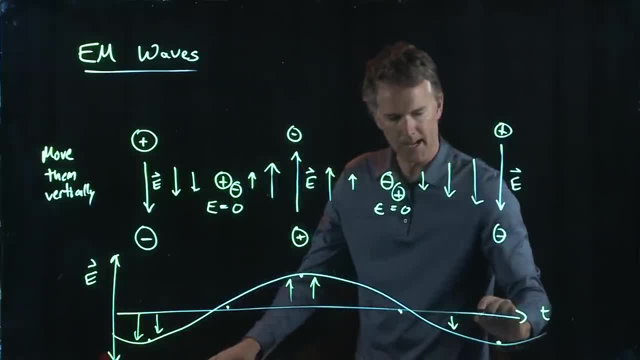 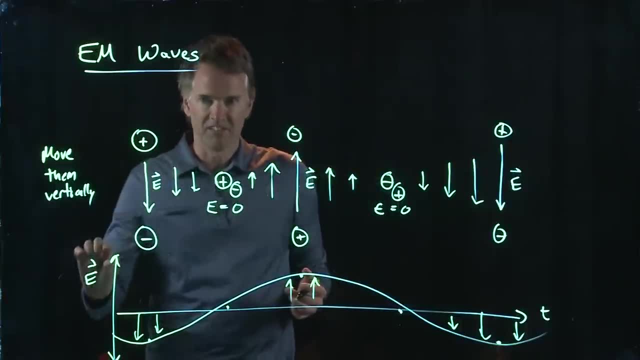 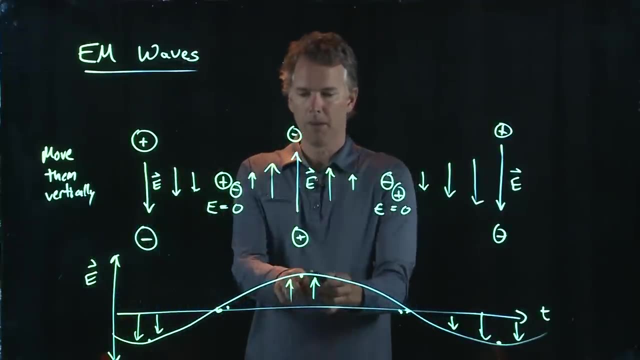 And then it's pointing up here, And then it's pointing down over here And so forth. A graph like this is just what is the size of the electric field as a function of time. So here the electric field is zero. Here the electric field is zero. 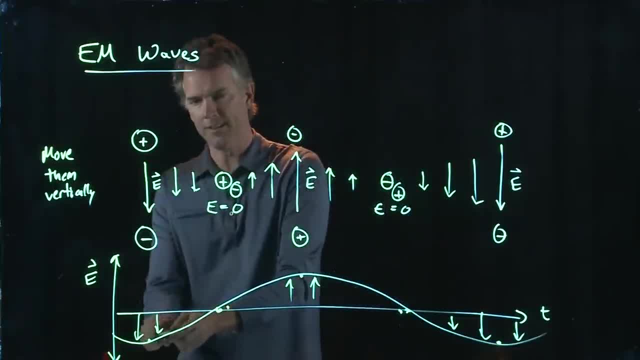 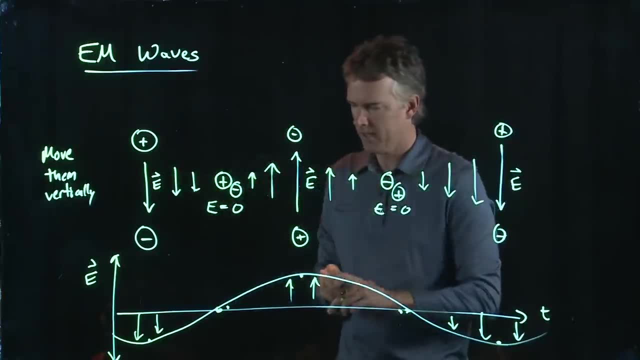 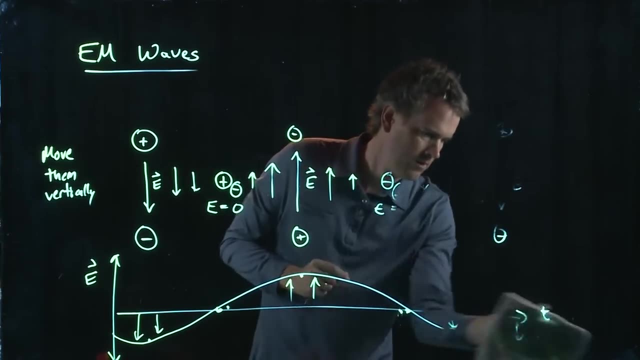 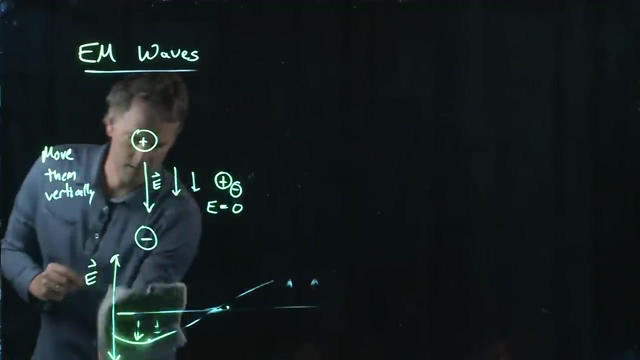 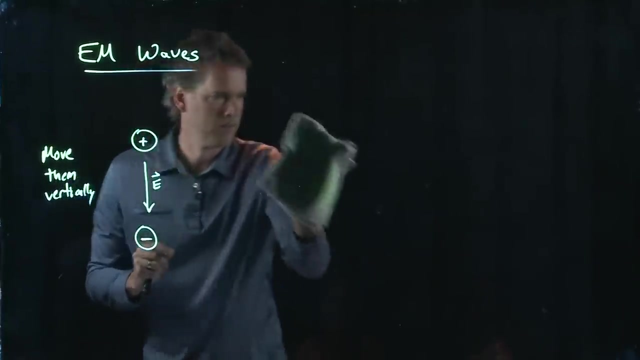 But at this point it's a positive number, At this point it's a negative number. All right, Let's go back to this picture here for a second And let's think about this: charge Okay, Charge Okay, Charge Okay. 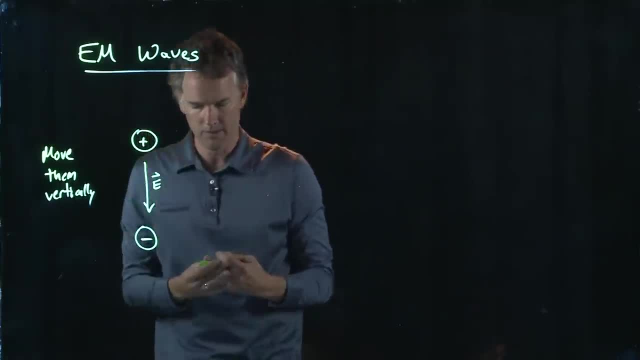 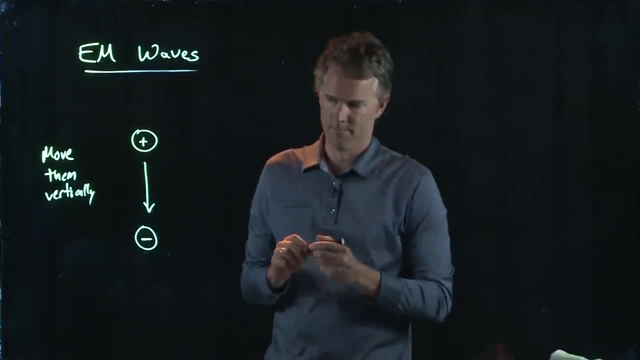 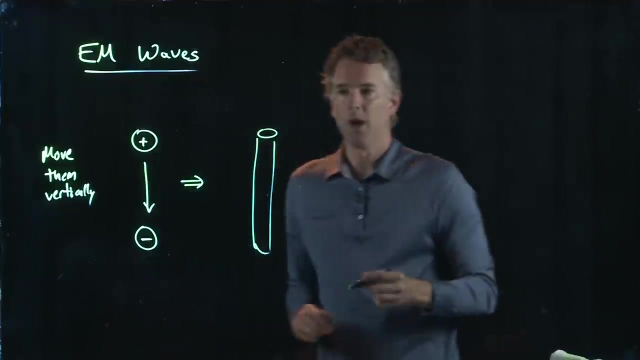 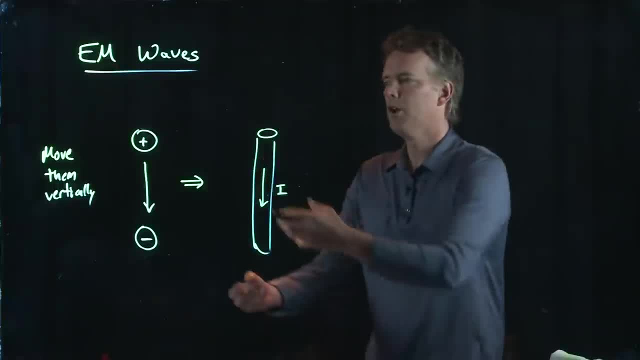 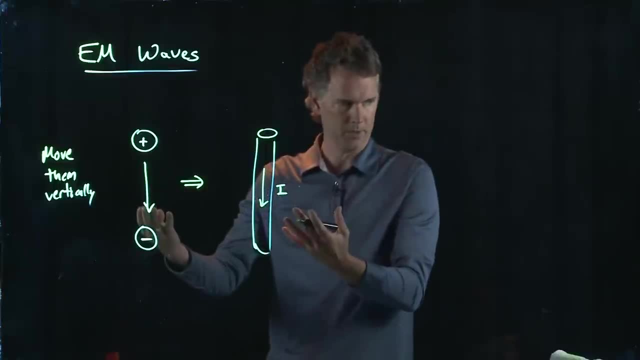 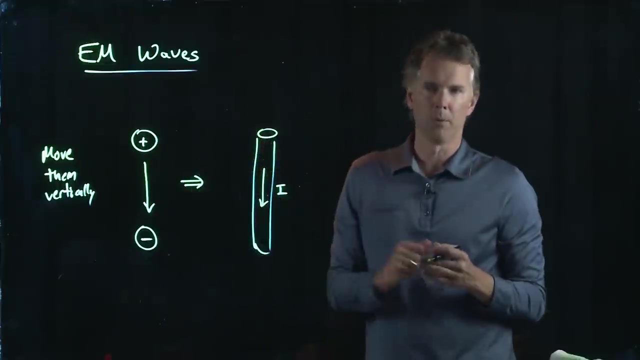 Power Car Car. Next is the magnetic field equivalent pictures. But we know what happens when we have current. What happens when we have current? What do we generate when we have current in a wire? It was the title of a couple chapters ago: Magnetic fields. right, If we have current, we have magnetic fields. 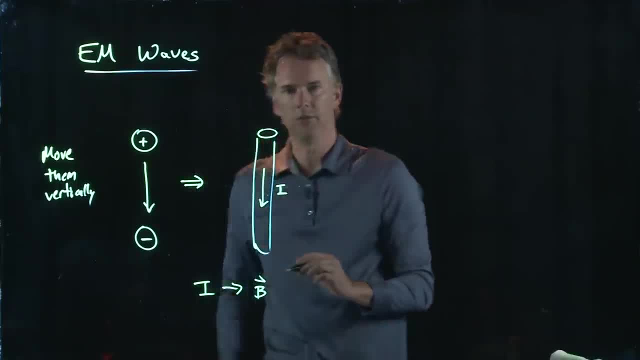 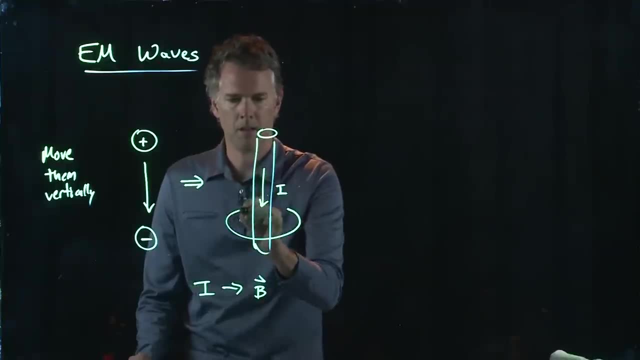 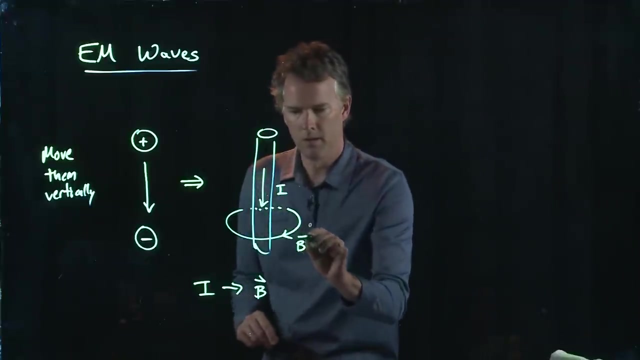 I leads to magnetic fields B, And so there is a magnetic field that develops here. How does it develop Like that? Okay, and you can pick the direction based on the right hand rule. Remember, you put your thumb in the direction of the current, So stick your. 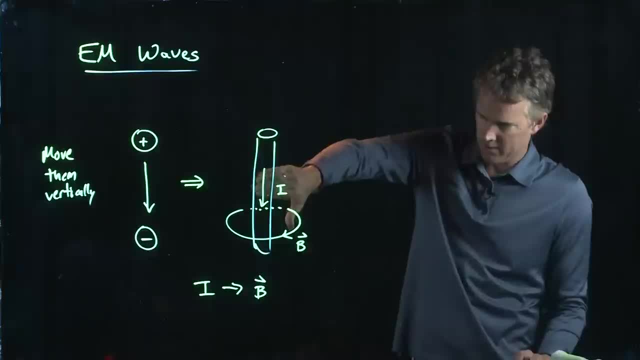 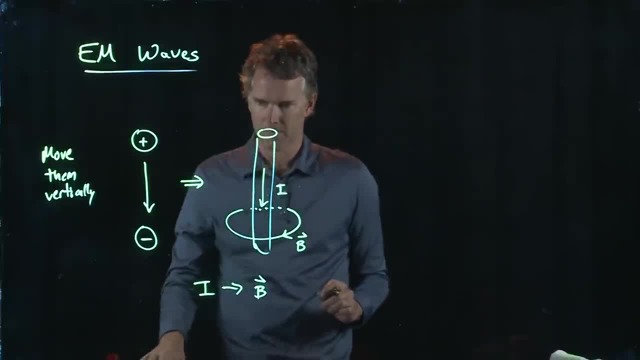 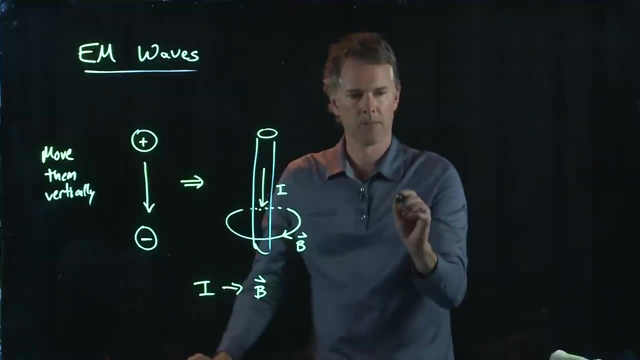 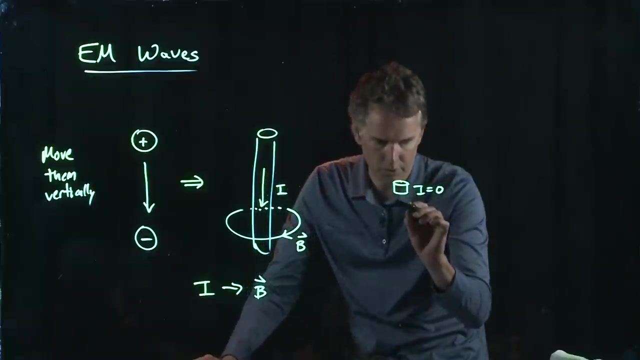 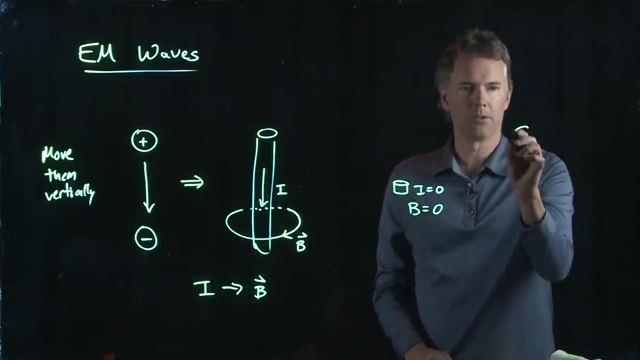 So we get a B field that looks like that for this particular picture. That was this case. But when those charges come together now the current is equal to zero, And if the current is equal to zero, then B is equal to zero, And later on, as we keep going, the 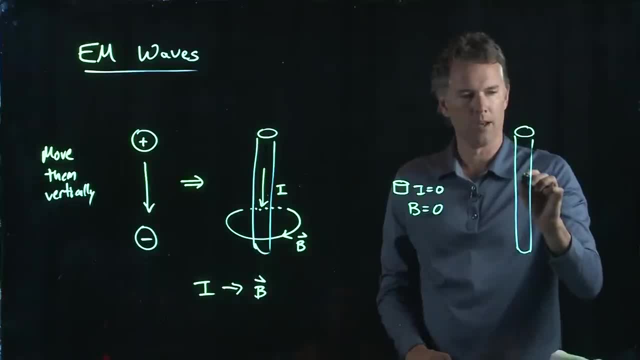 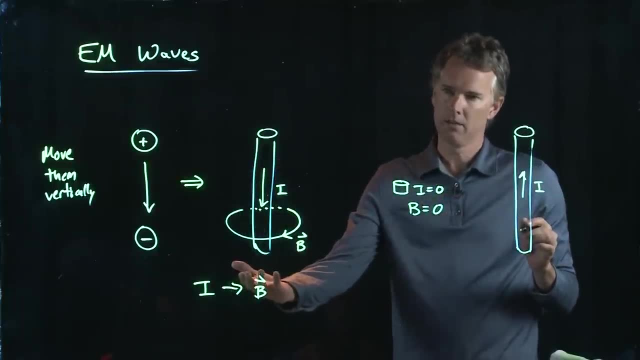 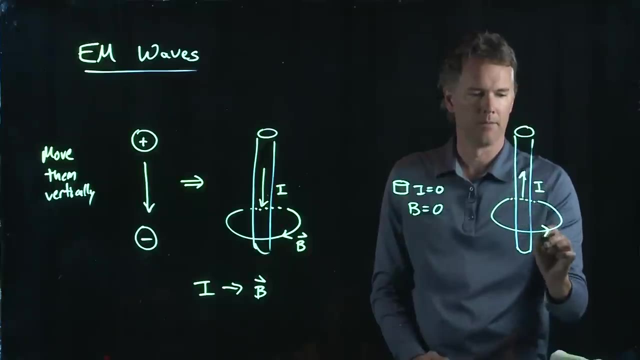 current is going to change direction. The current is going to be going up Later on And if current is going up, we again develop a B field And you use your right hand rule. And now it's wrapping around this way. Okay, Thumb in the direction of the current. 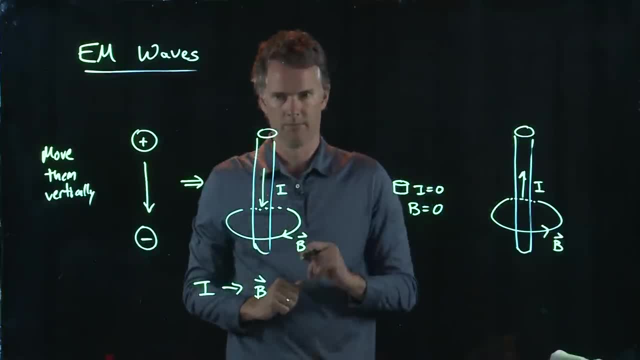 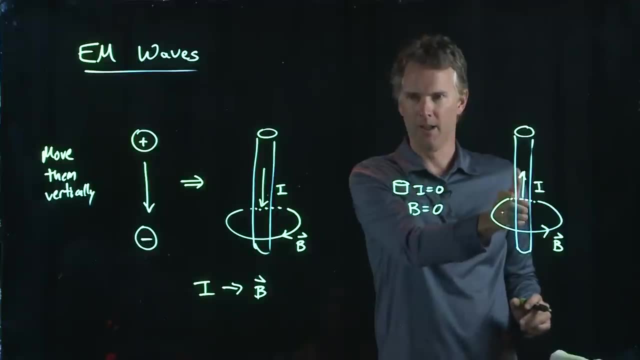 Fingers are wrapping around in the direction of the B field. Okay, Again, it's going to be confusing if you look at me in the glass here. So look at the computer monitor when I do this And confirm that your thumb going up is going to be in the direction of the. 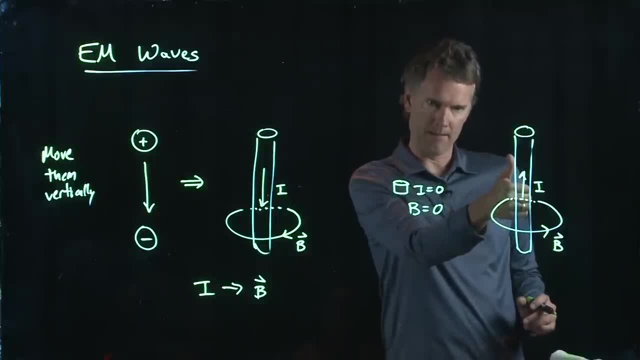 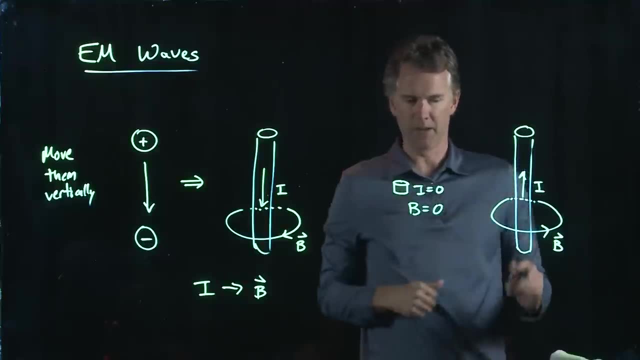 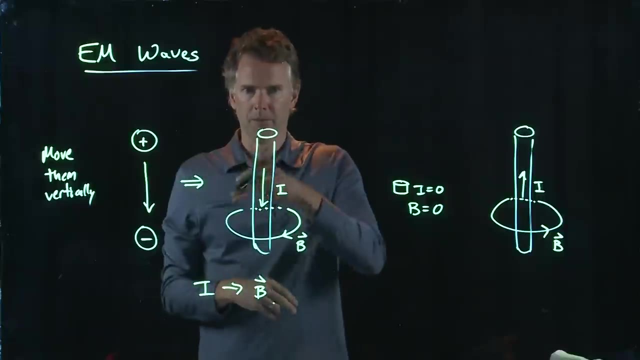 B field. The B field is going to be wrapped around in the direction of the B field And when you do it in the monitor, make sure you use your right hand. Does everybody see that one? Okay, So The charges went up and down. We develop an E that oscillates in time. But 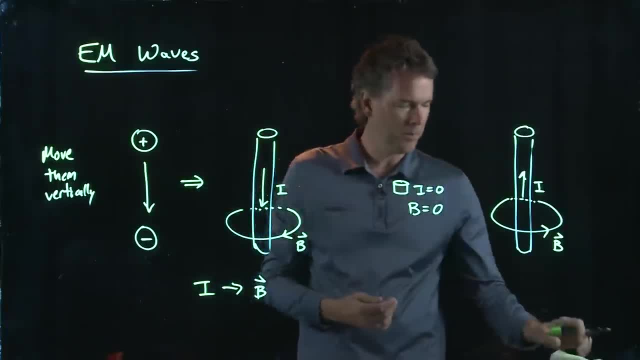 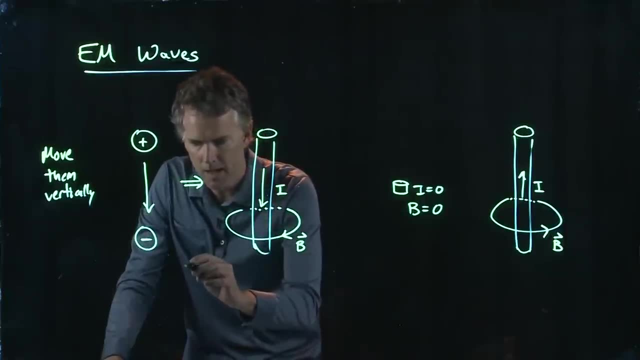 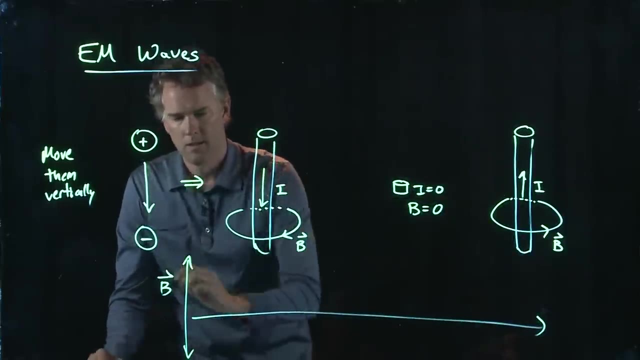 now we have a current that's going up and down And we're going to develop a B that oscillates in time And so if we draw B As if this was going to be, As if this was going to be function of time, it is going into and out of the screen. if I think about just 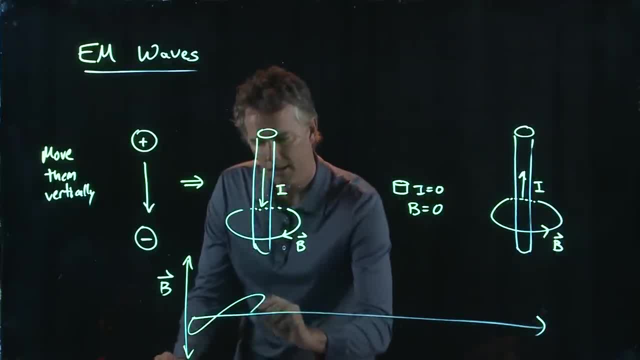 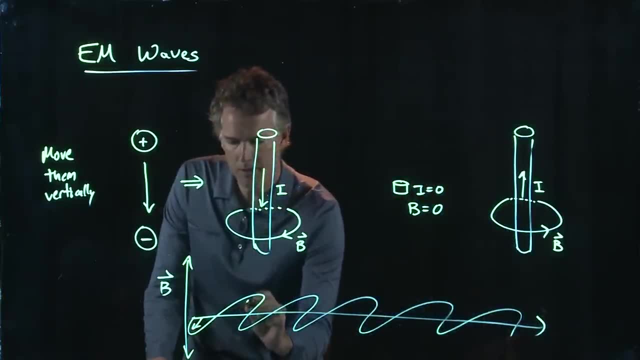 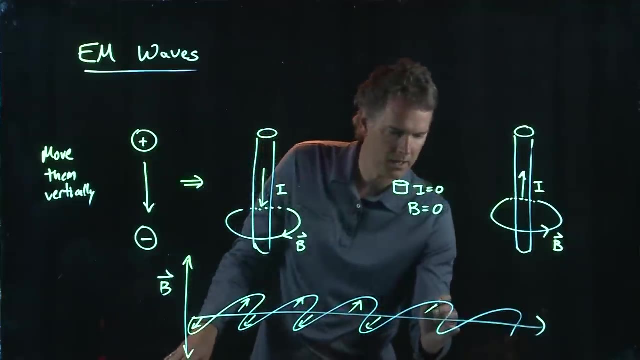 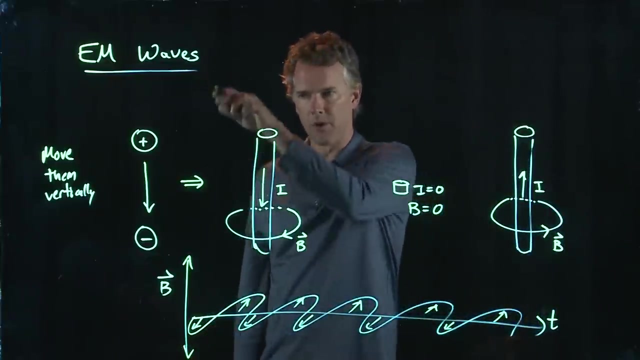 one side of this B is now going to be like this, and this is supposed to be coming out of the screen and into the screen over and over again, and we're trying to draw it in the third dimension here. so the E field was going up and down, but the B field is orthogonal to that. it is 90 degrees to. 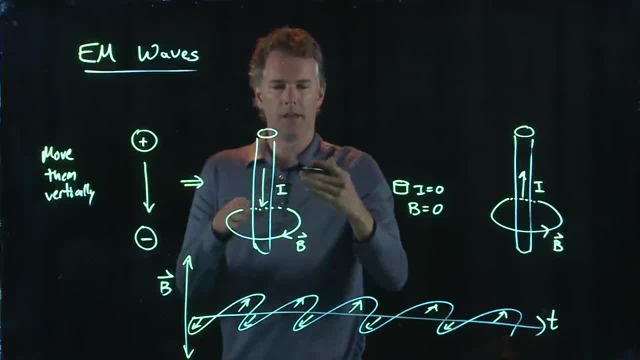 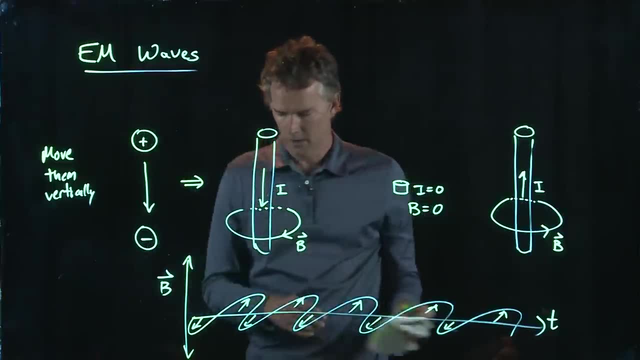 that. so if the B fields in the plane of the screen, then if the E field is in the plane of the screen, then the B field is in and out of the board. all right, but maybe we can put all this stuff in the middle of the screen, and then we can. 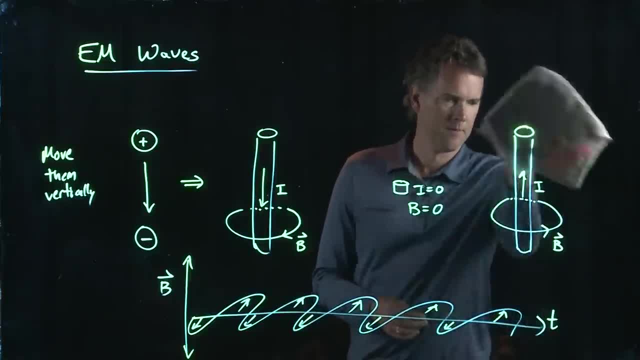 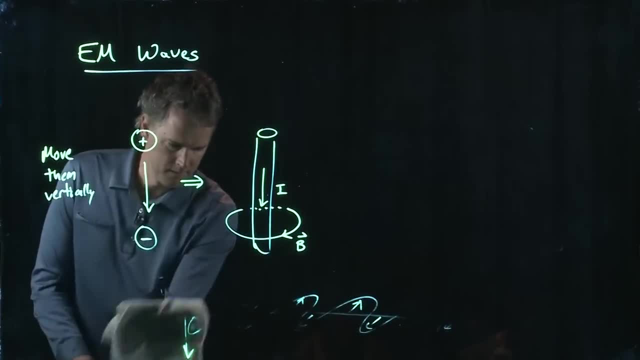 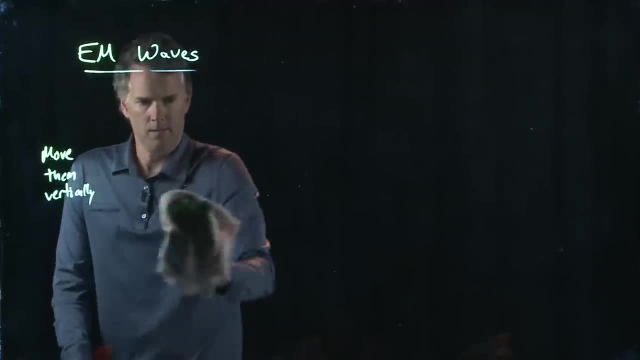 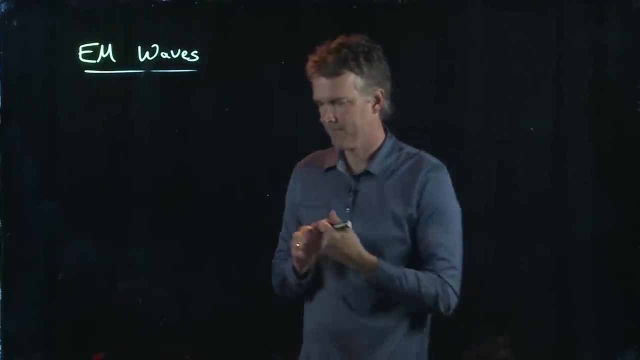 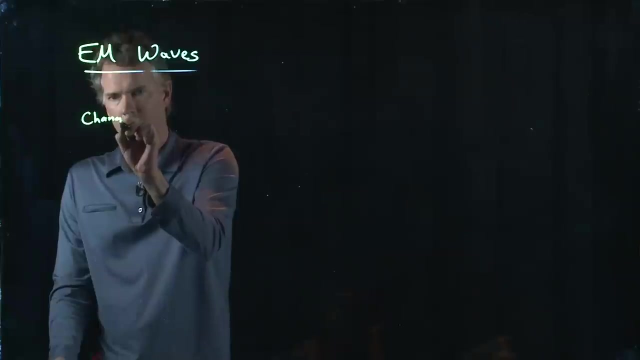 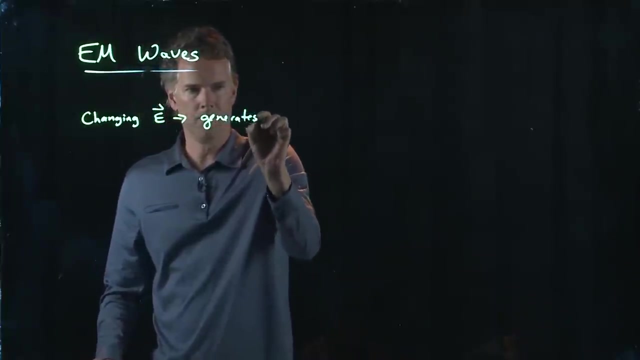 put all this stuff together. so the idea is this: a change in the little bit of time. if it's going to be in and out of the screen for the next five or ten seconds, there's going to be some kind of an interval between those fields that we're going to be using. okay, 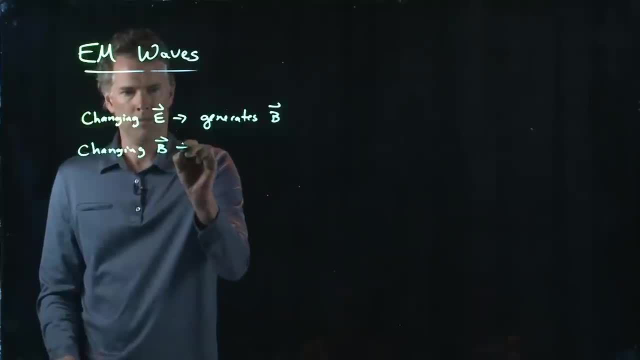 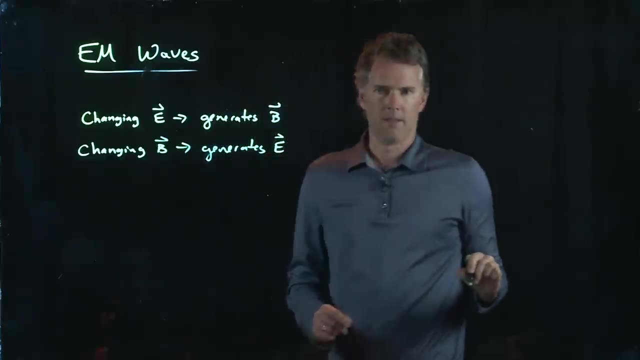 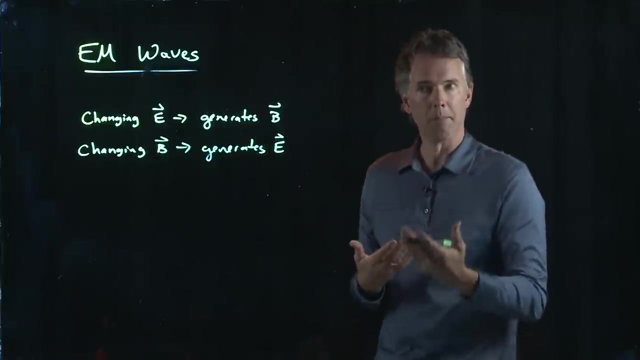 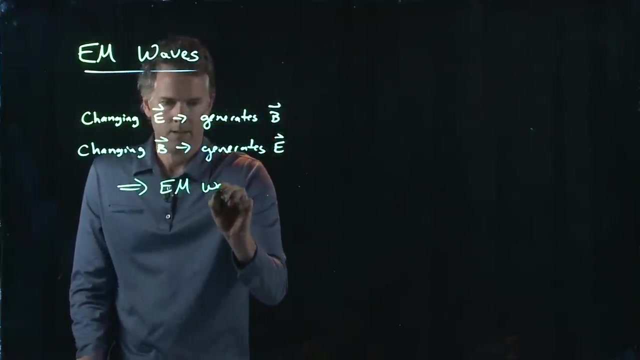 now, in the case of an E field, there's going to be a change in the time frame that we're going to be using. oh, that's right. so I'm going to go ahead and go ahead and put it in the middle of the screen here. Maybe these things can balance out just right, that you can generate electromagnetic waves. 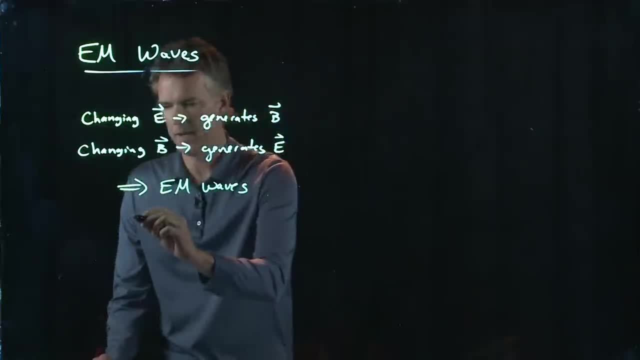 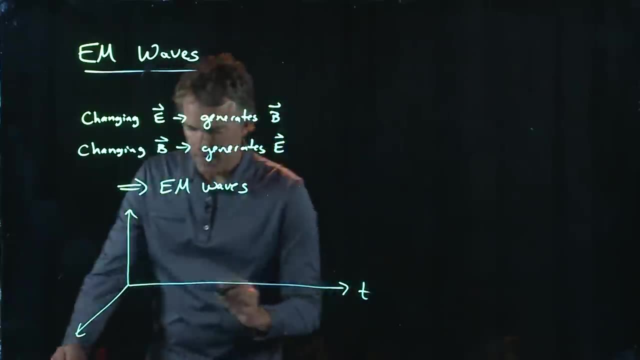 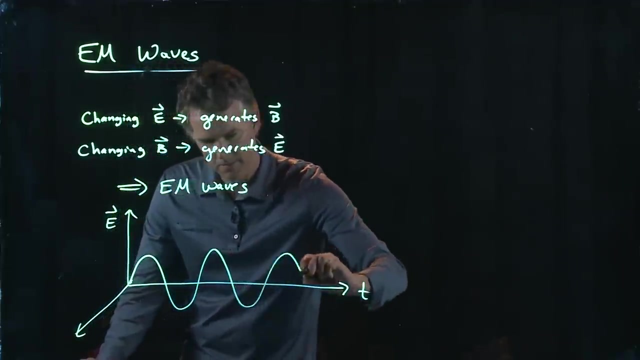 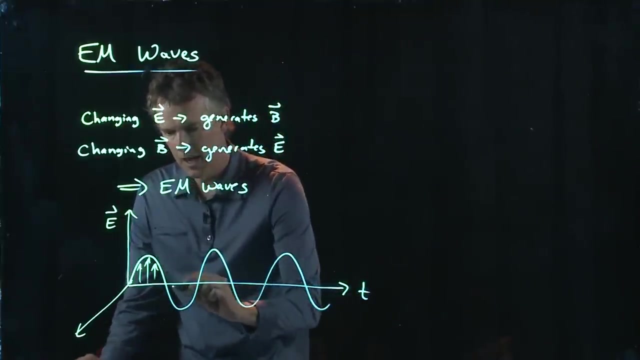 and that is indeed what happens. An electromagnetic wave looks like this: I've got an E field that is going up and down like so, and this means that it's pointing up in this region, and then it's pointing down in this region, and so forth. 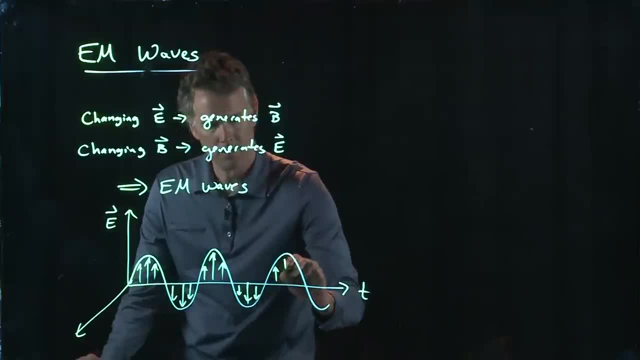 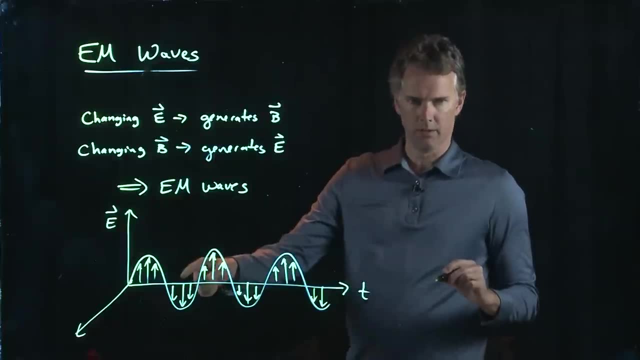 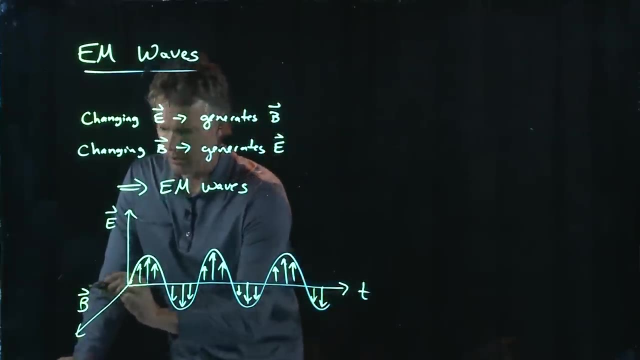 Up, goes through zero pointing down and just keeps oscillating back and forth. But that changing E field Can generate a changing B field and the B field is orthogonal to that. It's at a 90 degree angle to it. So if E is up and down in the plane of the board, then B is in fact going in and out of the board. 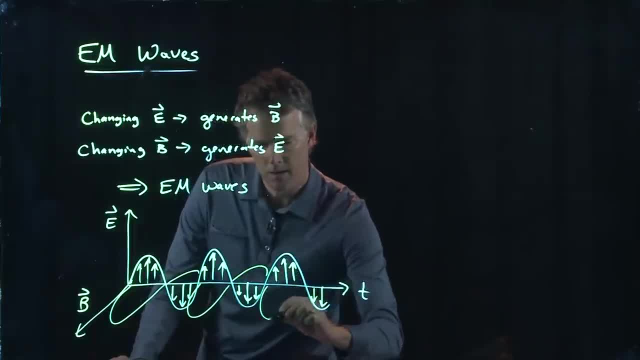 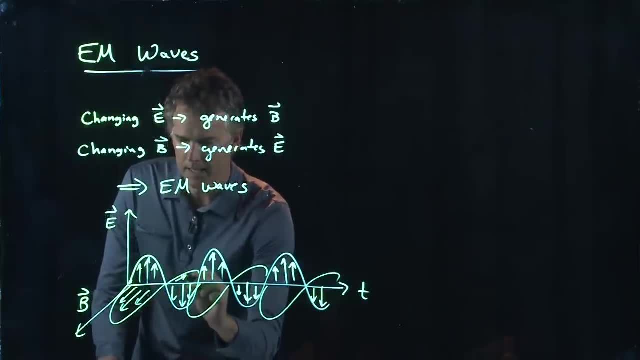 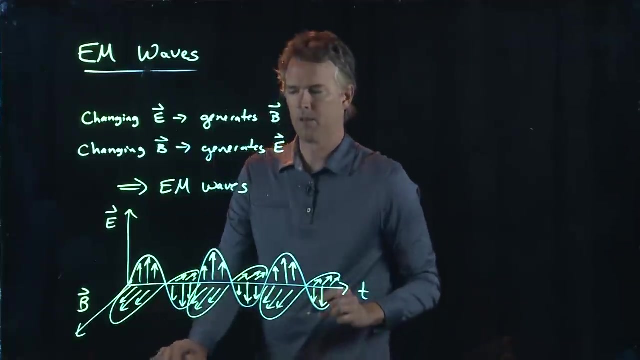 And this is a little hard to draw, but the idea is: B is pointing this way and then it's pointing into the board, And then it's pointing out of the board And then into the board, and so on. So these things are doing something like this. 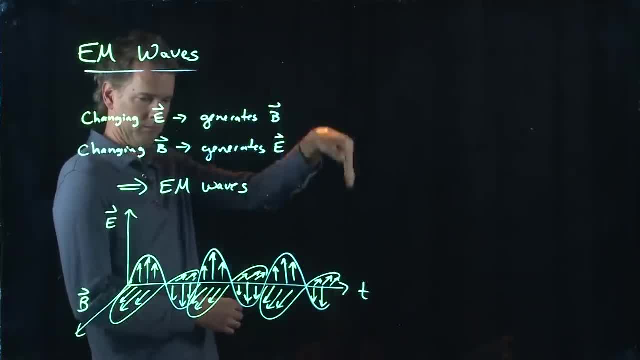 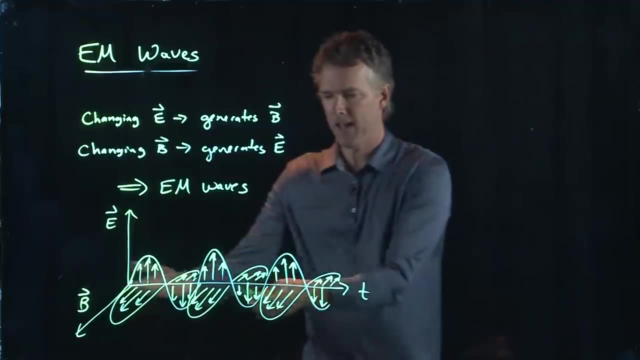 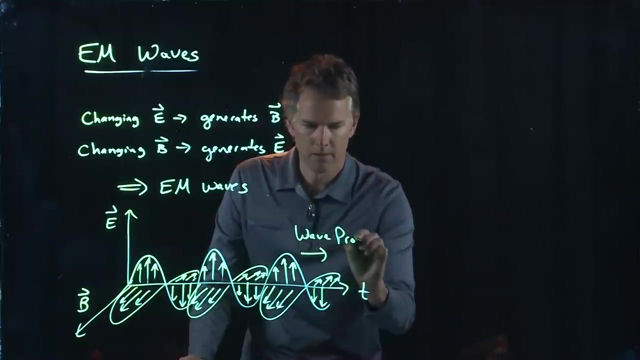 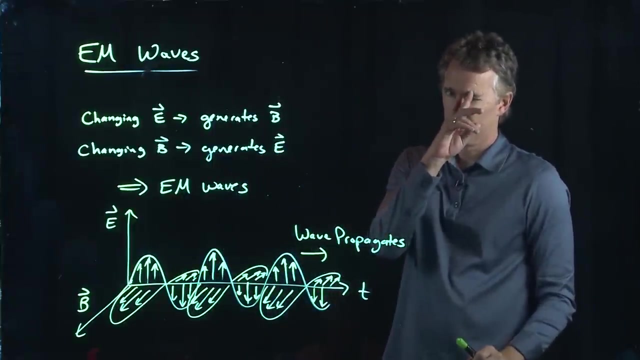 E field is going up and down, B field is going in and out, And so they're sort of doing this. It's like two fish Swimming along, one going up and down, one going left and right, And, as this happens, this entire thing propagates to the right. 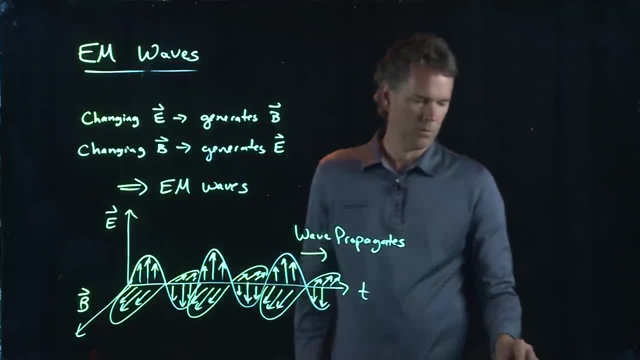 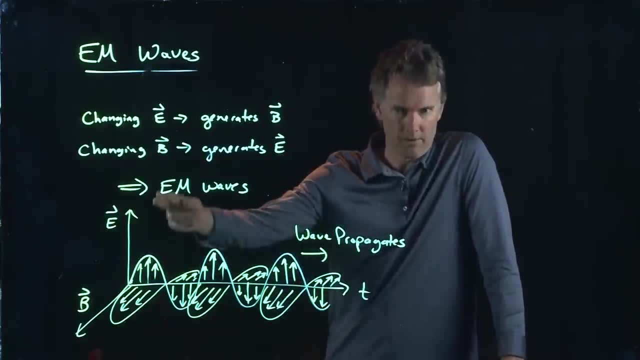 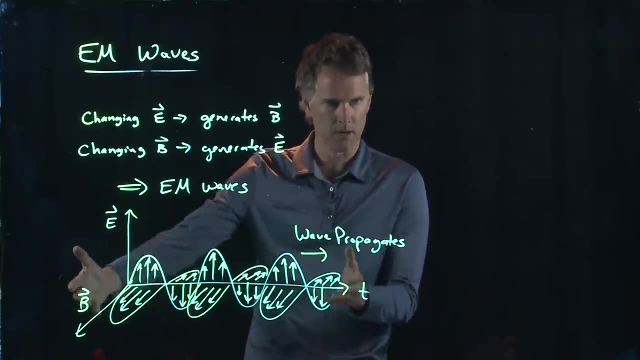 So what is weird about this? What's weird about this is there's no charges anymore, There's no, There's no wires of current anymore. These things can just propagate on their own, because the changing E field creates a B field. Changing B field creates an E field. 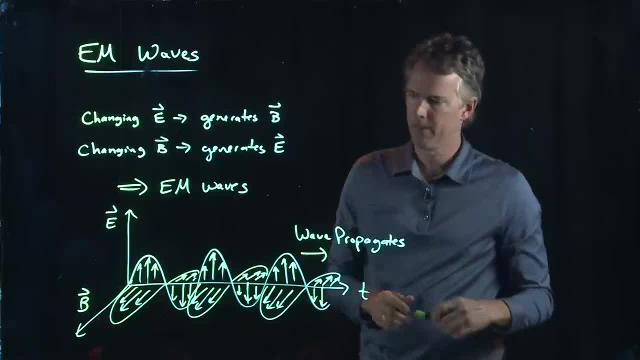 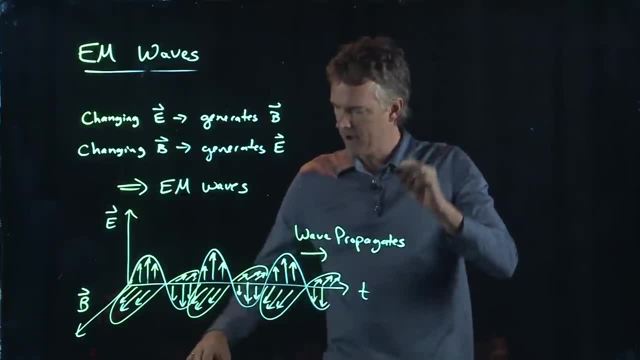 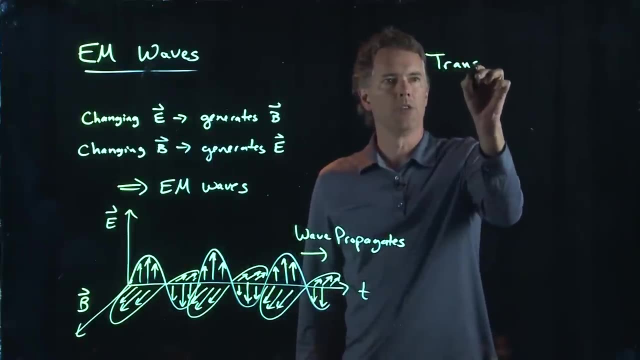 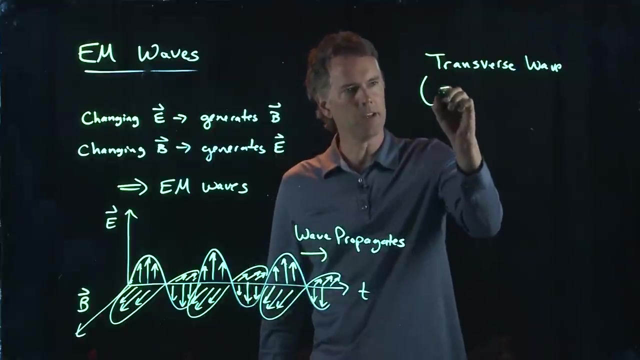 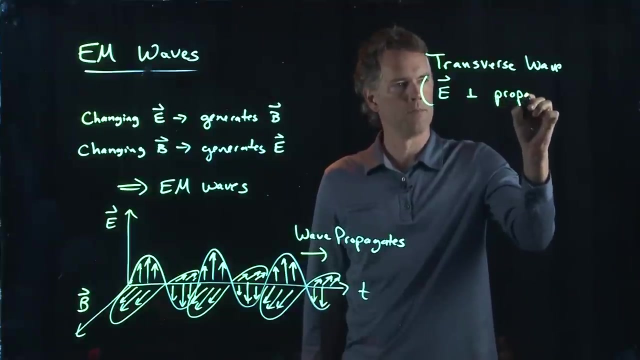 And they just keep going like that, sloshing back and forth, And this is called an electromagnetic wave. So how fast do these things propagate? We said that it's going to propagate to the right. It is called a transverse wave because the E field and the B field are perpendicular to the propagation direction. 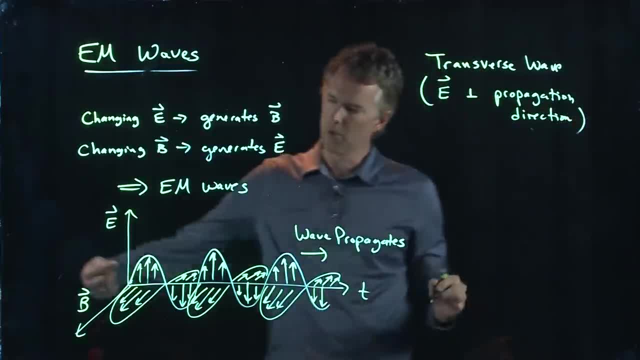 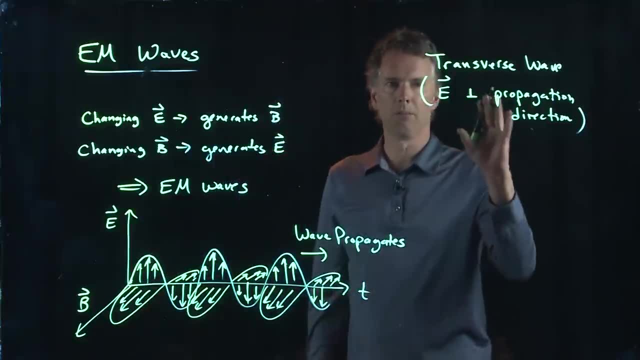 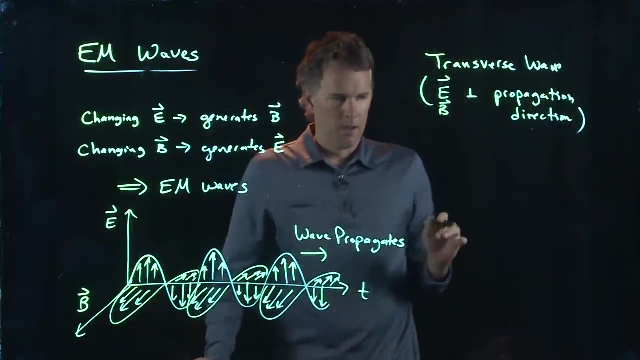 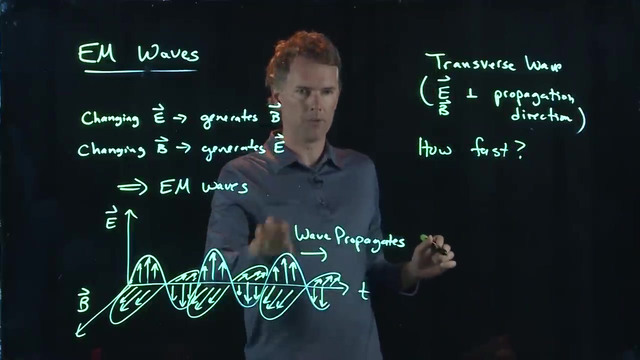 So, even though the wave is moving this way, the E field is oscillating up and down, The B field is oscillating in and out. Those are both perpendicular to the propagation direction. How fast are these things moving? How fast does an electromagnetic wave propagate? 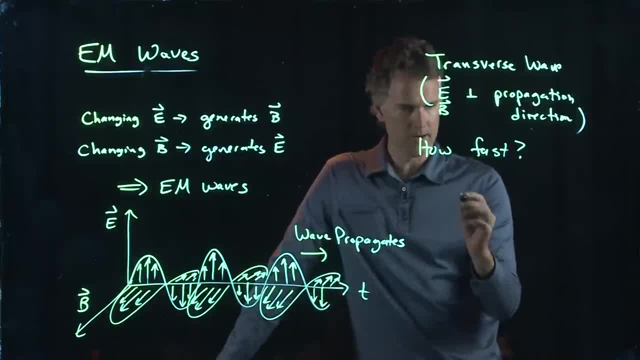 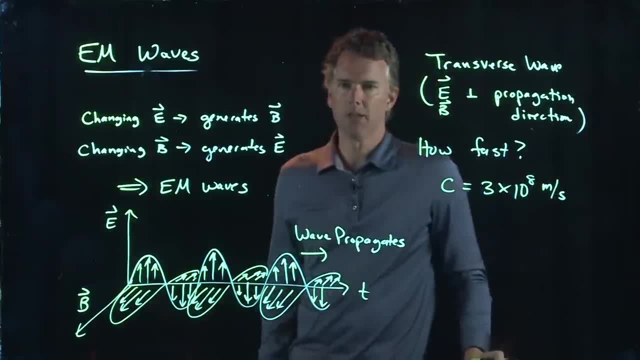 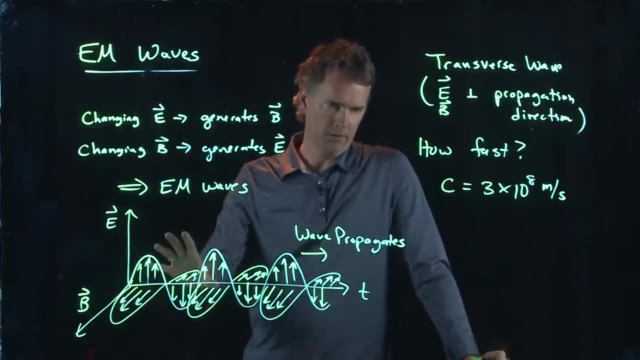 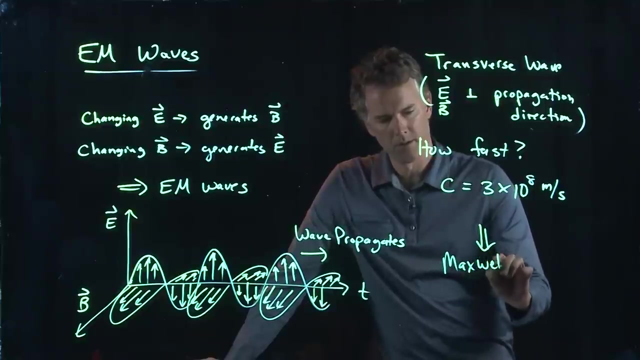 Well, I think we know the answer to that right. They propagate at the speed of light 3 times 10 to the 8th meters per second Right. So this stuff- electromagnetic waves- came about from something called Maxwell's equations. 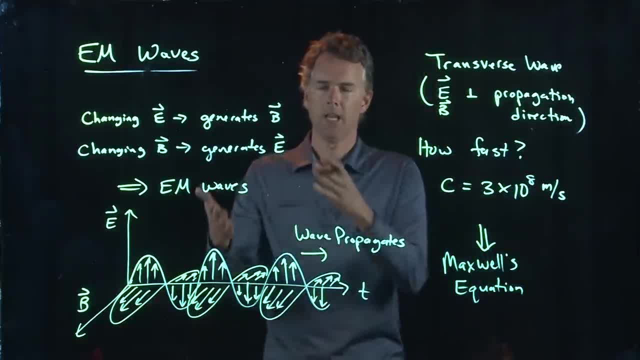 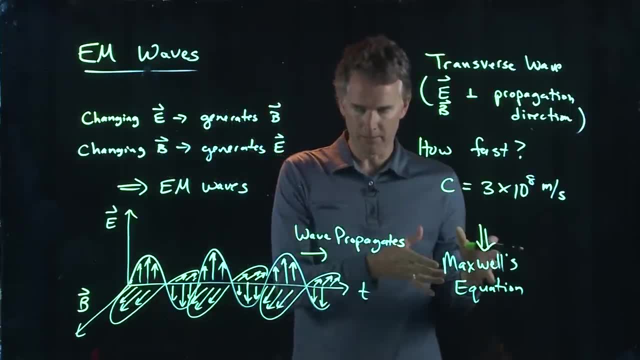 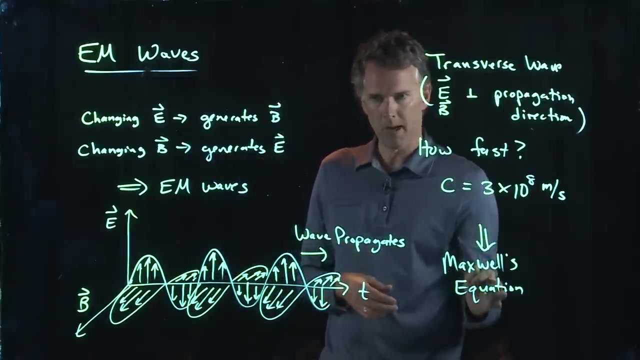 And up until Maxwell we had independent quantities, We had electricity and then we had magnetism. Electricity was governed by things like Coulomb's law. Magnetism was governed by things called Ampere's law. Faraday's law started to tie those two together, but it wasn't until Maxwell came along and 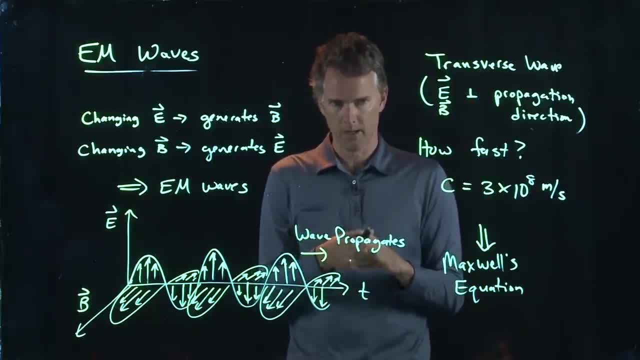 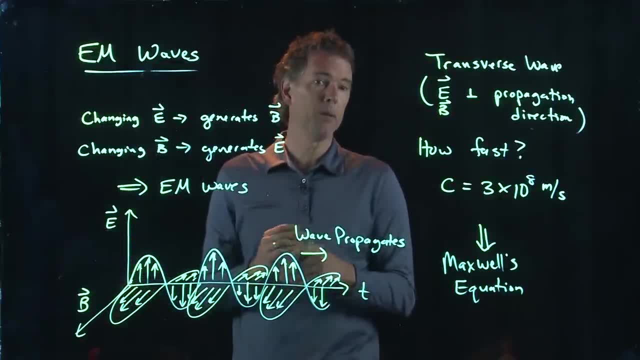 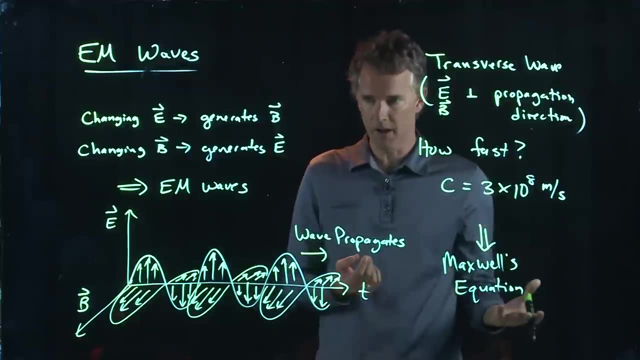 combined all of those things into one quantity that we ended up knowing that light itself is made up of electromagnetic waves. People knew a whole bunch about light. People knew a whole bunch about electricity and magnetism, but what they didn't know was that light itself was electromagnetic waves. 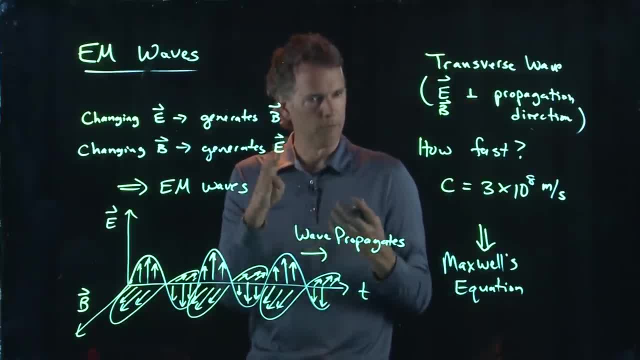 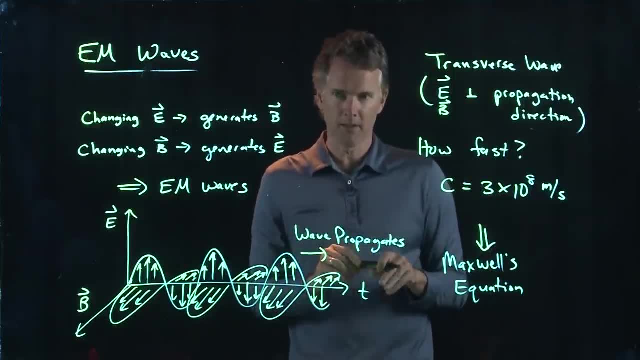 And Maxwell put all those equations together, combined them into four neat equations, And if you happen to continue in physics and take my upper division- electricity and magnetism- course, it's all about Maxwell's equations. Start with those four equations and spend an entire year trying to uncover all their. 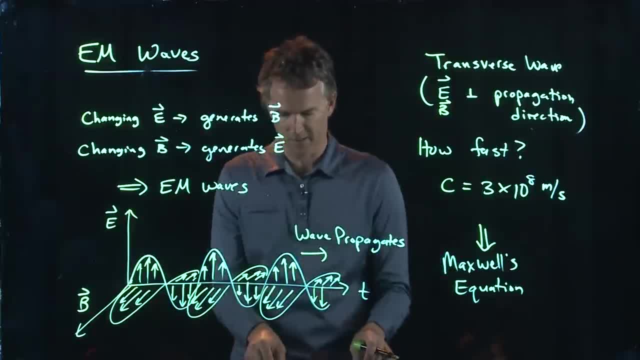 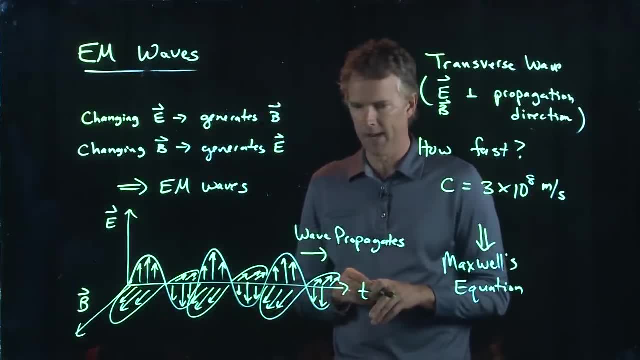 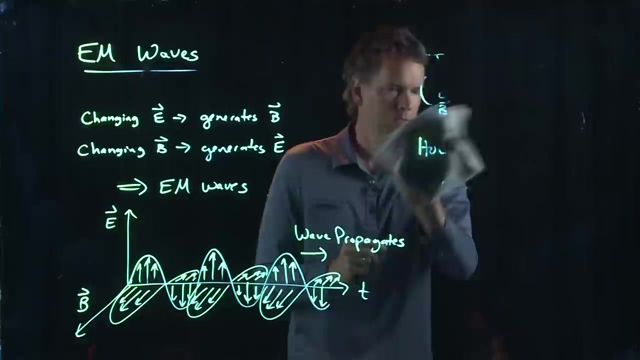 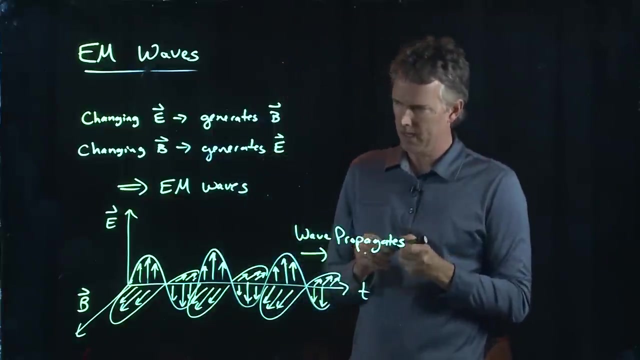 interesting phenomena. It's really very fascinating stuff. Thank you All right, If we have these changing electromagnetic waves that are flying around the universe, how do we detect them? Well, let's think about this wave right here. Let's say we do the following. 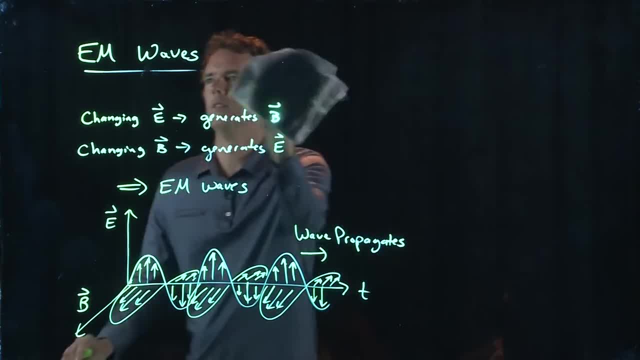 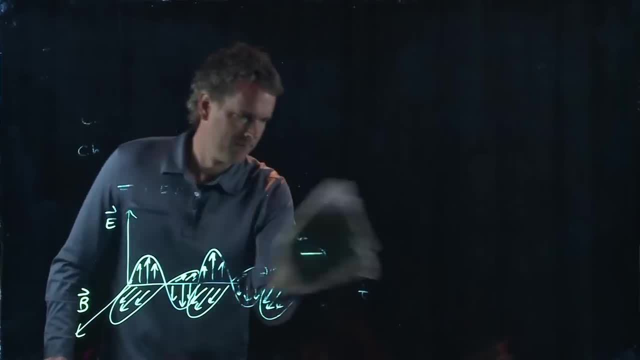 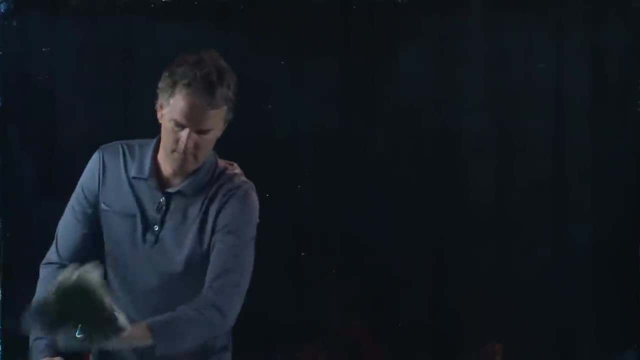 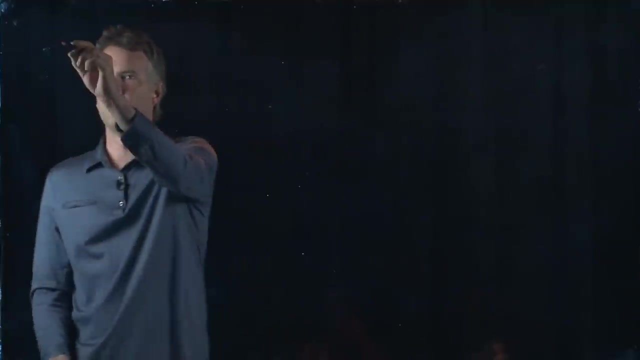 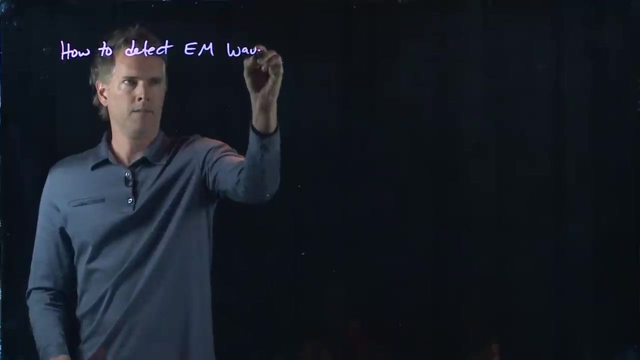 And let's redraw it, but let's erase the magnetic field, And if we say I'm a black hole, it derives our imaginary reality. All right, Okay, Okay, All right, All right, All right, Let's ask this question: How are we going to detect these electromagnetic waves? 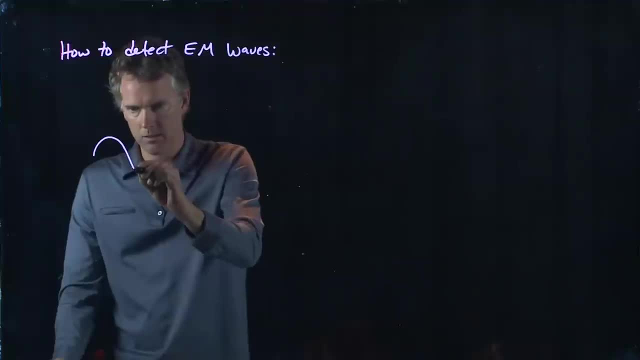 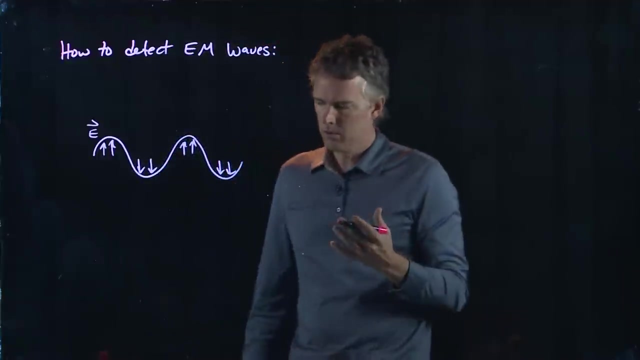 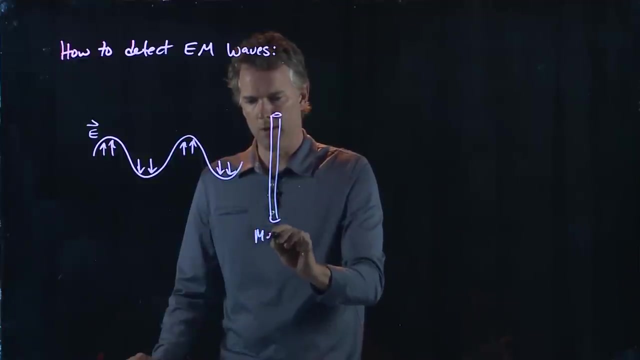 Well, let's draw the electric field coming along. Okay, it looks like that It's pointing up, then it's pointing down, then it's pointing up, and then it's pointing down. So let's take a wire And let's just hold it up right there in space, okay. 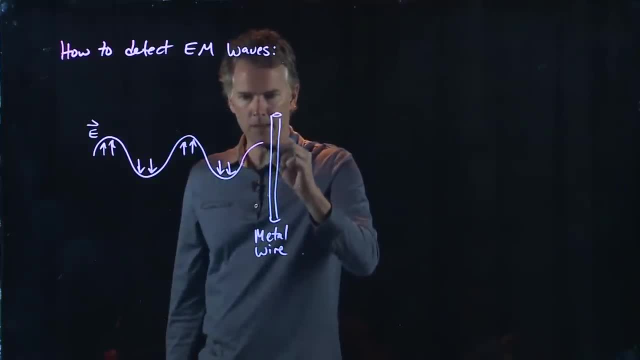 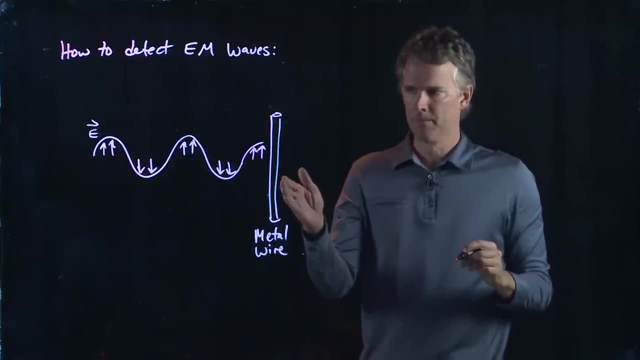 When the electric field comes along and it is pointing up what happens to the charges in the wire, They of course feel a force going up. The positive charges feel a force going up, the negative charges feel a force going down, And so there is a current 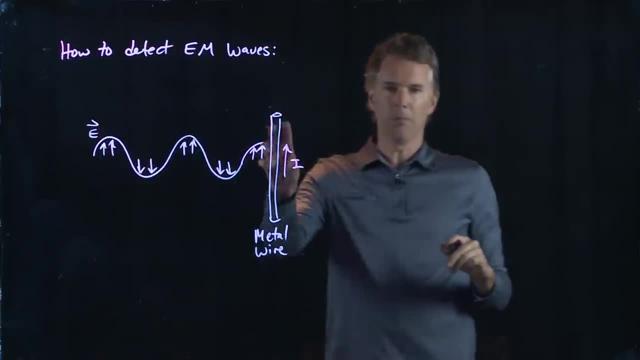 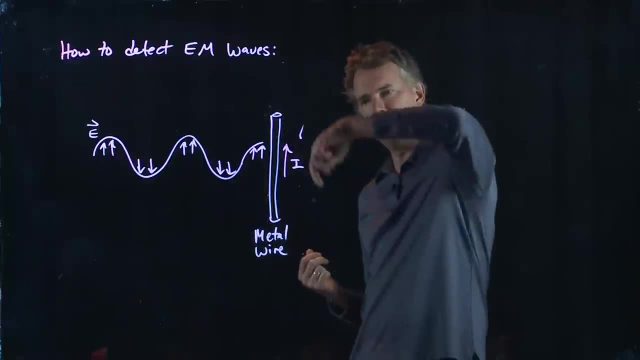 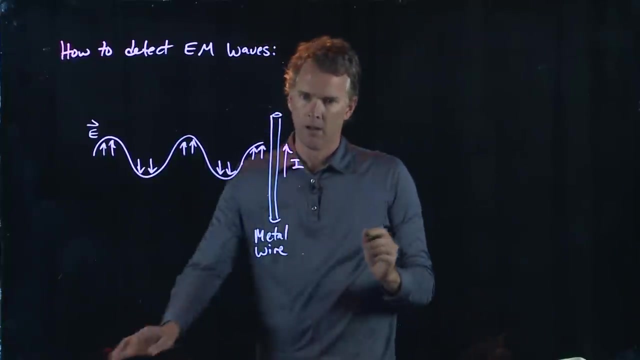 I, which develops in the wire. Okay, and later, when the electric field is pointing down, the current is going to flip and come back down. Okay, so the current will in fact oscillate up and down. Alright, let's take this whole wire and let's connect it to a circuit. 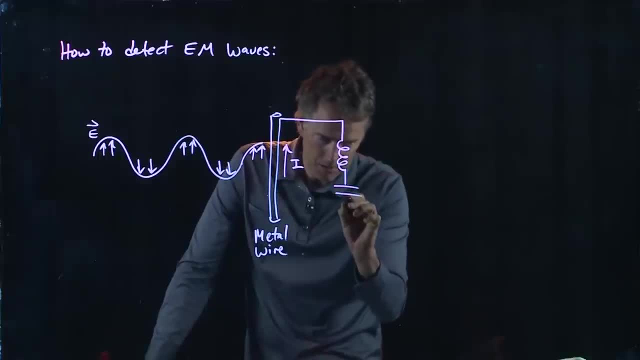 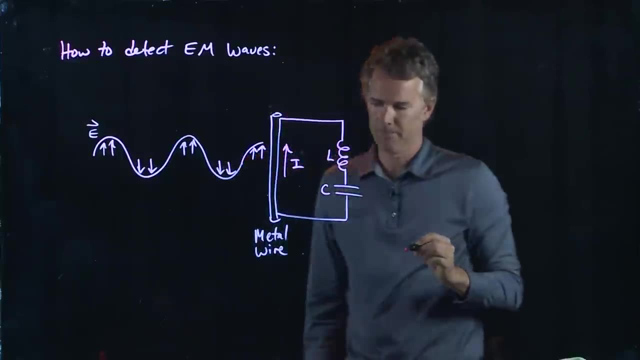 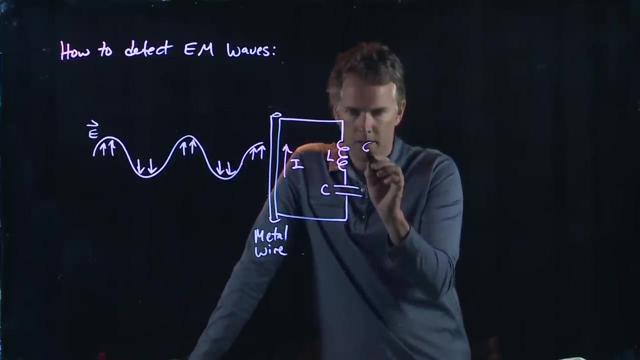 And let's connect it to a circuit that you are familiar with. now. Okay, and let's put in an L and a C in our circuit And let's connect another inductor right there. This looks like a transformer And we're going to send this signal to an amplifier. 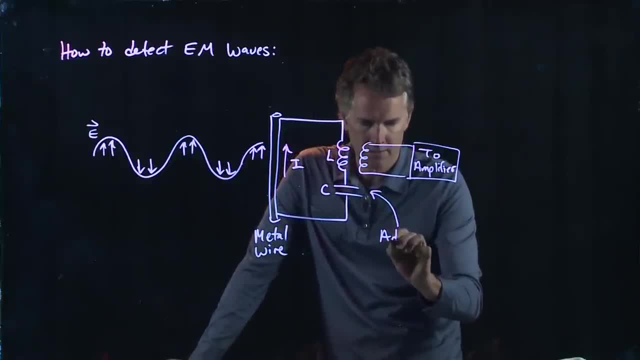 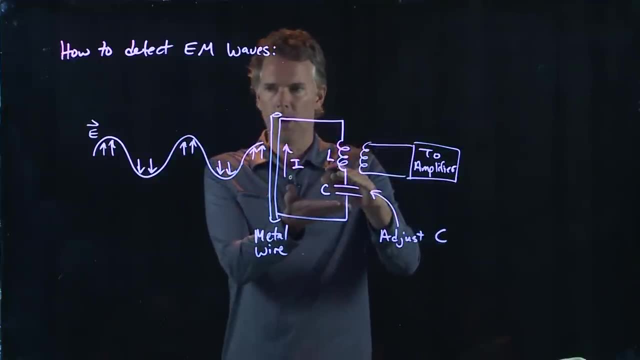 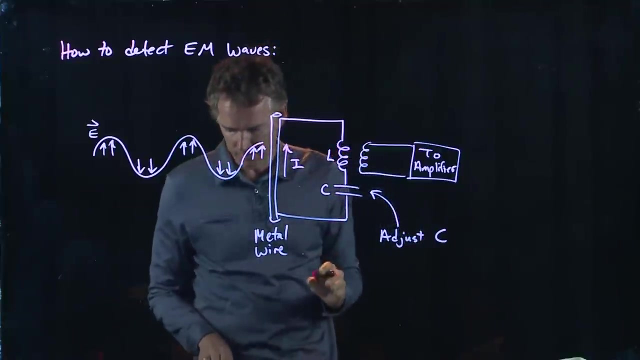 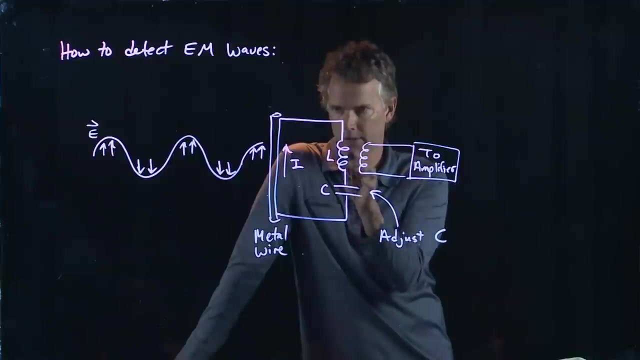 And now we're going to adjust the capacitor. How do you adjust the capacitor? Well, you can move the plates relative to one another and that will adjust the value of the capacitance. And if I do that, I can find a resonant frequency of this circuit that just matches the resonant frequency of the wave coming in. 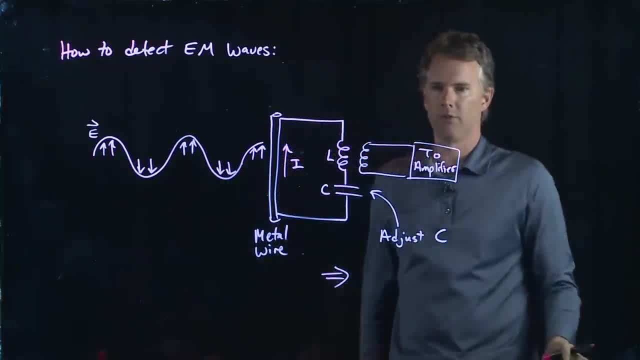 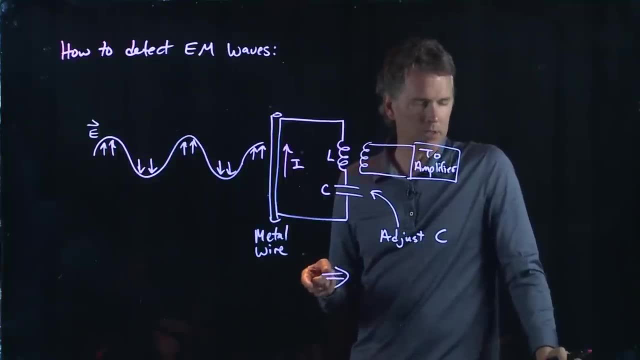 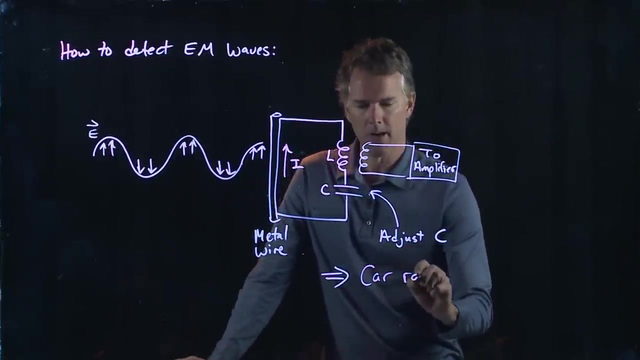 And this is a device that you're all familiar with. What device have we just drawn? I can almost guarantee you you've used it today. Anybody know what we just drew? Okay, nope, not your phone, It is your car radio. 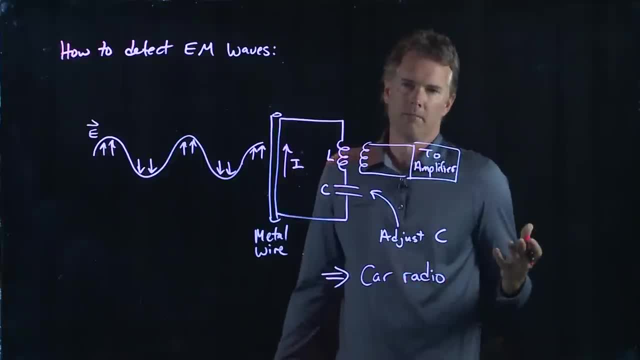 Okay, this is your car radio. You guys are like I don't have a fancy car with one of these radios in it. I did for a while, but then it got stolen, Haven't replaced it, So now I just listen to my iPod while I drive, which is illegal if you have two. 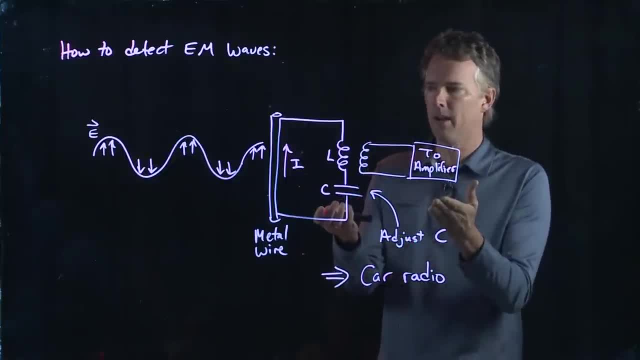 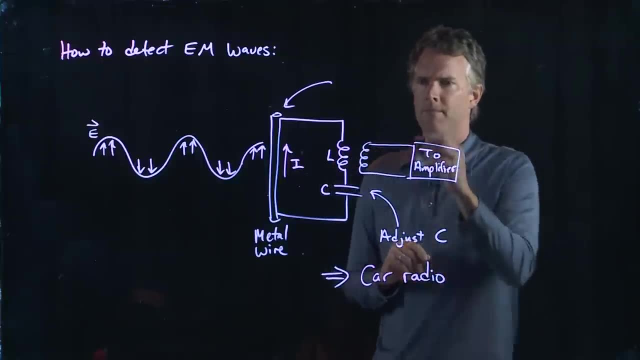 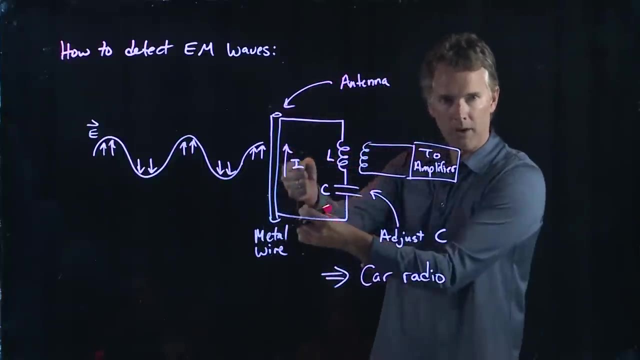 headphones in. So don't do that. Alright, this is your car radio. What is this thing? What is this big metal wire? That's your antenna. Right, You go outside your car, you reach in and you pull out this big telescoping wire. That's your antenna. What is it there to do? 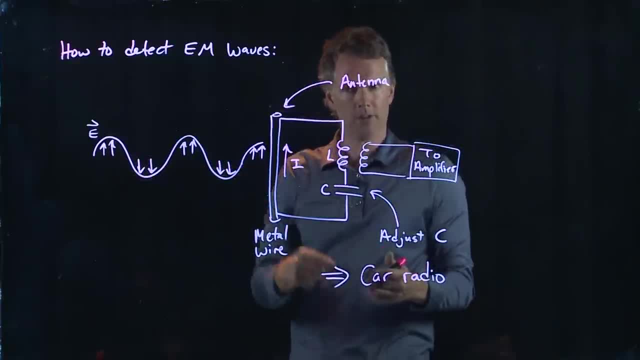 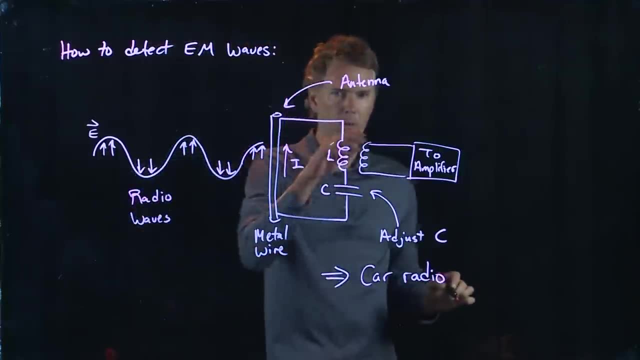 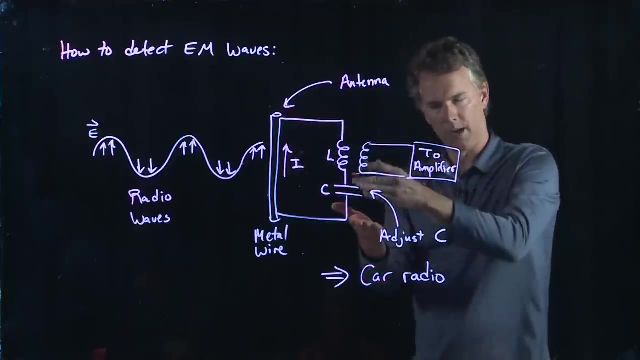 It's there to collect the radio waves that are coming in. This is from the radio station. Okay, those radio waves come in. they hit your big metal bar, it excites current up and down, it transfers to your car stereo system and when you pick just the right value, 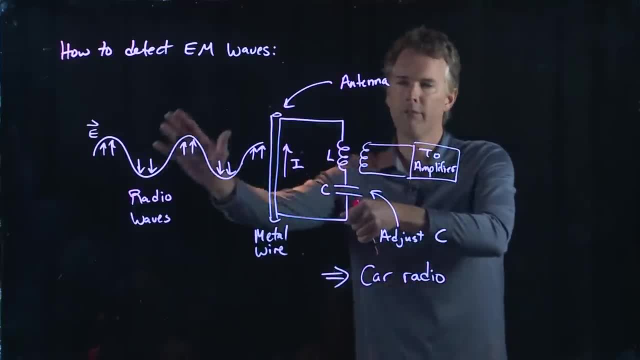 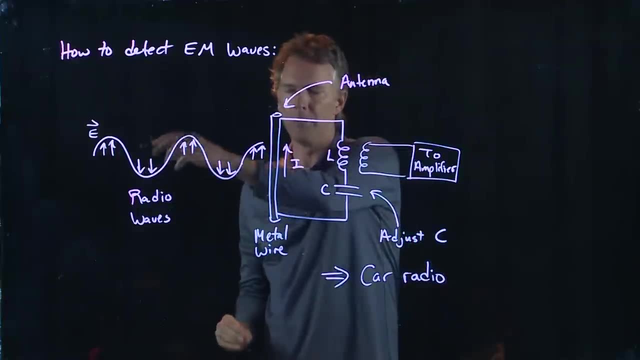 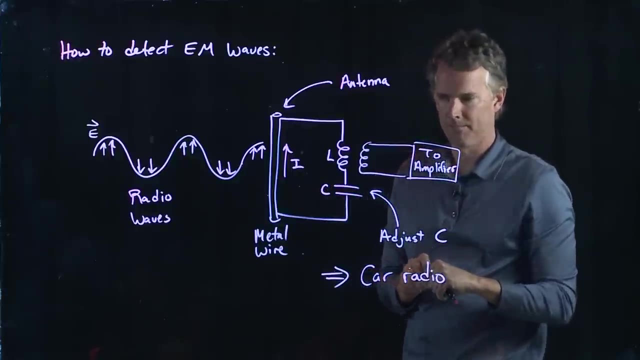 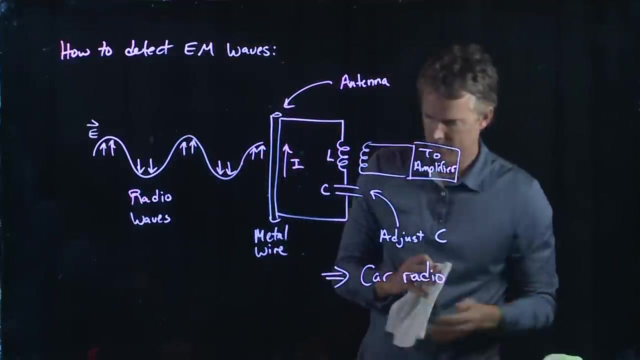 of the capacitor. it will go up and down. You tune in to a particular frequency, Every different station is coming in on a different frequency And so there will be different oscillations here, and by adjusting C you move that frequency up or down the dial. Okay, let's talk about the electromagnetic spectrum. 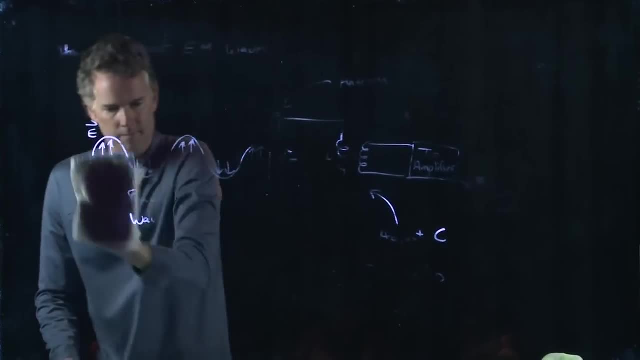 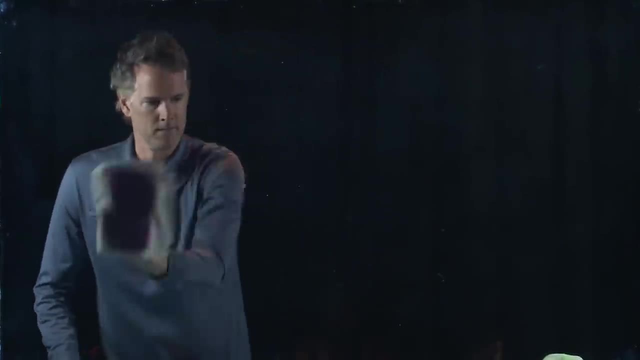 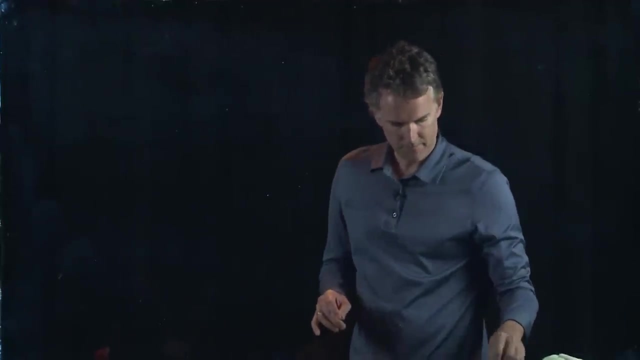 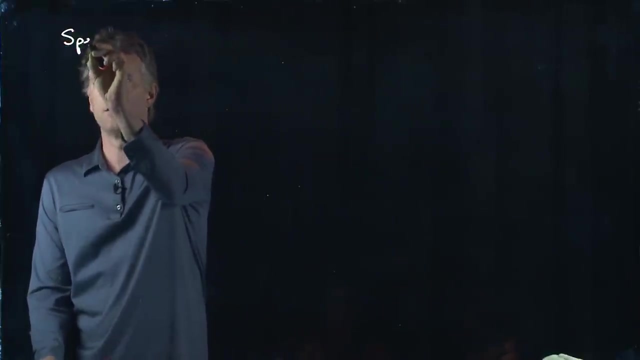 So one thing that we need to know is the speed of these E-M waves is going to be different. So one thing that we need to know is the speed of these E-M waves is going to be different. So one thing that we need to know is the speed of these E-M waves is going to be different. 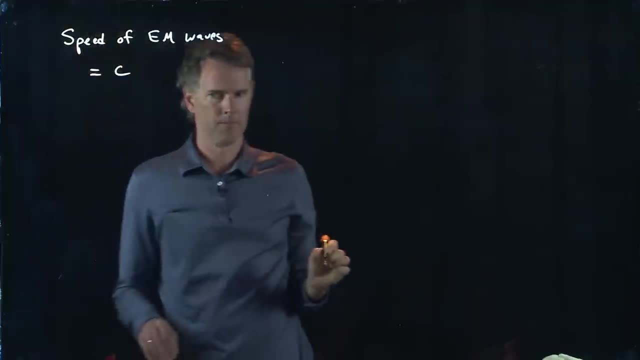 And the speed of these E-M waves is going to be different. Okay, so we have a 10 to the 8 meter per second, So the speed of this E-M wave was going to be equal to C, right, And C is 3 times 10 to the 8 meters per second. 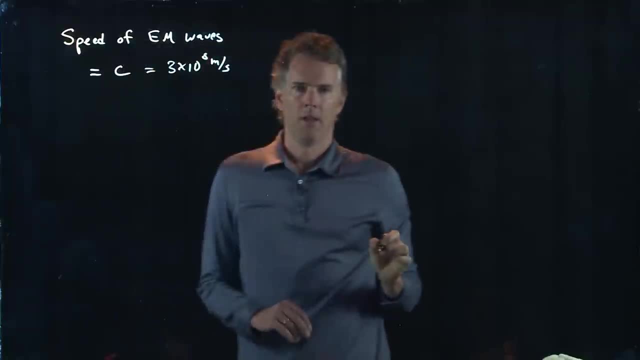 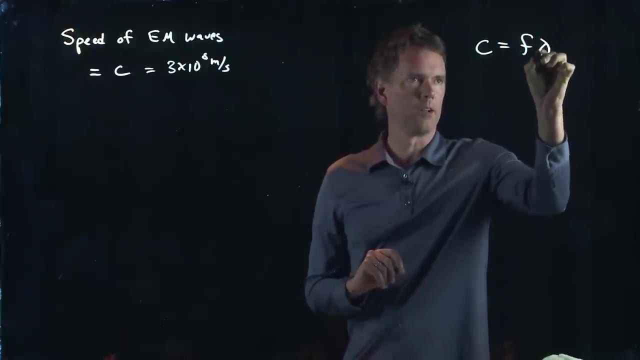 So the frequency of this E-M wave is going to be equal to the frequency of the current wave. The frequency of this E-M wave is equal to the efficiency of the current wave, which is the next constant. So if you look at this, 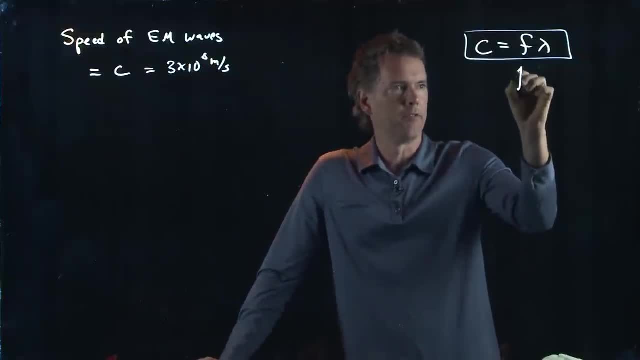 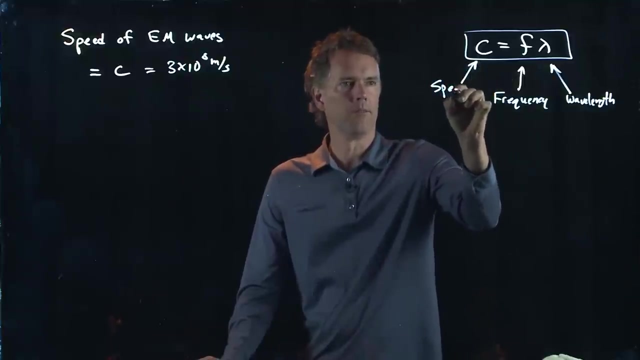 Let's go. we're going to do a function that will do that The whole thing. So let's do a function. Okay, All right, Okay, Good, All right. Lambda is the wavelength, C is, of course, speed of light. 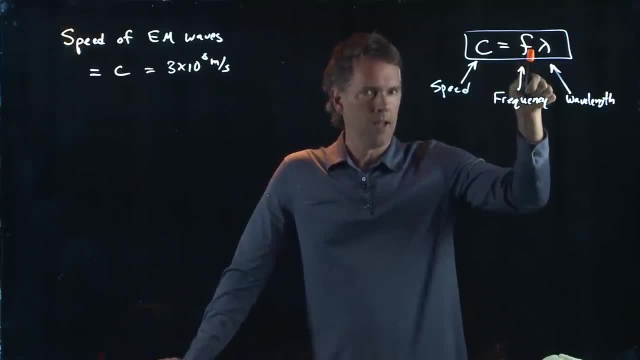 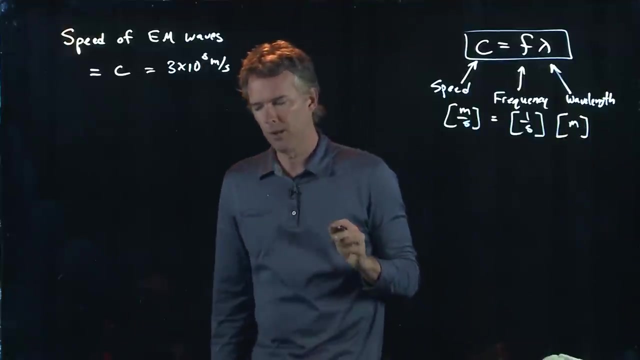 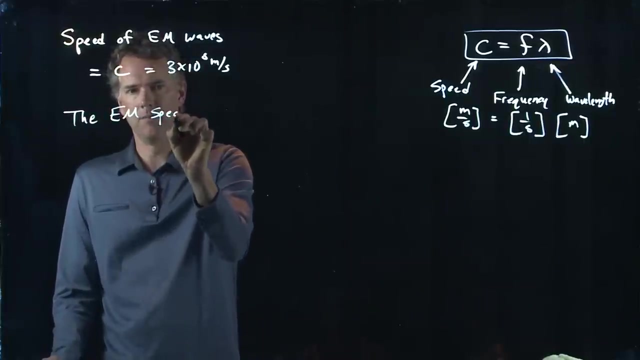 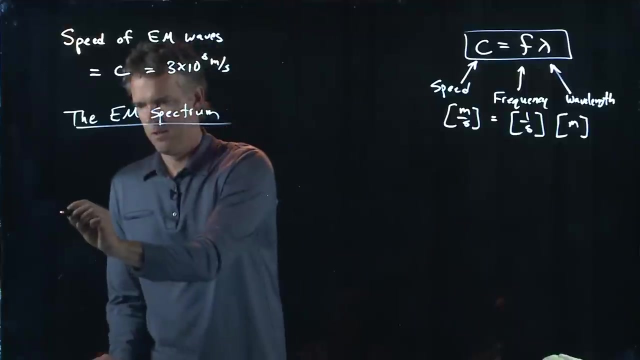 Okay, so meters per second is F, which is 1 over seconds times lambda, which is meters. Okay, so that's the relationship that we're dealing with, And now let's think about the full electromagnetic spectrum. So we have a big long line here. 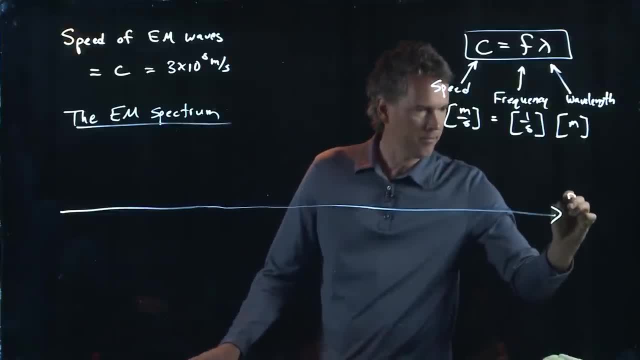 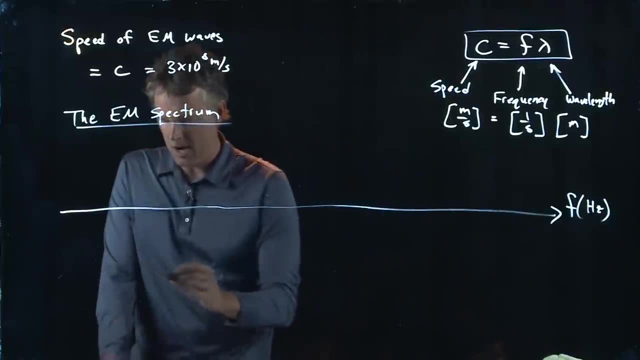 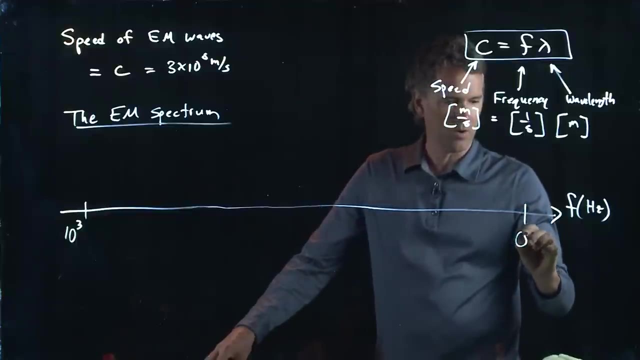 and let's label this one frequency F measured in hertz, And it's going to start down here at the low end, At something like a kilohertz, And at the high end it's going to go up to 10, to the 22 hertz. 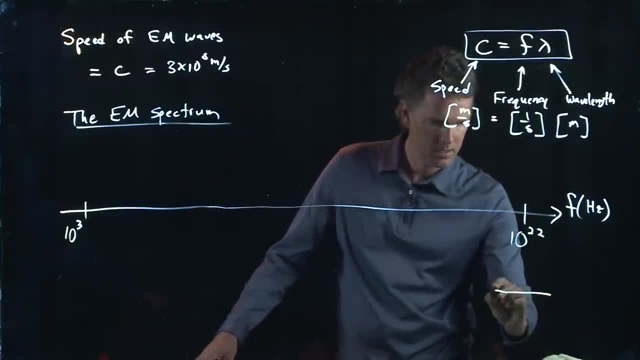 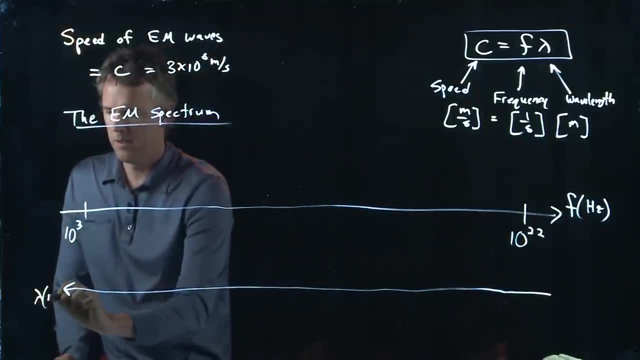 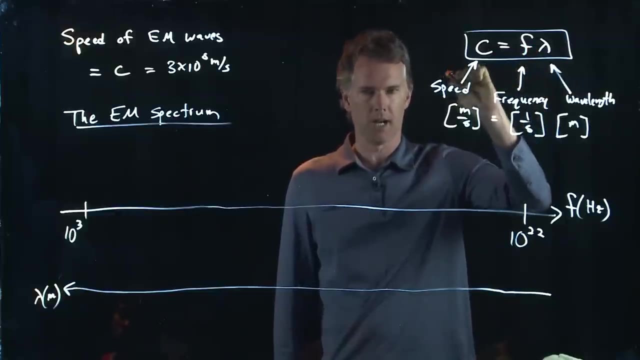 And then going the other way. we have lambda, And lambda is measured in meters. Those are inversely related, since C is a constant right. If F goes up, lambda has to go down. If F goes down, then lambda has to go up. 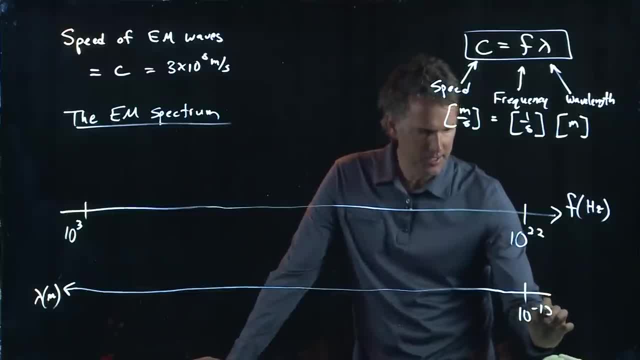 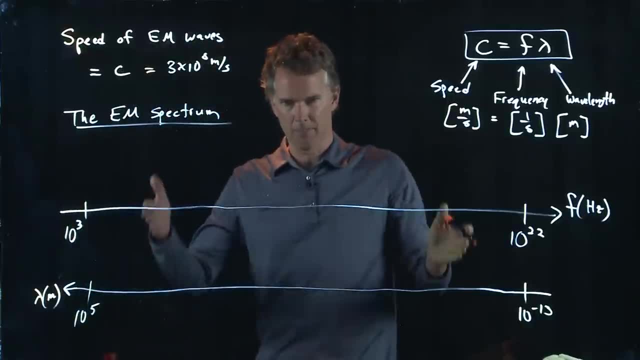 And this over here is on the order of 10 to the minus 13. And it goes all the way over to on the order of 10 to the 5.. Okay, so these things aren't going to line up perfectly well, but they're going to be roughly close. 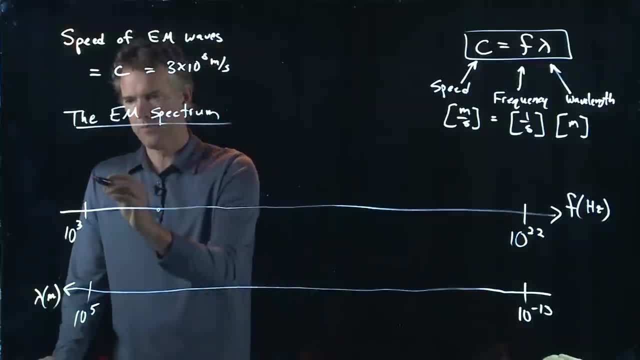 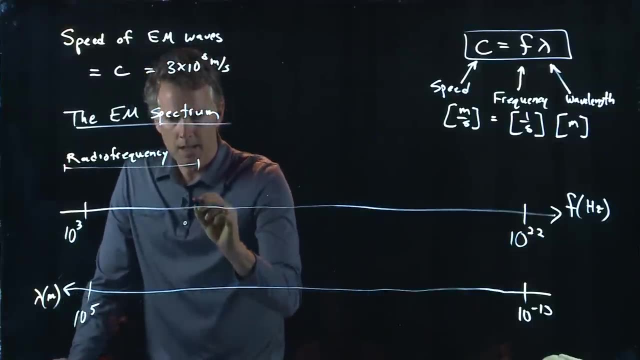 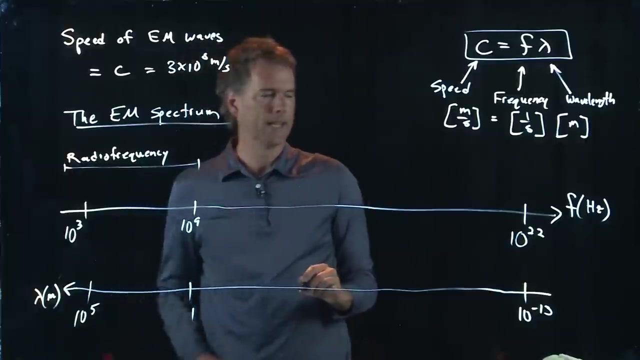 So down here at the low end of the spectrum, we have what is called the radio frequency, And the radio frequency extends up to about 10, to the 9 in hertz, or roughly 1 in meters. So radio frequencies contain, of course. 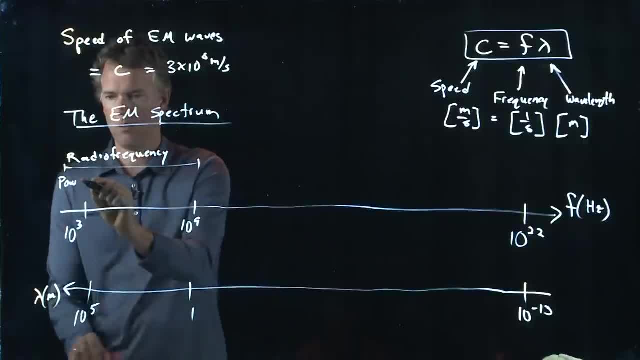 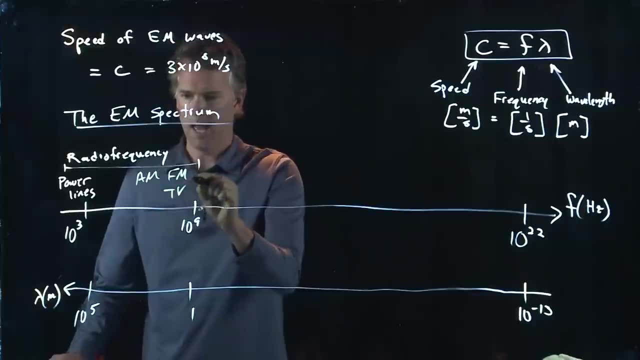 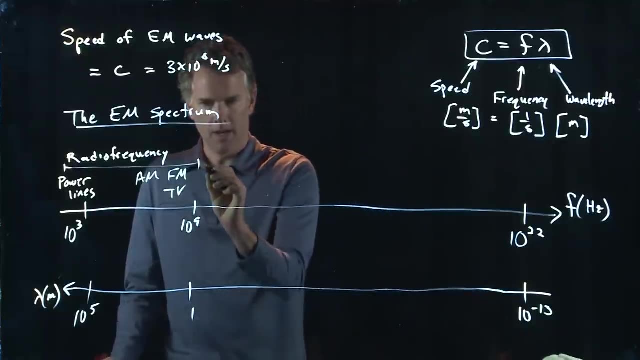 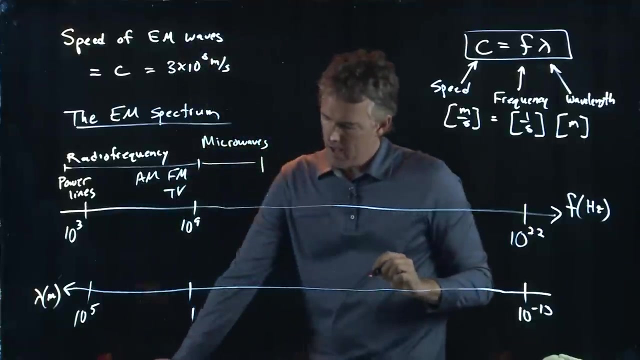 power lines way down here at the bottom end: AM radio, FM radio and television. Okay, these are all operating in the radio frequency. The next region is called microwaves, And microwaves are, of course, like your microwave oven. 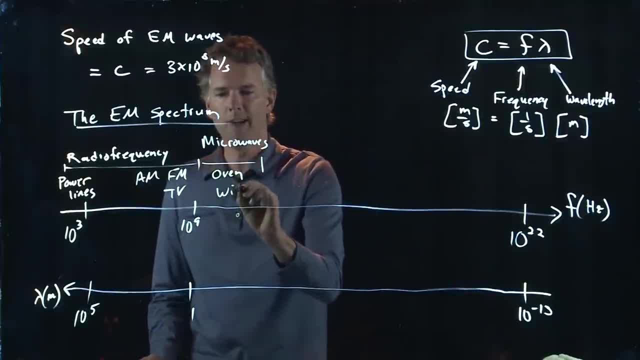 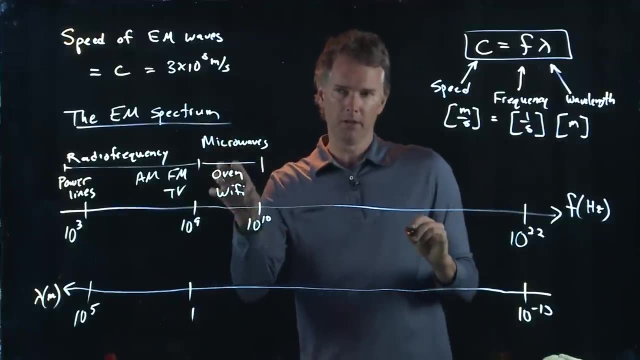 but also your Wi-Fi signals, And this is going to go up to on the order of 10 to the 10, or 10 to the 11.. Okay, so this is what we talked about in class. People are a little concerned about cellular phones. 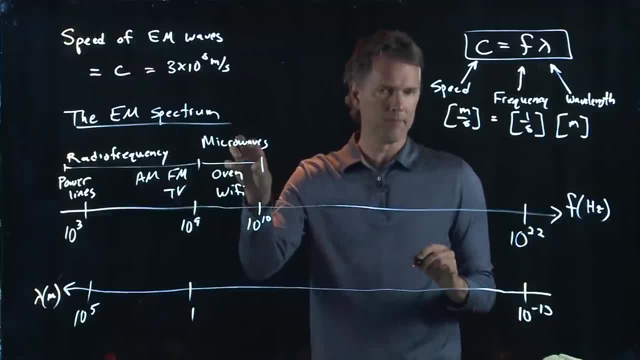 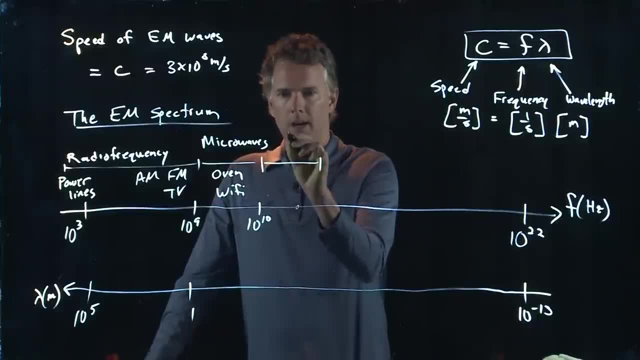 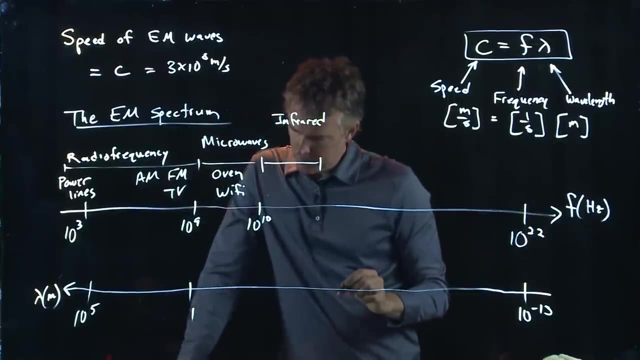 and Wi-Fi signals, because it's really close to the same frequencies that you use for your microwave oven to heat your food. After that we get infrared. Okay, infrared goes up to about 10 to the 14.. 10 to the 13,, 10 to the 14, somewhere in there. 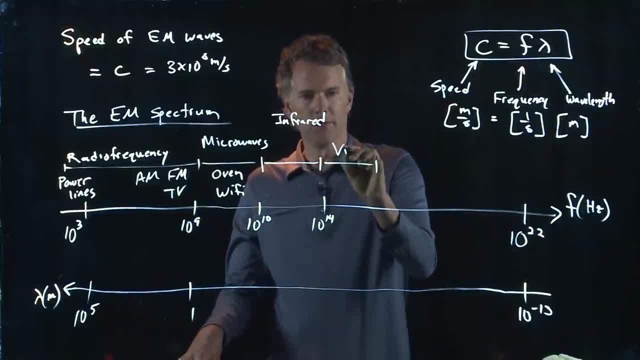 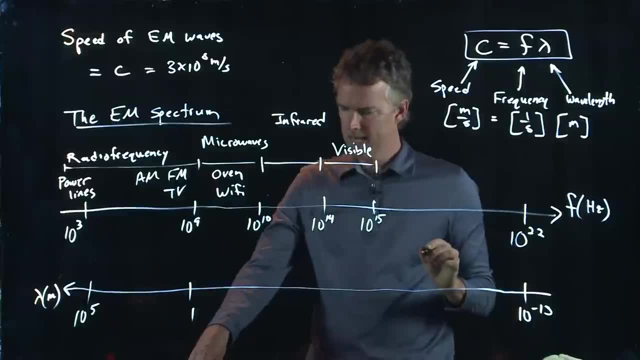 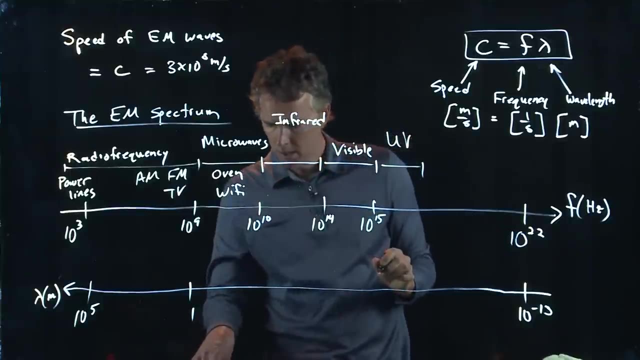 And then, after infrared, we get to visible, And visible goes from 10 to the 14, up to about 10 to the 15.. If we keep going to higher frequencies, we get to UV. UV gets up to about 10 to the 16.. 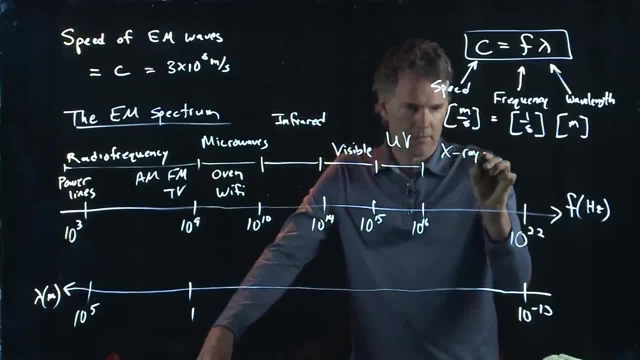 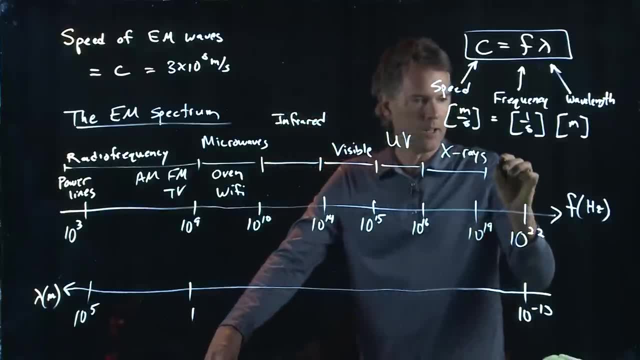 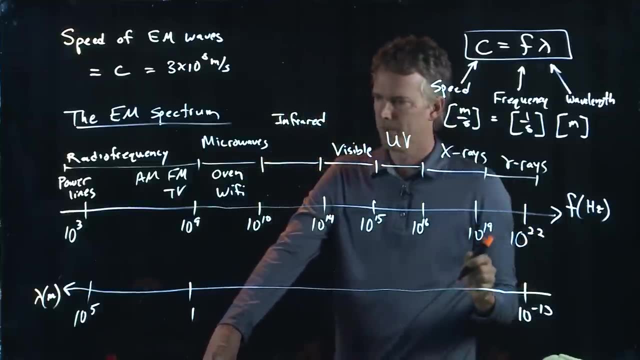 And then we get to. we get to X-rays. X-rays go all the way up to about 10 to the 19.. And then the very last bit is something called gamma rays, And gamma rays can go as high as 10 to the 22.. 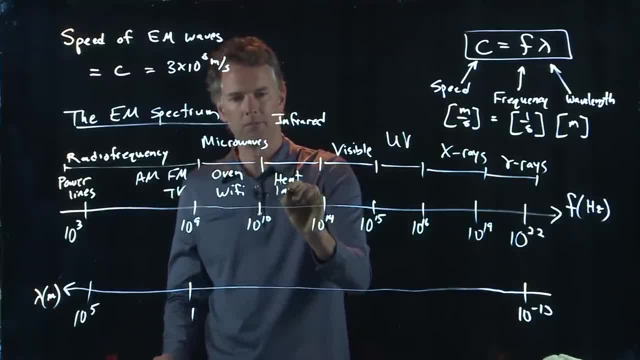 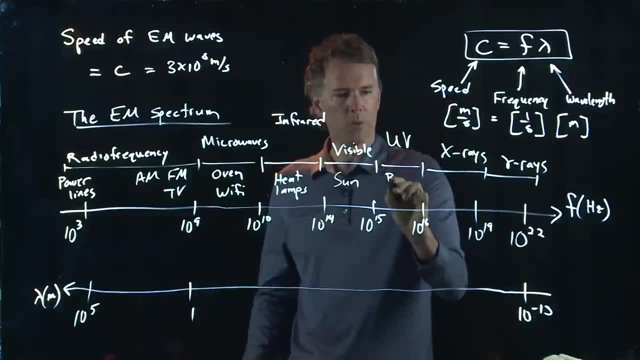 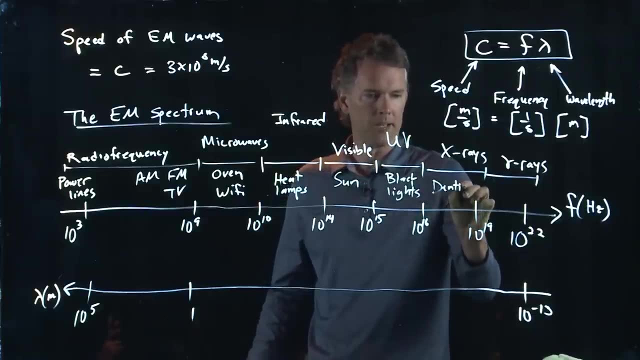 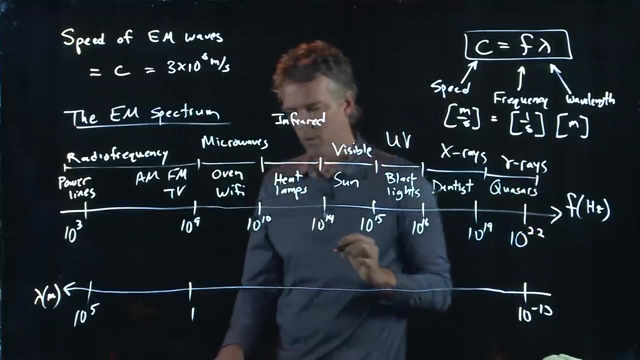 So infrared, that's stuff like heat lamps. Visible is, of course, the sun. UV would be black lights. X-rays you get when you go to the dentist. Gamma rays you only get from objects like quasars. Okay, And on the scale here, 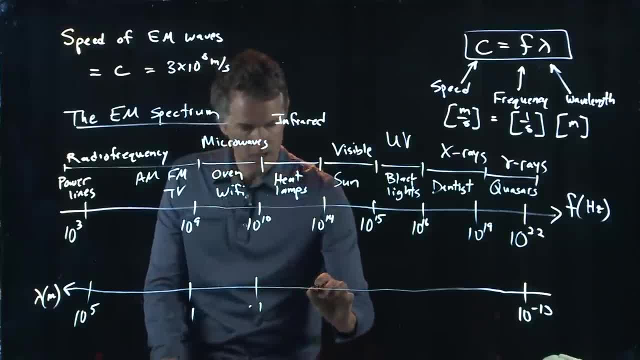 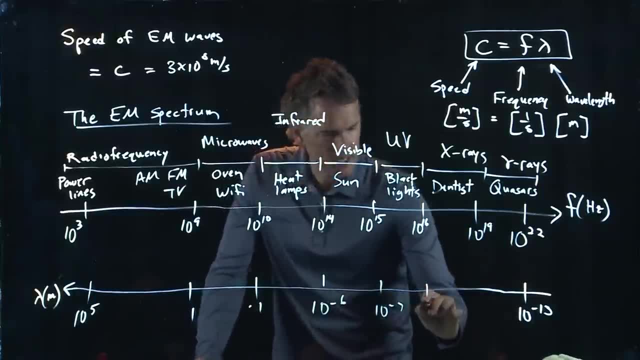 10 to the 10 corresponds to about 0.1.. And then we get to 10 to the minus 6 up here and 10 to the minus 7. And 10 to the minus 8. And 10 to the minus 10.. 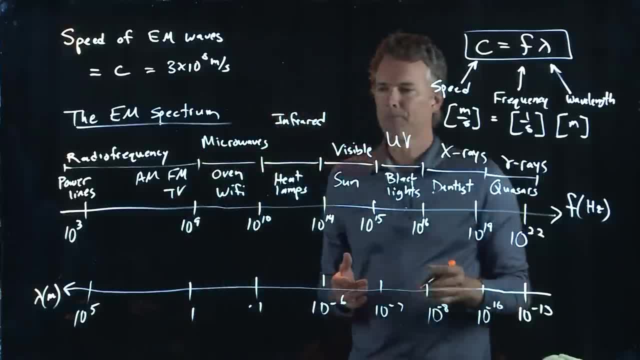 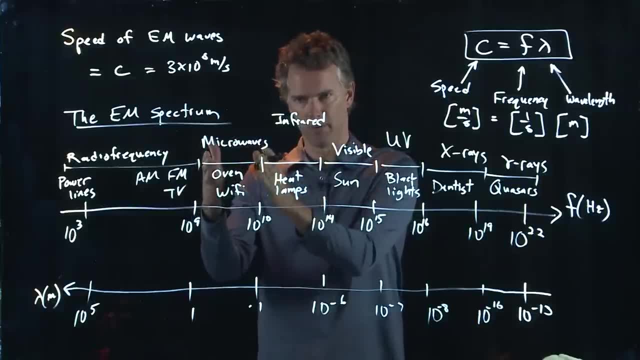 And so on. Okay, These numbers aren't going to match up exactly And in fact these divisions are not precise. Okay, They just say this region is microwaves, But nobody says this is the hard cutoff for the microwaves on the right side. 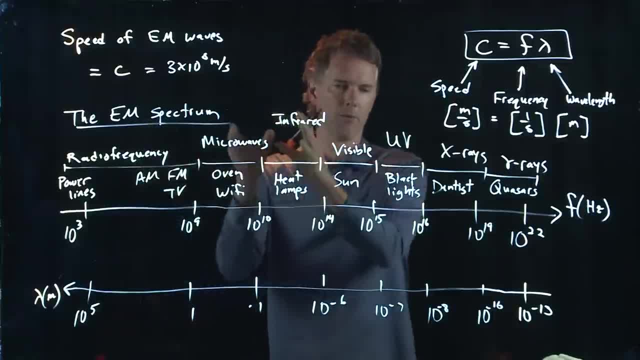 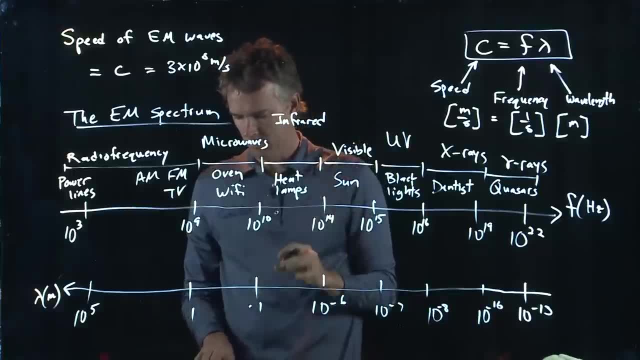 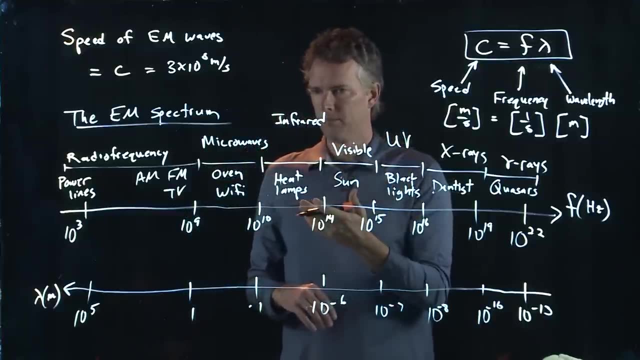 and the hard cutoff on the left side. Okay, These are general regions, except with regards to visible. Okay, Visible we describe in exquisite detail And that's largely because we operate on the visible wavelengths. Remember, we asked that question a second ago. 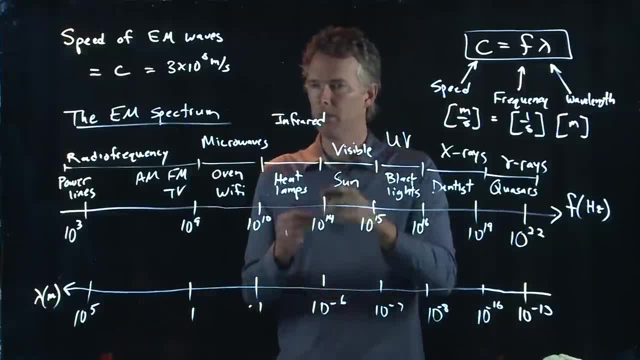 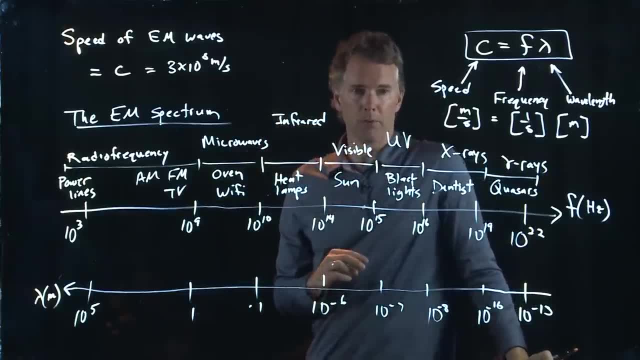 How do you detect electromagnetic waves? Well, you can use your car antenna and detect radio frequency waves. But if you want to detect visible light, how do you do it? How do you guys detect visible light? You're doing it right now. right. 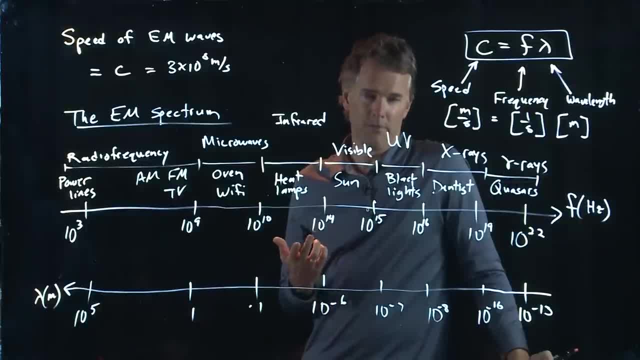 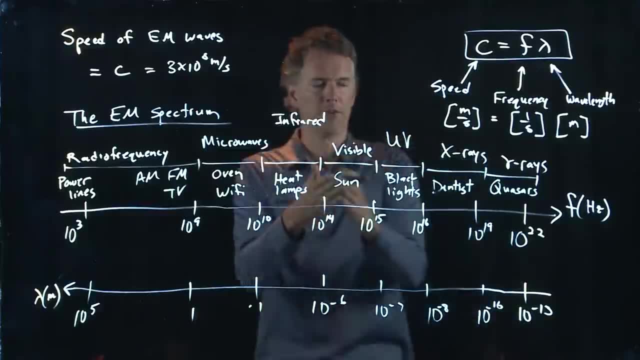 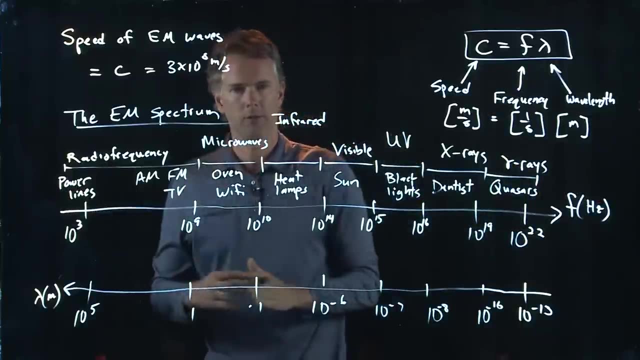 You use your eyeballs, Visible light is what you see. That is the light that you see, And it's sort of interesting that there's this huge range available and it's all electromagnetic waves, All the way from gamma rays down to radio frequency waves. 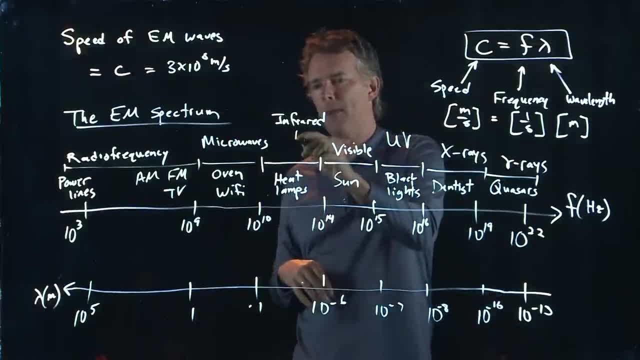 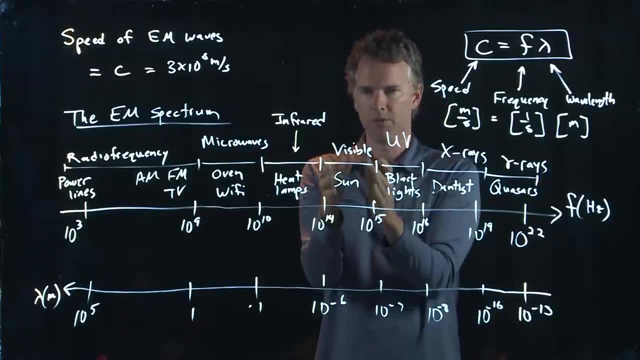 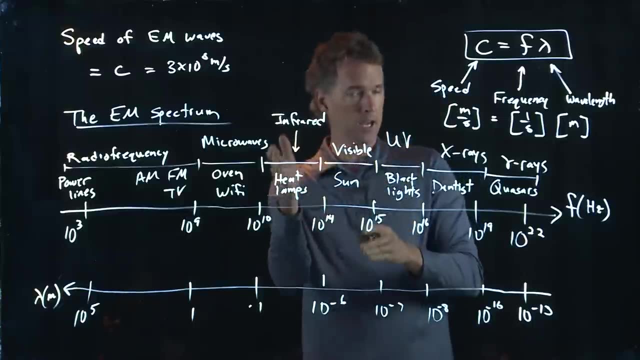 It's all the same stuff. It's all electromagnetic waves, But we only detect visible, Which is a really small portion of the spectrum. If somehow you could detect UV and infrared and x-rays and microwaves, you could see a lot more of what's happening in the world. 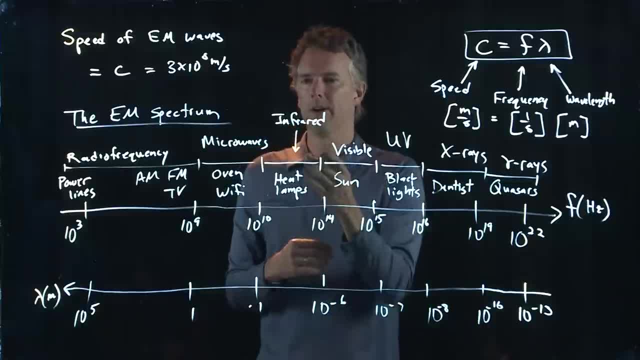 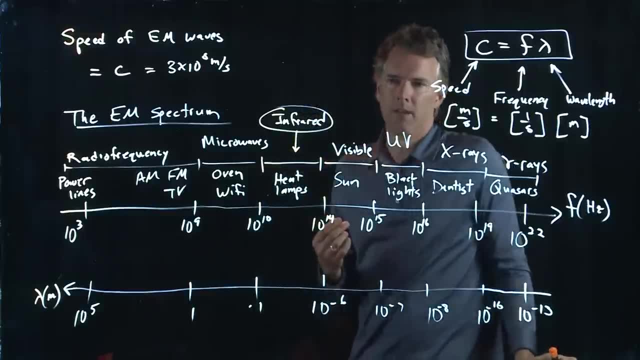 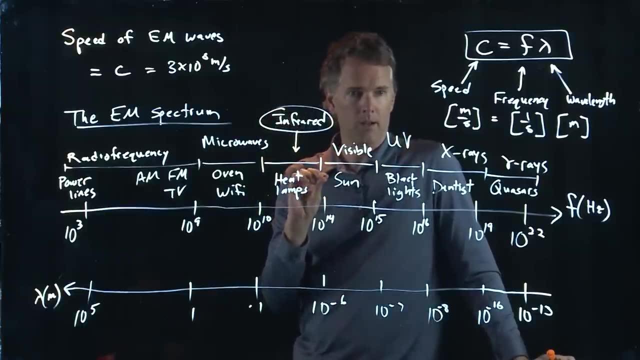 And, in fact, you're familiar with one area, which is this right here: Infrared, Because you've all seen the Arnold Schwarzenegger movies where they use infrared, Infrared goggles, Which is adapted from the military, And the idea is you can detect infrared waves. 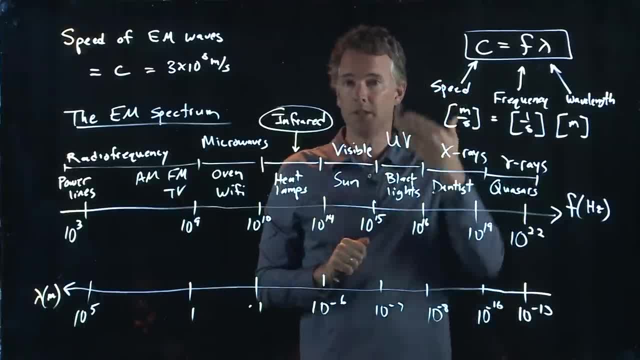 and if you have a special device- infrared goggles- you can turn it to visible, And so now you can see things out there that are emitting infrared light even though they're not emitting any visible light, And this is kind of weird, right. 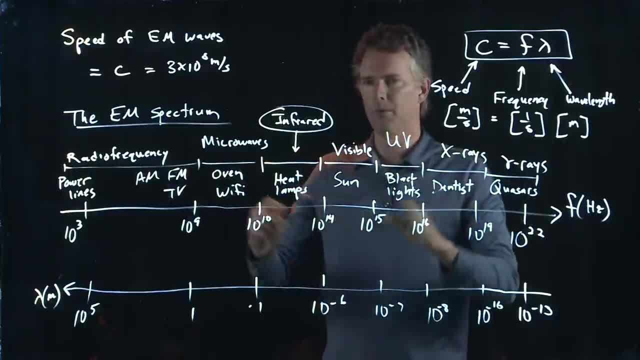 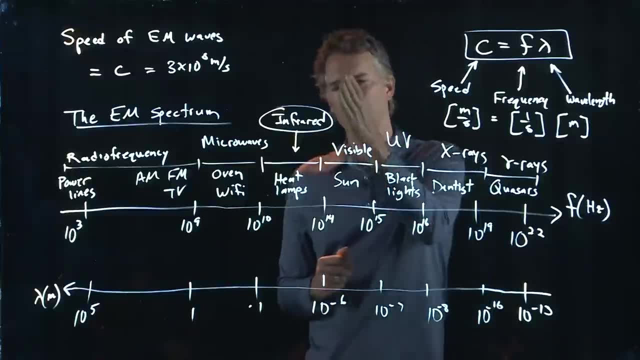 Because if we turned off all the lights in this room and turned off the board, you guys would be in the dark And if I looked at you I can't see you. But if I could look at you with my infrared goggles, all of a sudden I would be able to see you. 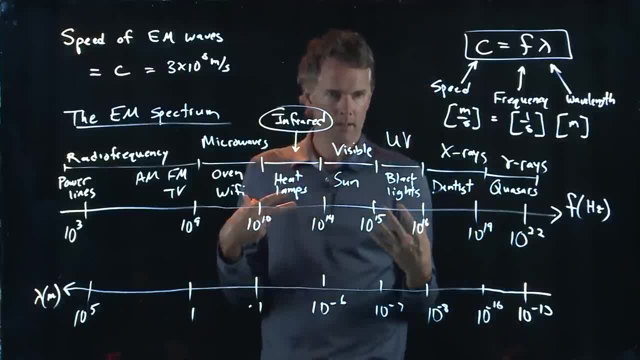 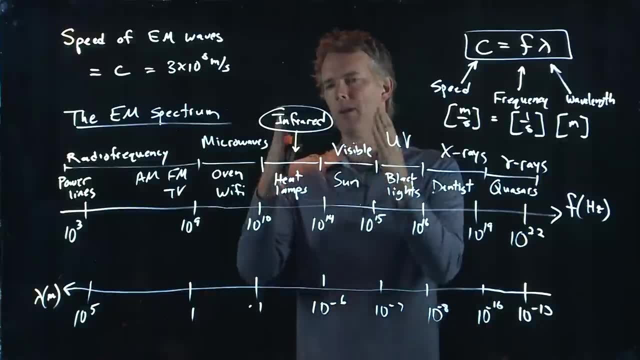 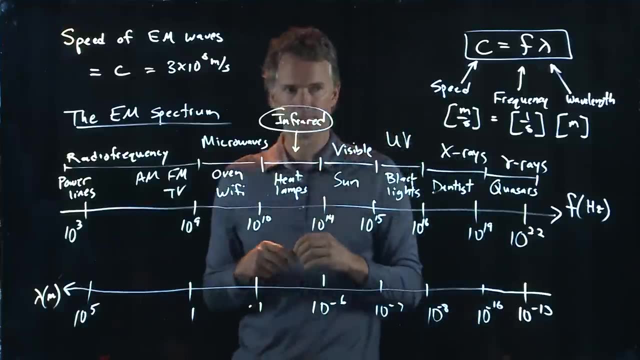 Because, as humans sitting here emitting light, it's in the infrared region. You're at a temperature of 98.6 degrees. You are emitting light that is about 10 microns long, And so with my goggles I'd be able to see you. 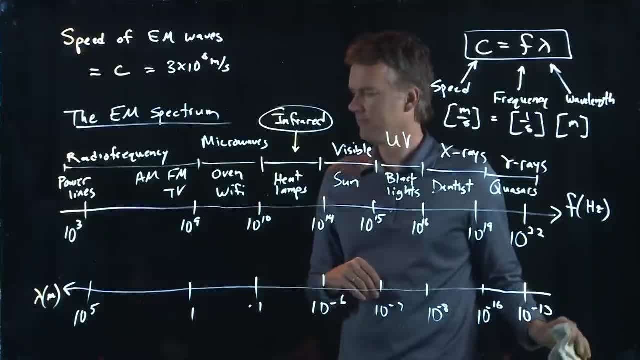 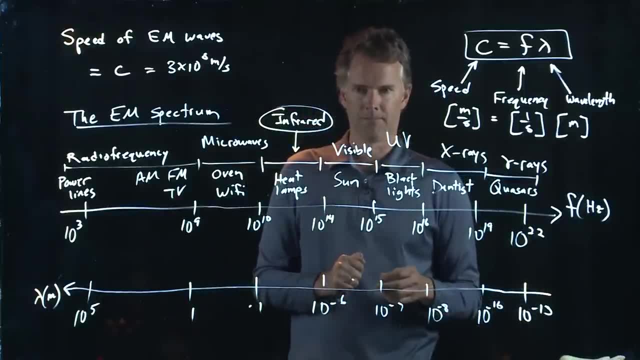 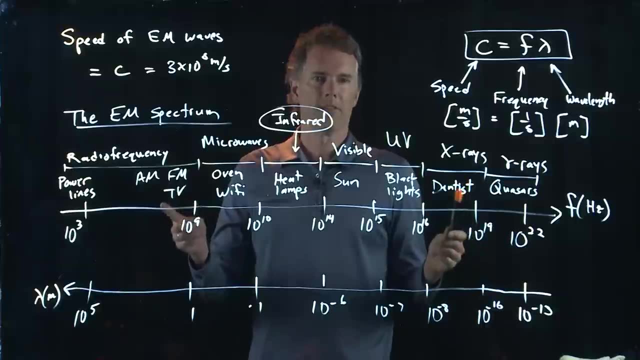 Maybe I'll bring some in. We'll try that sometime, Maybe it'll be good. Okay, Questions about this electromagnetic spectrum. All right, There's one other point that I wanted to make, and this is something that we're not going to see a lot of. 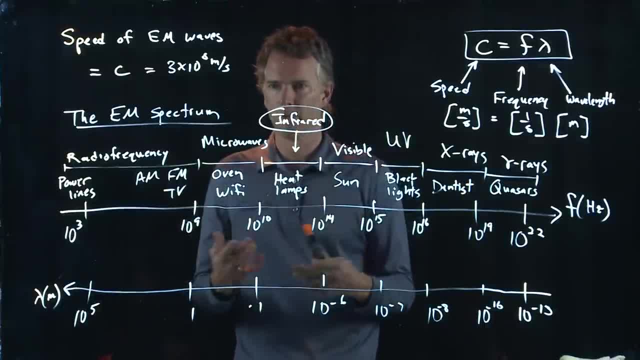 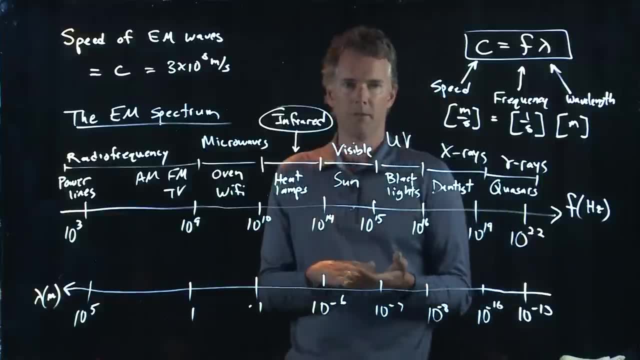 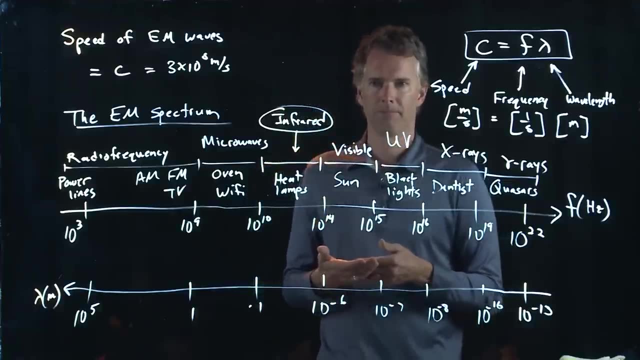 in this class, but I wanted to give you a taste for where you might be going in your physics education, which is this idea of quantum physics. Has anybody ever heard of the wave-particle duality in quantum physics? Okay, There's this notion in quantum. 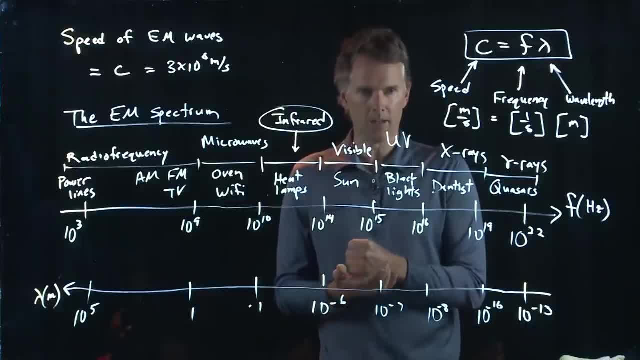 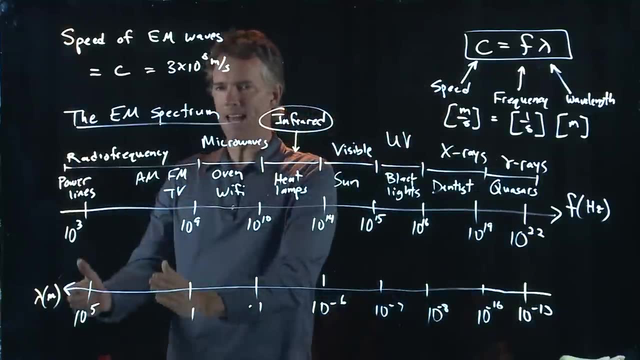 that everything behaves like a wave and a particle simultaneously, Even things like electrons. they're not really just point particles, They also have this wave-like property to them, And it turns out that when you're looking at this end of the electromagnetic spectrum, 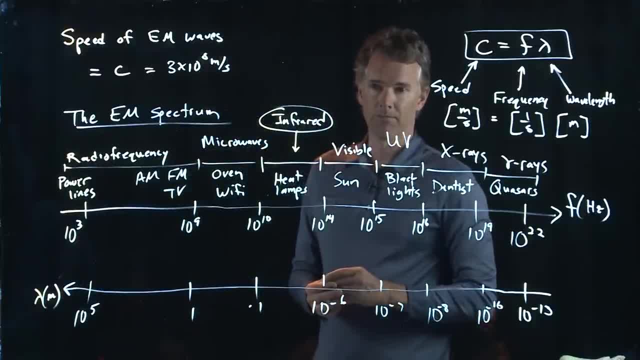 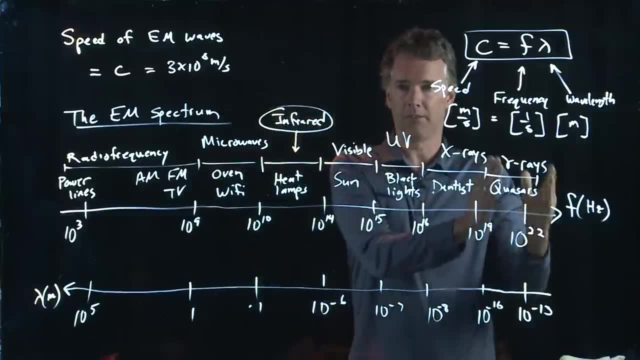 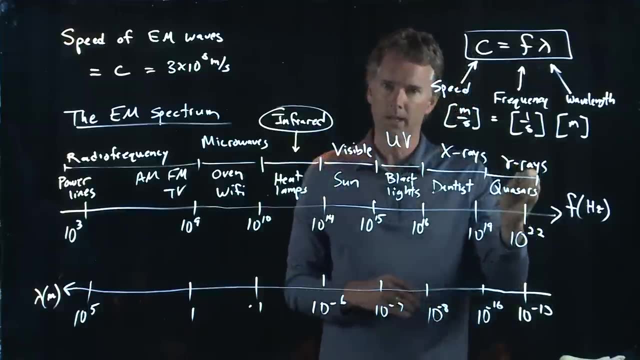 everything behaves like waves. Everything looks like a wave. It doesn't look like a particle. But up at this end of the spectrum, everything behaves like a particle. It doesn't behave like waves. So gamma rays really act like little tiny bullets. 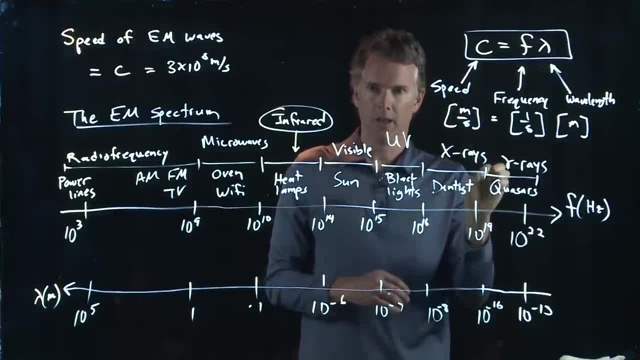 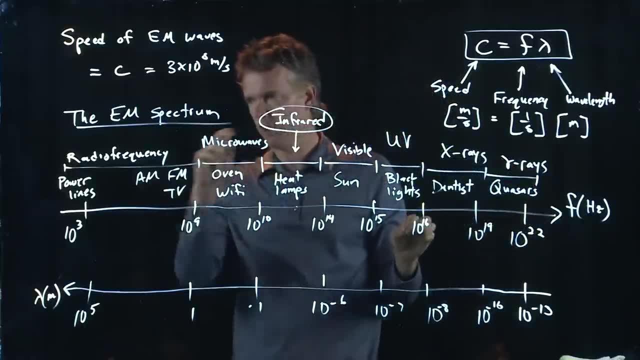 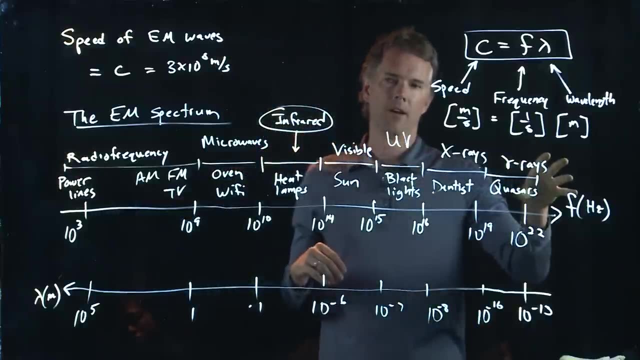 little particles just flying through the universe. It's very hard to discern any wave-like property At this end And it's very hard to discern any particle-like properties at this end. So at either end you have waves over here and particles over here. 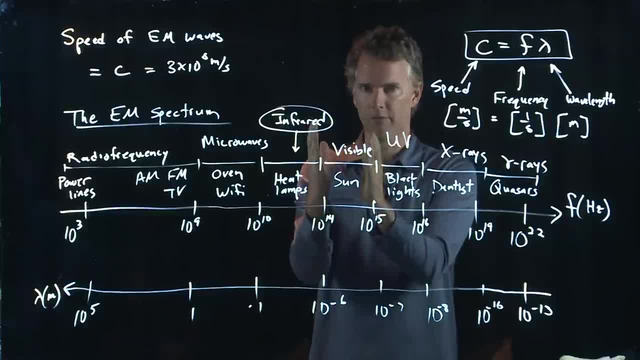 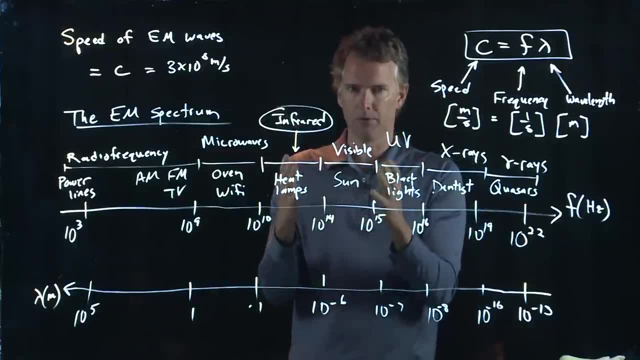 But where we sit in the middle in this visible spectrum, light acts like a wave and a particle, And this is the basis for the wave-particle duality, And light in this region has been shown to behave like both Simultaneously. 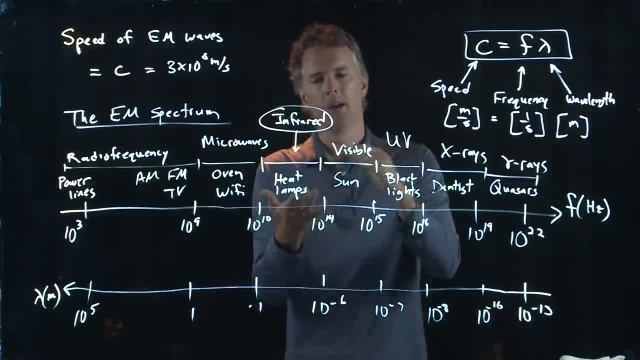 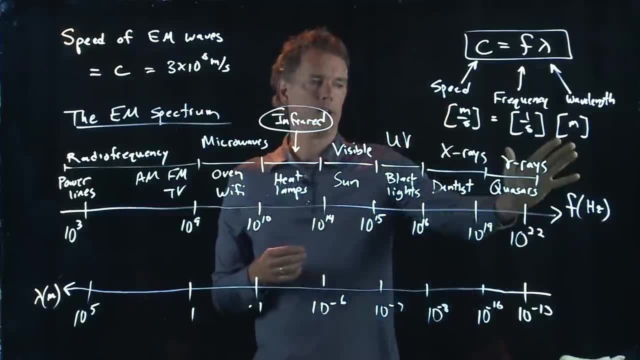 Depending on how you design your experiment. you might look for the wave properties, Different experiments, you might do the particle properties, But over here at gamma rays, particles, Over here at radio waves, it's waves. So it's kind of interesting. 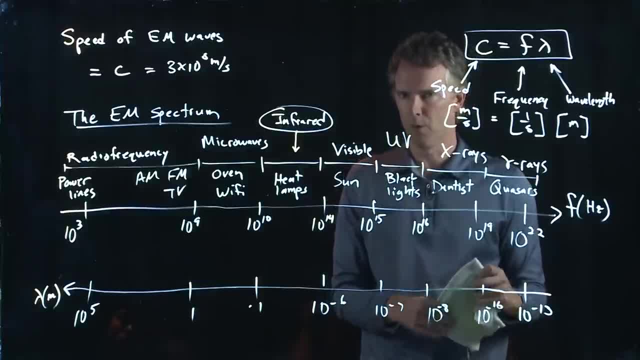 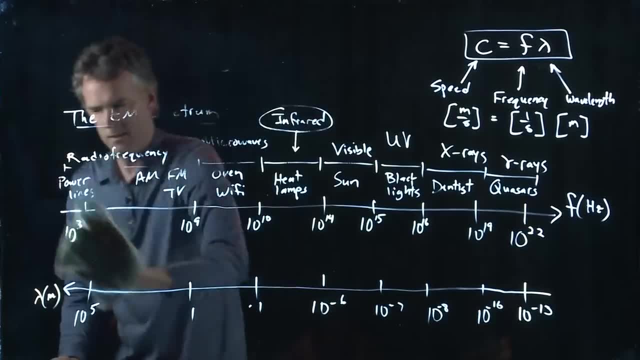 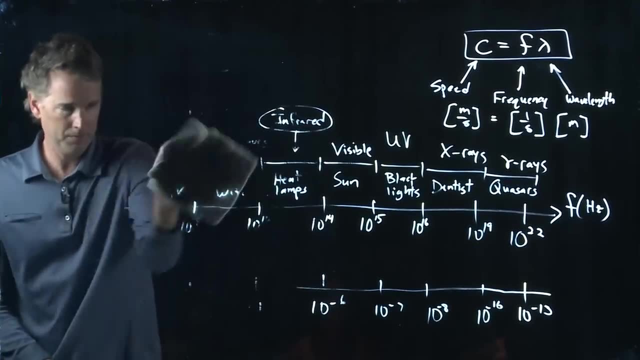 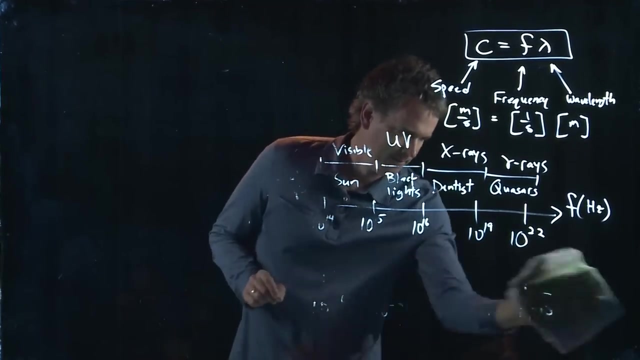 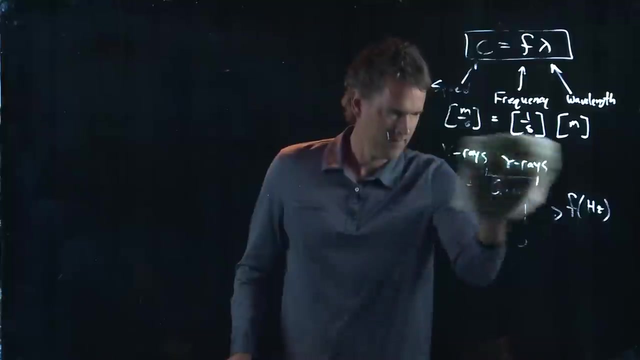 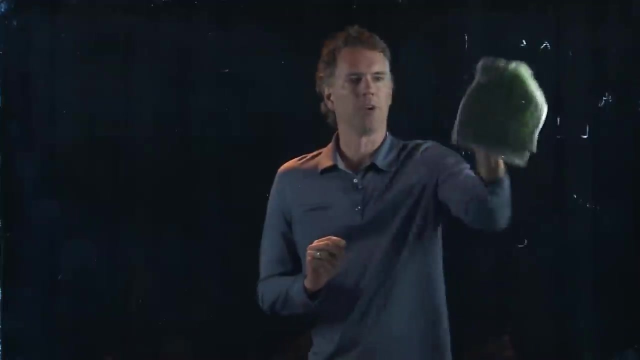 And we'll learn more about that when we get to a bit of quantum physics. You guys have any questions up to this point. Why don't we see if we can pull up one of your next chapter's homework problems And we'll take a look at one that is. 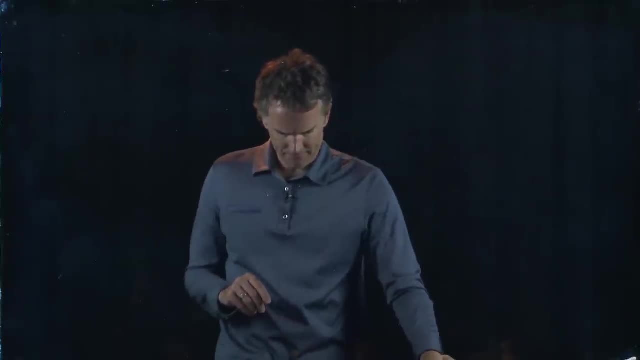 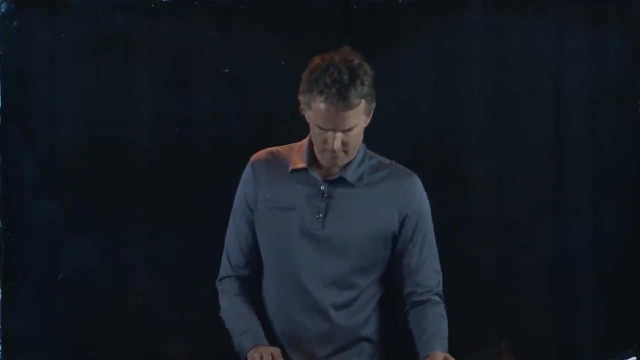 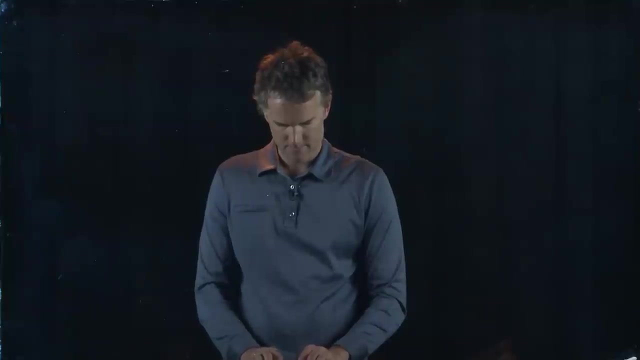 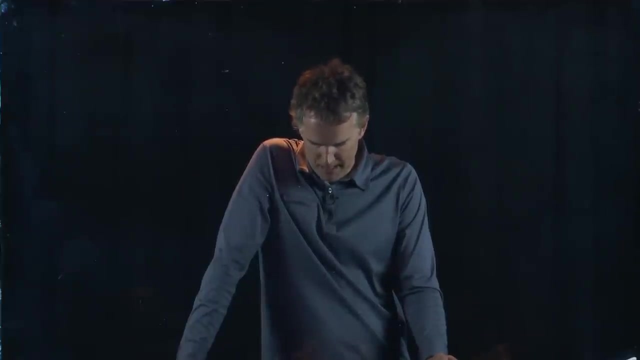 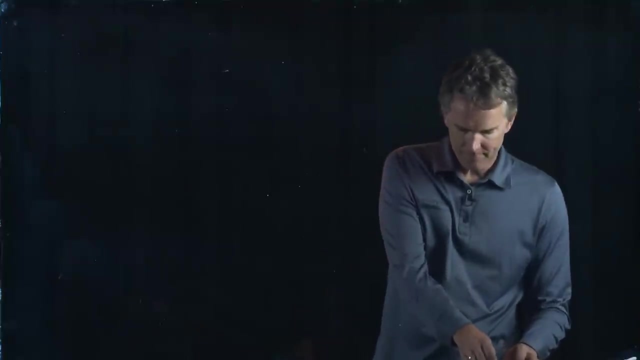 hopefully relevant. I just posted this this afternoon, So it's up on mastering. It's due Friday night And let's take a look at- Let's look at- 22.07.. Okay, so in this one it says the following: It says: 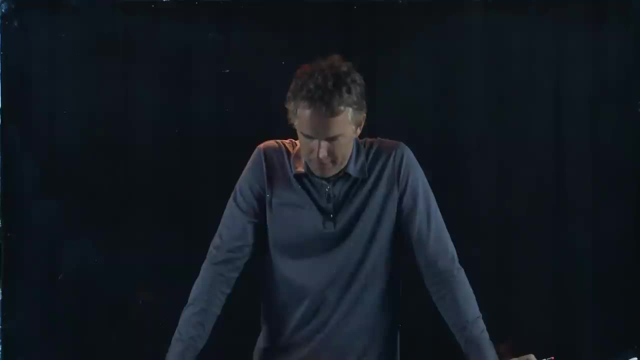 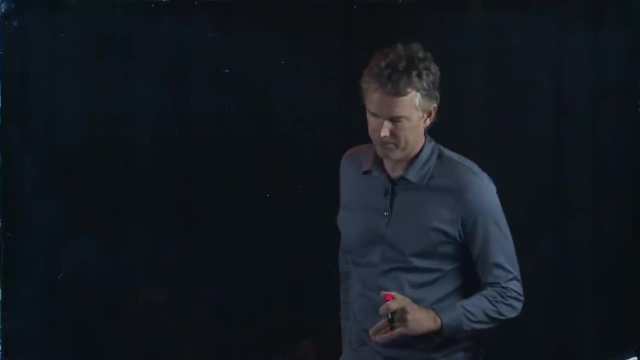 In an electromagnetic wave traveling west. the B field oscillates up and down vertically and has a frequency of 93 kilohertz and an RMS strength of 7.15 times 10 to the minus 19.. So let's assume that the wave travels in free space. 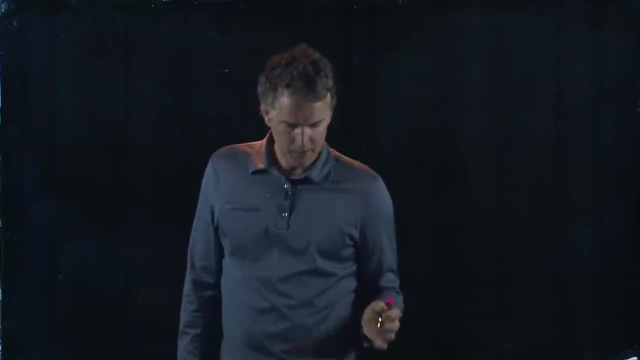 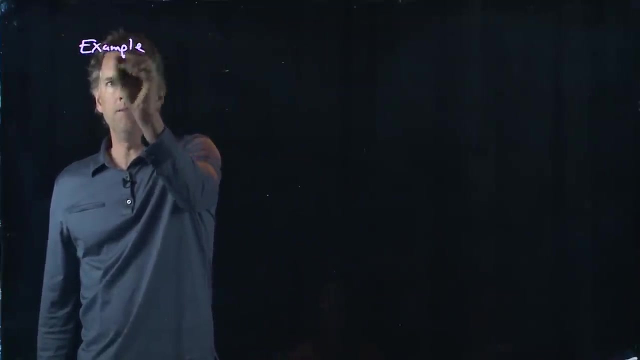 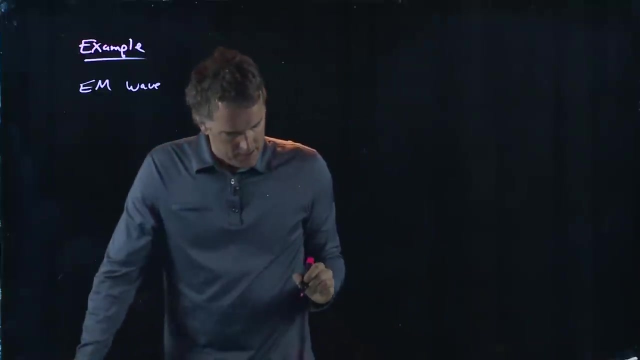 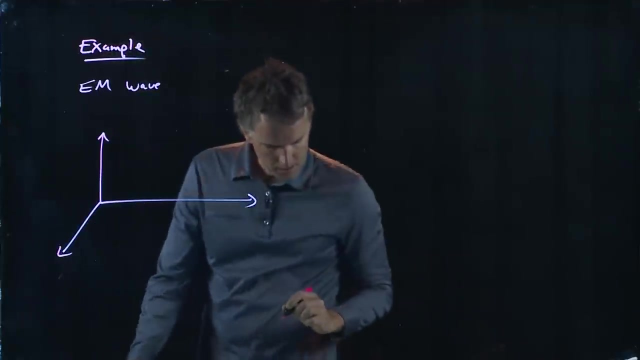 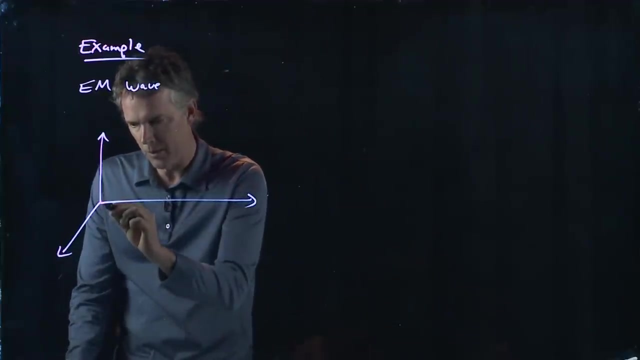 And part says What is the frequency of the electric field? Okay, so let's start with part. And we have an electromagnetic wave And it says that we're going to describe the B field And the B field that we drew before was going in and out of the board. 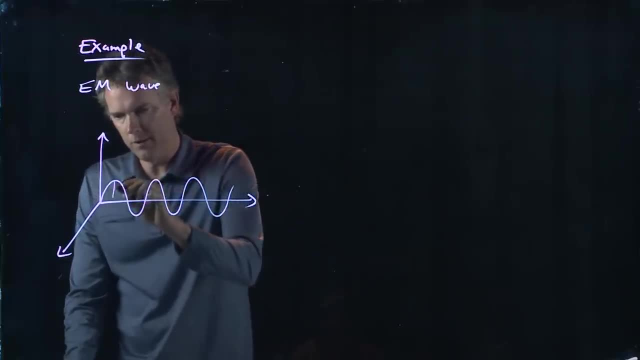 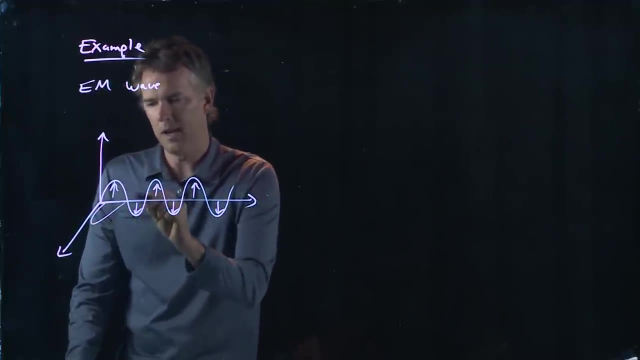 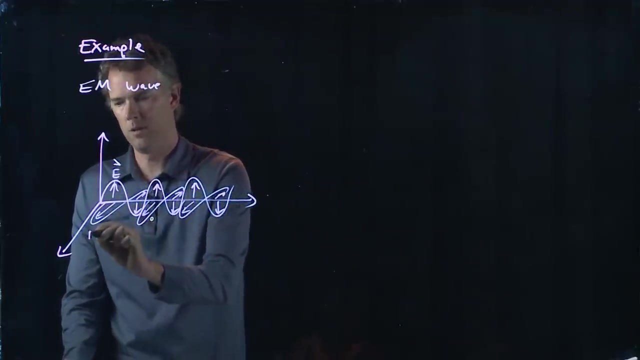 So let's draw the whole thing again. Here was our E field going up, going down, going up and down, And the B field was coming in and out of the board. Okay, E going up, B like that. So the first thing they tell us is: 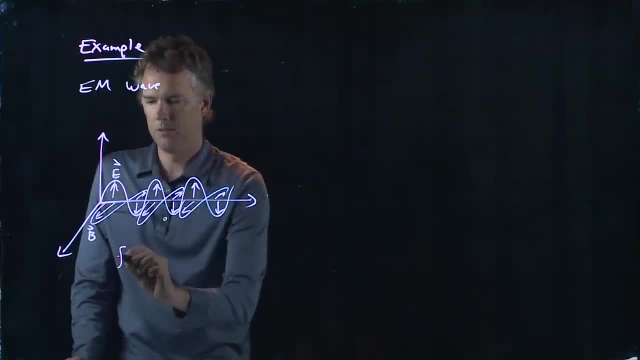 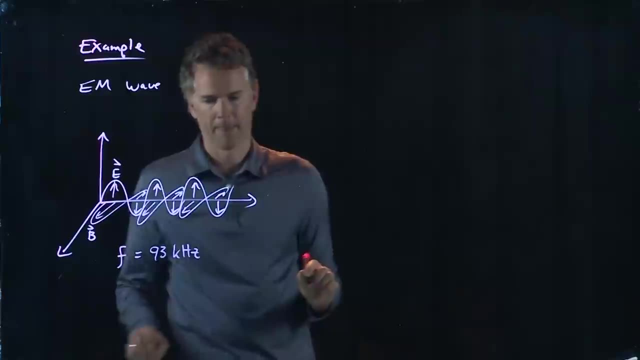 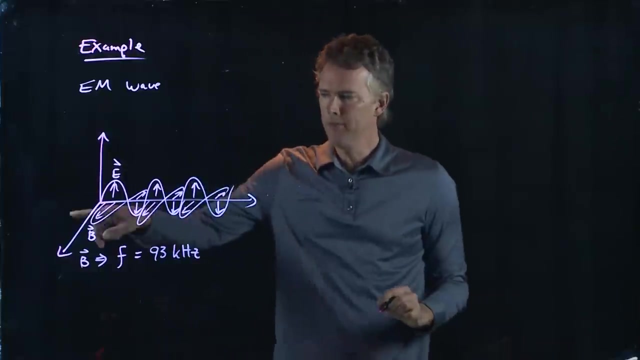 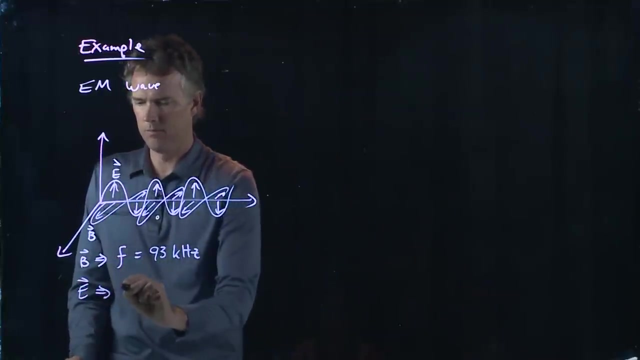 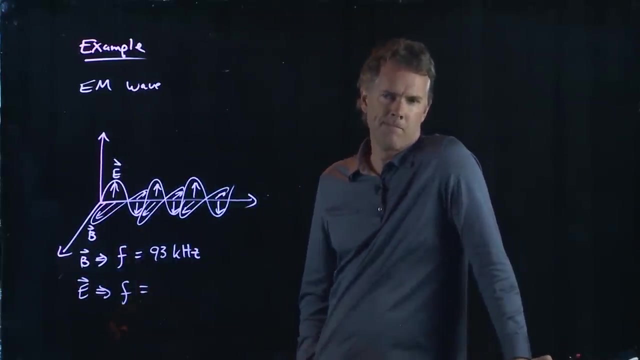 the B field oscillates with a frequency of 93 kilohertz. So if the B field is oscillating at 93 kilohertz, what do you think the frequency of the electric field is? What do you think It's got to be the same right. 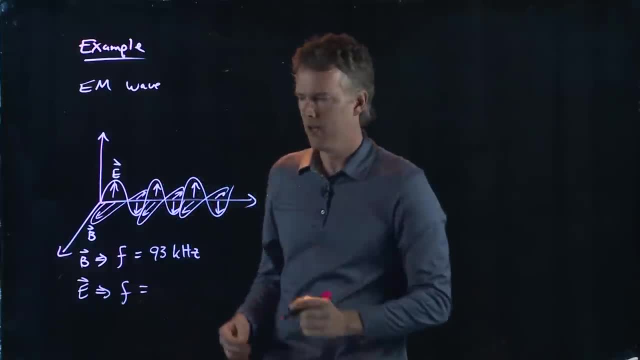 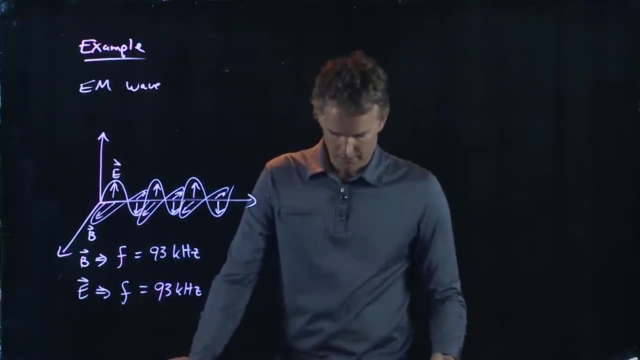 I mean, look at the picture: E is going up and down at exactly the same rate as the B is going. So this has to be 93 kilohertz as well. All right, let's try it 93,. let's see if it'll take a kHz for our kilohertz. 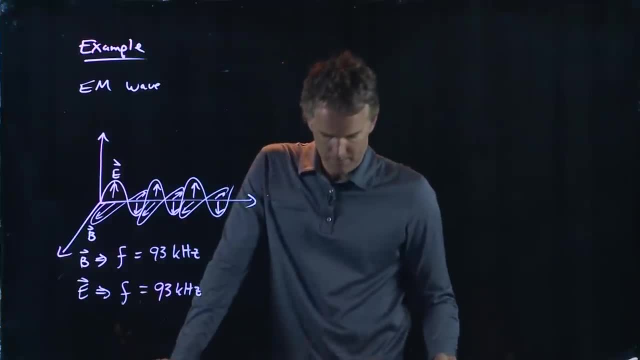 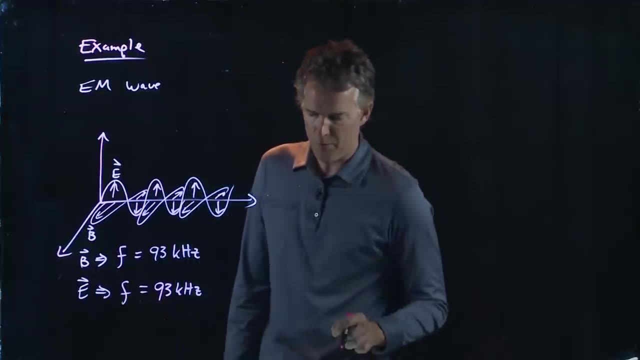 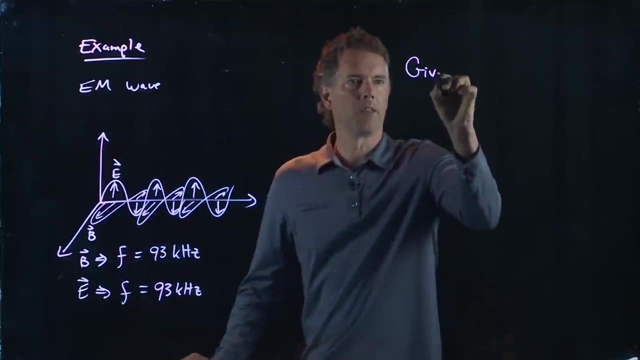 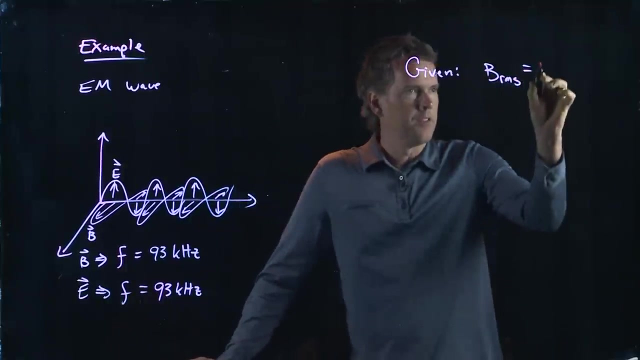 And in fact it does And it says we are correct. All right. part B says what is the RMS strength of the electric field? And what they gave us was the strength of the B field, RMS, And they told us it was 7.15 times 10 to the minus 9.. 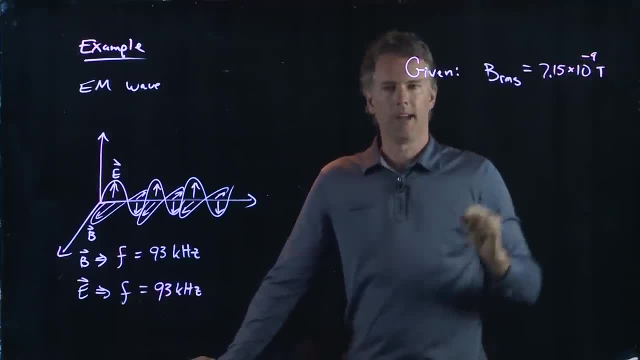 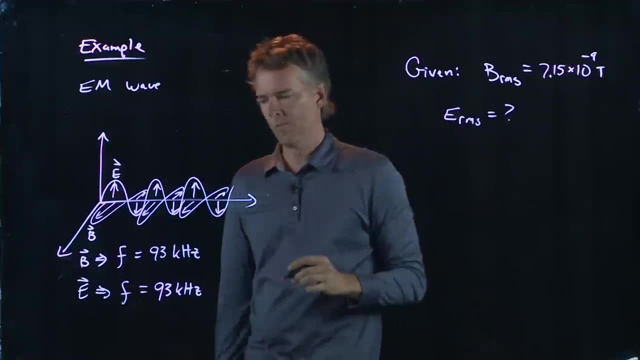 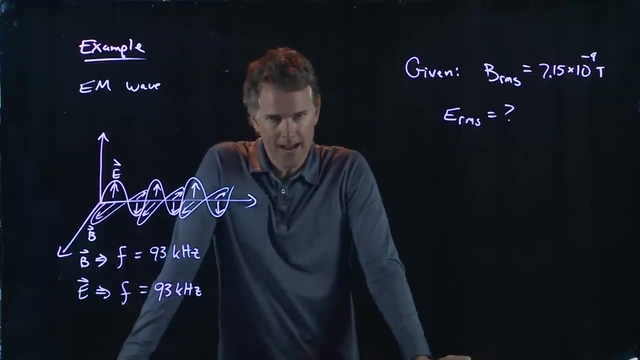 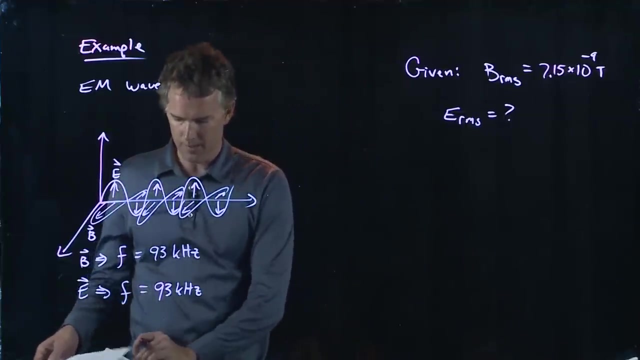 Okay, Tesla, And so now we're looking for E, RMS. Hmm, Well, we're not really sure how E relates to B yet, But if we push forward a little bit in the discussion, there is a very nice and simple relationship between E and B. 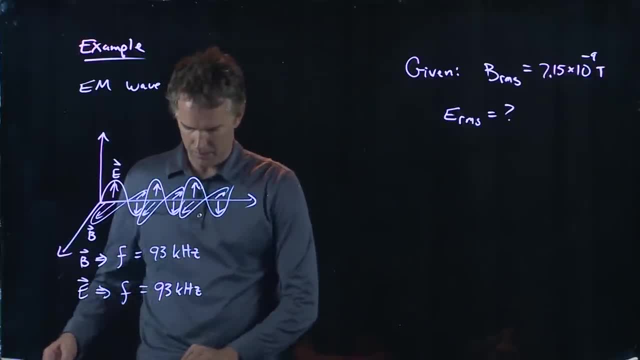 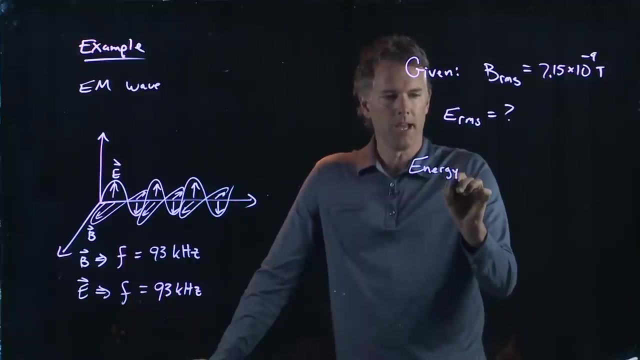 And let me Pull it up here- And this is going to be a little bit ahead of ourselves, but we'll get back to it in a second- What we can say is the following: The energy in the E field is, in fact, equal to the energy in the B field. 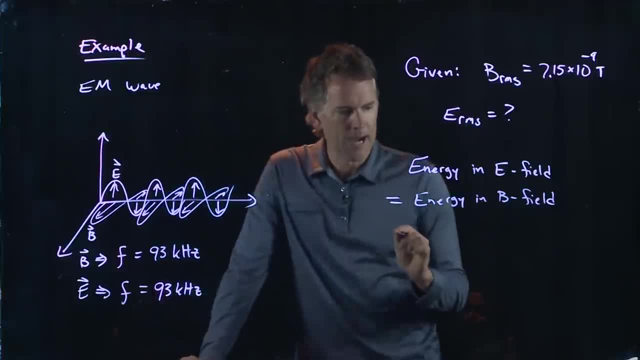 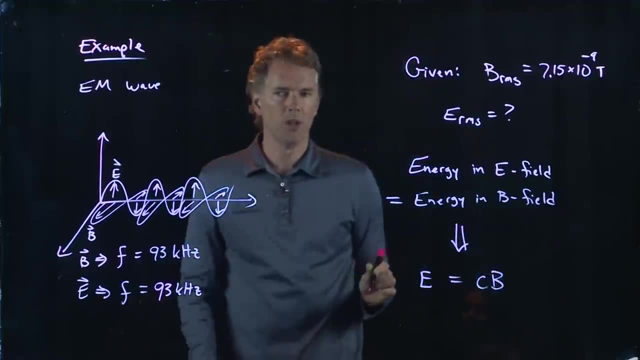 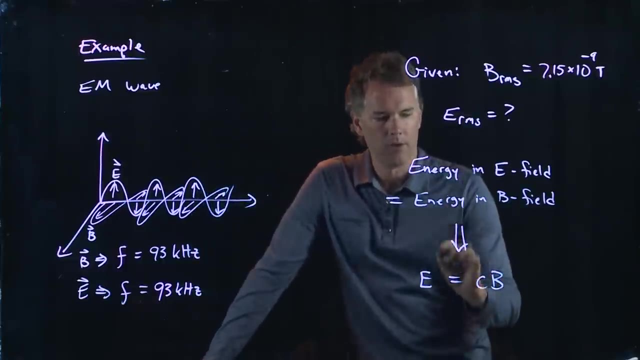 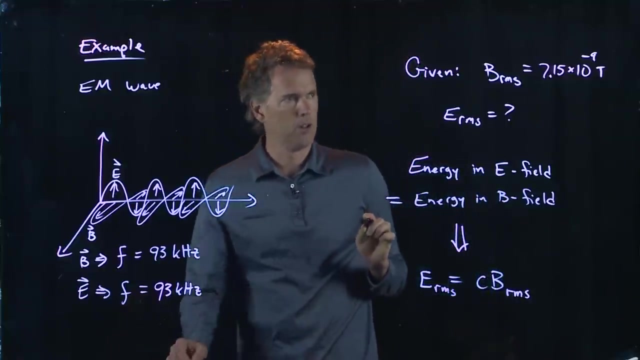 And those things relate to each other by the speed of light. So what is the electric field? It's equal to C, the speed of light times the B field. Okay, So E RMS is just equal to C times B RMS. So if I take this value of B, 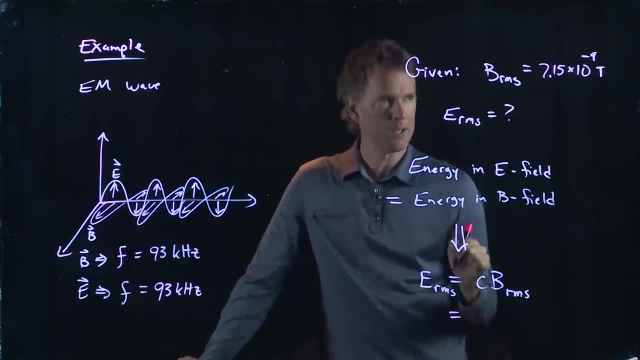 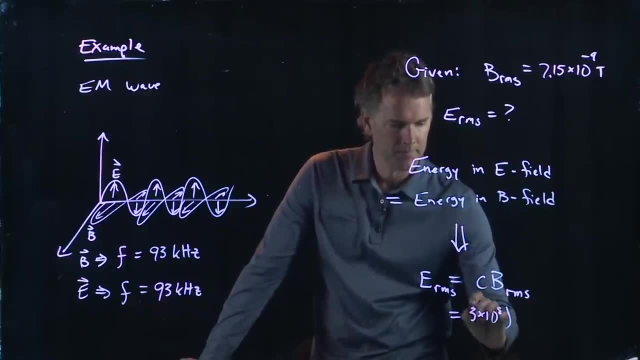 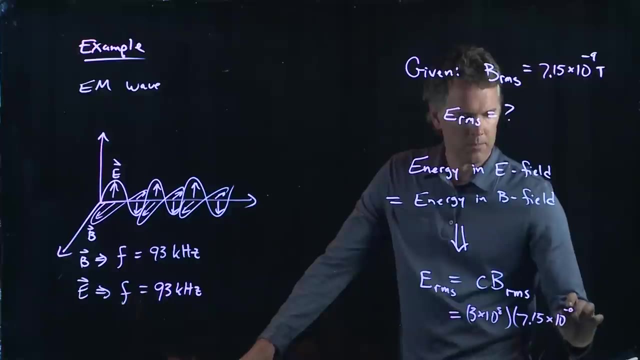 and I multiply it by C, 3 times 10 to the 8th meters per second, we're going to get the right answer. Okay, And if somebody wants to try that in your calculator, tell me what you get Should be about. 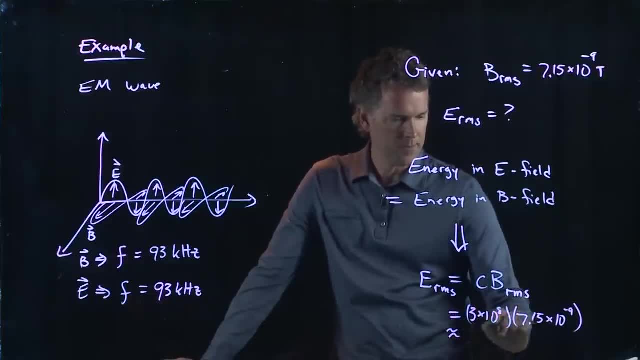 What's that? 3 times 7 is 21.. And then we've got 3 of those 15s, which is a 0.1.. We've got 15s which is a 0.45.. And then we've got a 10 to the minus 1.. 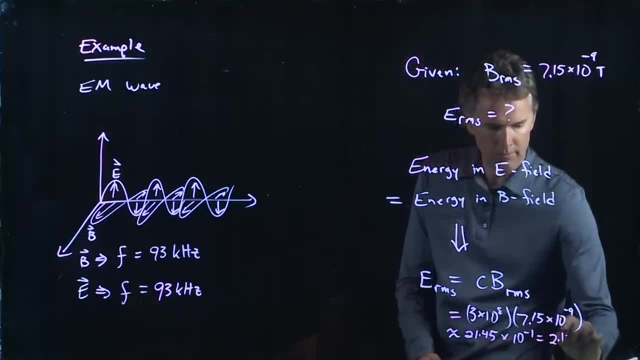 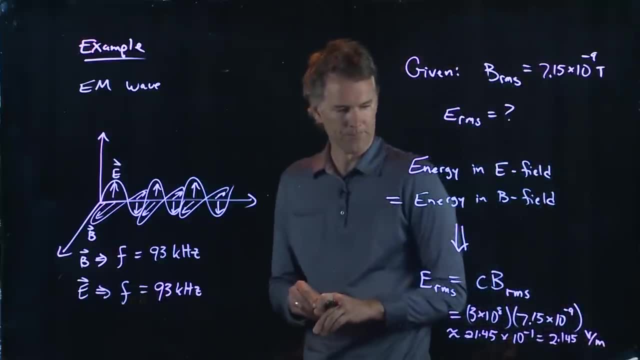 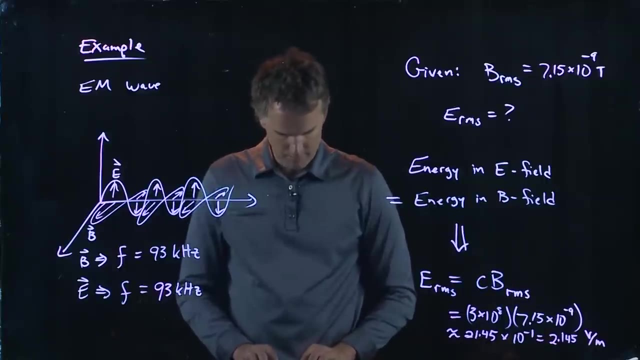 So I'm going to say this thing is 2.145.. And it's the value of electric field, which is, of course, volts per meter. Okay, So let's try it: 2.145 volts per meter. Submit it. 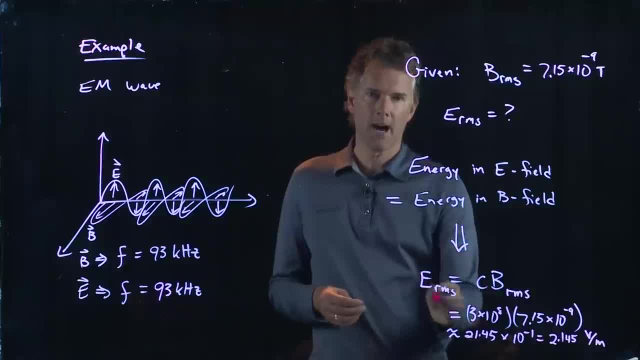 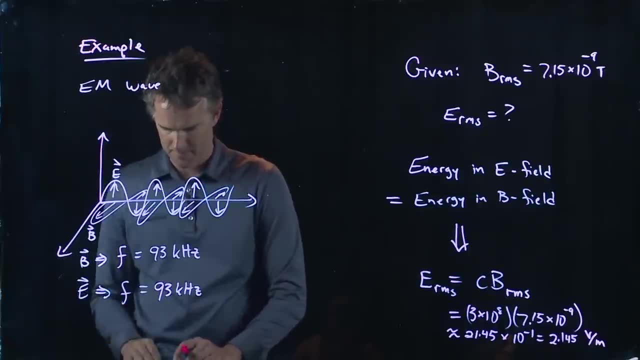 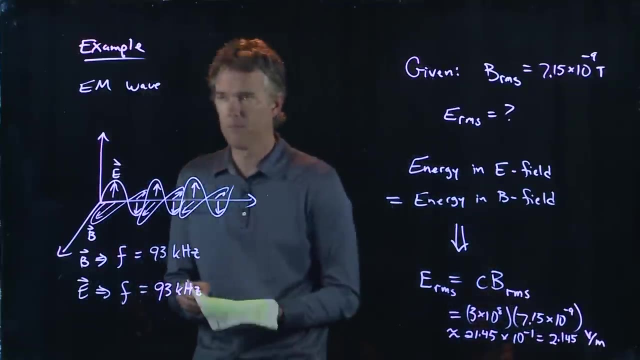 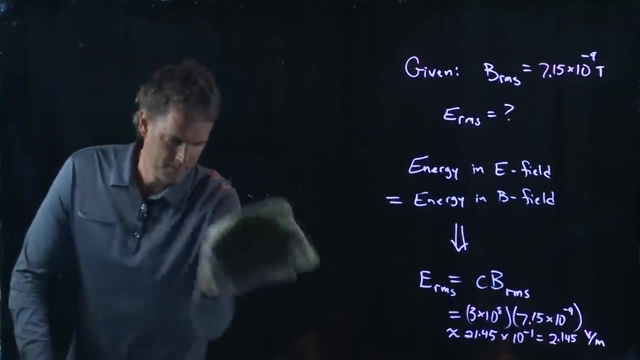 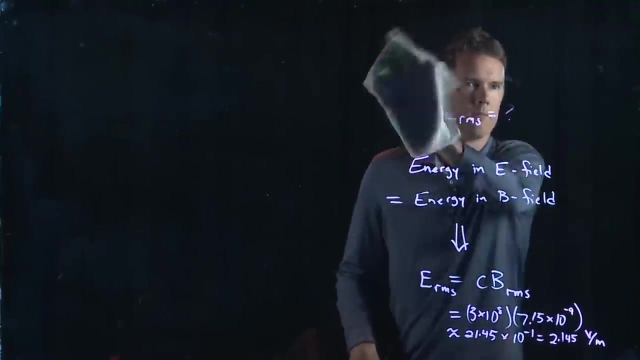 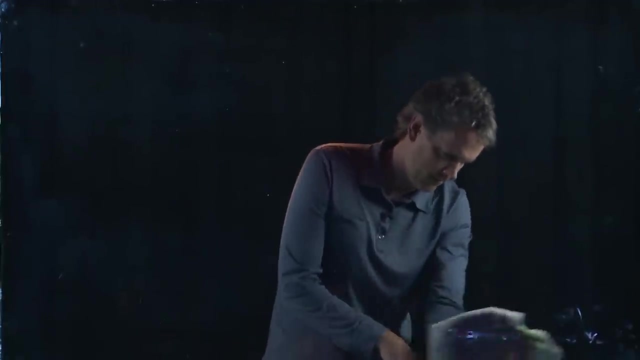 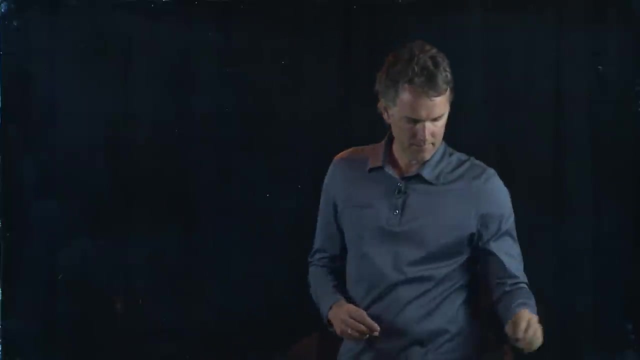 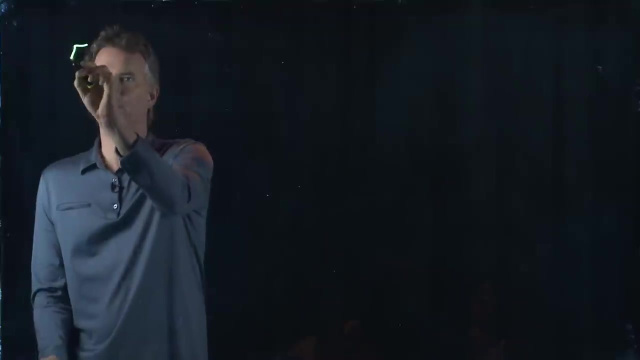 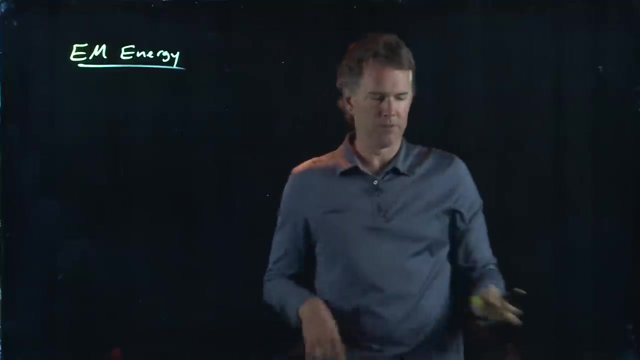 And we are correct. So let's see how we're going to get to this discussion right there. All right, To do that, we need to think a little bit about electromagnetic energy. First off, let's ask you guys a question: Do electromagnetic waves carry energy? 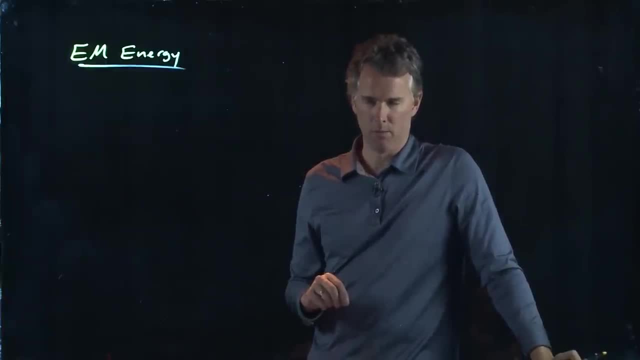 Sure, How do you know that? What happens when you go outside and sit in the sunshine, Especially on today? What happens when you absorb a lot of sunshine? You get warm, right, You get hot, And that's because those electromagnetic waves 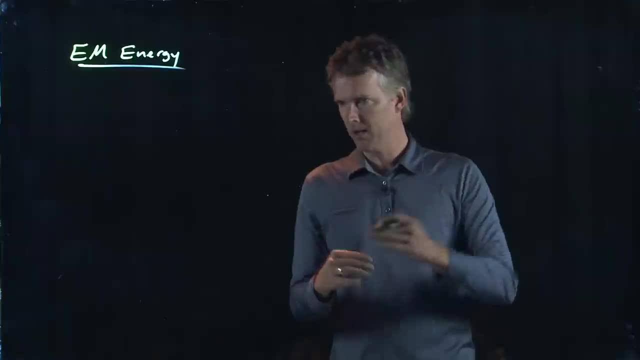 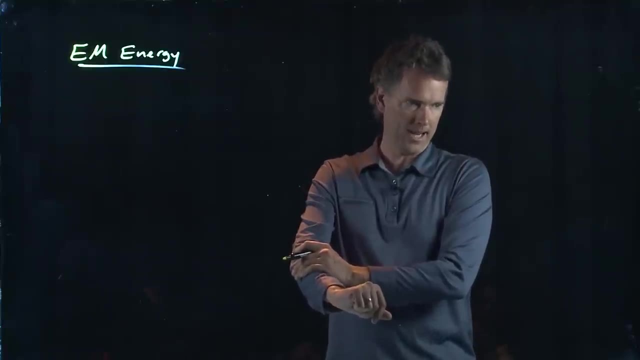 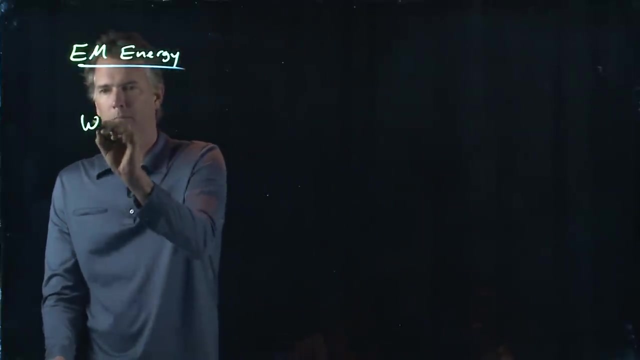 which are coming from the sun, travel all the way across space, punch through our atmosphere, come down, hit you. You're absorbing it. You are absorbing that energy. You get warm, Okay, And so electromagnetic waves clearly carry energy, And we talked about this a little bit before. 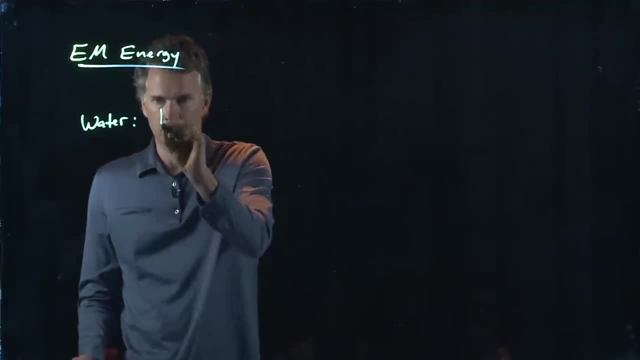 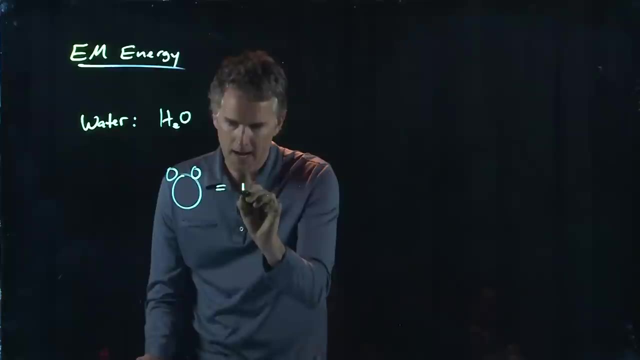 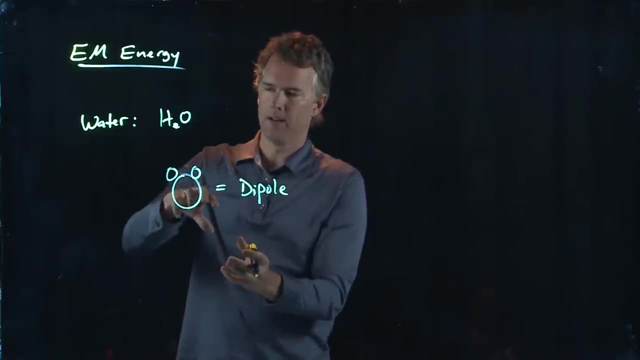 with the idea of water. right, Water is H2O, It looks like that, But it also has a dipole moment to it, And so if we flip this thing to the right and then flip it to the left, and flip it to the right, 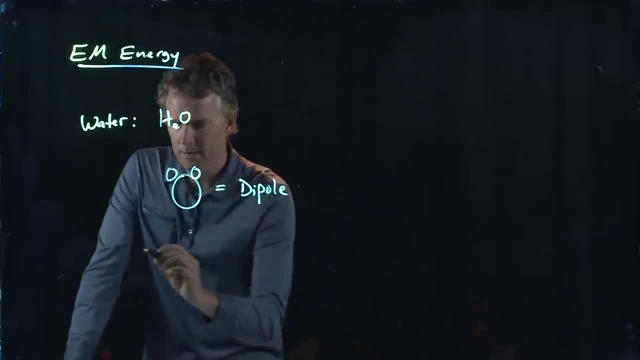 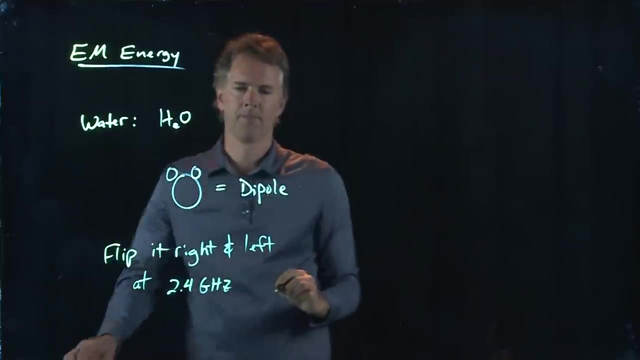 and flip it to the left. we can do that, Yeah, and you'll get a little seasick. But if you do that at a particular frequency, 2.4 gigahertz- this thing turning right and left, that is of course. 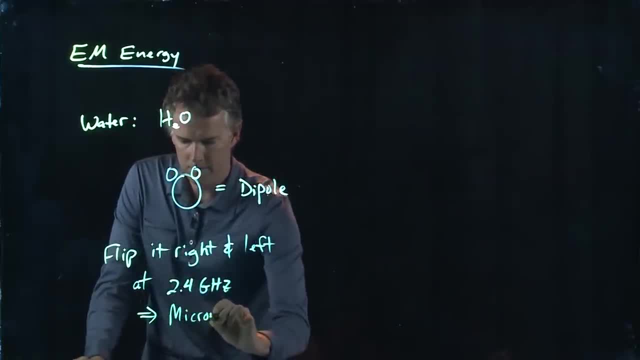 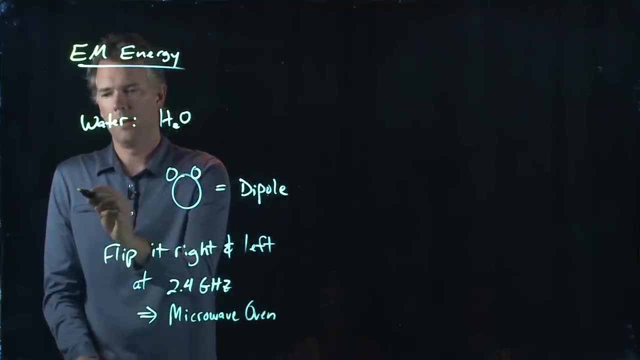 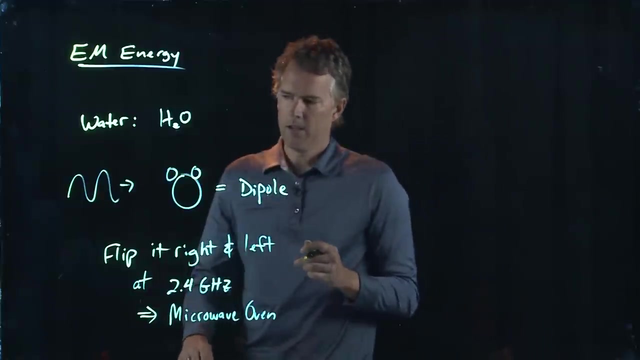 your microwave oven, Okay, And there's an electric field that's going to do that, And so we can draw this electric field coming in to do that. Now, if that electromagnetic field is carrying energy, which it is, it's transferring it to the water. 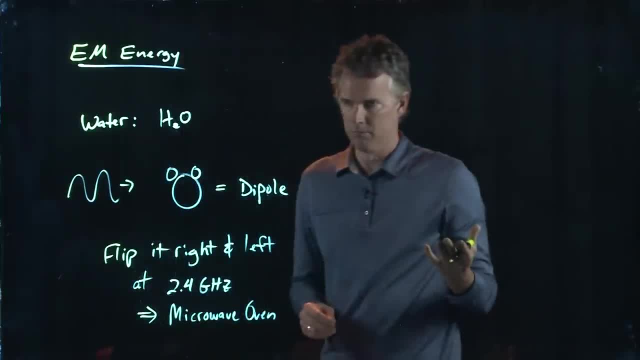 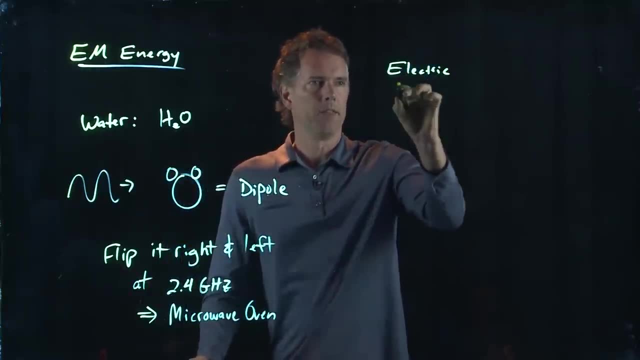 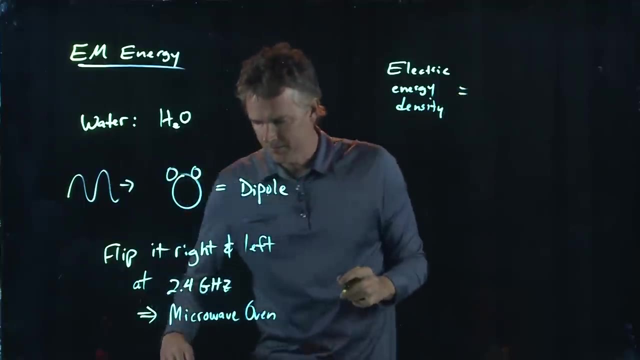 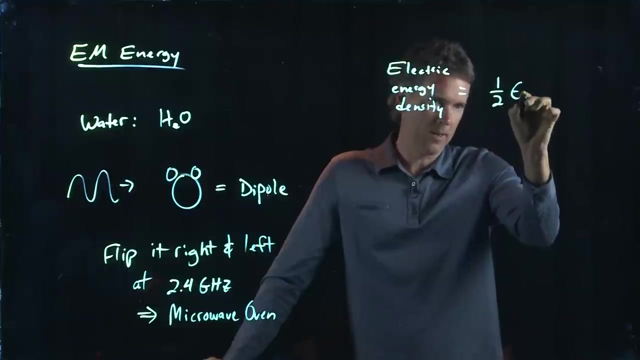 And that's heating up your food. So there is some electric energy density, which we talked about before, And the electric energy density was the following: Remember, energy density is just energy per volume And we ended up with one-half epsilon-naught e-squared. 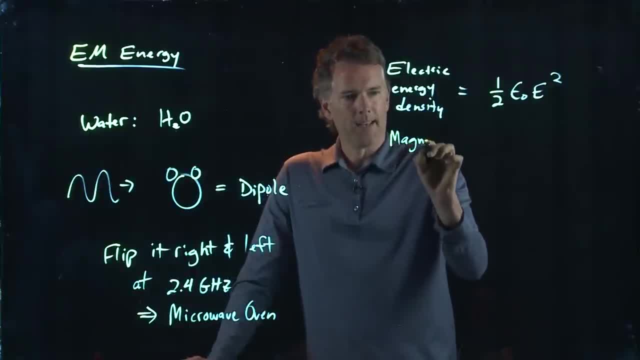 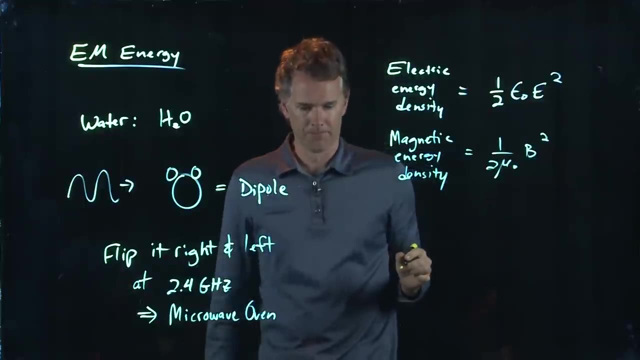 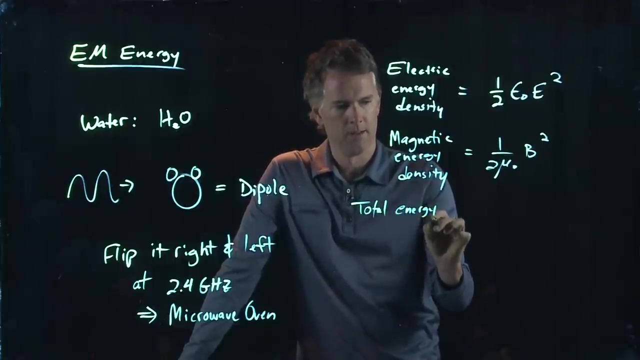 In the last chapter we talked about the magnetic energy density- how much energy is in a magnetic field, And that was one over two mu-naught b-squared, And so the total energy density in a wave is just going to be the sum of those two. 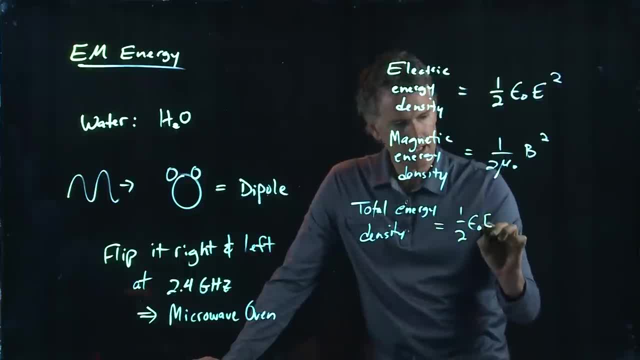 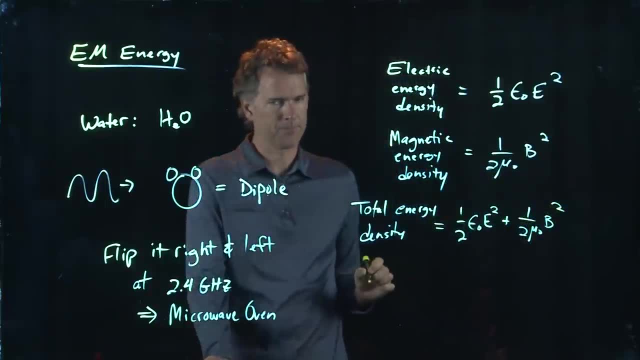 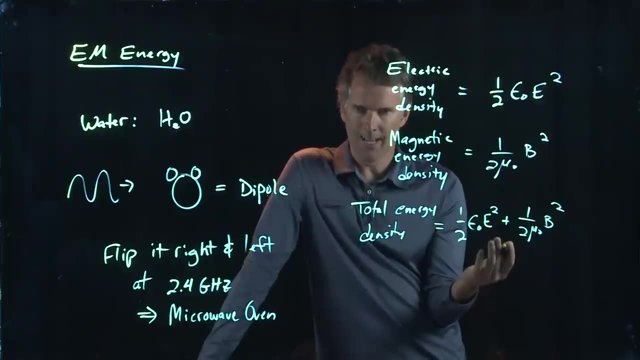 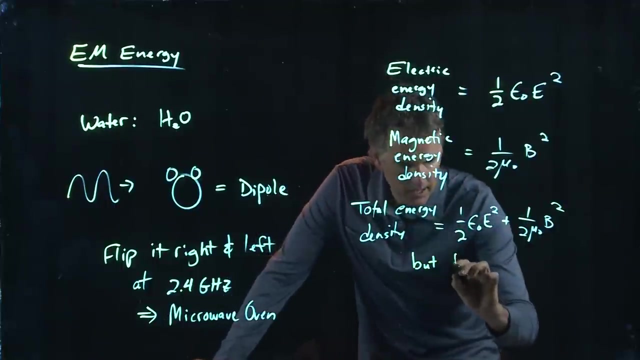 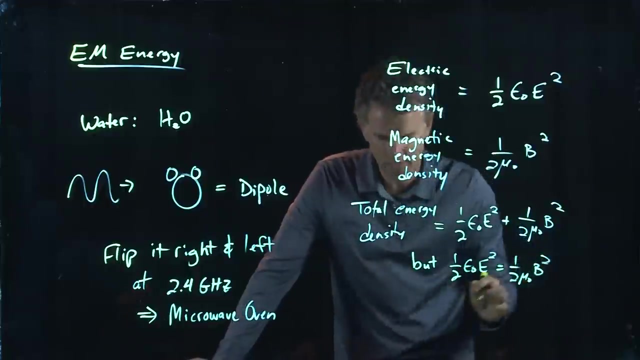 It's one-half epsilon-naught e-squared plus one over two mu-naught b-squared, But the two components have equal contribution to the overall energy density, And so we have the caveat that the electric energy density is in fact equal to the magnetic energy density. 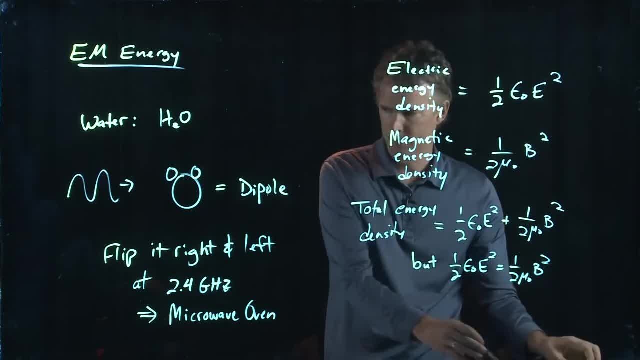 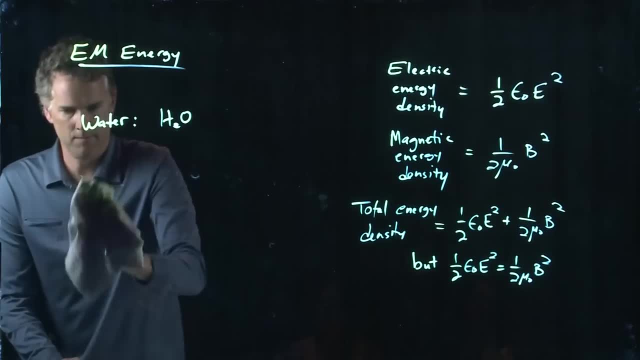 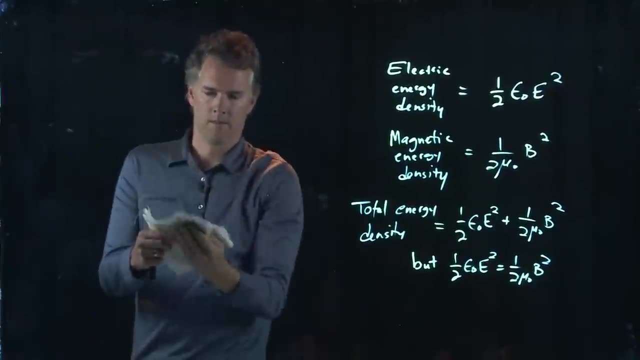 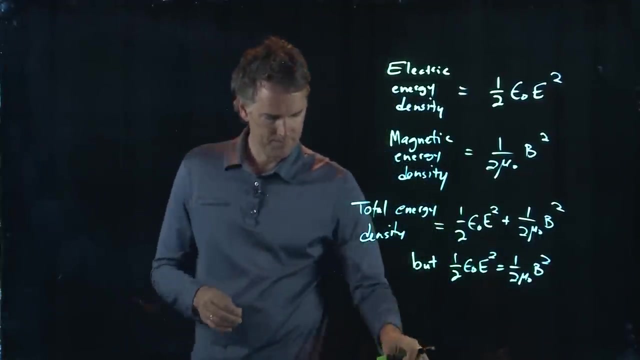 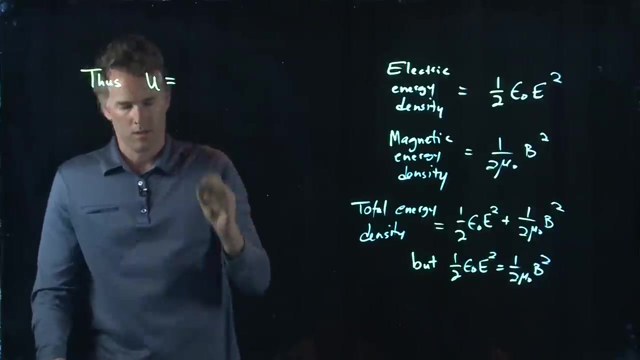 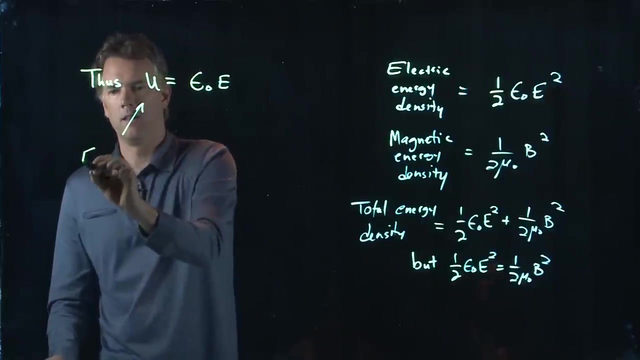 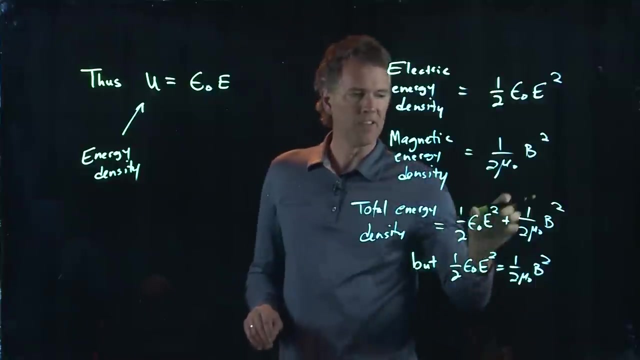 And so we can write the total energy in that wave. u is what we're calling the energy density, And we can write it in terms of e, And if the electric part is equal to the magnetic part, we can just write it as twice the magnetic part. 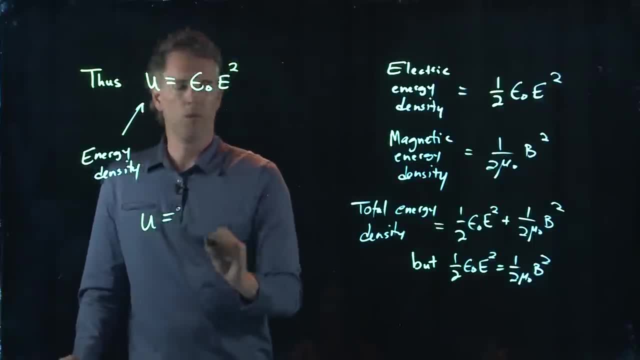 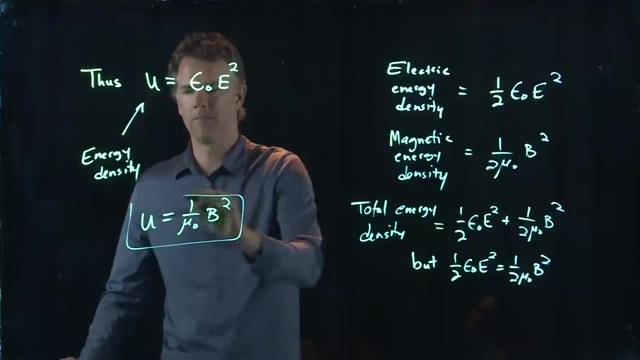 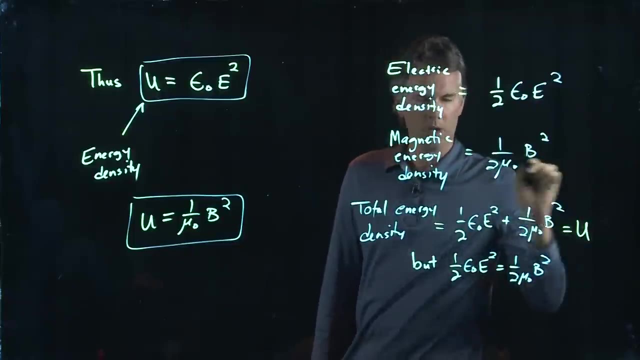 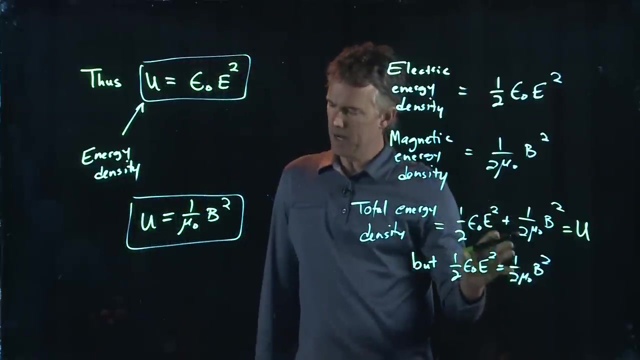 Epsilon-naught e-squared, Or we can write it in terms of the magnetic part One over mu-naught b-squared, And this is what we're calling u the total energy density. Okay, so we have equal parts e and b. 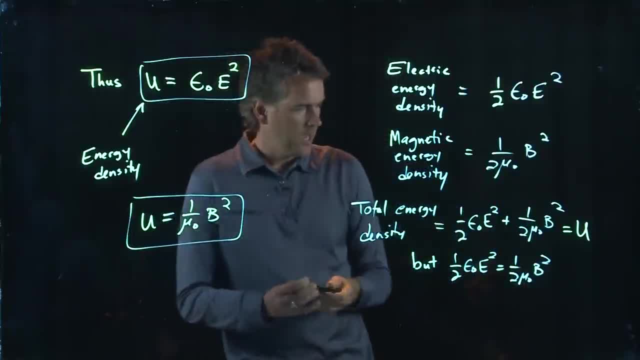 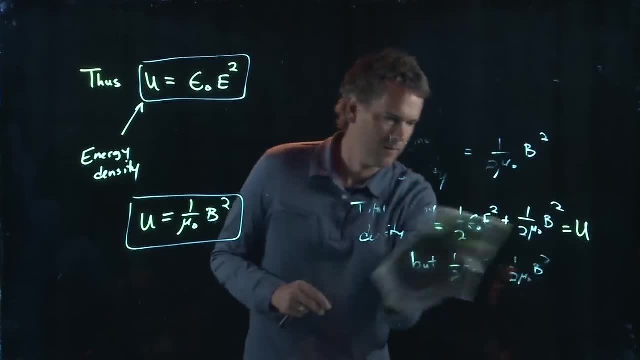 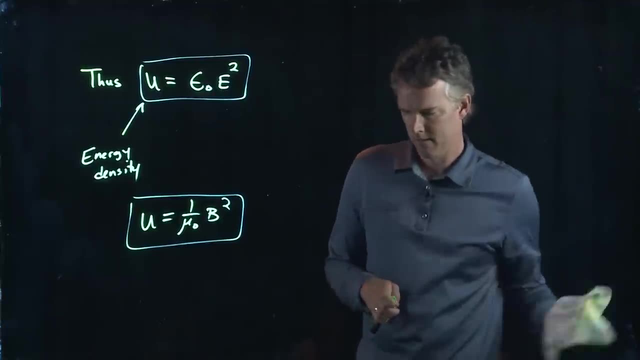 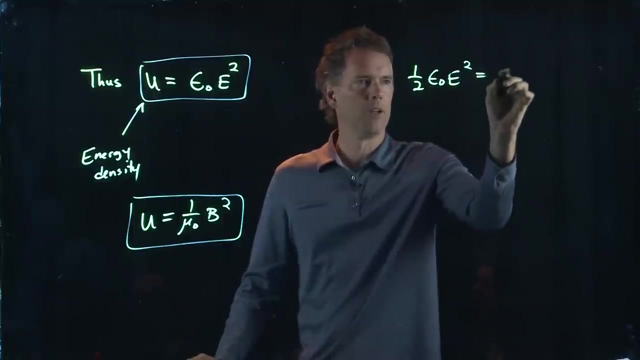 But let's take a look at this last equation here and see if we can determine the relationship between e and b. So what we said was one-half epsilon-naught e-squared is the same as one over two mu-naught b-squared. 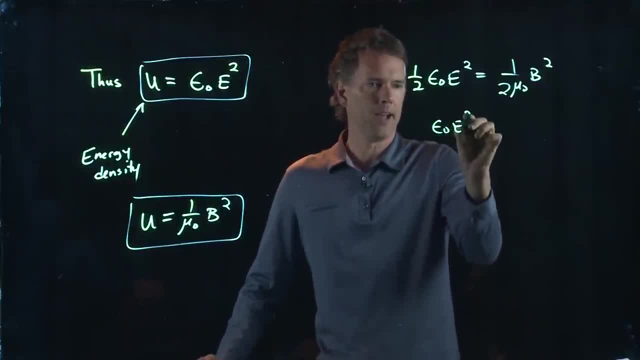 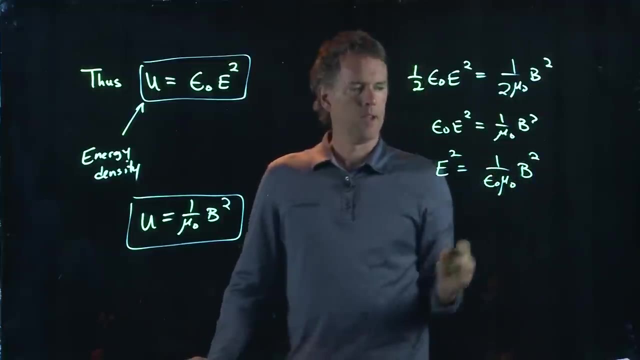 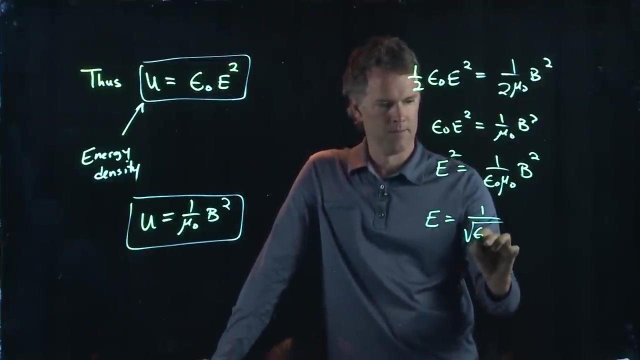 Let's multiply by two on each side, get rid of the half. And now let's divide by an epsilon-naught. And now let's take a square root of both sides. Okay, but we know what these values are. We know what epsilon-naught is and mu-naught is. 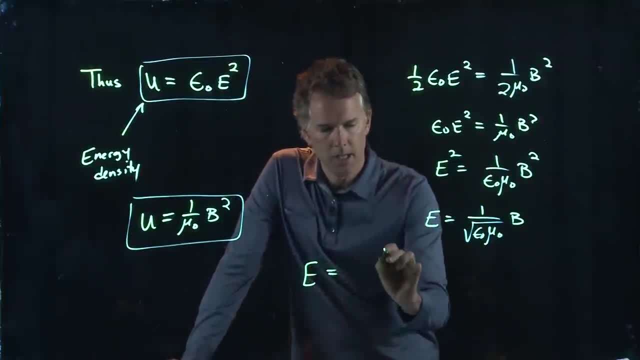 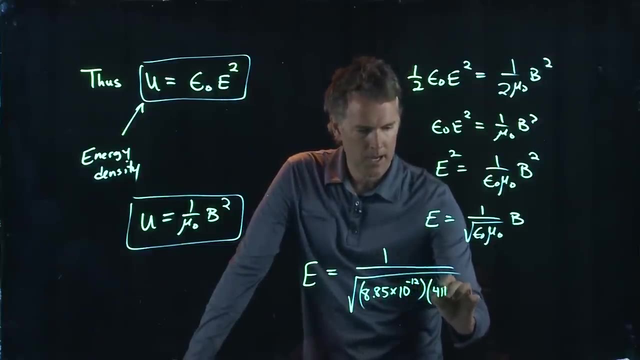 So this becomes the following: E is one over the square root of epsilon-naught, which we said was 8.85 times 10 to the minus 12.. Mu-naught was 4 pi times 10 to the minus 7.. 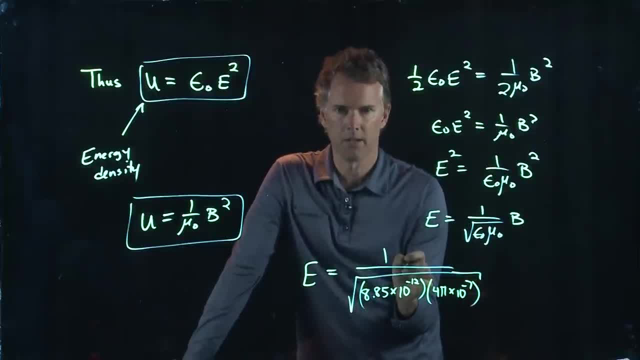 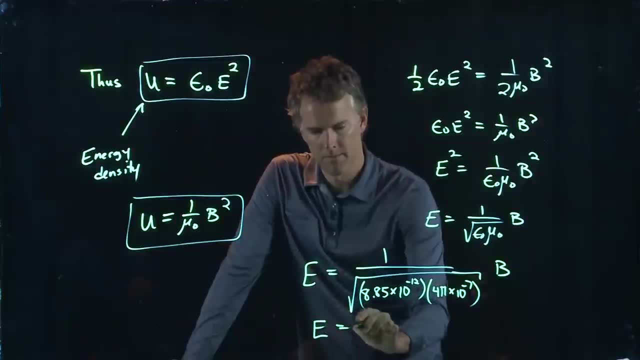 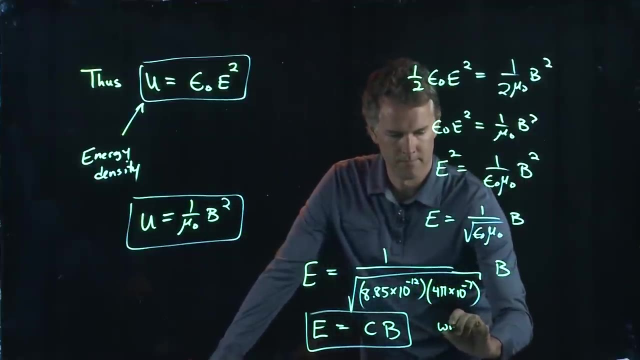 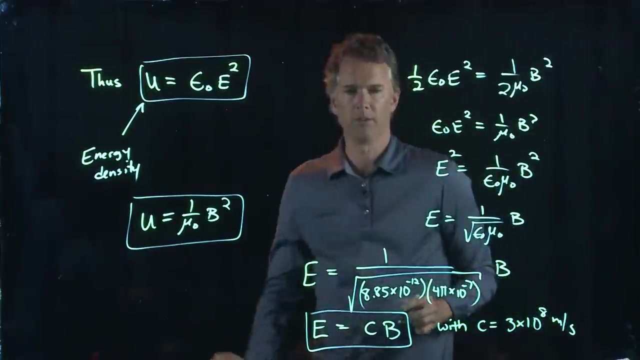 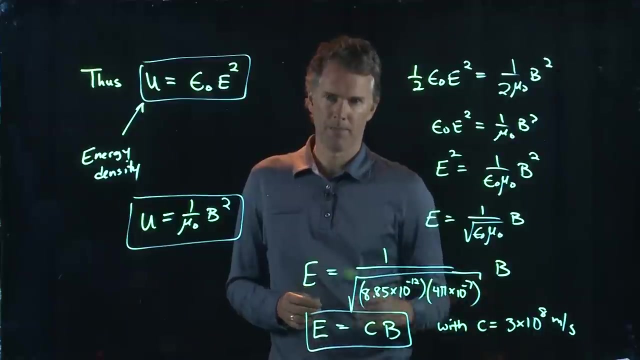 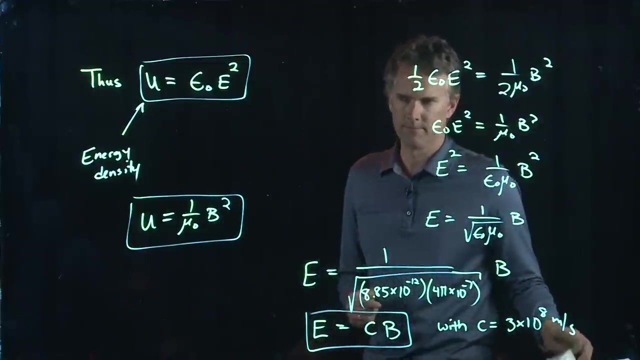 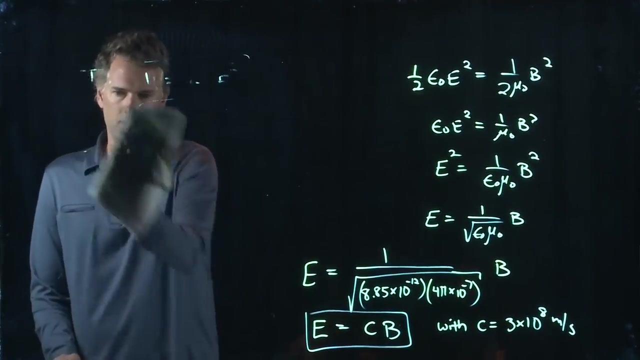 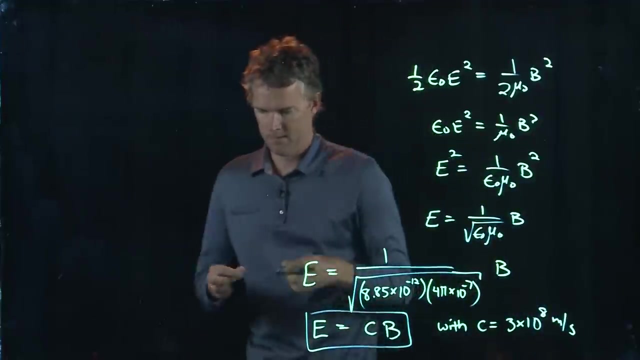 And somebody punch this stuff into your calculator and tell me what you get And I will approximate it here And hopefully you got that. Anybody get that number when they did one over the square root of all this stuff right here. That's right. 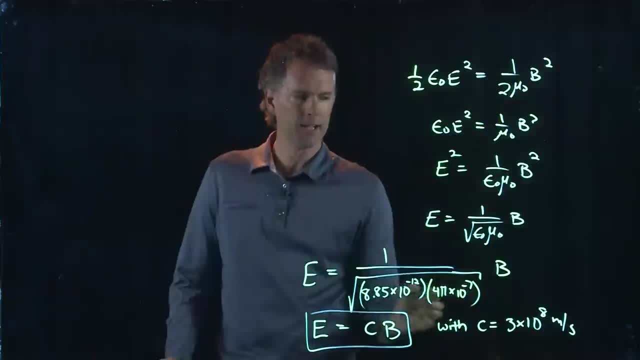 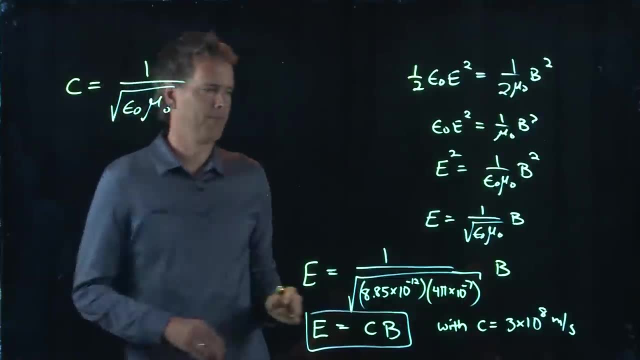 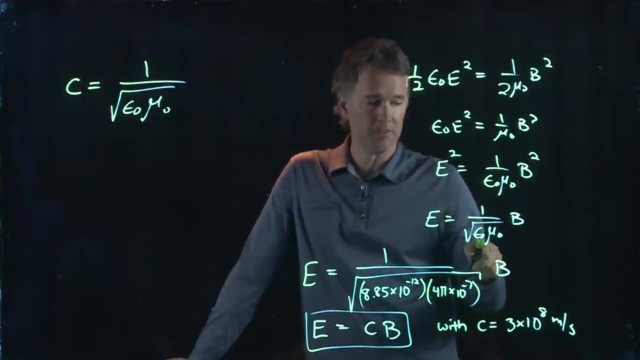 So this is kind of cool, right. C- the speed of light came about from Okay, Okay, Okay That You take those electric experiments that you did and you figured out what epsilon-naught was. You did some magnetic experiments and you figured out what mu-naught was. 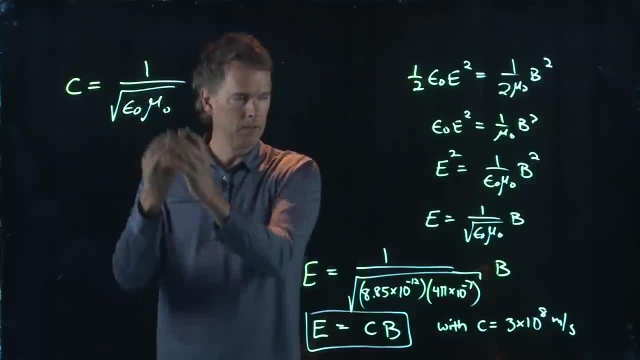 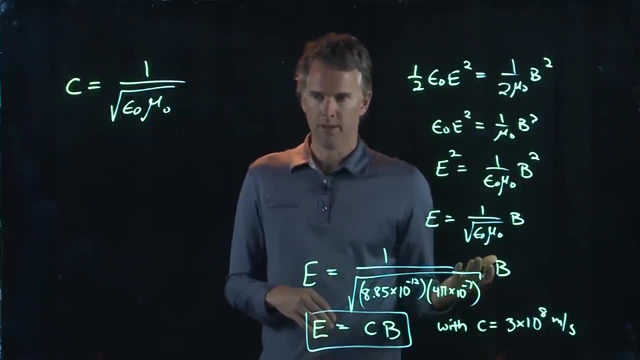 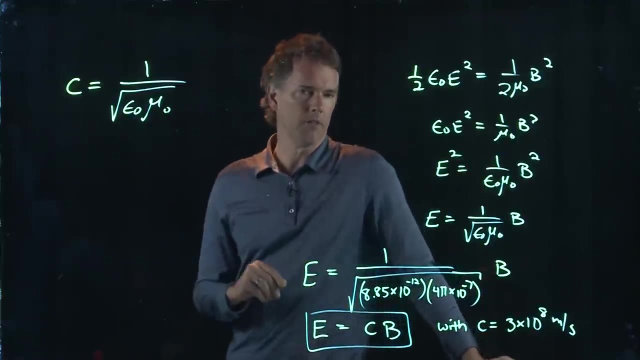 And suddenly you put them together in this special way and you get the speed of light, You get how fast electromagnetic waves travel across the universe. And this is the beauty of Maxwell's equations, This is Maxwell's derivation of this problem. Before Maxwell nobody really knew definitively that light was electromagnetic waves. 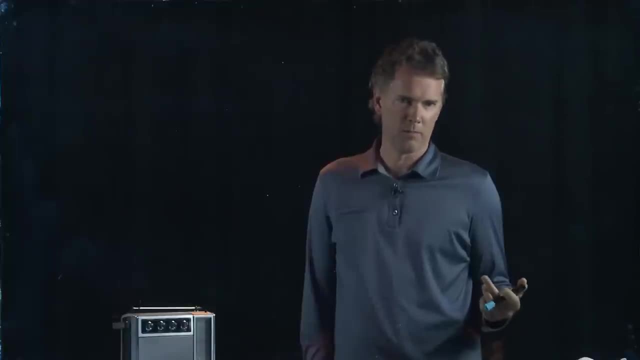 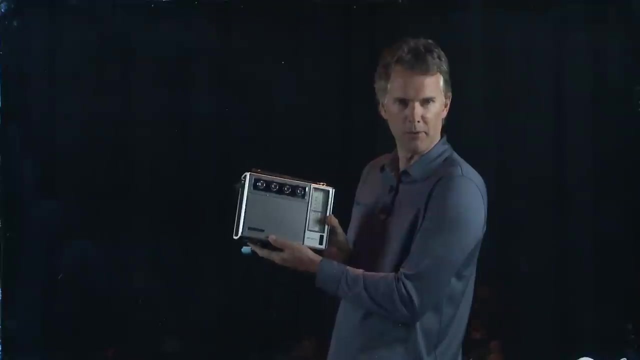 And it was only after Maxwell that we knew that. Okay, Welcome back everybody. If you're at home watching and want to chime in Ian's monitoring the computer over there, Dave brought in one of his cool radios. This is what a radio looks like. 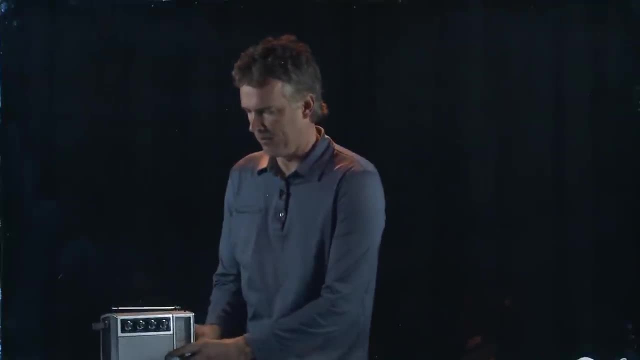 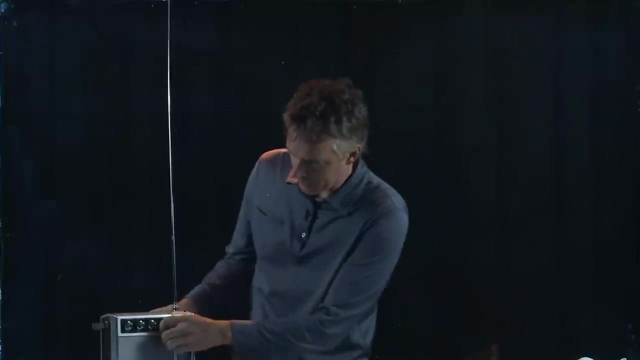 Are you guys familiar with these devices? Okay, So this is the big metal bar that we were talking about. All right, You lift it up like that And then you can turn it on. Trouble boy, We know where you've been. 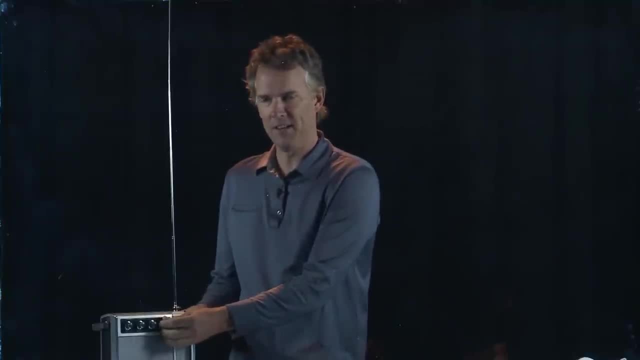 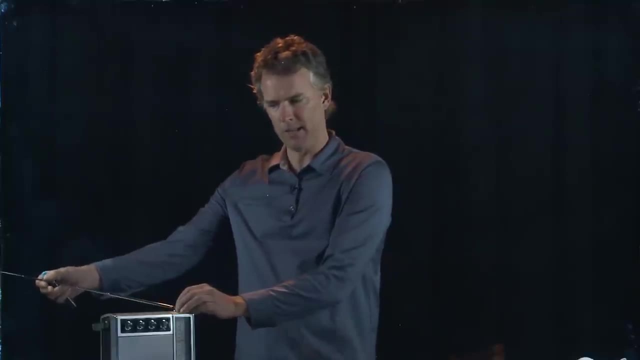 Yeah, Okay, That sounds pretty good. Now let's say, your reception is not very good. What can you do? You can move your antenna around And in fact, if I point it like that, now listen, that doesn't sound very good. 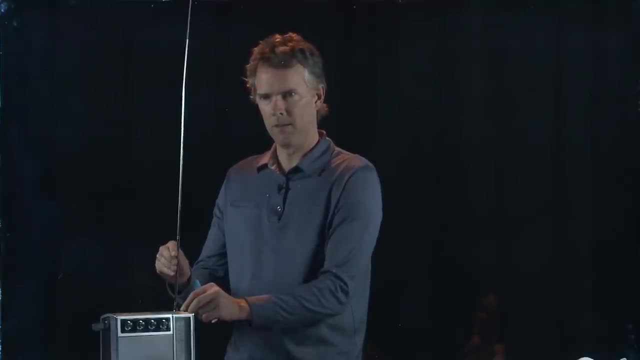 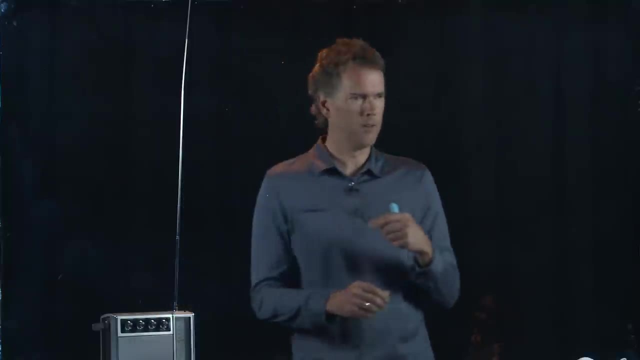 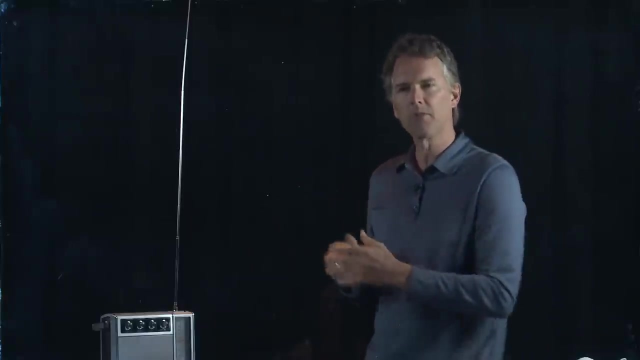 Right, Okay, So let's move it back up, And now it sounds quite a bit better. So what can you tell me about the electromagnetic wave that's coming to our radio from the radio station, Just on that little experiment that we did? what can you tell me about the electric field? 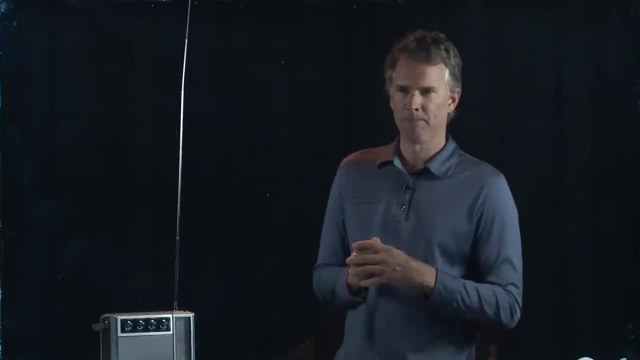 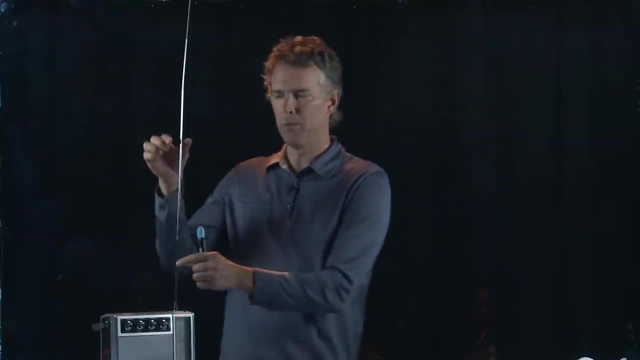 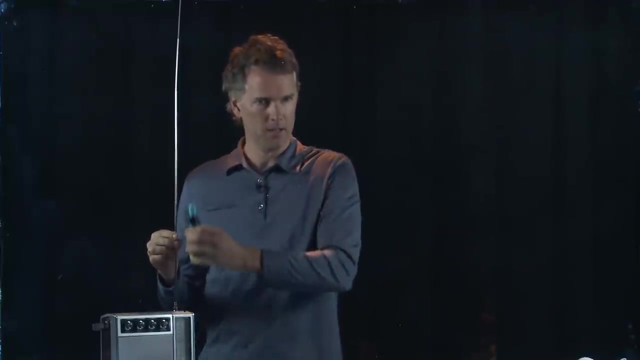 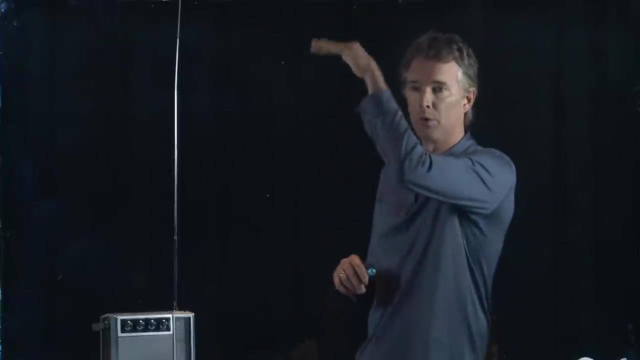 that's coming. Can you tell me anything? Okay, Ian says. Okay, Ian says if we're getting better reception like this, then the electromagnetic wave must have an electric field that is pointing up and down this metal bar. And so the electromagnetic field that came in was going like this: 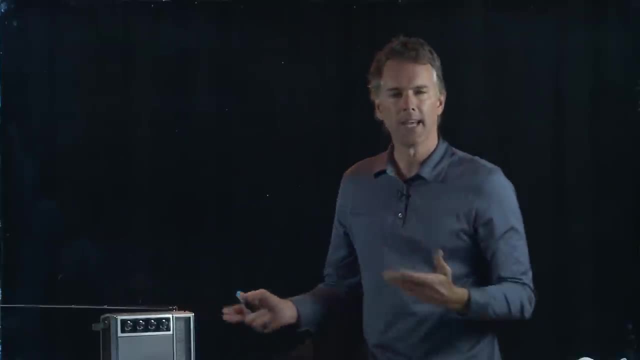 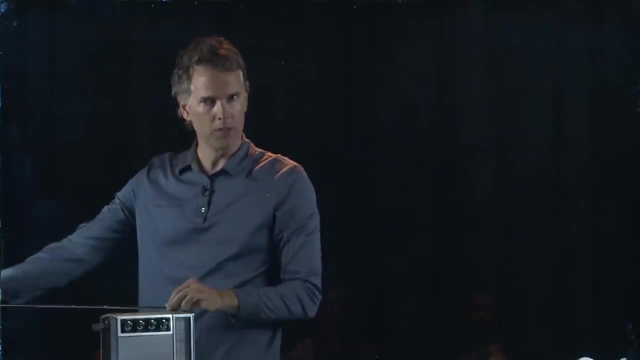 And when I turn this bar over to the side it doesn't get as good reception because that electromagnetic field that's going up and down can't excite the current. It can't excite the current along the length of the wire. So this is kind of cool. 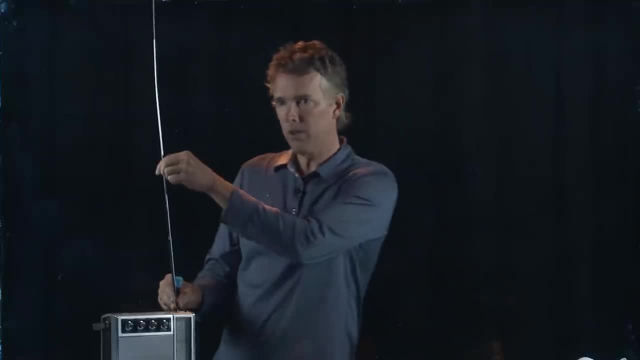 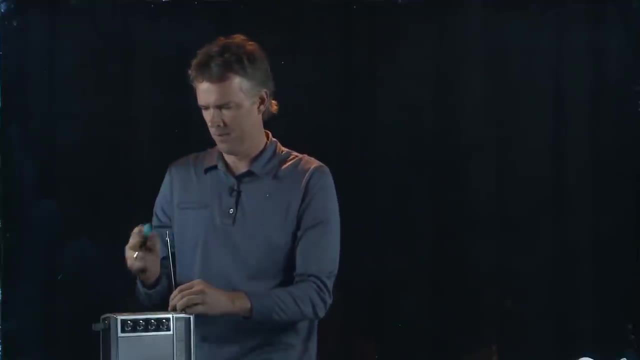 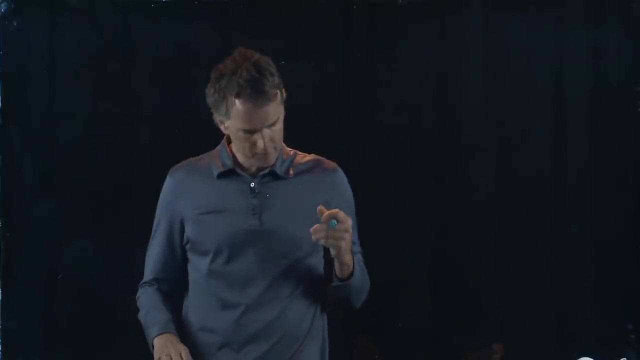 You can actually tell what the electromagnetic field is just by one of these things, moving it around in space and checking your reception. All right, Very nice. Okay, Let's take a look at one of your homework problems from chapter 22.. And this is number 2215.. 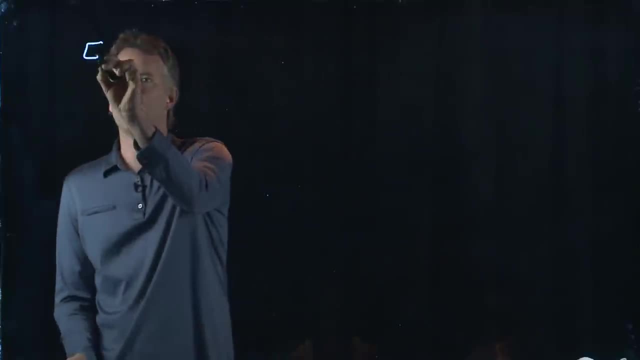 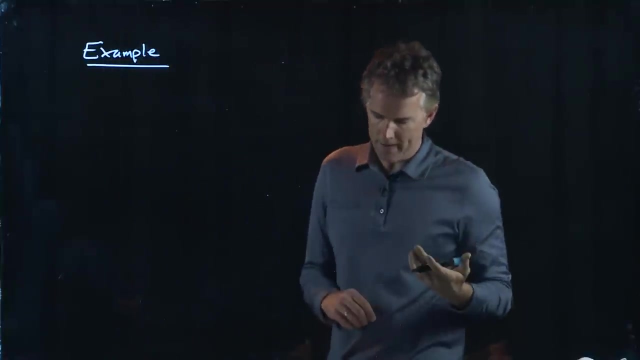 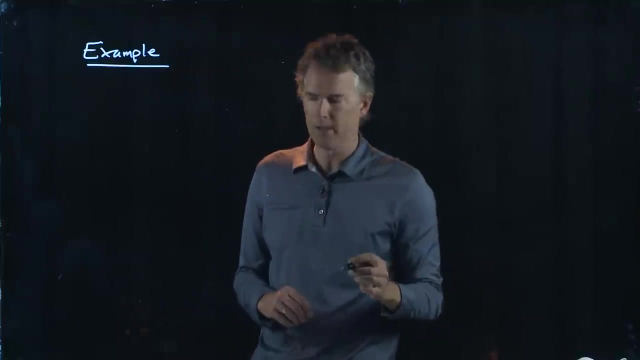 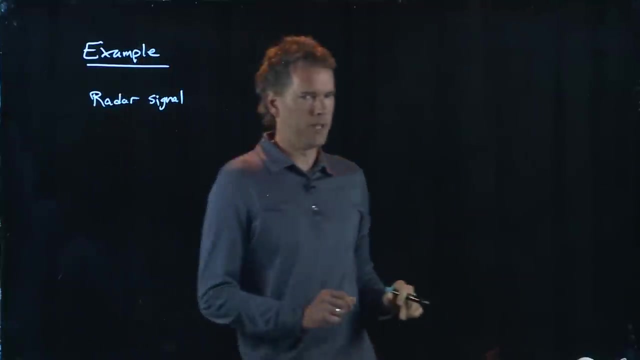 All right, All right, Let's do it again. Okay, In this example it says: what is the wavelength of a 25.75 times 10 to the 9 hertz radar signal in free space? Okay, So radar is just another region of the electromagnetic spectrum, and they're telling us that the frequency 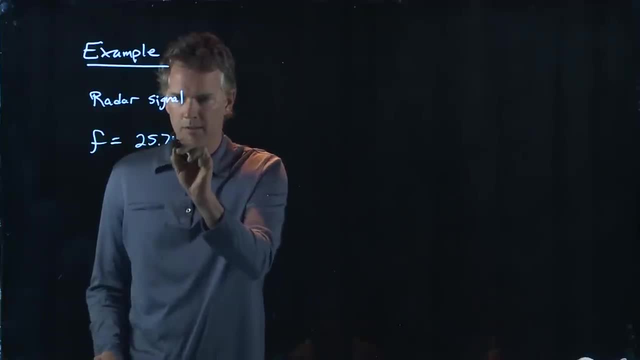 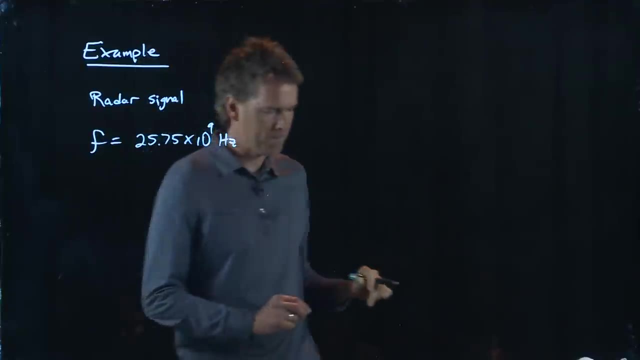 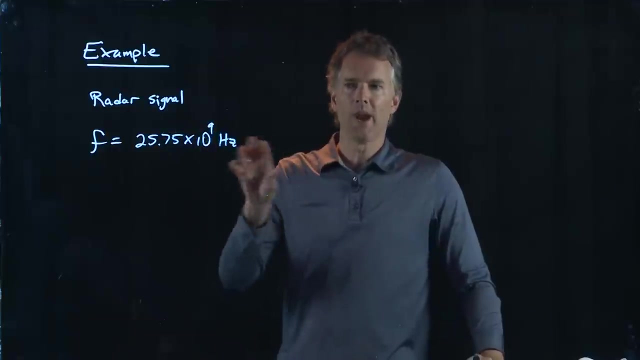 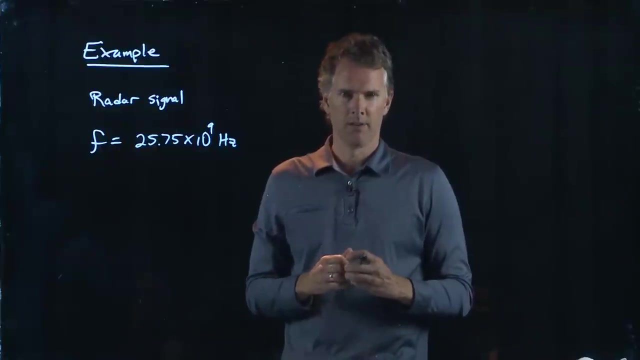 is 24.75.. Okay, 5.75 times 10 to the 9 hertz. okay, Radar being a frequency of this range means it's in the radio frequency of the spectrum. Anybody know what radar stands for? Anybody in the ROTC program here? 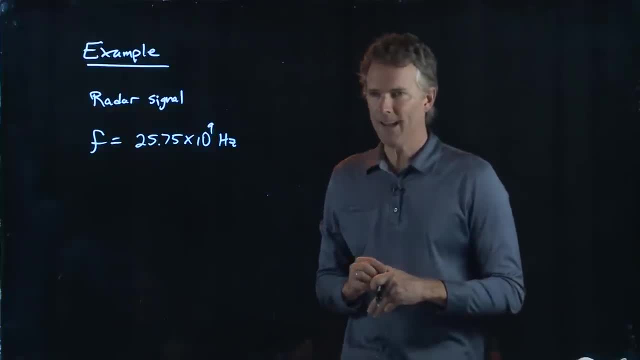 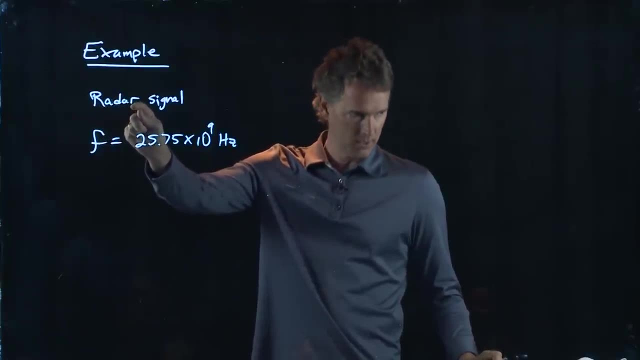 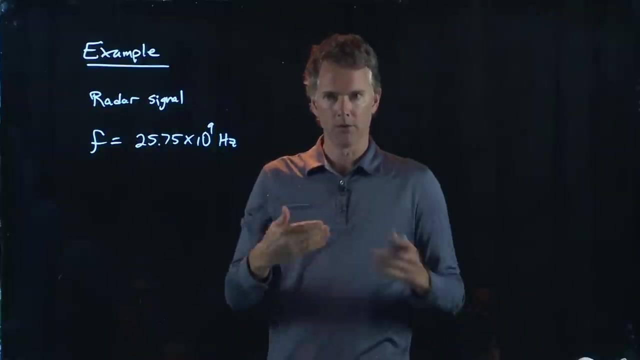 Okay, Radar stands for radio detection and ranging. That's what radar means: Radio wave detection and ranging. And so you can use radar to detect opponents and range How far away are they? Okay, So that's what radar means. So the speed of light, they tell us. 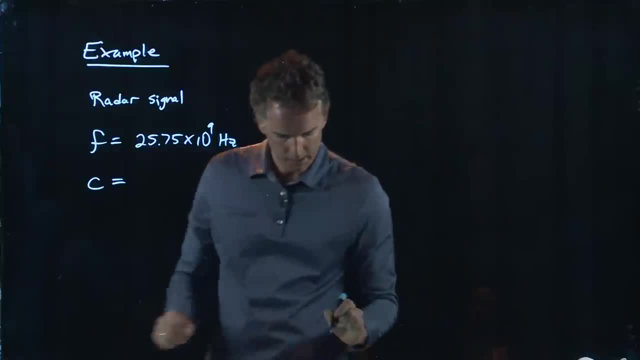 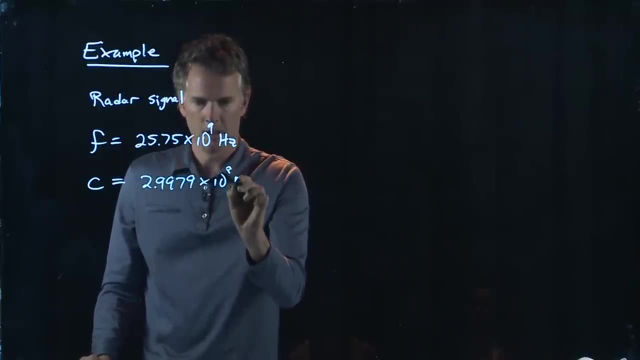 is 10 to the 9 hertz, Not really 3 times 10 to the 8.. It is actually 2.9979 times 10 to the 8 meters per second. So it's pretty close to 3 times 10 to the 8,. 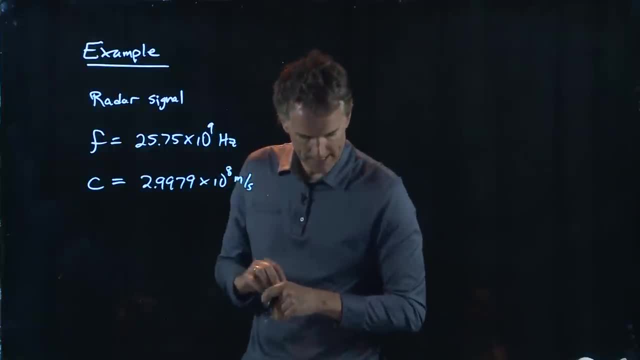 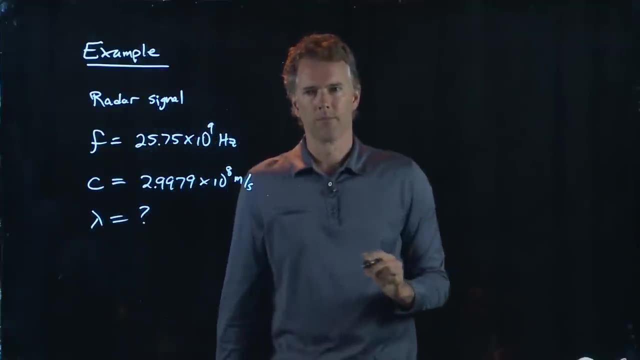 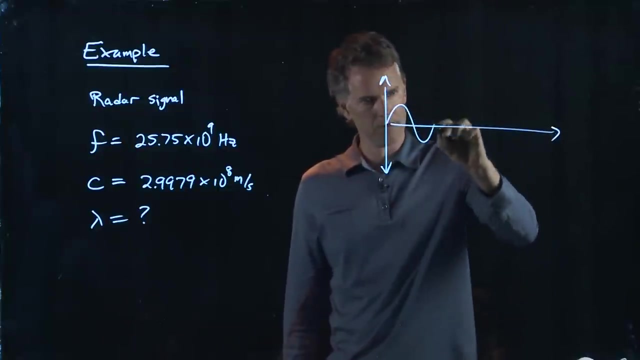 and that's why we usually approximate it. But this is the exact value. And now they want to know what is lambda. Okay, When you think about these electromagnetic waves, what we said was: the electric field is going up and down like that. 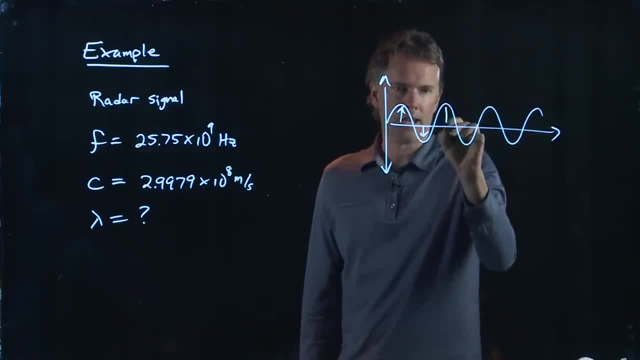 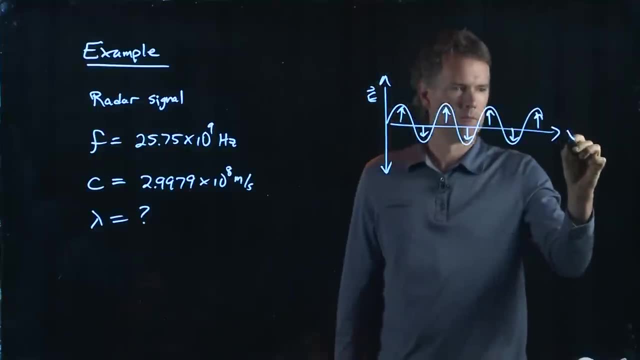 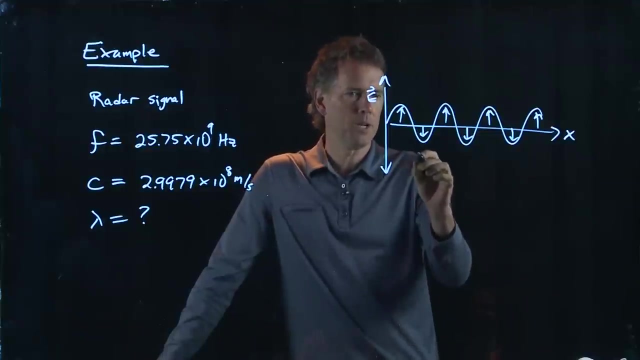 And if we're thinking about a wavelength, That's my jam, It's not my jam. What are we talking about? We're talking about how far is it from there to there. Okay, Which is the same as how far is it from there to there. 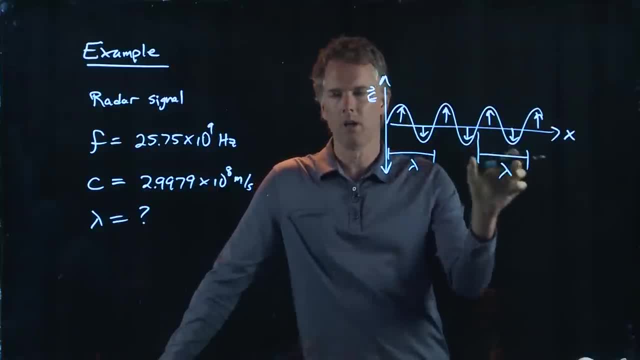 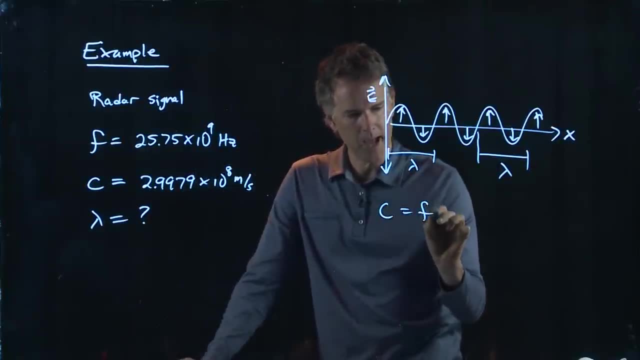 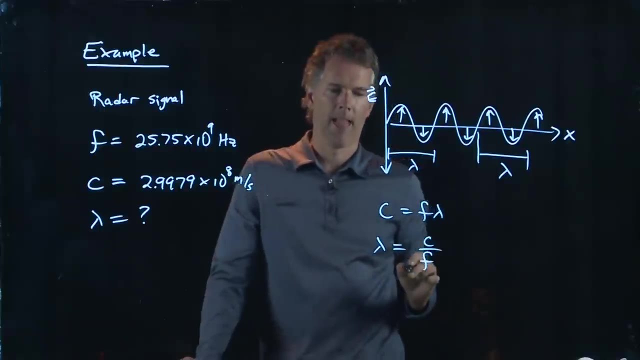 Any time the wave repeats itself. that is 1 lambda. All right, And we know the relationship, right. We know that C is equal to F times lambda. So what is lambda? It is C over F. And now we have all those numbers, right. 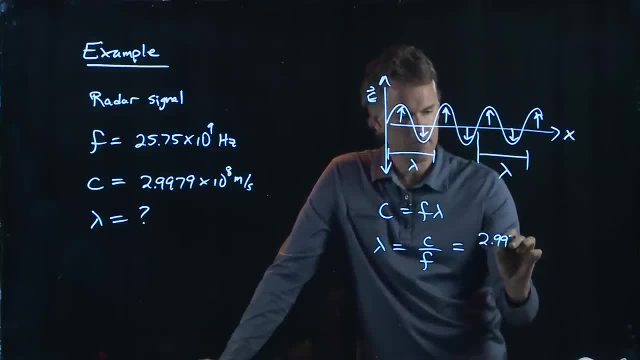 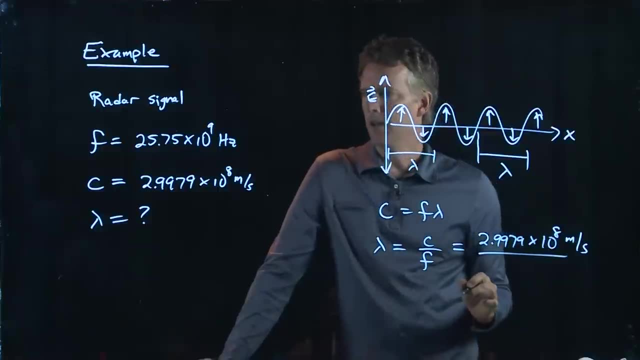 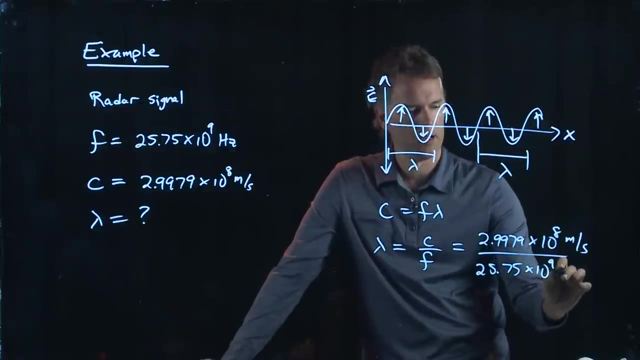 C is 2.9979 times 10 to the 9 hertz. Okay, So that's 10 to the 8 meters per second. F we said was 25.75 times 10 to the 9 hertz is 1 over seconds. 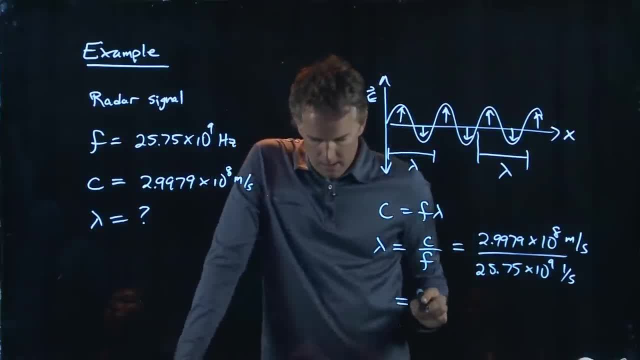 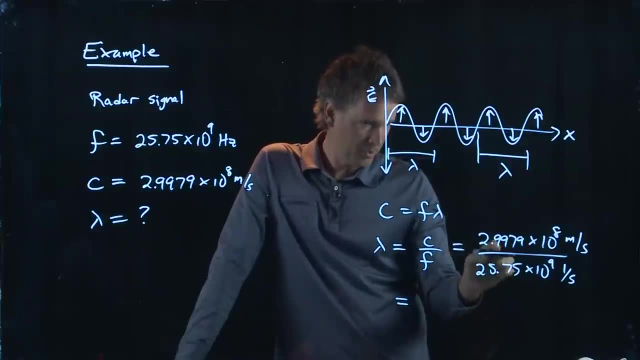 And so we're going to end up with something in meters, And they want four significant figures. Okay, So that's going to be tough for me to approximate it here. So somebody punch this into your calculator and tell me what you get for that. 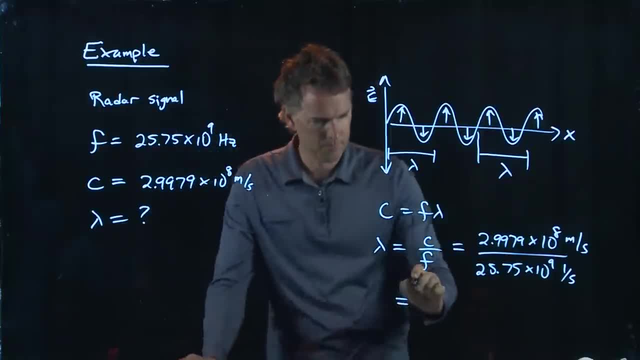 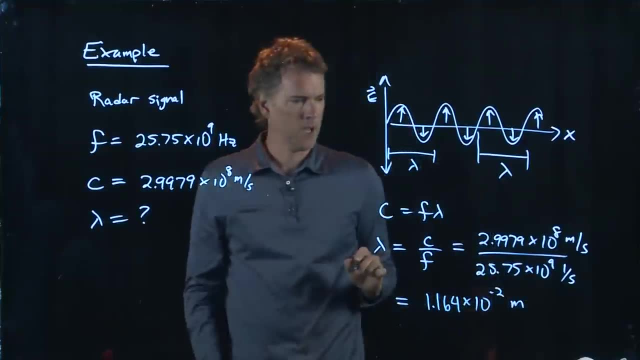 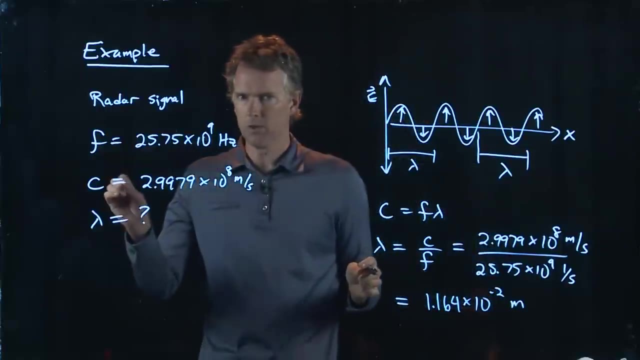 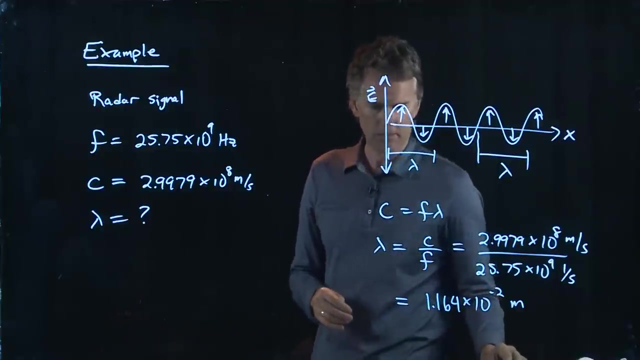 For that answer, right there. Okay, And the units are meters. The per seconds are going to cancel out 10 to the minus 2.. That sounds good, right, That sounds like radio wavelengths. Why does it sound like radio wavelengths? 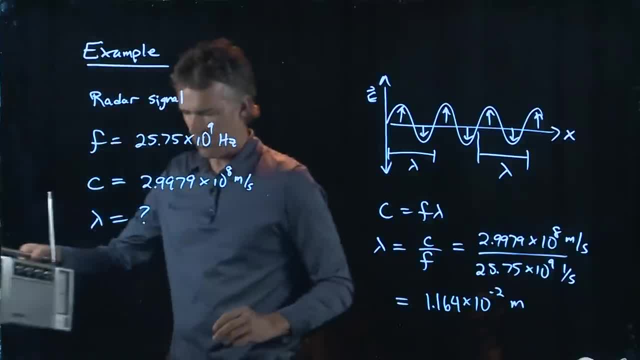 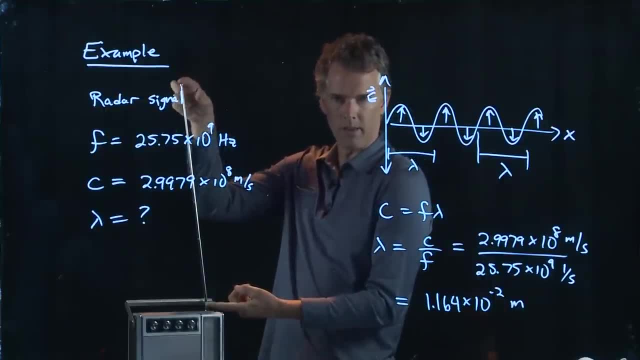 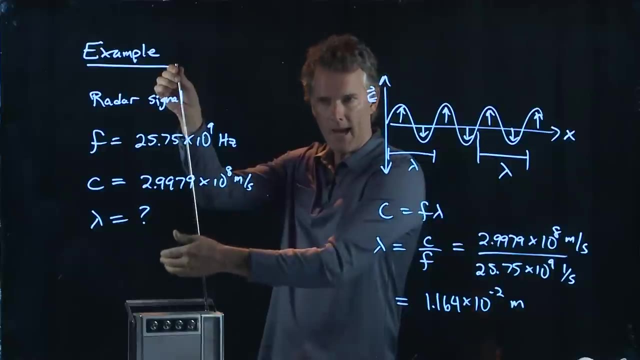 Because it's centimeters And when you think about a radio, the antenna has to be on the order of the wavelength. So if this is my wavelength of a half a meter, that would be AM radio station or maybe even FM. This is centimeters, but that's okay. 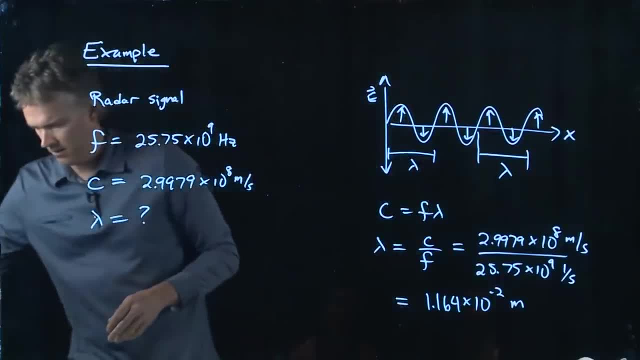 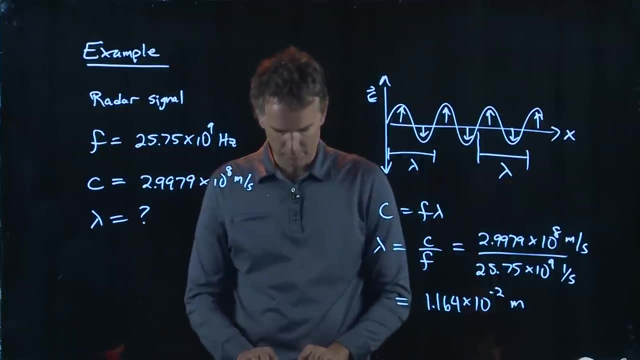 That's on that order, right there. All right, So let's punch in that number and see if we get the right answer: 1.1.. 1.164 times 10 to the minus 2. And the units are meters. 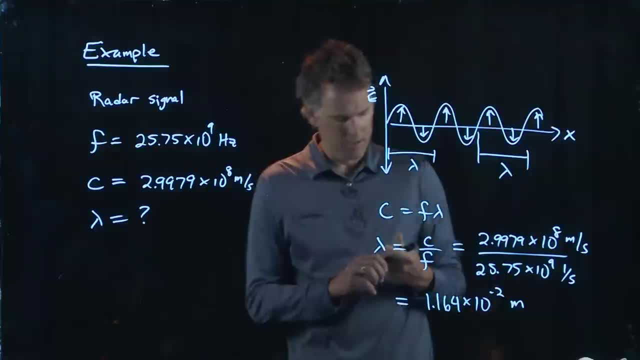 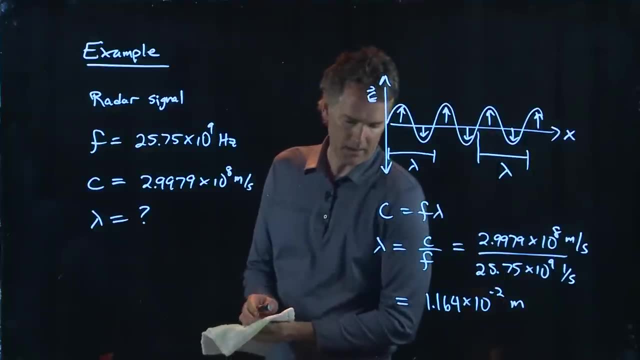 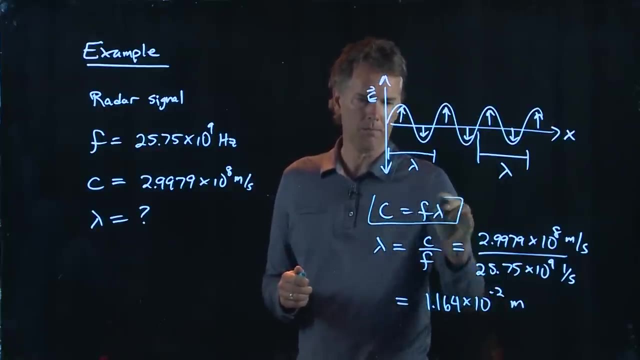 And that is indeed the correct answer. Okay, And now, as a follow-up to Part B, it says what's the frequency of an X-ray with wavelength 0.11 nanometers, So that one you can handle on your own. You're, of course, going to use the same relationship. 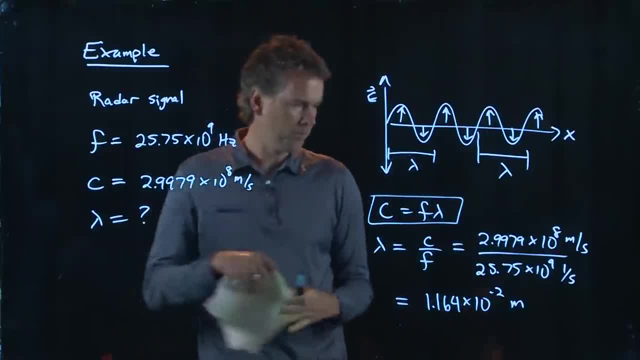 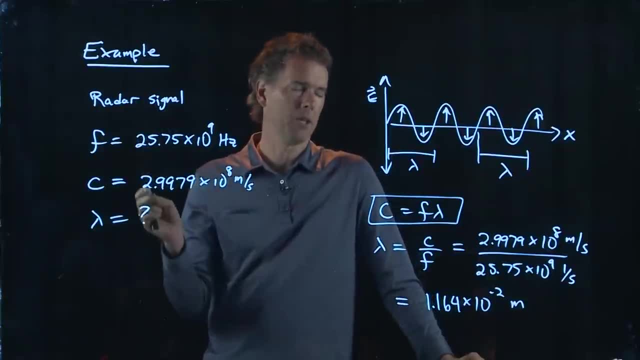 C is equal to F lambda. But there's an important point here, which is, if I'm thinking about radar waves moving through space and then I'm thinking about X-rays moving through space, are both of those things really moving at the same speed? 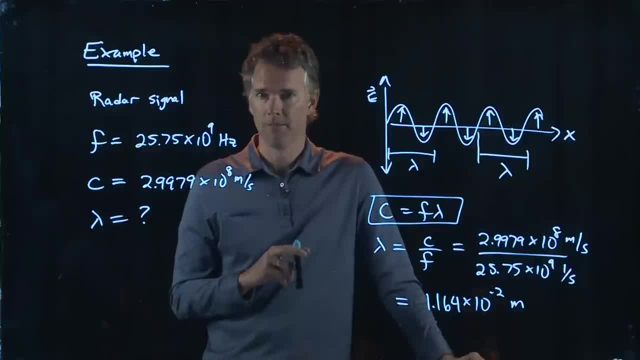 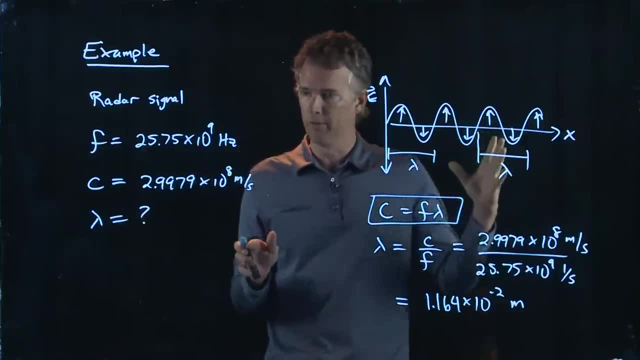 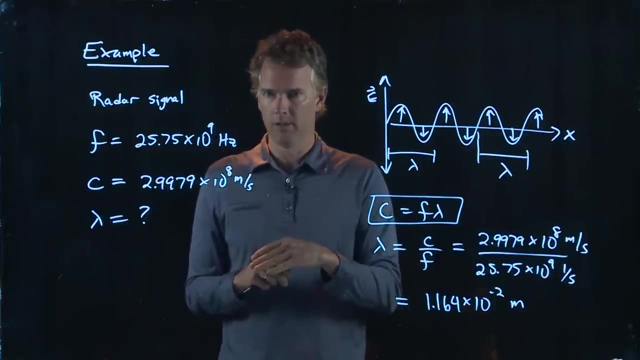 And the answer is yes, they are All. electromagnetic waves travel through free space, through vacuum, the universe, at this particular speed. It doesn't matter if they're X-rays or if they are radio waves, They all go through at the exact same speed. 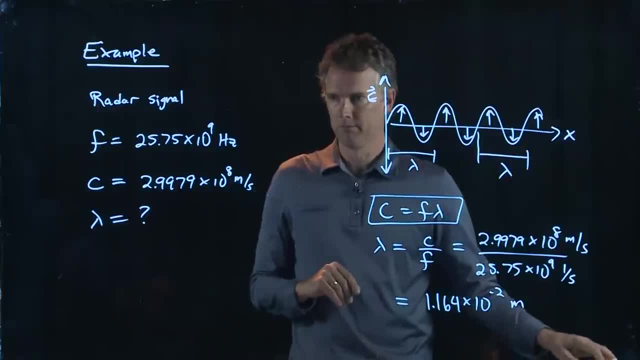 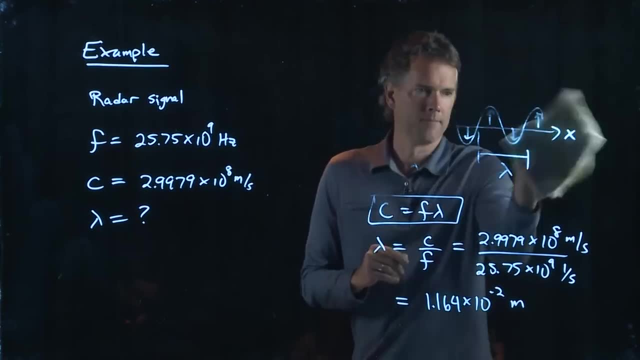 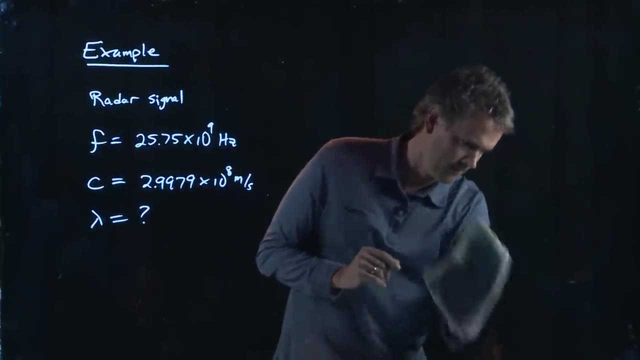 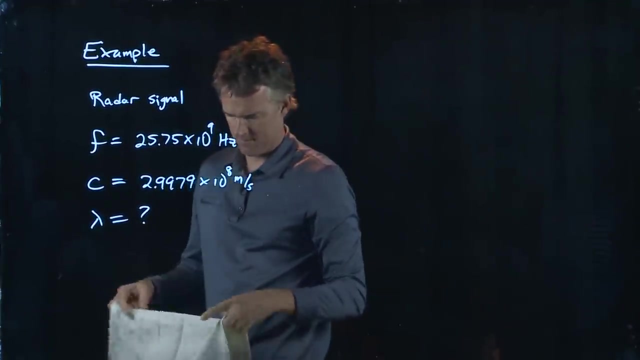 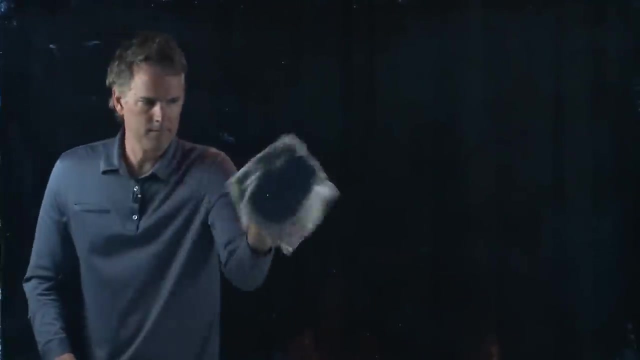 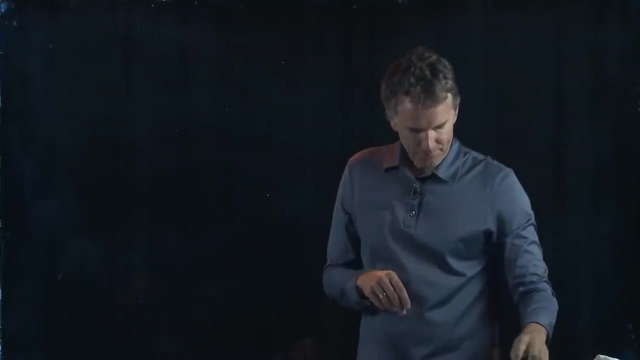 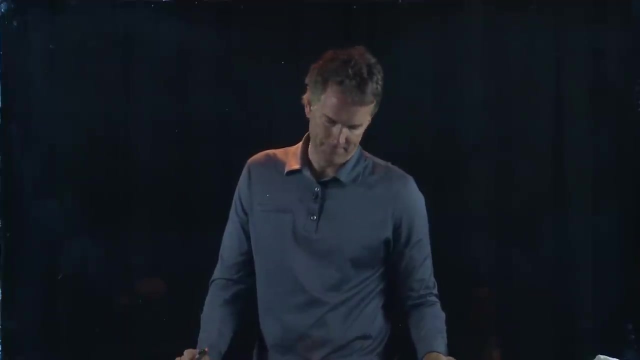 This is the universal speed limit for the universe. Okay, This is as fast as you can go. Okay, Let's think about intensity. Okay, This is as fast as you can go. So, when we talk about electromagnetic waves and we talk about these things carrying energy, 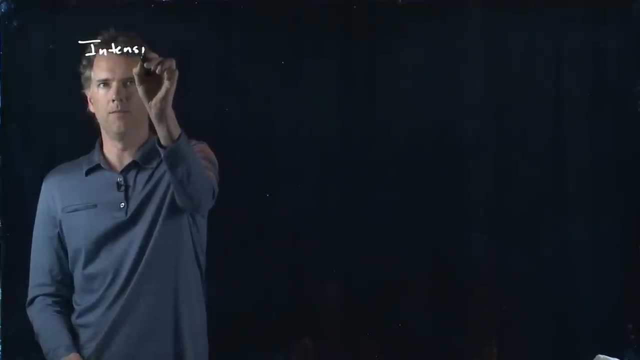 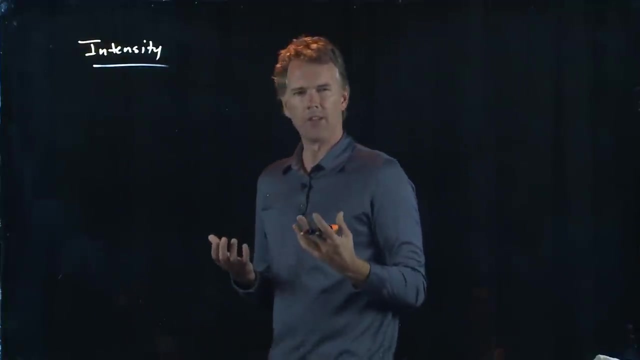 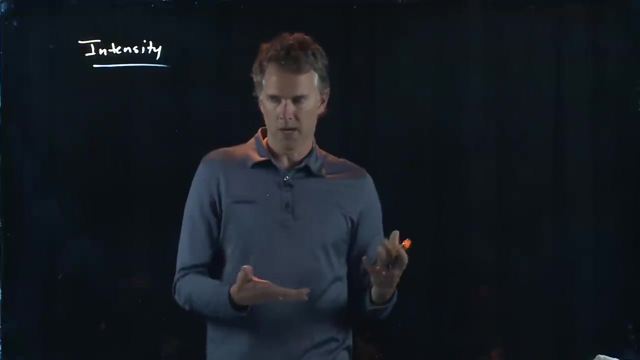 we need to talk about intensity of the electromagnetic wave. So you're familiar with this idea, right, When you go out and lay in the sunshine, you get warm, Okay, But that sunshine that is hitting the ant on the ground warms up the ant. 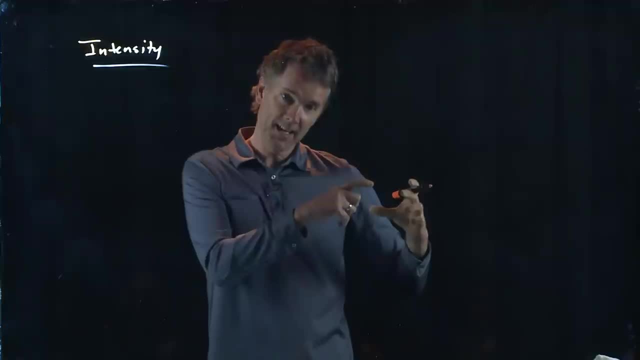 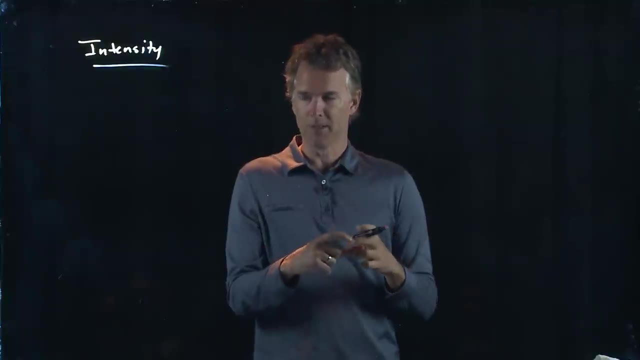 But if I take a big lens right and I focus a whole bunch of sunlight onto that poor little ant, I can in fact burn up the ant right, And you've probably done this experiment when you were kids. So what has changed? 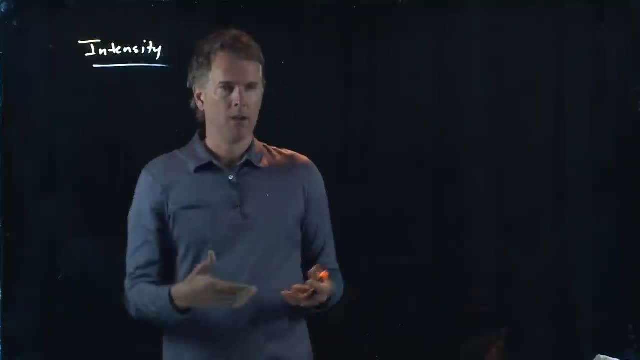 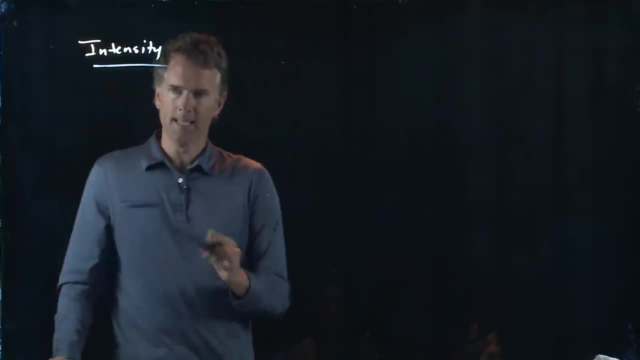 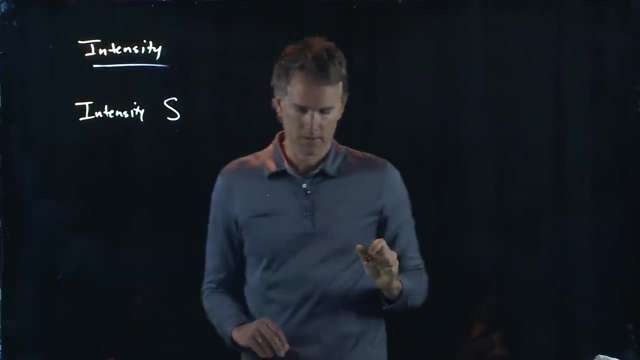 Okay, What has changed is the intensity of the electromagnetic wave at that focal spot. So let's talk about intensity. Intensity: we actually are going to write, so we're going to be writing the energy time every three minutes. We're going to divide the energy with an S. Okay, 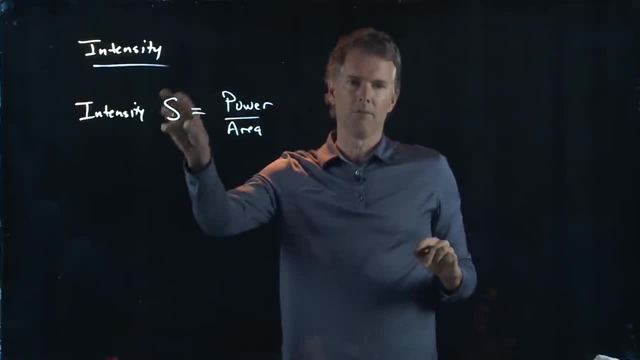 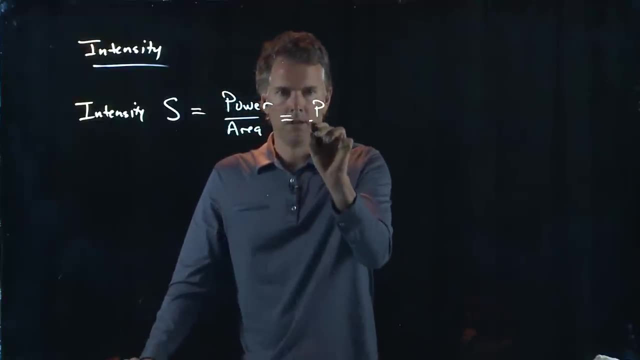 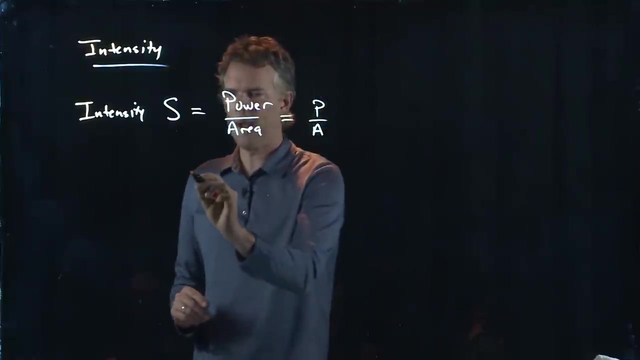 An S is power divided by area. The reason that we use an S is this comes from something called the pointing vector, and the pointing vector traditionally they use an S. So power is P, Area is A, But we know that power is energy per time. 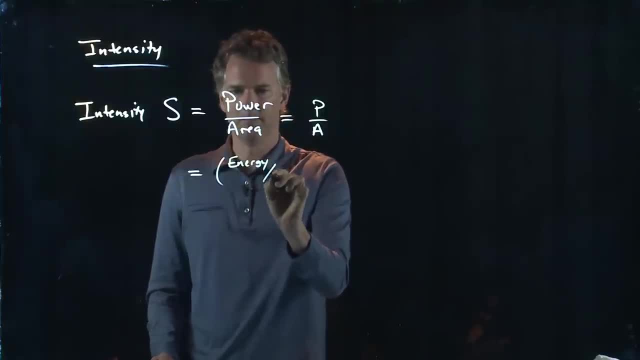 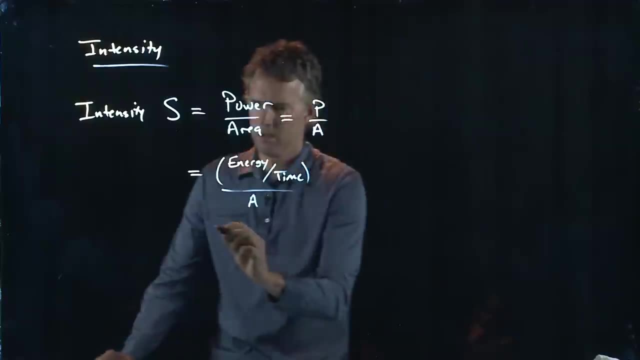 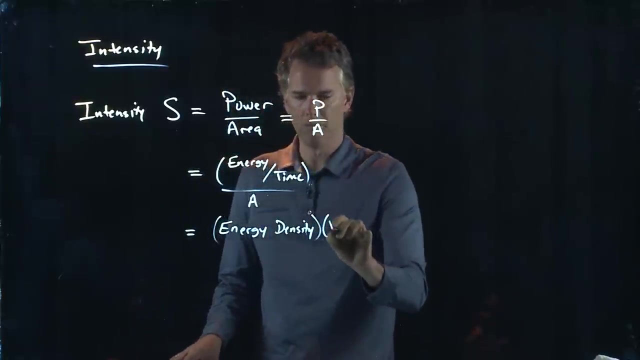 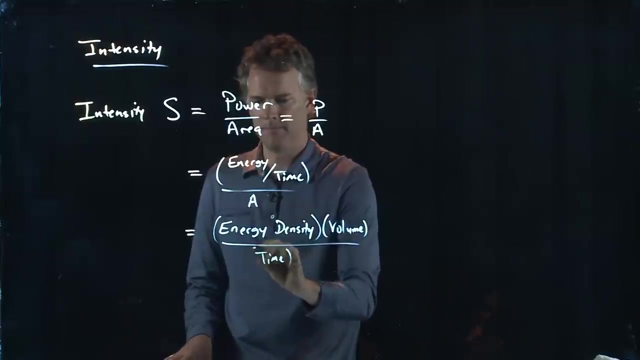 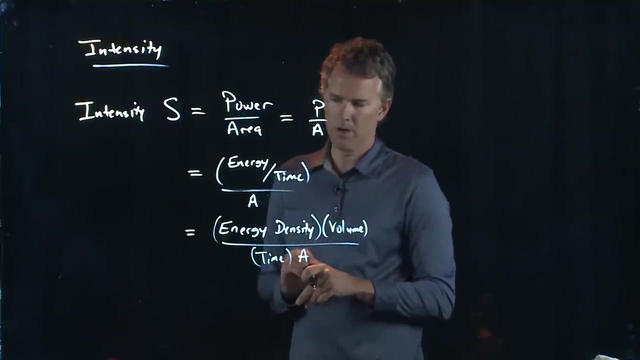 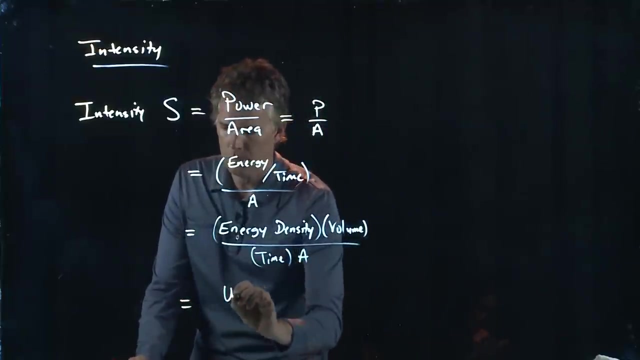 time And we're going to divide that by area A. Okay, Energy per time is the same as energy density times volume divided by time times, area A. Okay, And we know what some of these things are. We know what energy density is. Energy density was our good old U. What about? 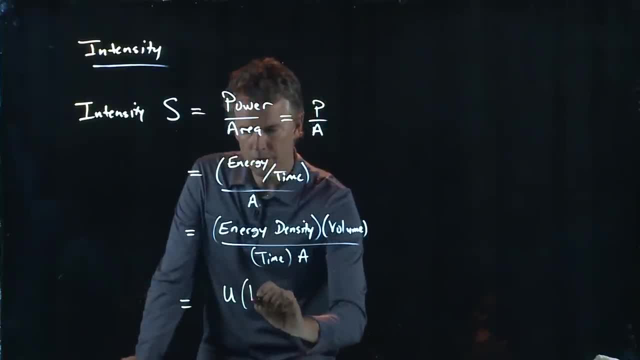 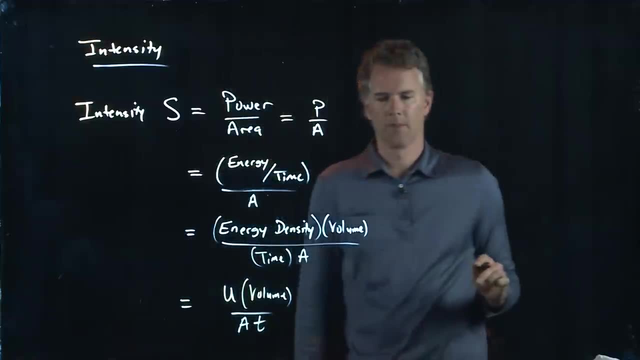 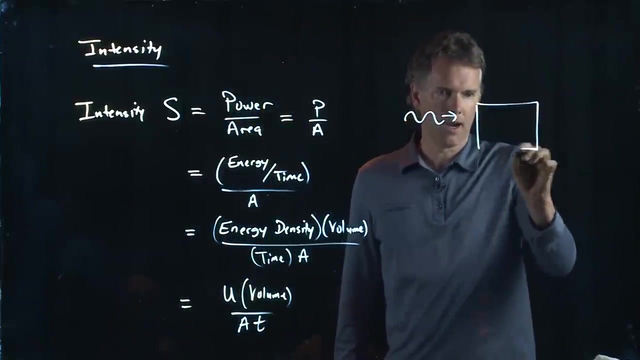 volume. Volume, we're not really sure yet, so we'll leave it right there. Time is just T, So what do we mean by volume? Well, let's think about an electromagnetic wave propagating along. Okay, This electromagnetic wave propagating along is going to occupy a region of space. 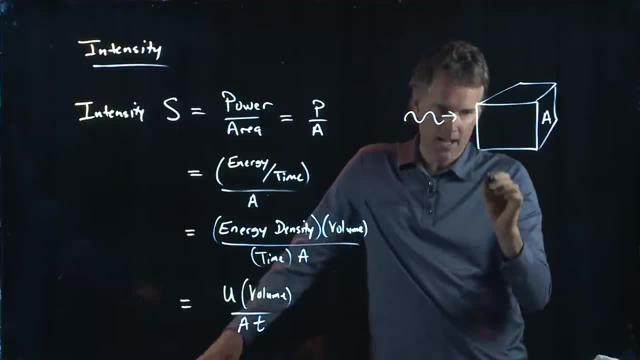 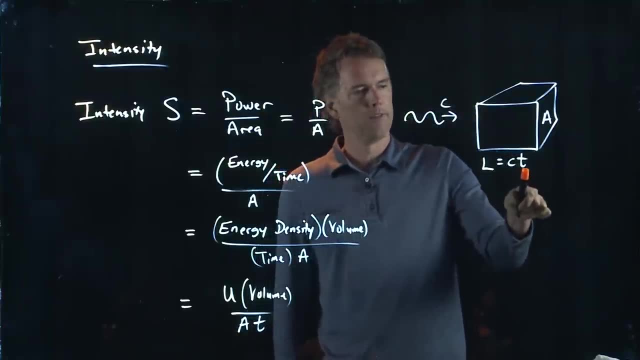 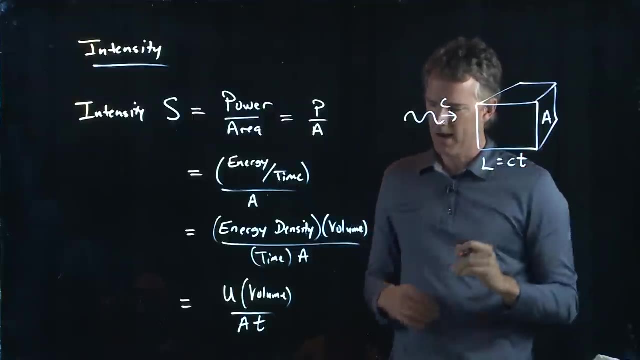 that has a cross sectional area A to it, it, and it has a length here, l, which is equal to how fast it's moving. for how long It moves at c, it does that for a time t, that's the length of this box. So what's the volume of? 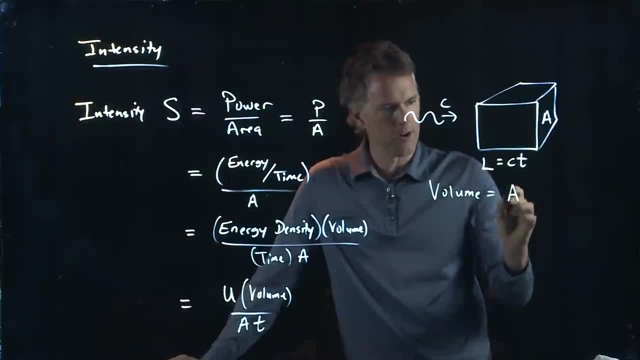 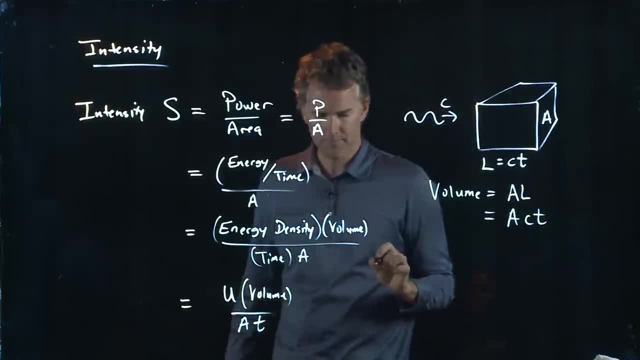 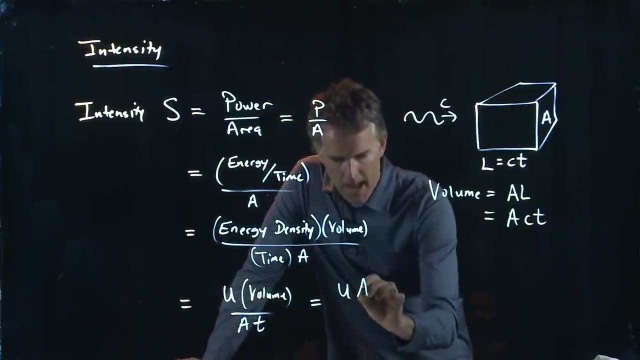 the box. Well, it's just cross-sectional area a times the length l, so it is a c t. So what do we get here? We get u times the volume a, c, t, and we're going to divide it by a. 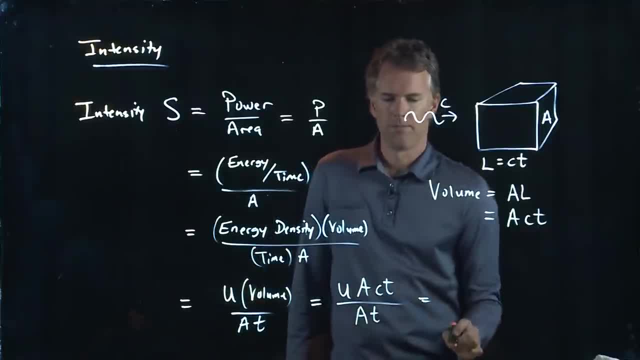 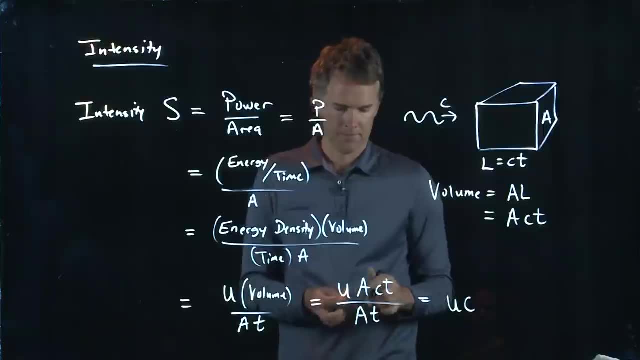 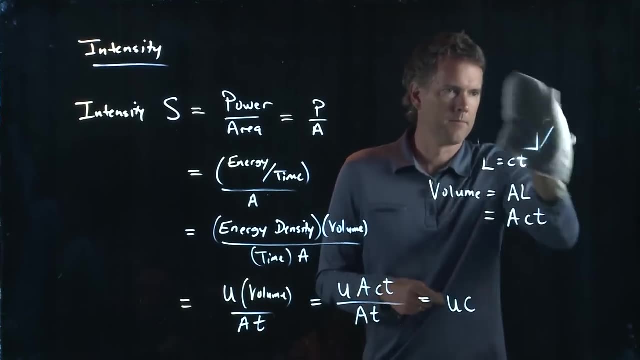 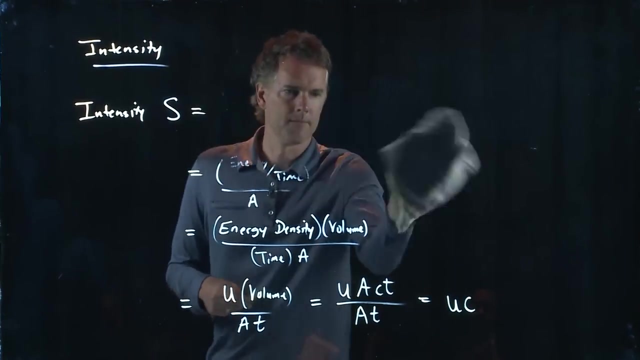 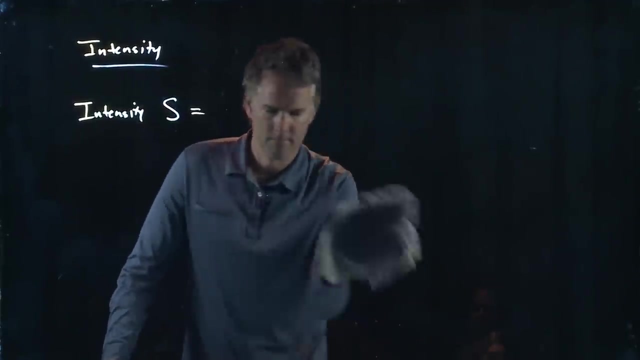 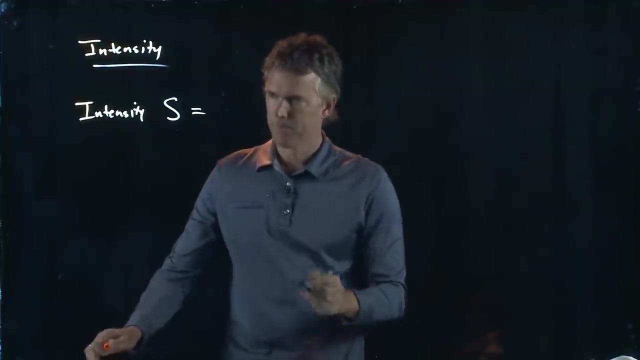 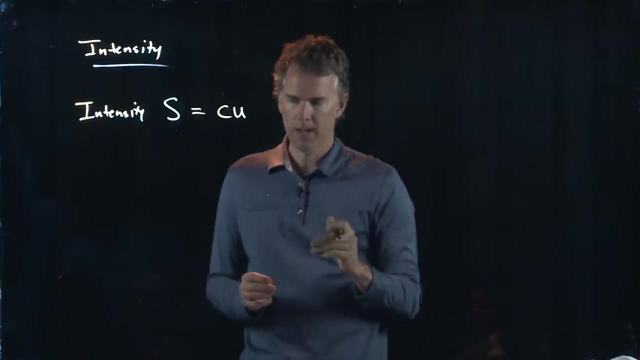 t, The a's cancel out, the t's cancel out and we just get u times c. Okay, So S is equal to u times c, But we know exactly what u is. u is. u is a t c. 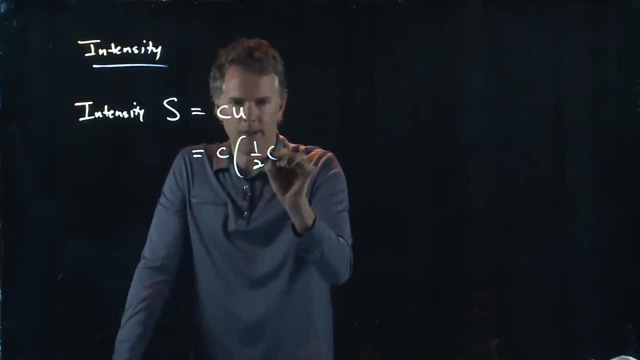 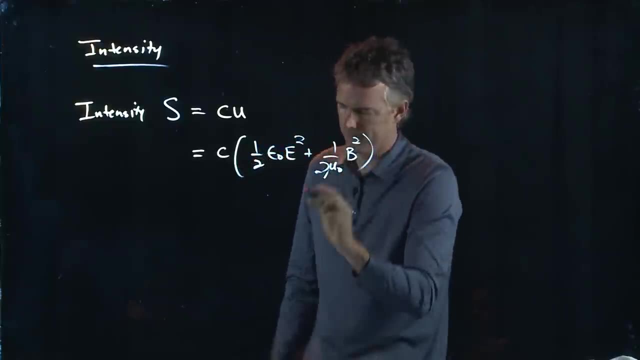 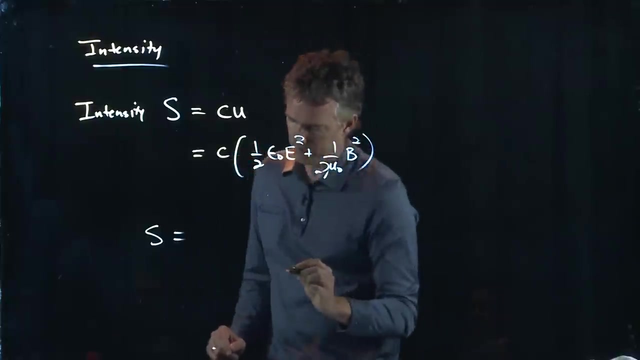 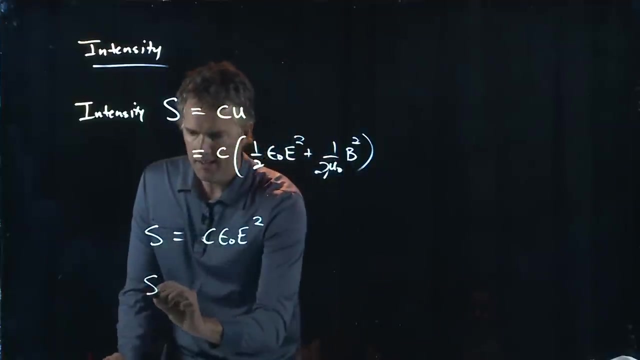 is 1 half epsilon-naught e squared plus 1 over 2 mu-naught b squared. But those are equal, and so we can just double one of them. We can say s is equal to c epsilon-naught e squared, or s is equal to c over mu-naught b squared. 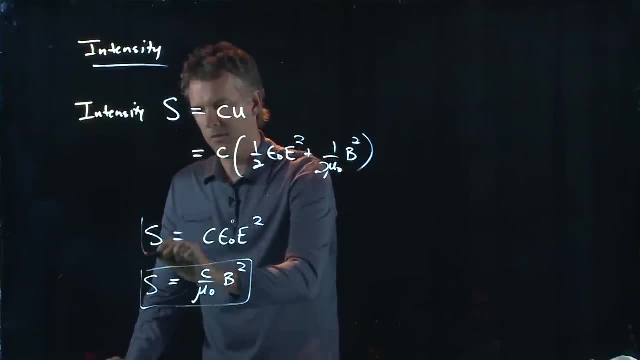 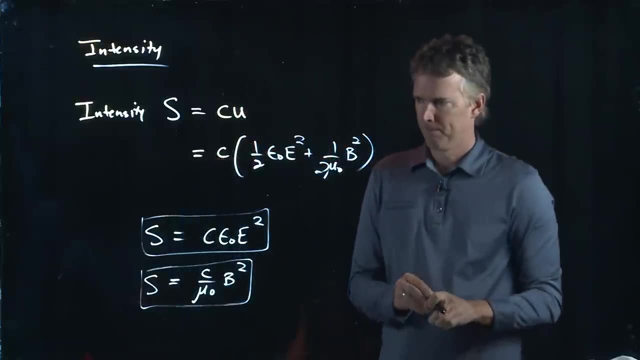 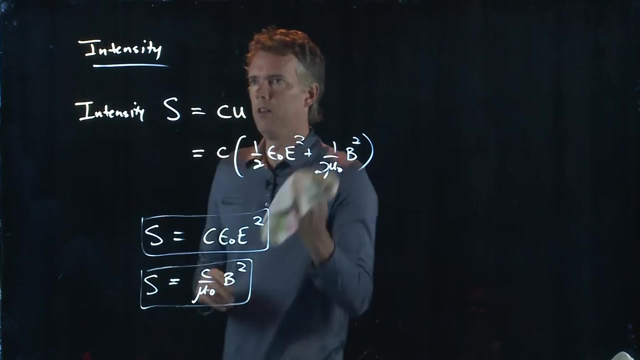 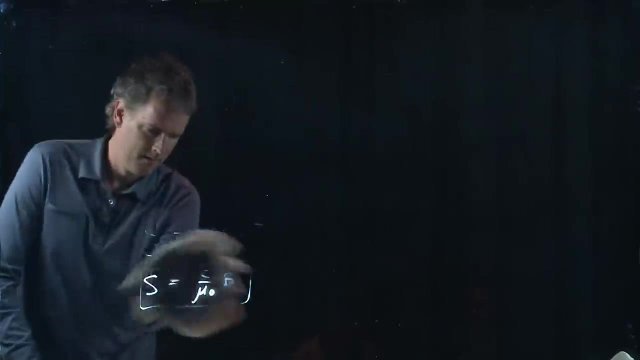 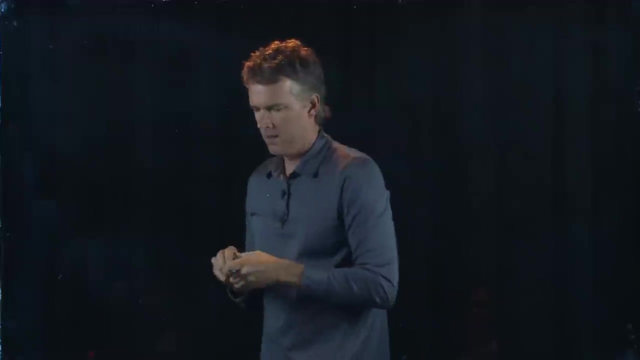 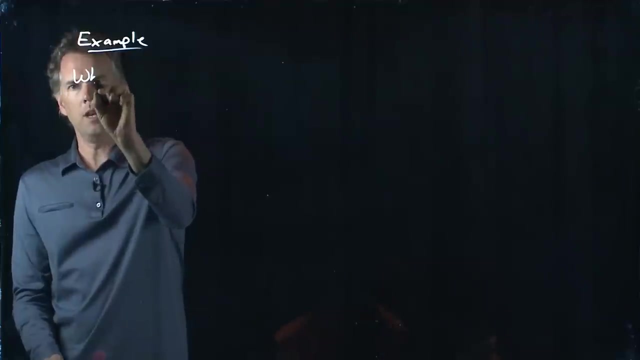 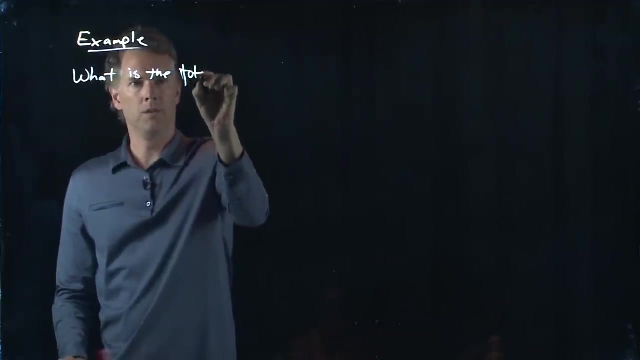 Those are equivalent statements. Okay, so, with this information, now let's see if we can understand something about our sun. How about something relevant to our particular situation on the earth? How about the sun? And let's ask the following question: What is the total power output of the sun? 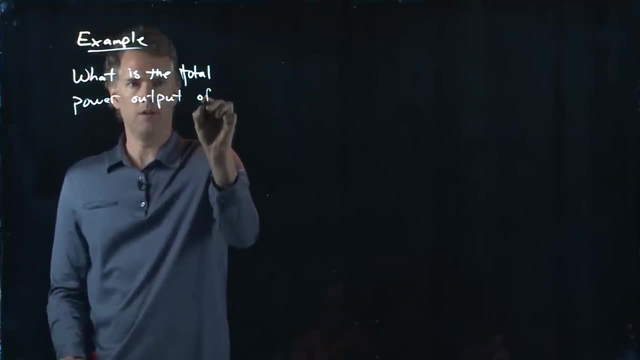 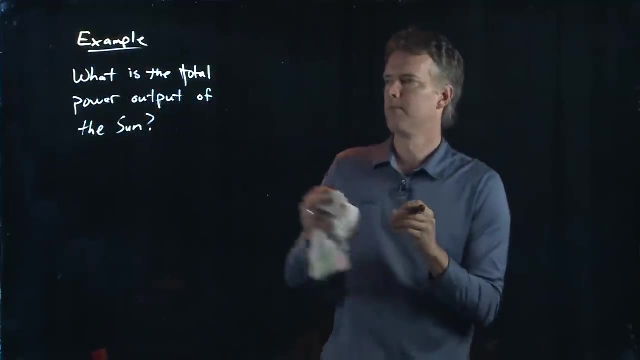 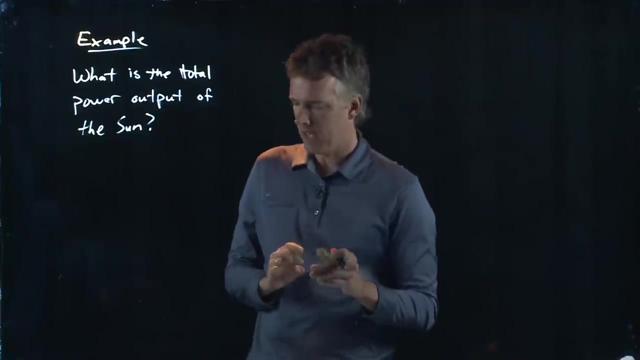 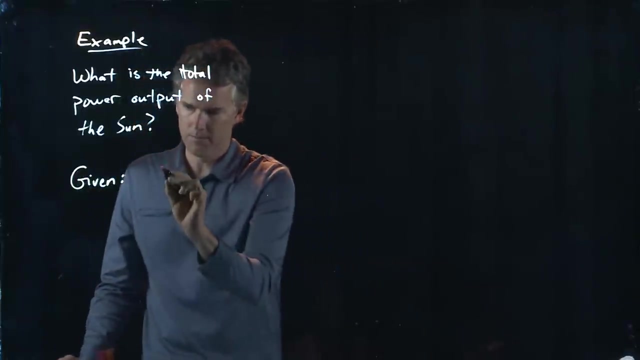 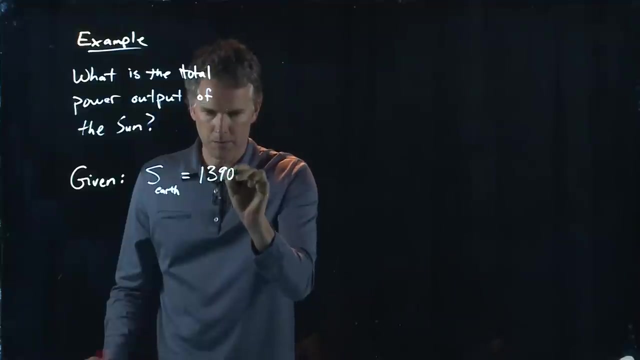 What is the total power output of the sun? What is the total power output of the sun? sun, What is the total power output of the sun? And let's say that we know a couple things. We're going to say that the intensity at the earth is equal to 1390 watts per square meter. 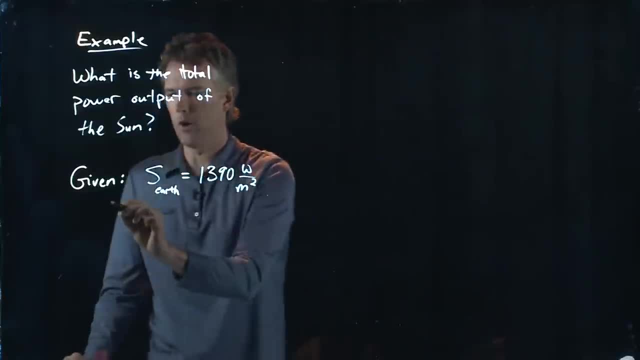 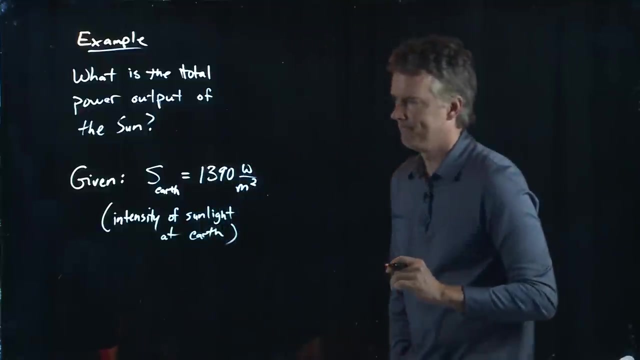 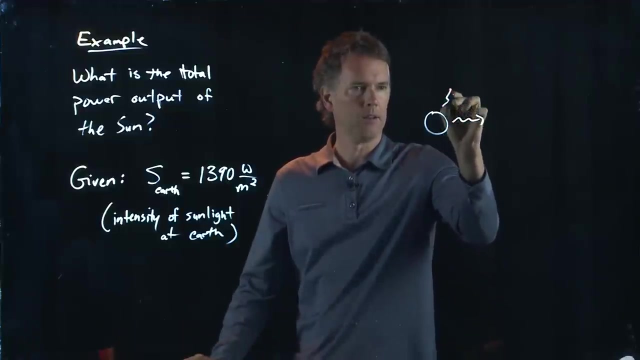 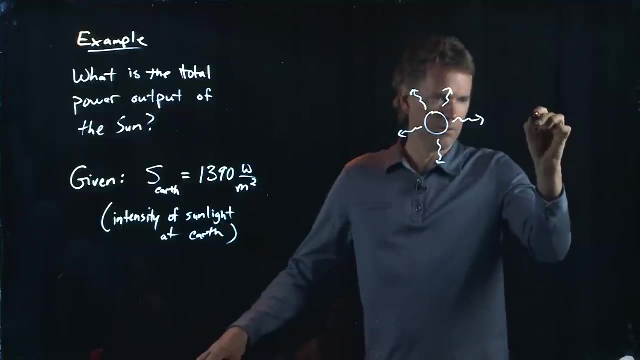 This is the intensity of the sunlight at the earth. Alright, let's draw a picture of this thing. Here's our sun. It is spitting out electromagnetic waves in all directions, Some of those we collect right here on the earth And we know. 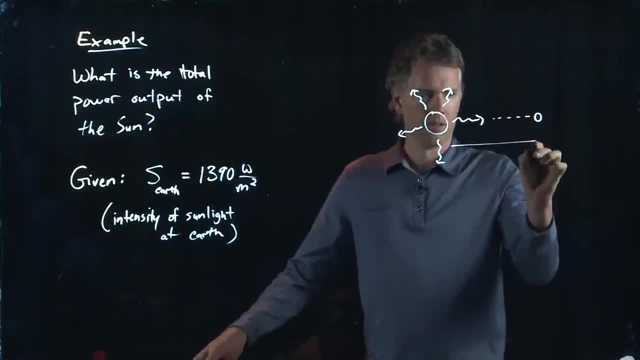 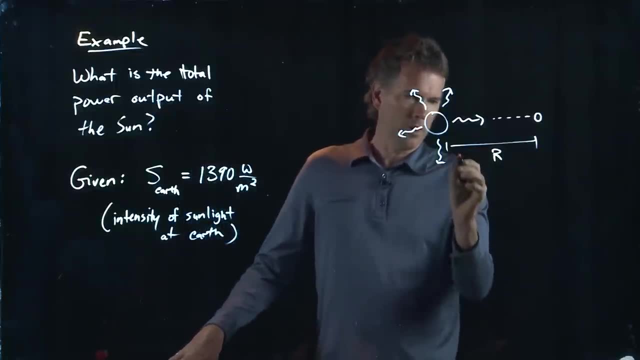 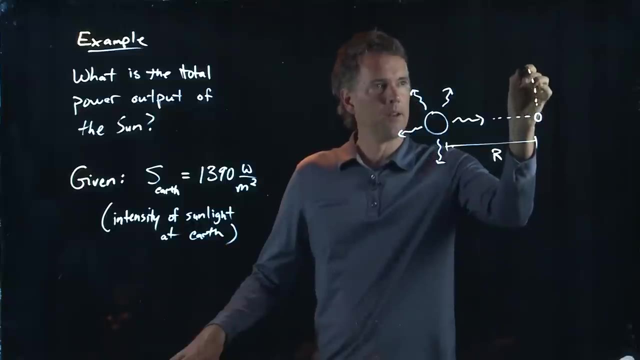 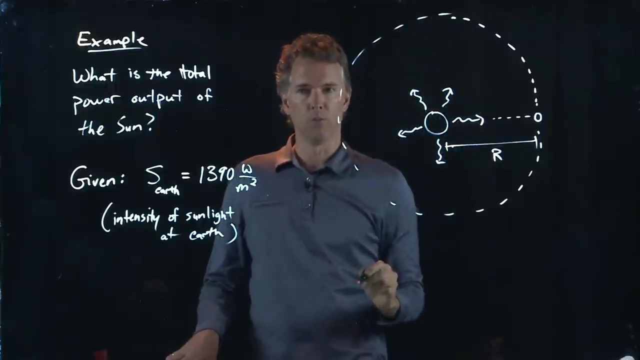 that we are a distance capital R- away from the sun. So if I want to think about how much power is emitted by the sun in total, I have to worry about this sphere right here of radius capital R, The total power emitted through. 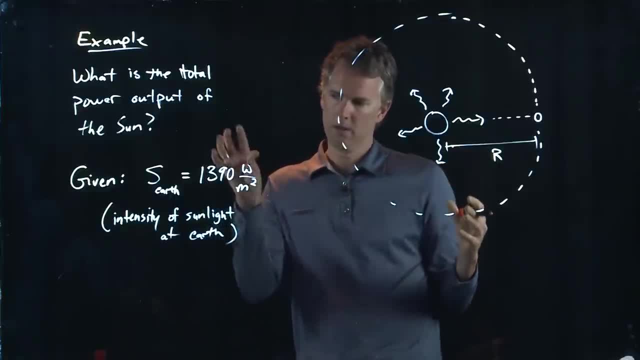 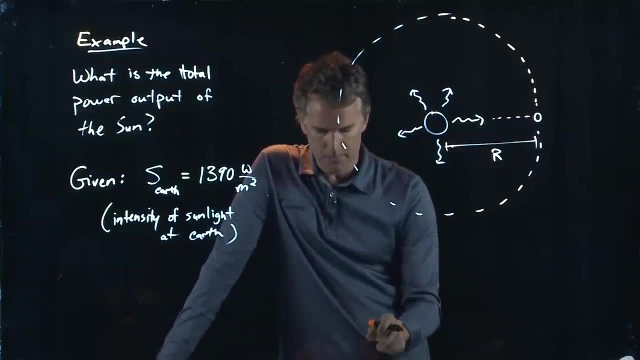 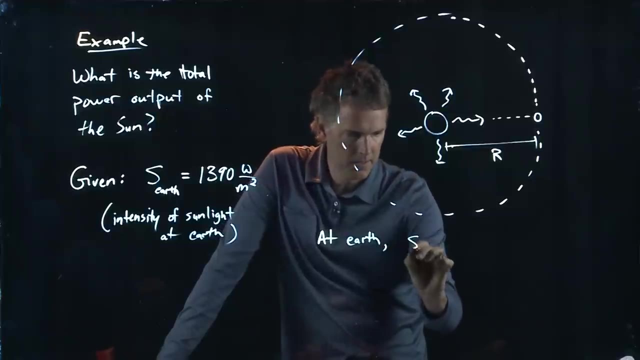 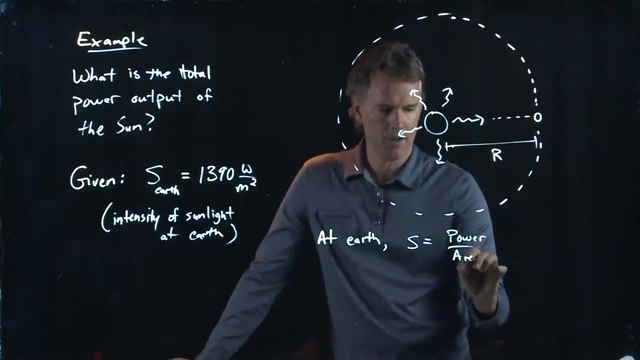 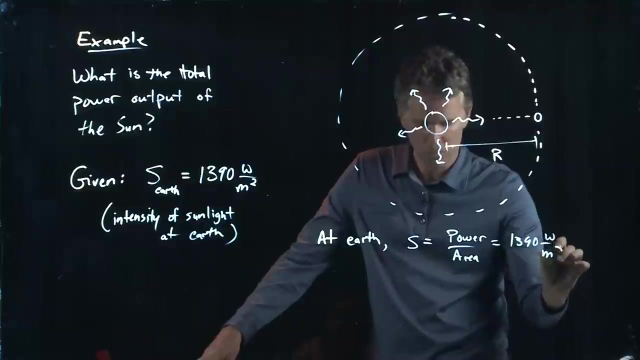 that sphere is hopefully something we can calculate based on the intensity at the earth. Alright, how do we do it? Well, at the earth, the intensity that we measure is just power over area, And that is what we said was 1390 watts per square centimeter, But the total 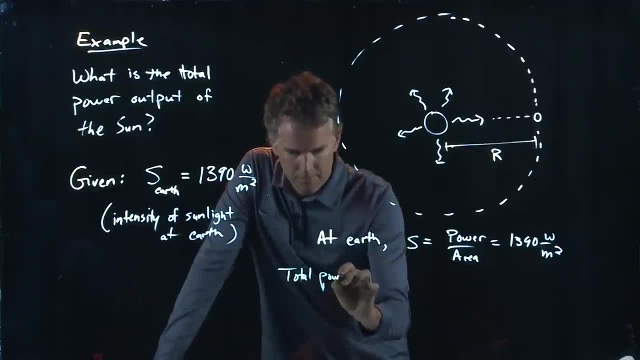 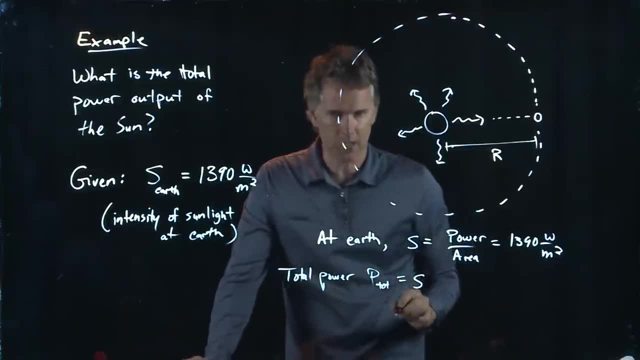 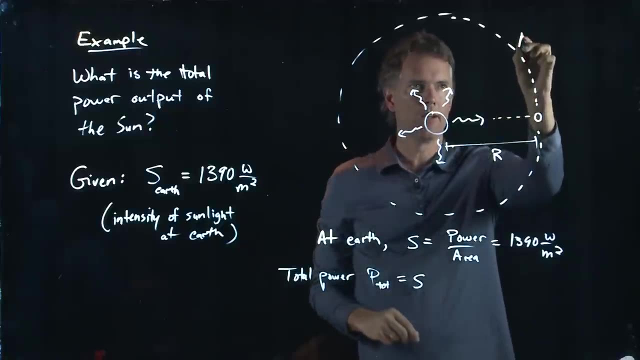 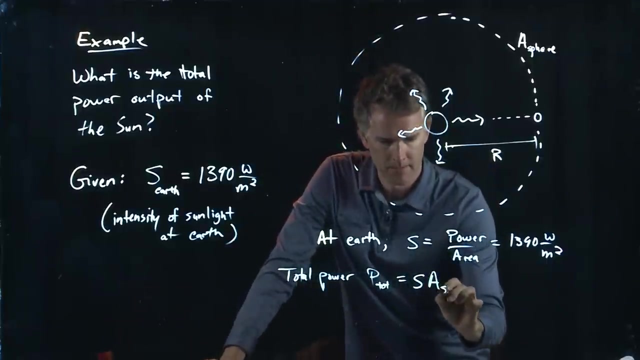 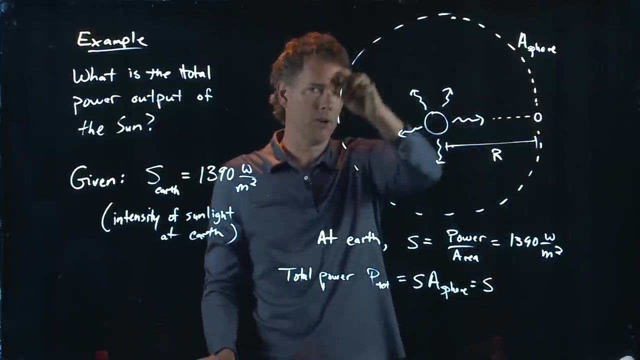 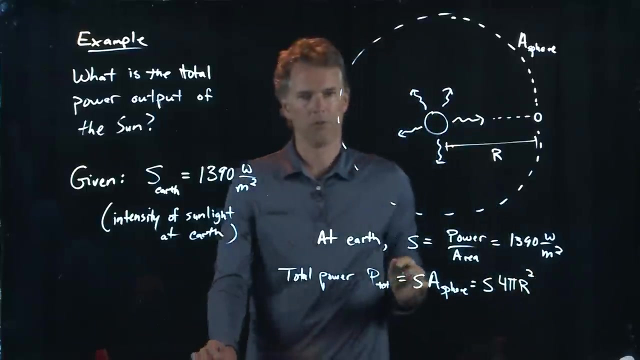 power coming out of the sun is going to be that intensity that we measure here, multiplied by the area of this giant sphere. Okay, We know S What is the area of this giant dashed sphere? It is 4 pi capital R squared. Now take our. 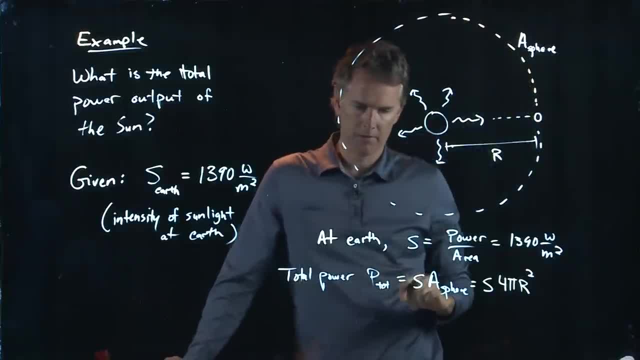 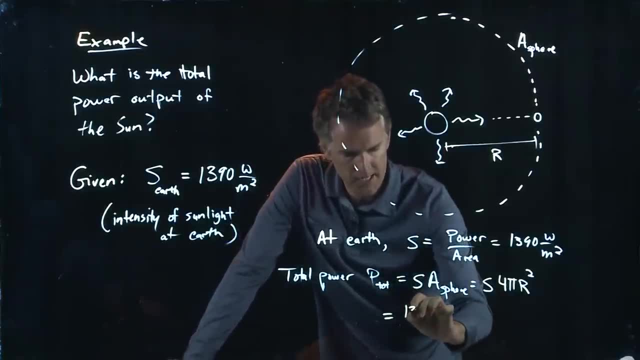 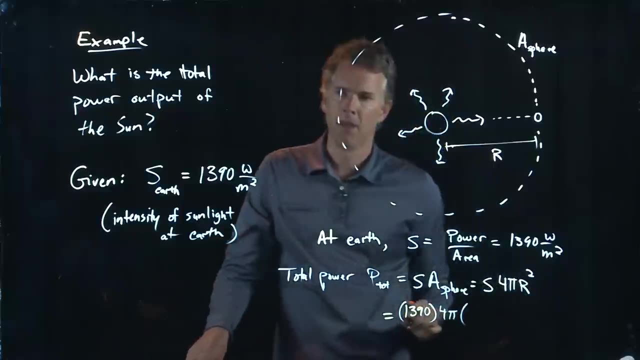 little intensity and multiply it by the area of this sphere And, as you can imagine, that's going to be a pretty big number. So we have 1390 for S, We have a 4.. We have a pi And now we need this number, R, And this you can look up in your textbook. How far is the? 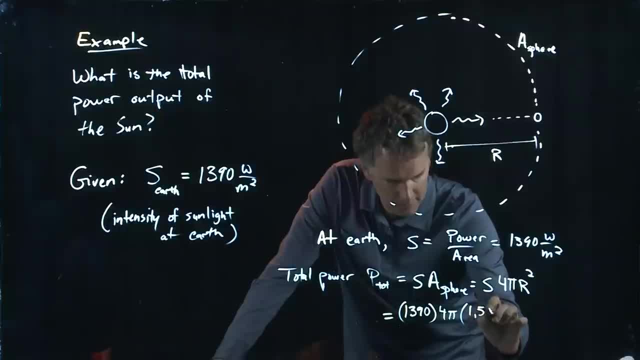 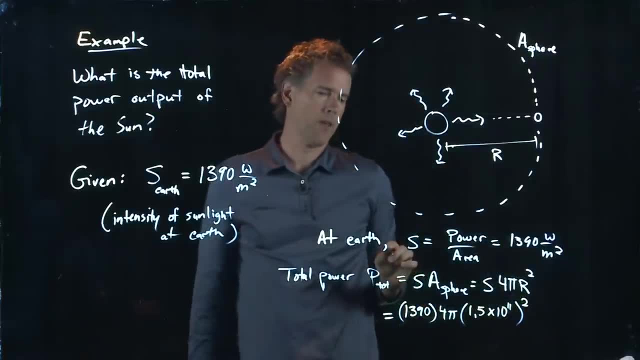 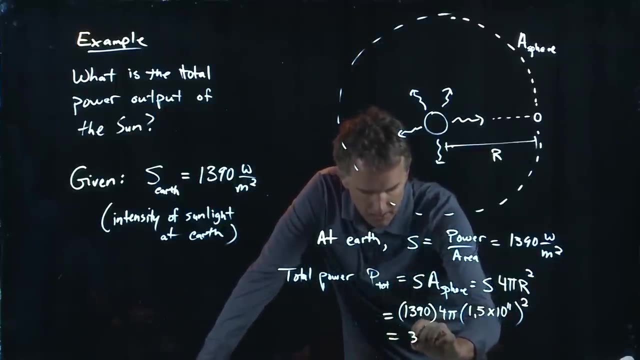 earth from the sun. It is 1.5 times 10 to the 11 meters, And so you're going to square that, And somebody double-checked my calculation. I ran this earlier but maybe you can double-check. I get 3.93 times 10 to the 26.. 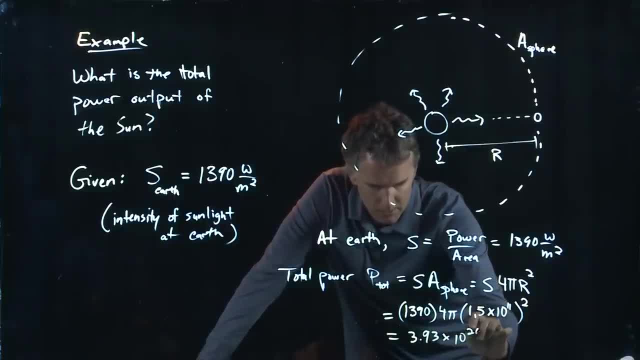 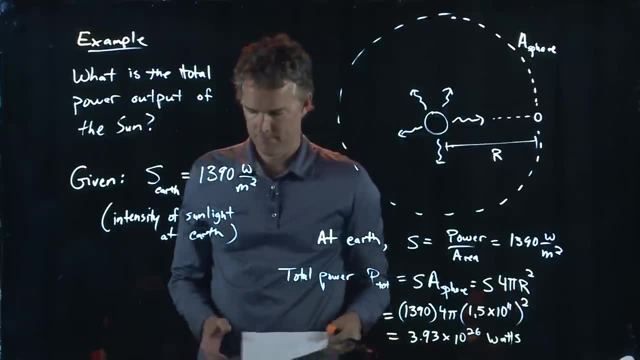 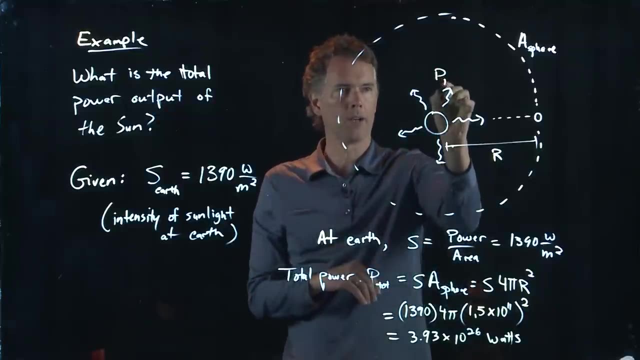 Okay, We've got a 3.93.. Okay, What's the distance? What's the area of the sun? I don't know, I don't know The area of the sun, I don't know. Okay, watts, 3.93 times 10 to 26 watts for the total power coming out of the sun, which is a pretty 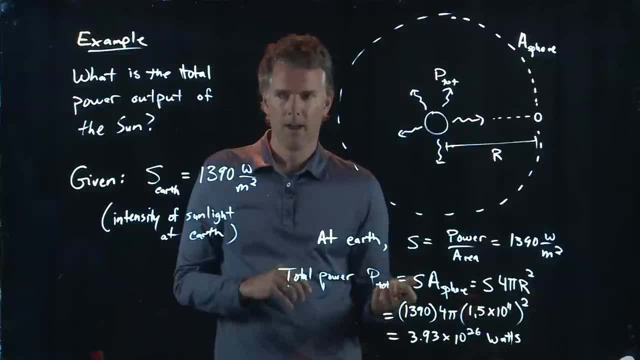 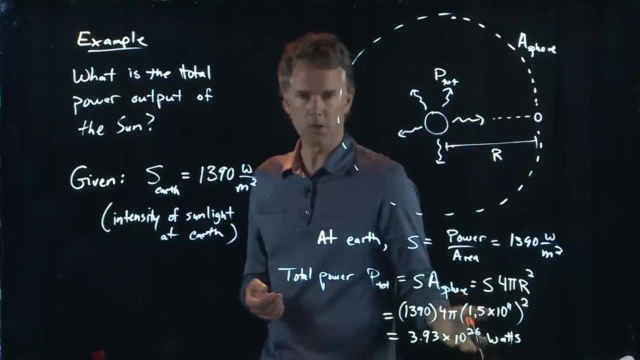 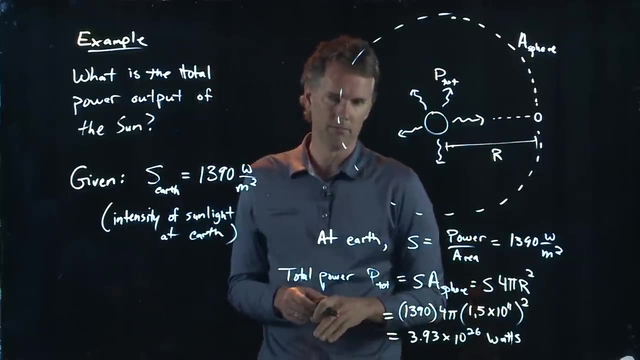 big number right. When we were talking about how much power your hairdryer uses, it was like one and a half kilowatts. right, It was like 10 to the 3 watts. And here's something that is 23 orders of magnitude bigger. So, like you would expect a lot of power coming. 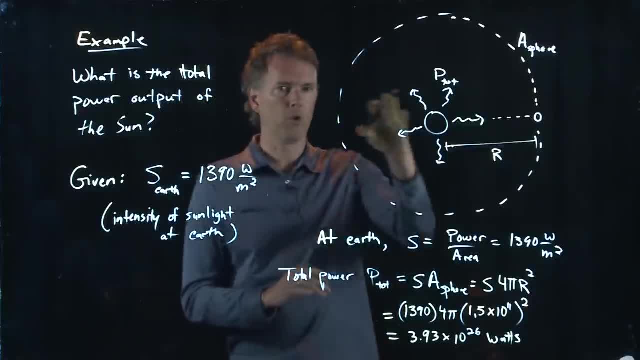 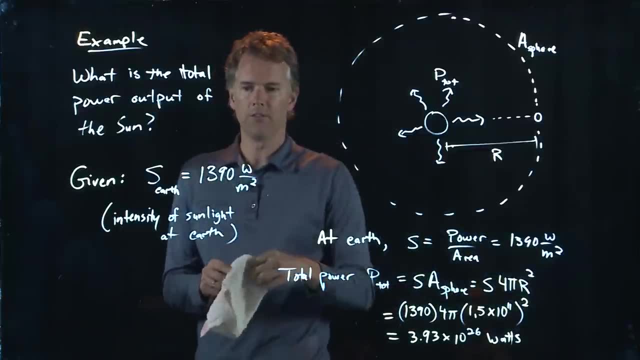 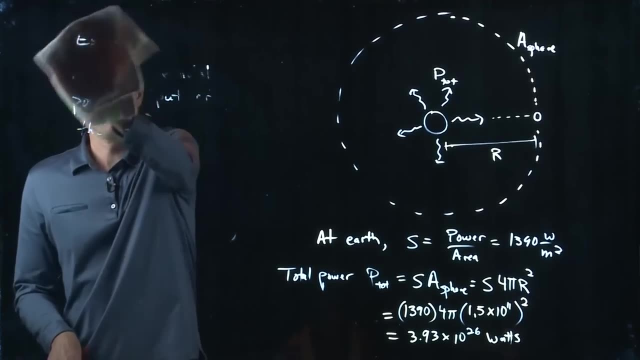 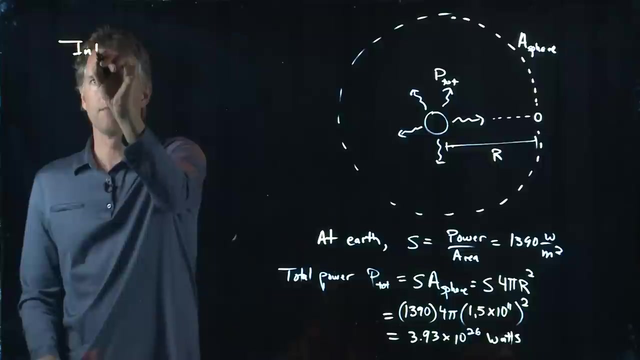 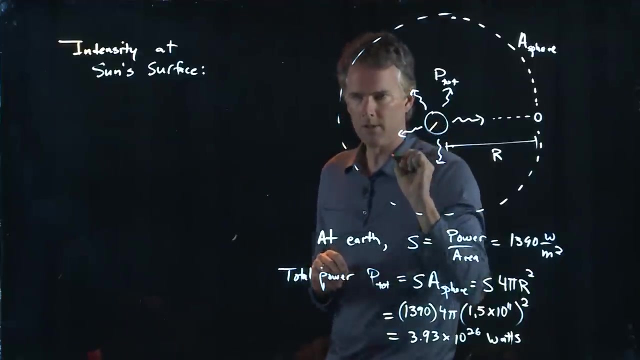 out of the sun? Okay, but if that's the total power coming out of the sun, let's ask a follow-up question: What is the intensity at the sun's surface? Okay, how do we do that? Well, we're going to need to know the radius of the sun, And 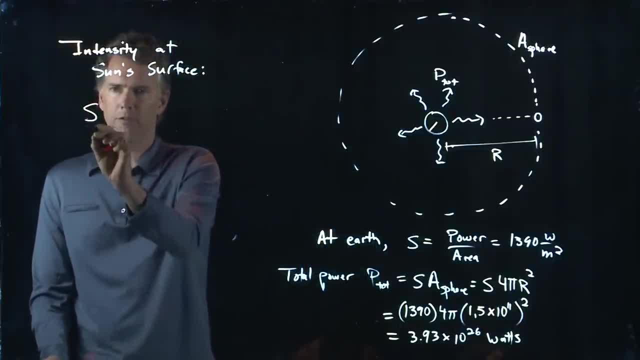 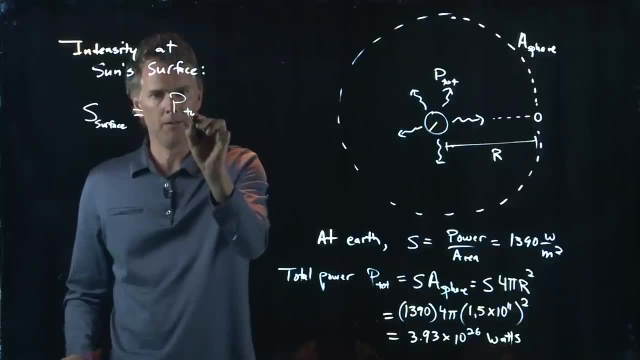 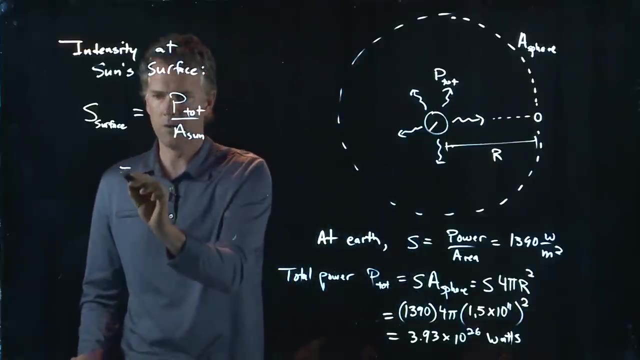 if we do that, then we can calculate the intensity at the sun's surface, because it's just going to be that total power divided by 10 to the 3 watts, Okay, And we know the total power And the area of the sun is 4 pi times the radius of the 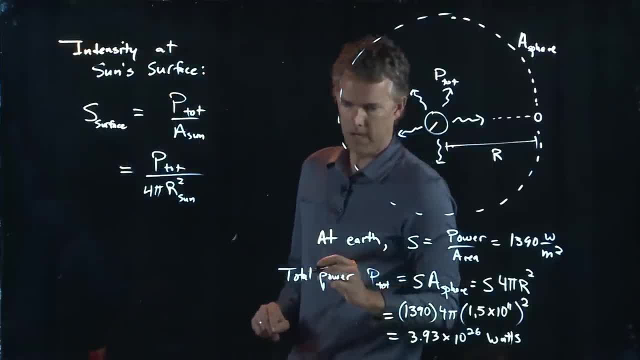 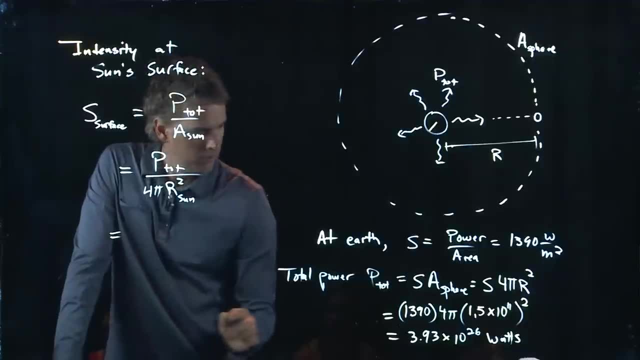 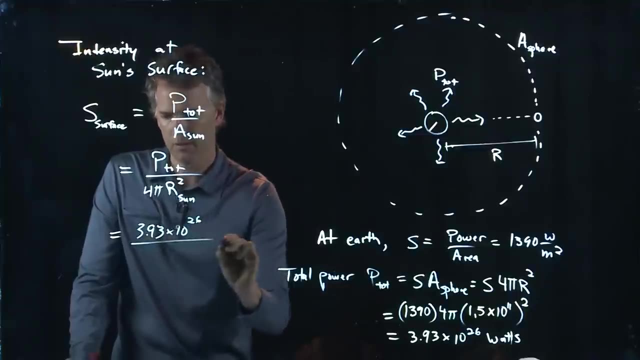 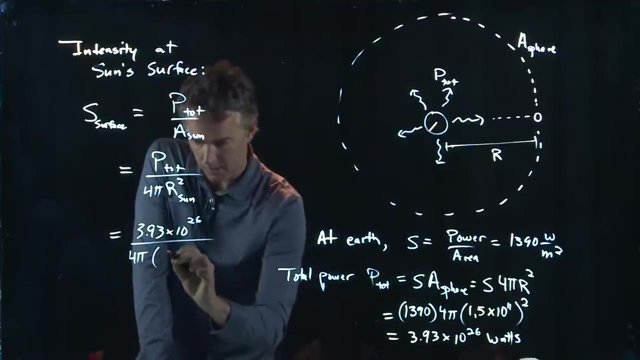 sun squared. And so now again you can look up that number And let's punch it in right here. So P total, we said, was 3.93 times 10 to the 26. We've got a 4 pi And then we have R squared which, if you look it up, is 6.96 times 10. 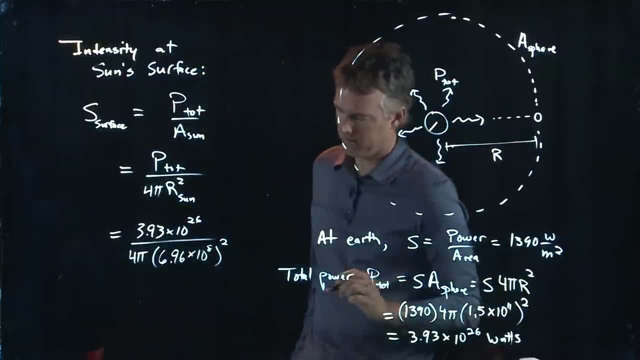 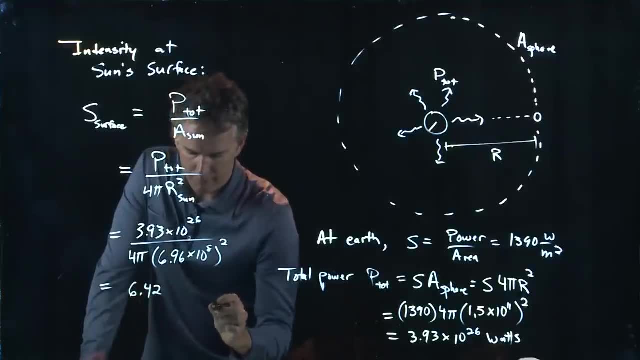 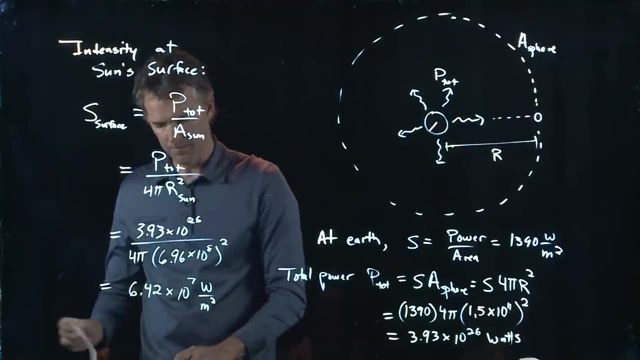 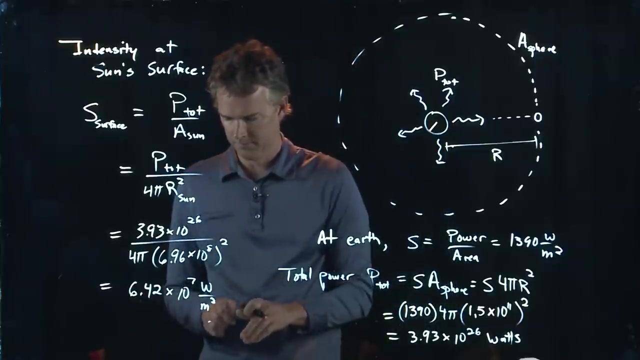 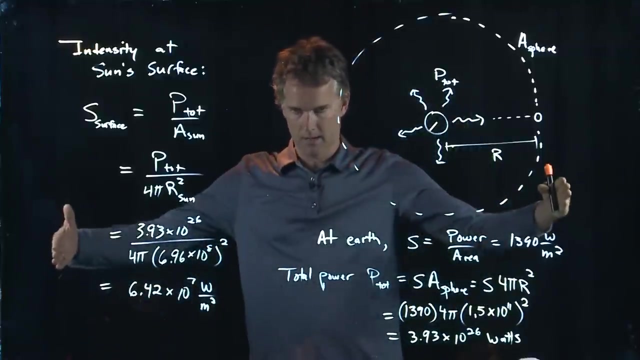 to the 8 meters. That's the radius of the sun, And if you put all this together you get 6.42 times 10. to the 7 watts per square meter. Okay, Which is a big number, right? Think about a square meter. It's like that And it's going. 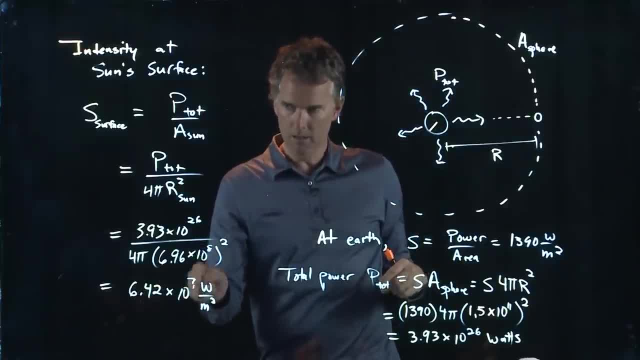 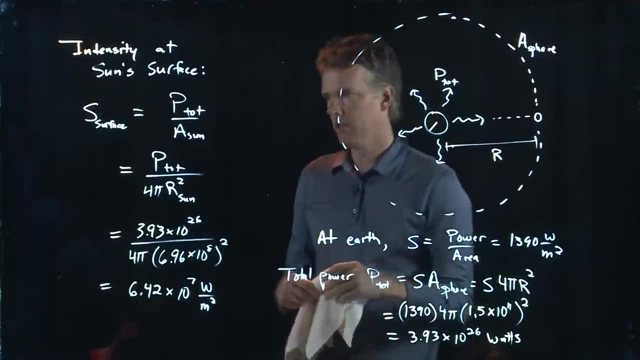 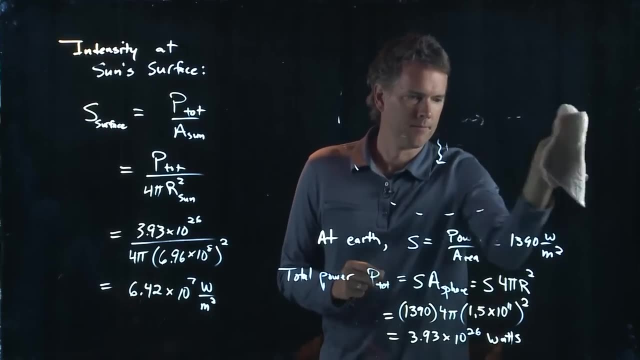 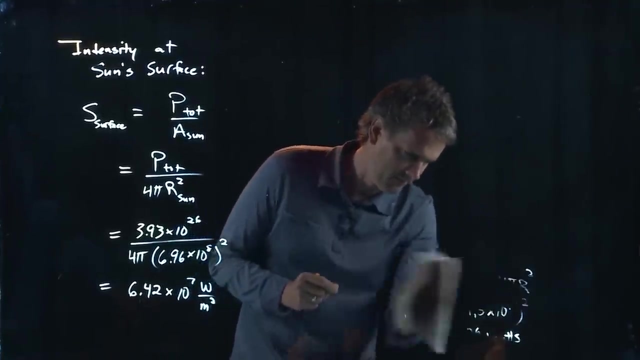 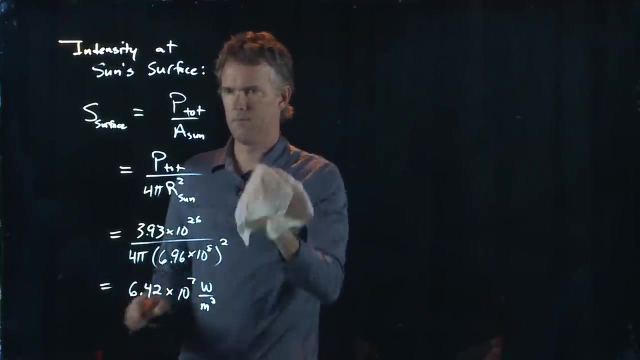 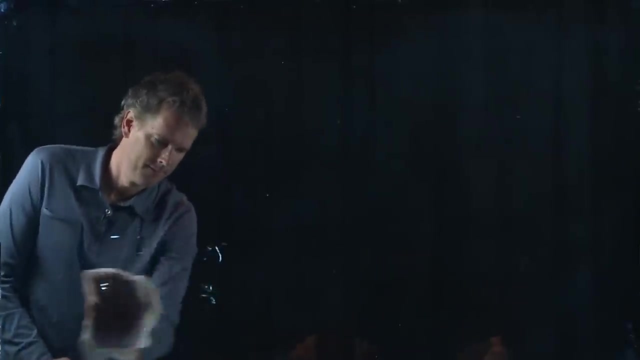 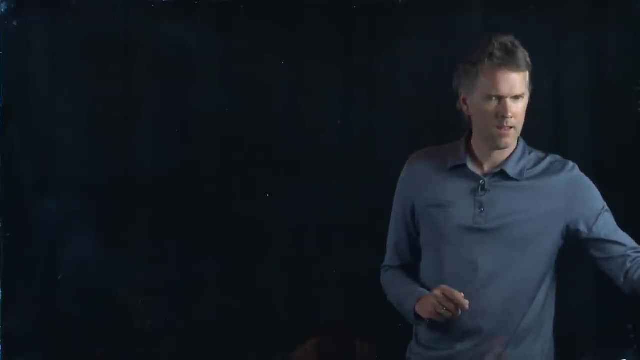 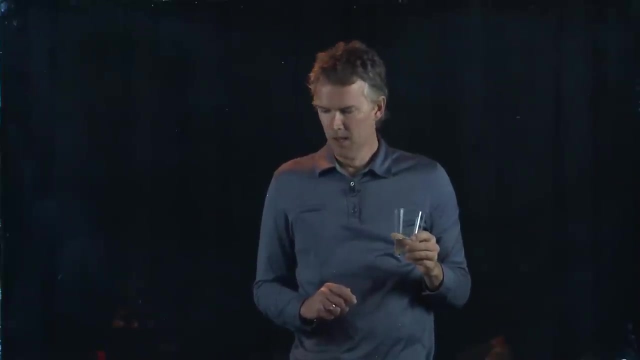 to have 64 million watts in that square meter. That is a lot of electromagnetic intensity, Okay, So all right, Okay, Question for me. Yeah, Somebody's got a question out there, Ian. Oh, never mind, I sent that one in myself right here. 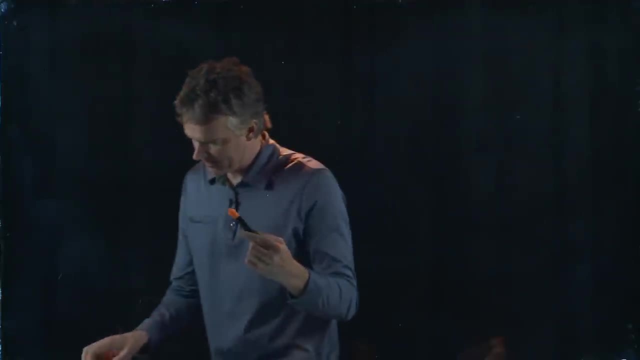 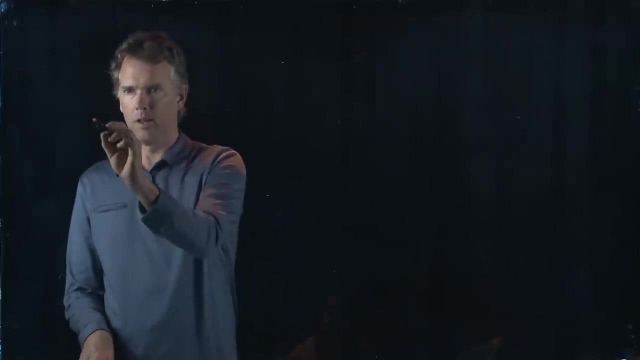 Did somebody get a different number for that last calculation? I did: Okay, what did you get? I got 4.49.. That doesn't sound quite right, but let's just double-check. So we had 3.93 times 10 to the 26th, and then we had a 4 pi. 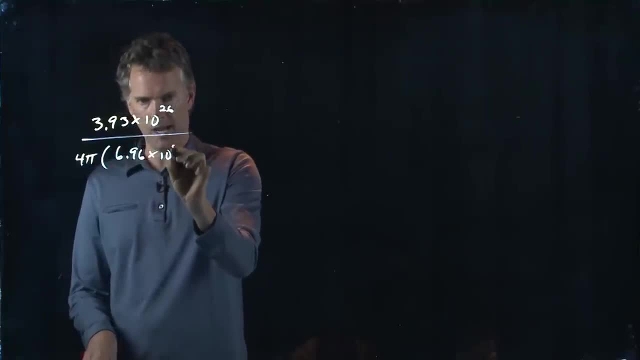 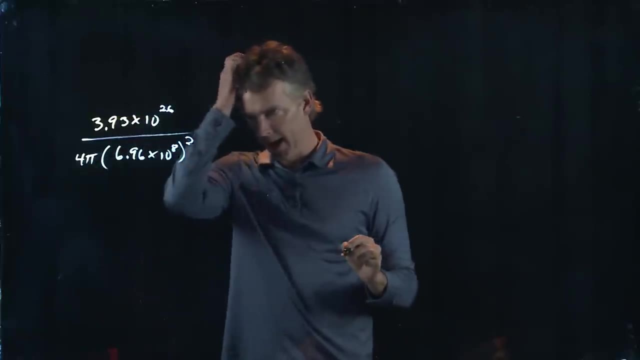 and then we had 6.96 times 10 to the 8th, but that whole thing was squared. Did you remember to square it? No, Okay, All right. good Yeah, it couldn't be that high, right? because this is going to get us like a 10 to the 16th. 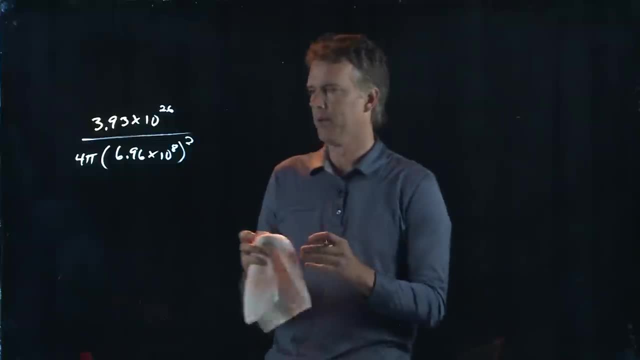 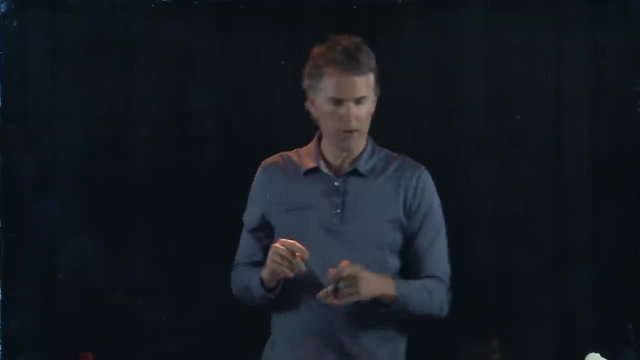 so it's got to be less than sort of 10 to the 16th, Less than 10 to the 10, which is where we ended up. Okay, Ian, ask who that was out there watching or if you're watching still. 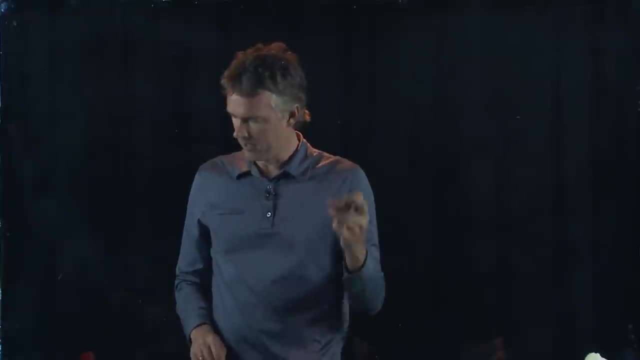 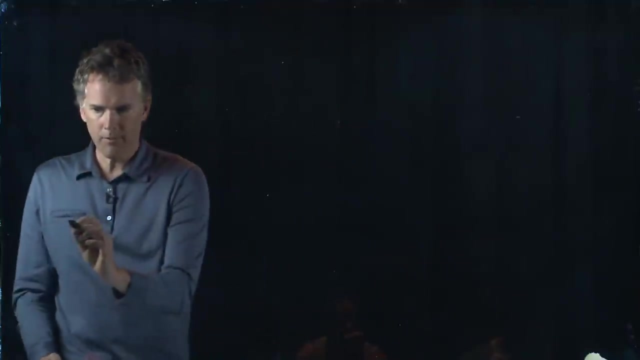 Who is that then? Who, Kelly, Kelly? All right, Hi Kelly, How are you doing? Hopefully you're sitting in a cool coffee shop somewhere watching this. So let's go back to the burning ants question, right? What we said was: 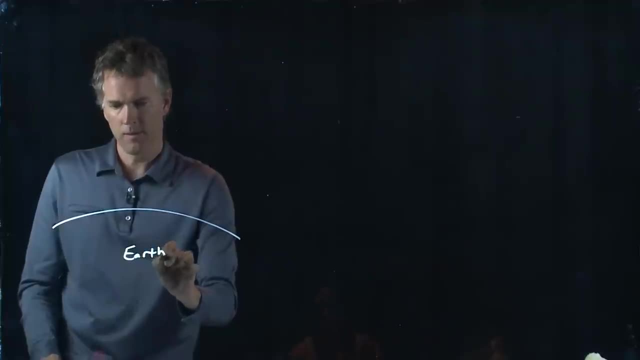 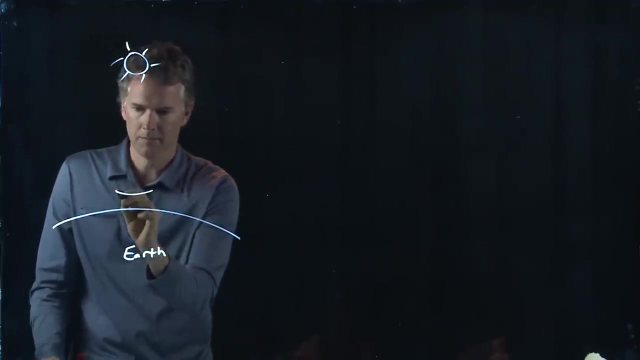 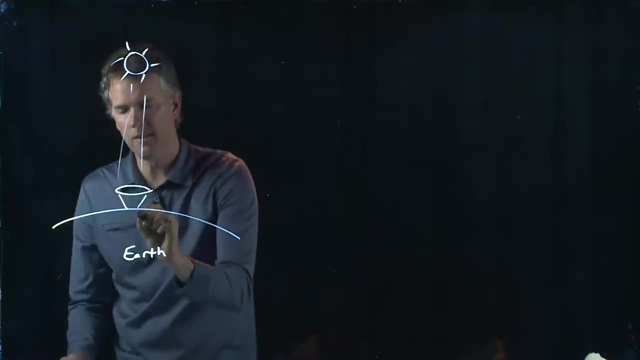 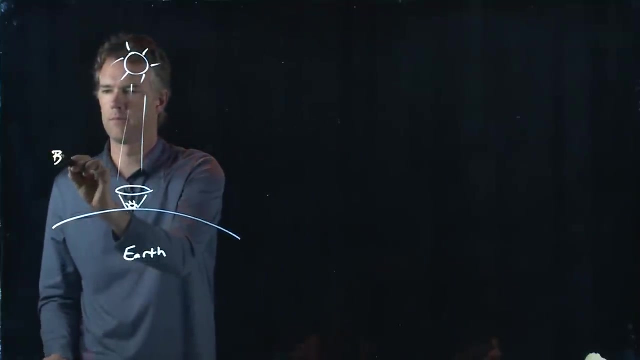 I'm sitting here on the earth and the sun is up above you, and now I take a big lens. I can in fact create an intensity here that will burn up the poor little ant right. Here's a little ant not so happy. 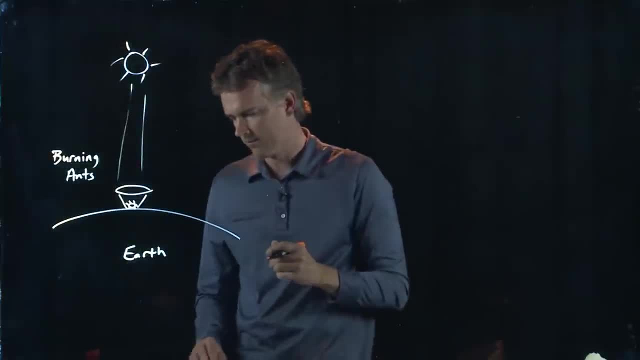 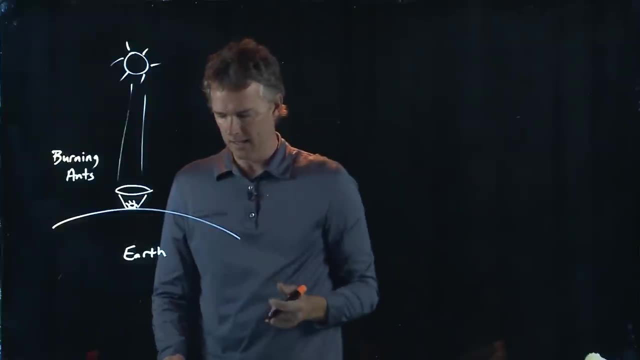 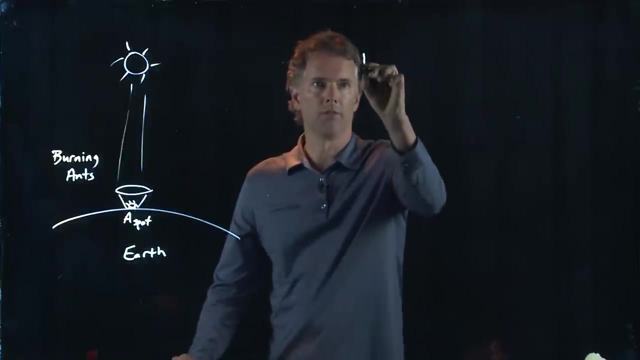 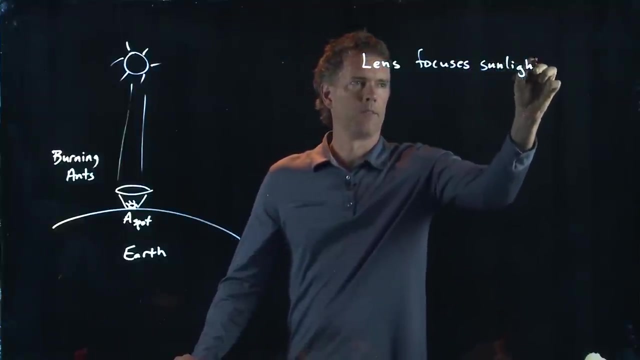 Let's see why that works. okay, And let's say that we're going to use a lens to focus the sunlight down to an area which we will call a spot. Okay, so the lens focuses the sunlight and therefore the intensity at the spot. 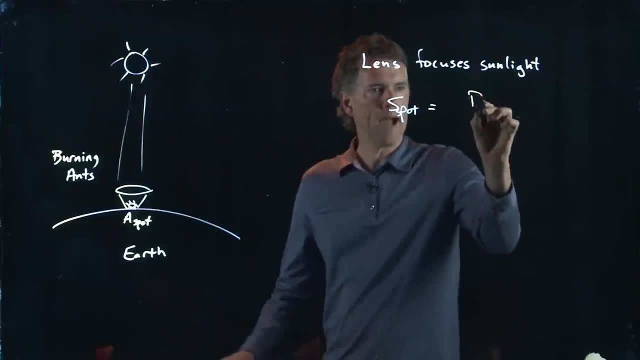 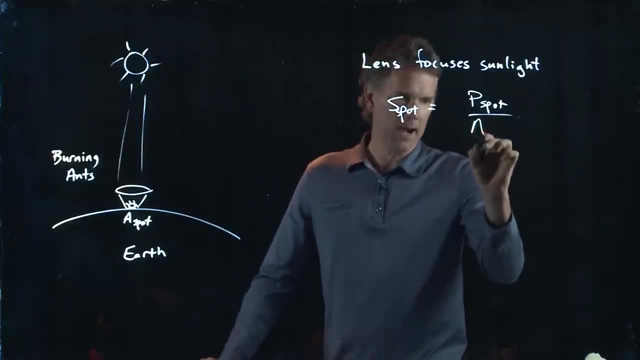 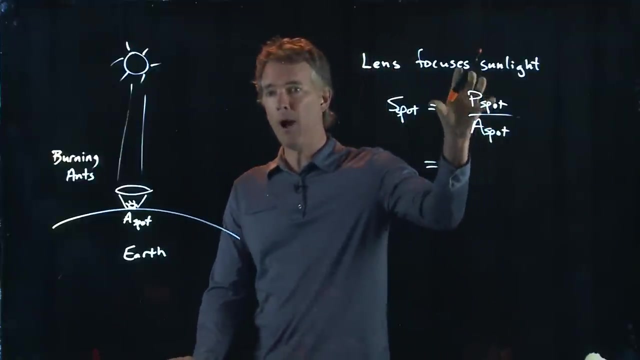 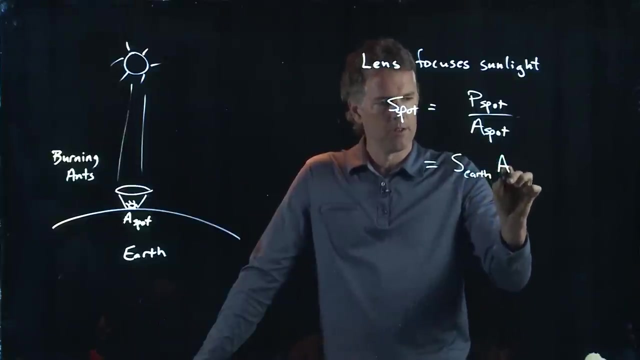 is going to be how much power you collected with your lens, or how much power is in that spot divided by the area of that spot, But how much power you collect with your lens, that is just S at the earth times, the area of the lens. 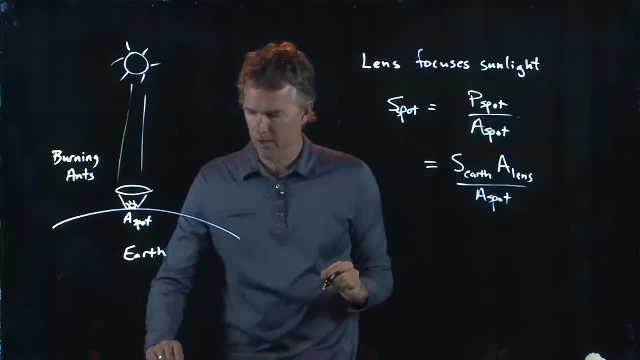 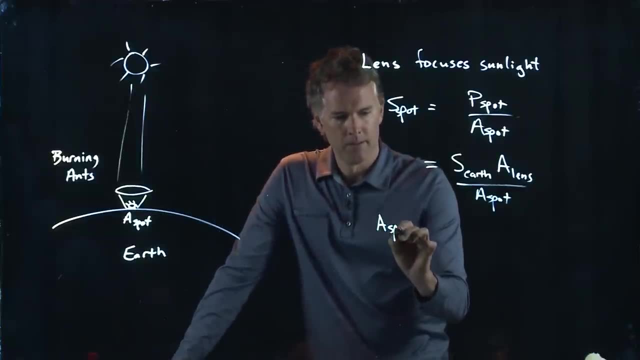 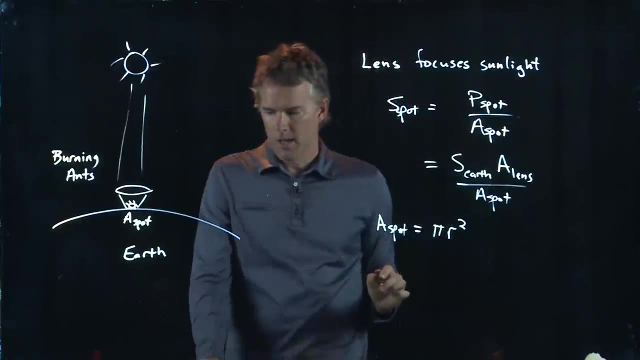 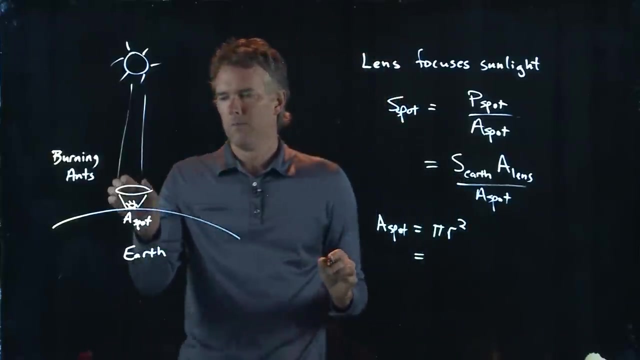 And then we have to divide by the area of the spot. So how big is your spot? Well, it's a circular lens, and so it's just pi? r squared. Okay, and let's say that the spot is pretty small. 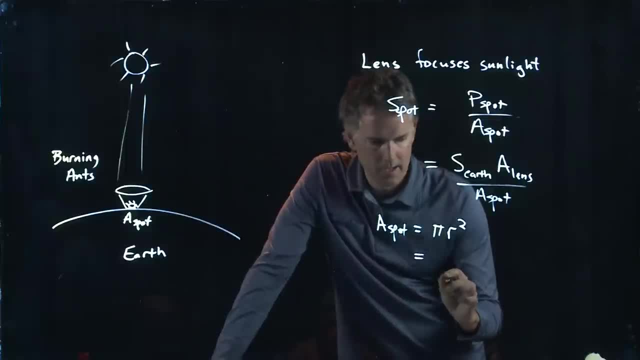 Let's say that it has a diameter of about a millimeter. Okay, so we'll let r be something like a half a millimeter. And then we need to know the area of the lens and that's the pi r of the lens squared. 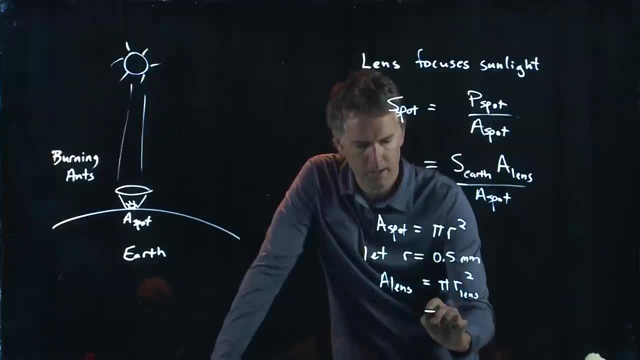 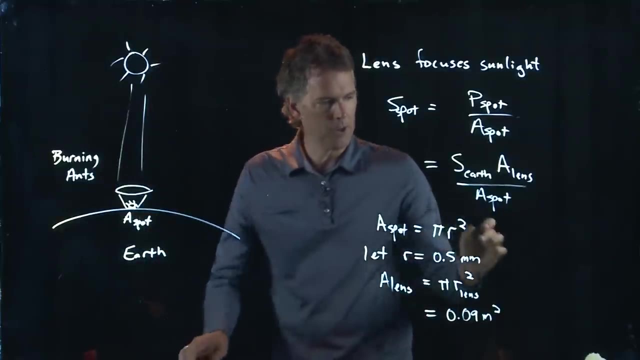 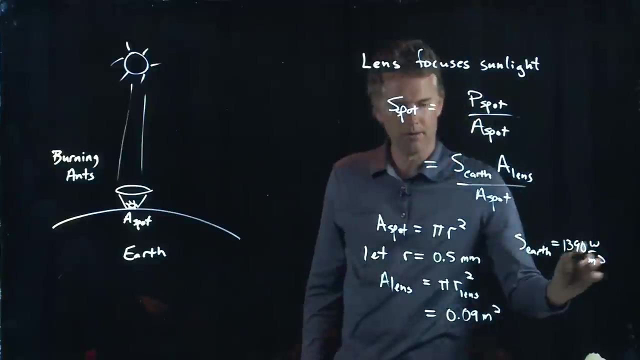 And that can be pretty big, And let's say that the area ends up about 0.09.. Okay So it's a square meters. Okay so it's a lens, maybe that big We already know S at the earth. That was our 1390 watts per square meter. 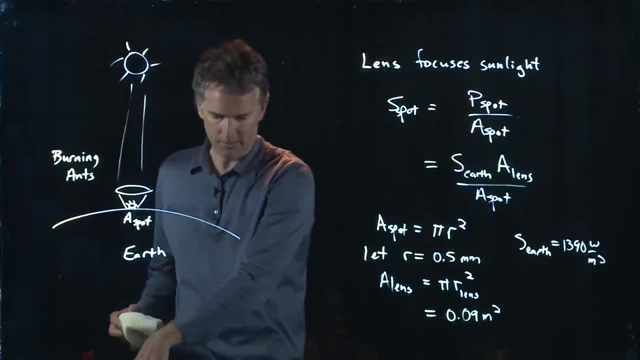 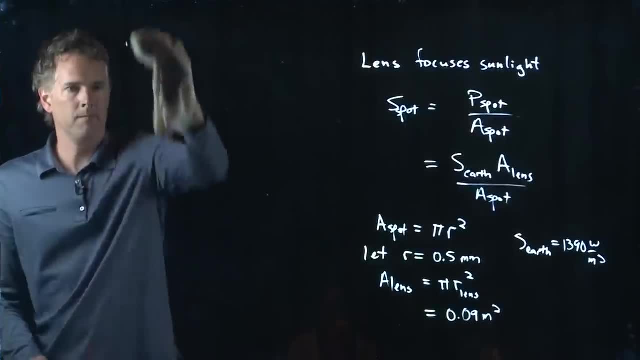 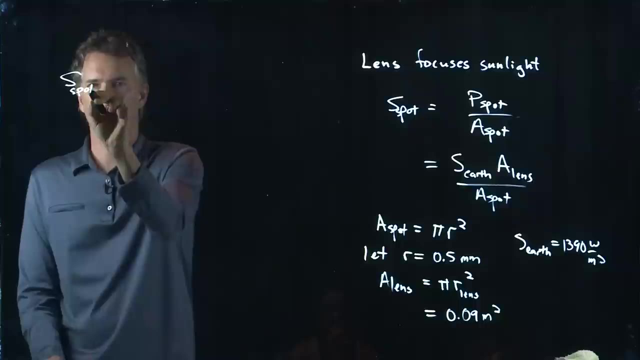 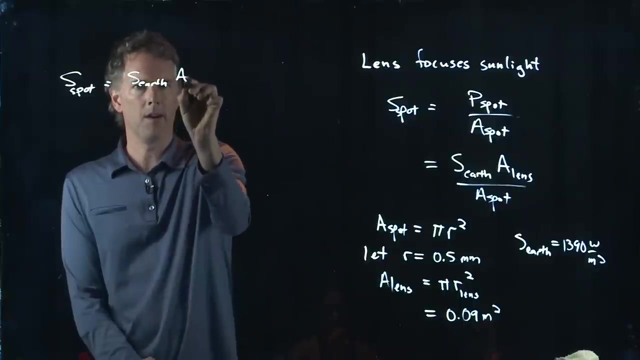 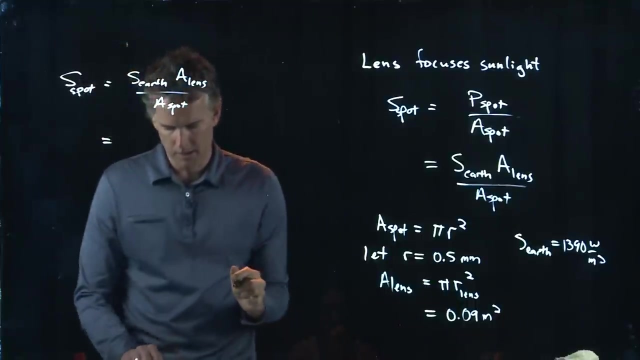 And so now we can put all this stuff together and calculate the intensity at that spot. Okay, So the intensity at the spot is going to be S at the earth area of that lens divided by the area of the spot And S at the earth we said was 1390. 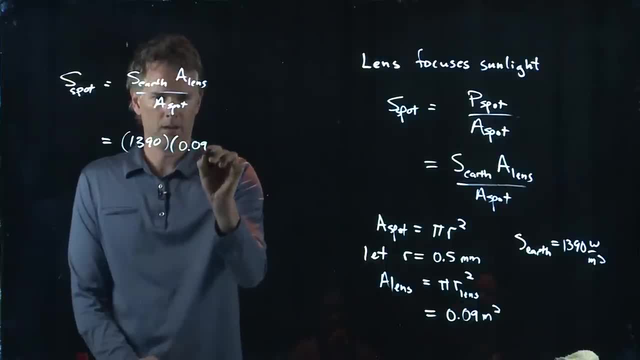 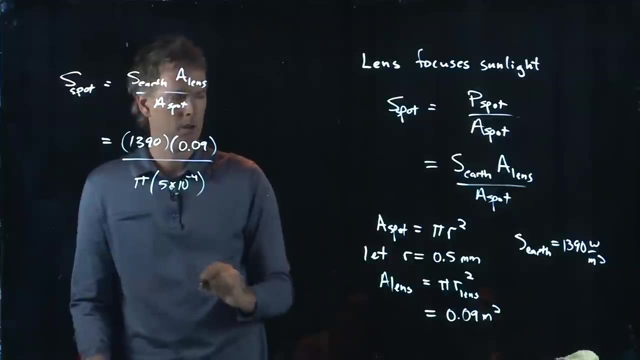 Area of our lens we said was 0.09.. We're all in SI units here. We need a pi r squared for this guy. So we have pi times a half. a millimeter is 5 times 10 to the minus 4 meters. 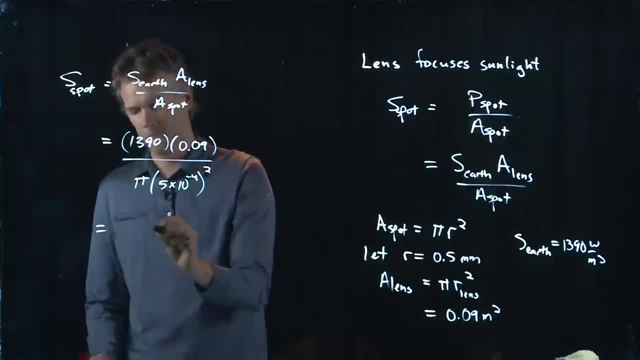 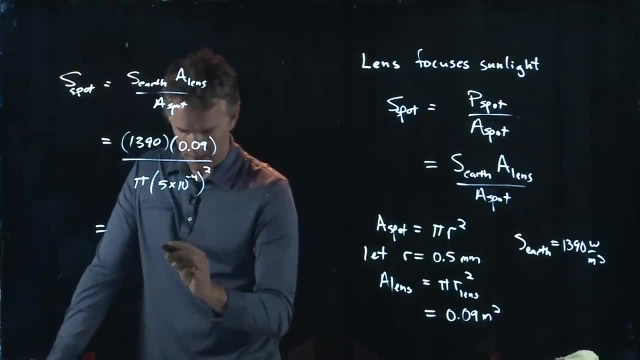 And we got to square that thing. Okay. So if you punch in all those numbers, tell me what you get. When I did it earlier, I got 1.6 times 10 to the 8. Times 10 to the 8 watts per square meter. 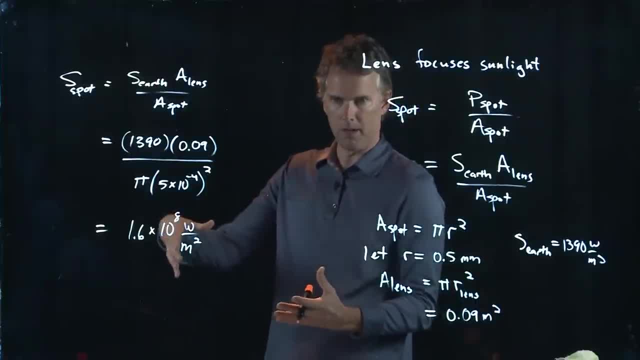 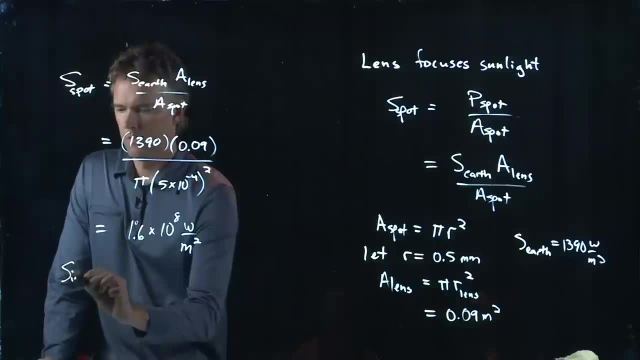 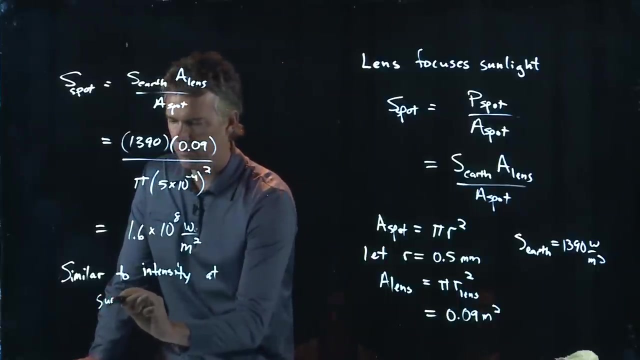 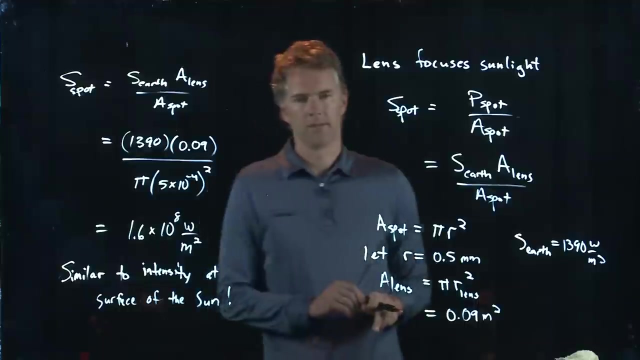 Okay, And this is with a lens about: yay big, Anybody else get that number. How intense is this? It's similar, In fact a little bit bigger. It's comparable to the intensity at the surface of the sun. Okay. 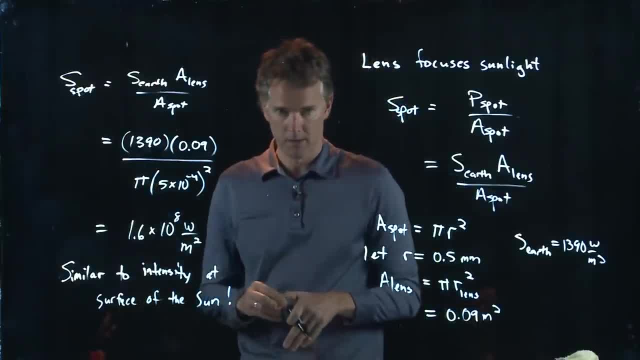 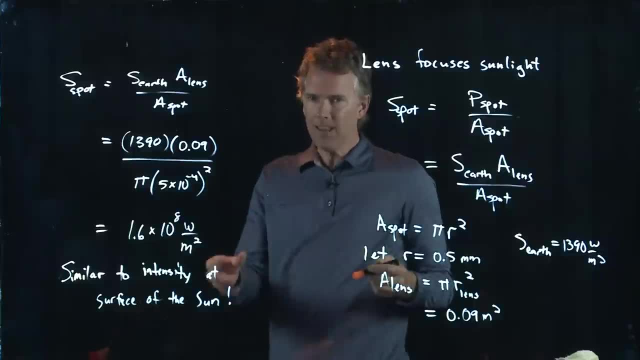 Remember, at the surface of the sun we got something like 6 times 10 to the 7. And now we've got something 10 to the 8. So it's extremely comparable, In fact a little bit bigger than the intensity of the surface at the sun. 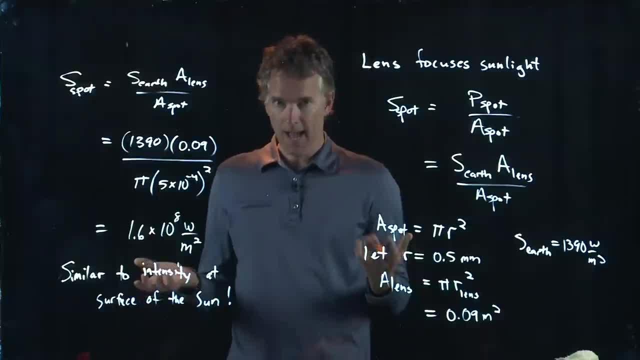 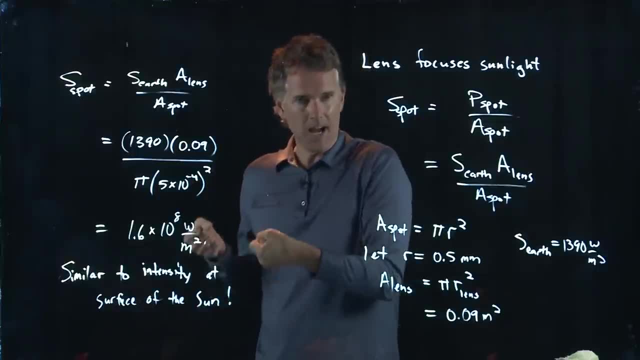 So it's no wonder that ant burns up Right. In fact, if you do this experiment yourself, if you go out with a big lens like that big and you go outside on a hot, clear day- it's got to be a nice clear day- 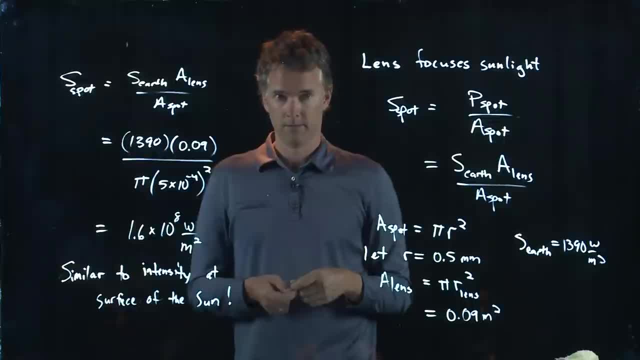 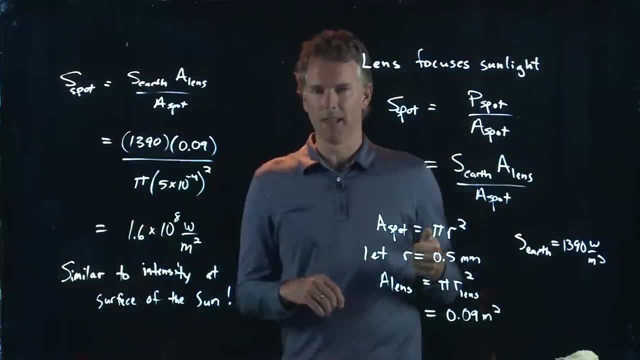 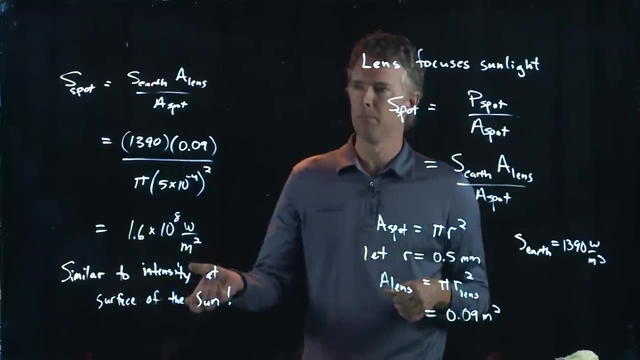 you can burn holes in concrete. Okay, You can burn holes right into the concrete itself. Really fun. I got a big lens in my lab. We'll try it on one of these really hot days. You got to be a little careful, obviously, because you know it's an intense spot and you can burn it yourself. 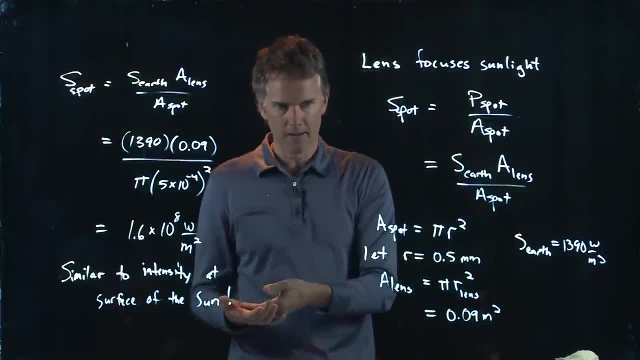 But also you can't really look at the spot because it's sort of like looking at a welder's arc. It's just so intense that you can hurt your eyeballs when you do this experiment, So you definitely got to be a little careful. 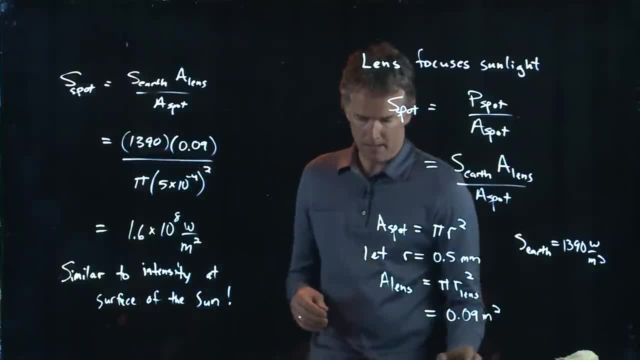 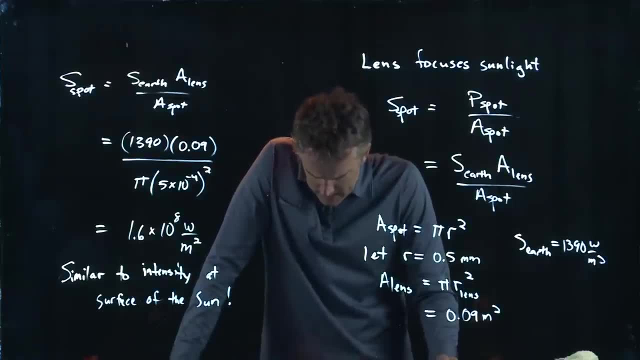 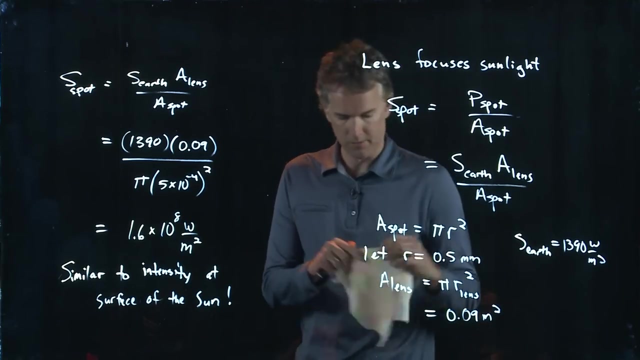 All right, Let's see. Let's try just one more of your homework questions And let's take a look at: Let's see, Let's take a look at the misconceptual question 22.07,, which is number two on your homework. 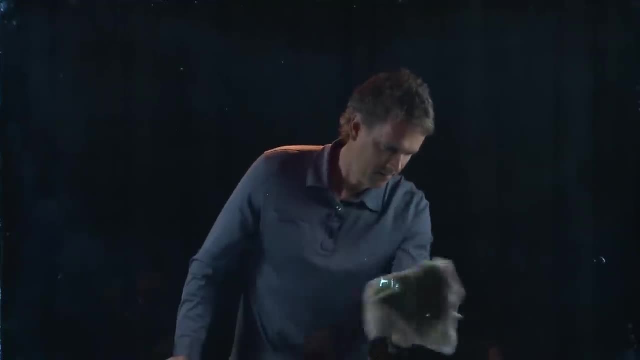 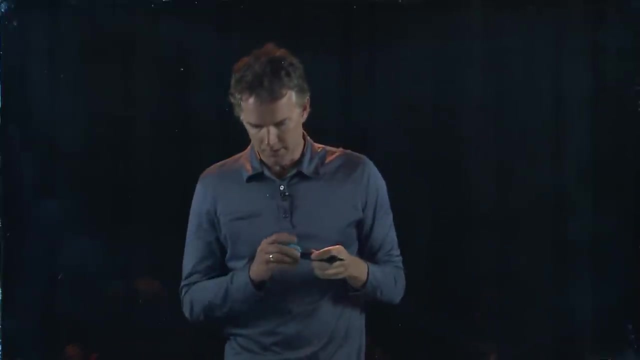 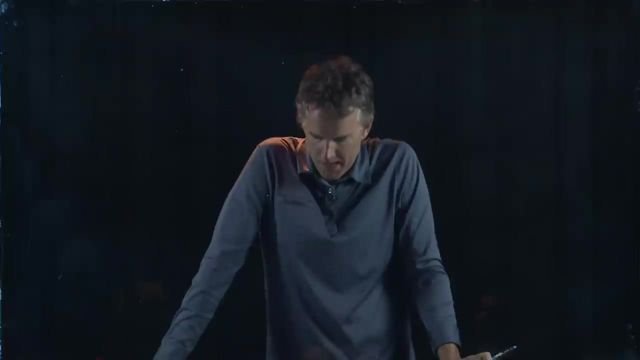 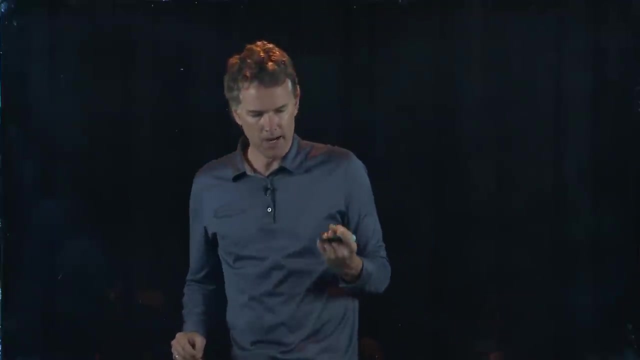 Okay, So this is misconceptual question 22.07.. And it says: if the Earth-Sun distance were doubled, the intensity of the radiation from the Sun that reaches the Earth's surface would do what? And your options are: drop to a quarter, quadruple, drop to a half or double. 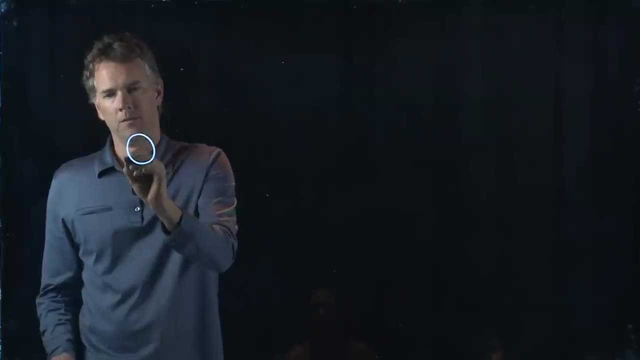 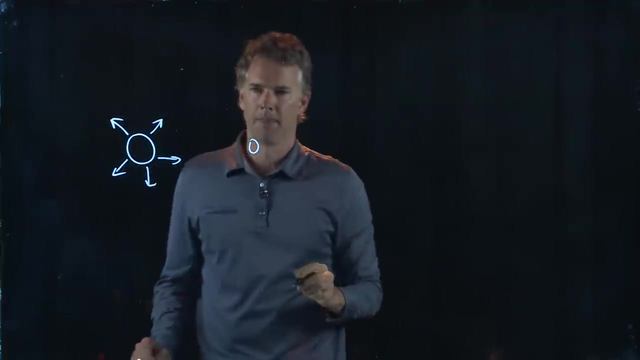 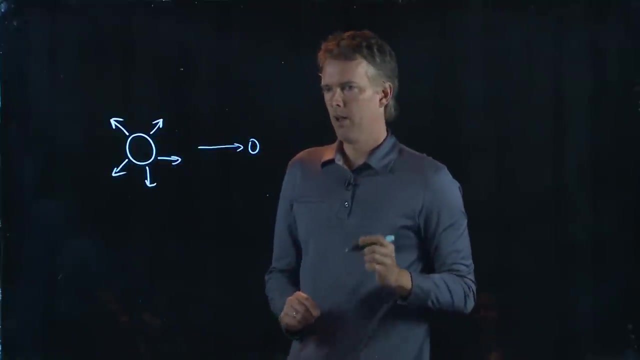 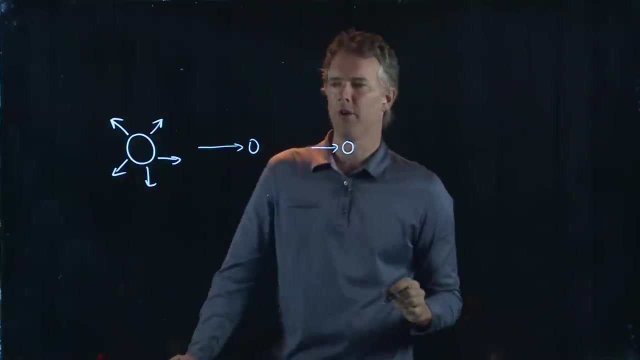 So let's go back to our picture. Here's our Sun, Here's the Earth. Okay, Some of that sunlight is getting us here on the Earth, But now we're going to take that Earth and move it out to a distance twice as far away. 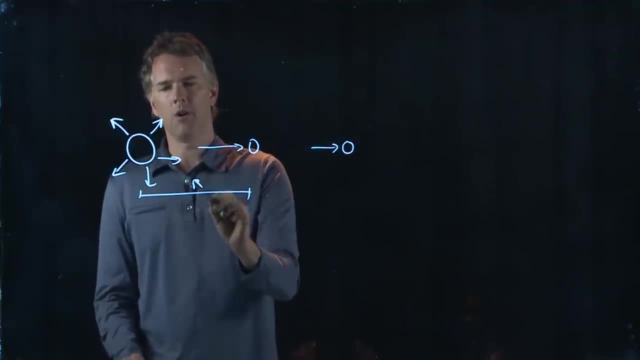 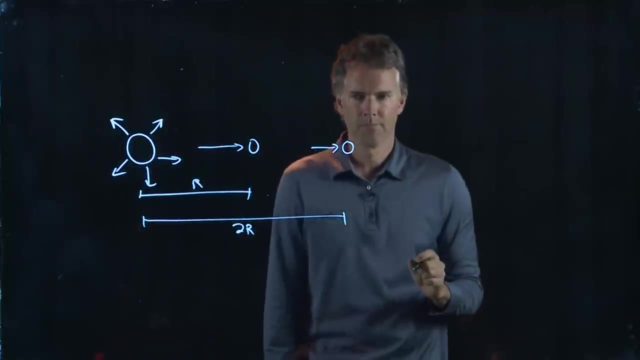 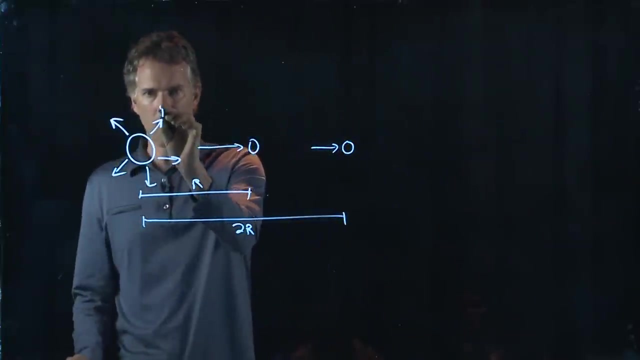 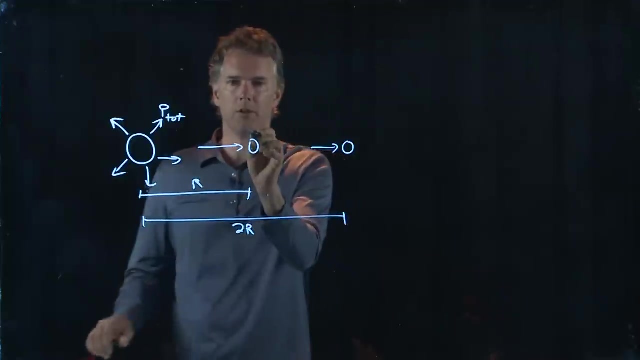 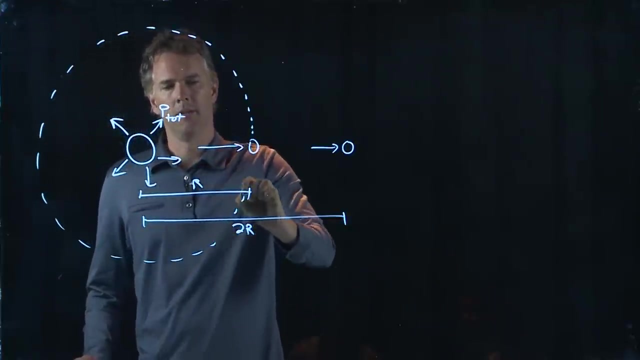 So if this was R, now we are two R away. So how do we think about this? Well, there is a finite amount of power that's leaving the Sun. All of that power is going to be intercepted by this sphere of radius R. 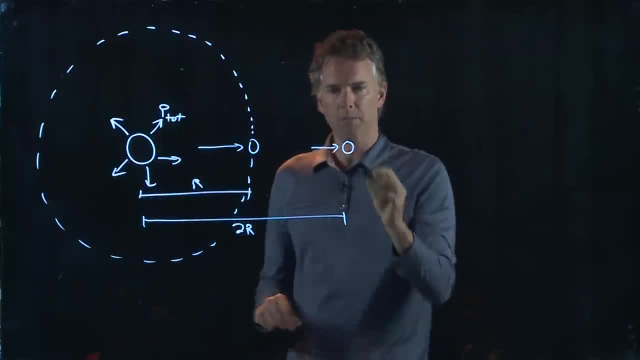 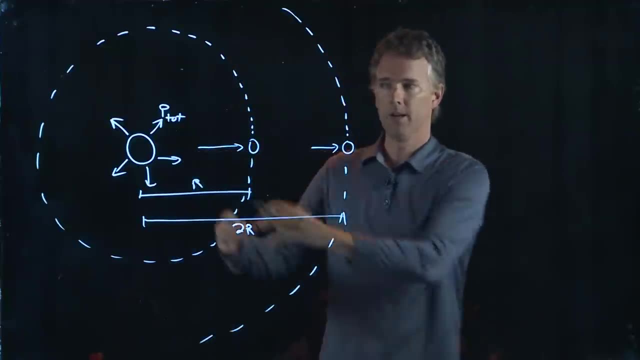 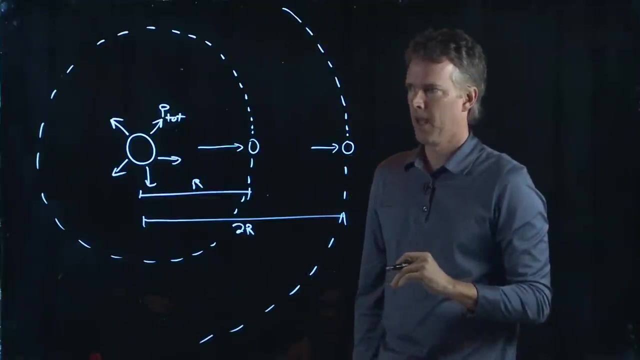 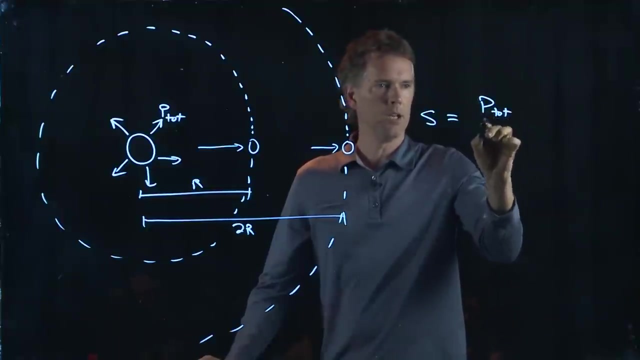 But all of that power is also going to be intercepted by this sphere of radius 2R Right. All that light that's coming out of the Sun eventually is going to go through this bigger sphere, And so the intensity at any location is just P total divided by area. 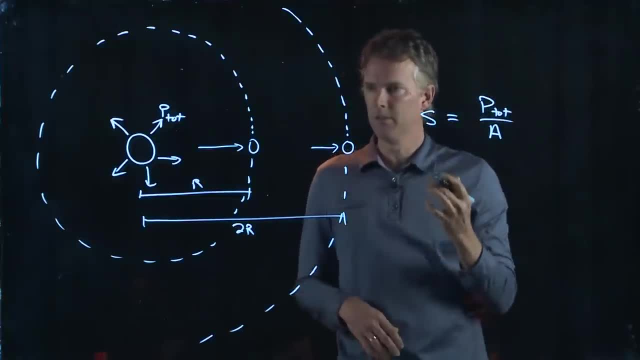 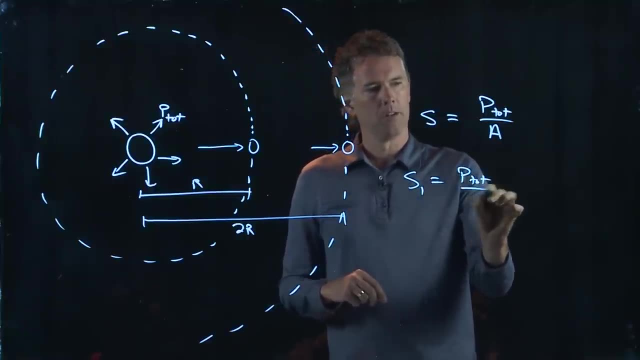 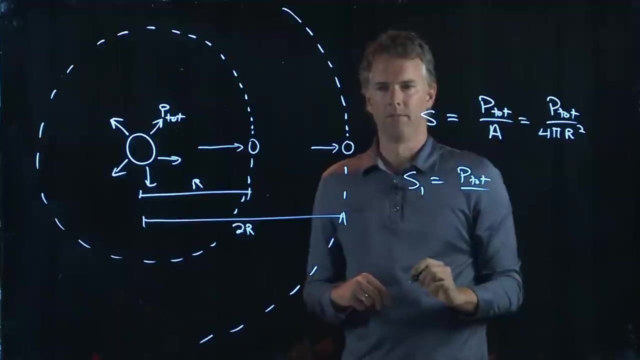 where it's the area of these spheres. So for the first case we've got P total divided by what is area. Area of a sphere is 4 pi R squared. So in the first case it's just 4 pi R squared. 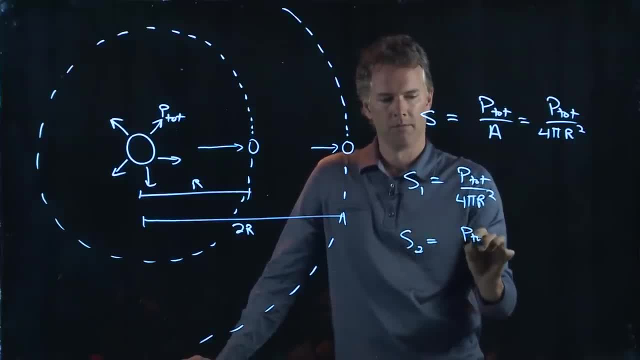 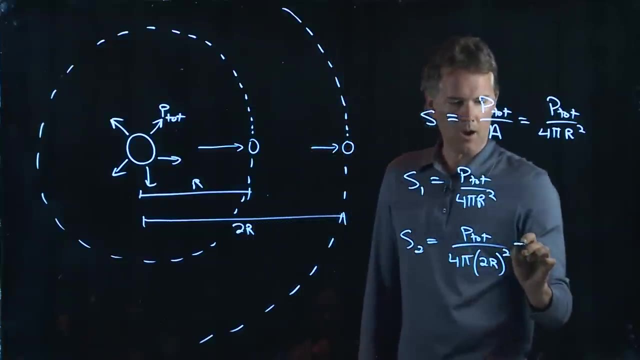 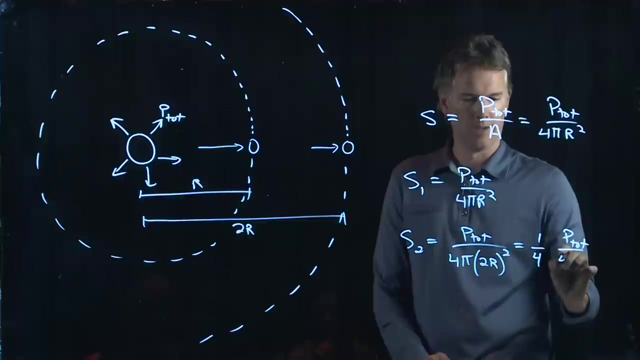 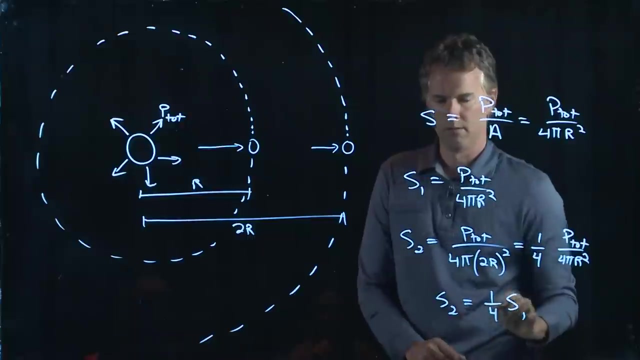 But in the second case the power doesn't change. But what does change is this: radius down here becomes 2R, quantity squared, And now I have a 1 over 2 squared, and that's the same as 1 over 4 of what we had before. 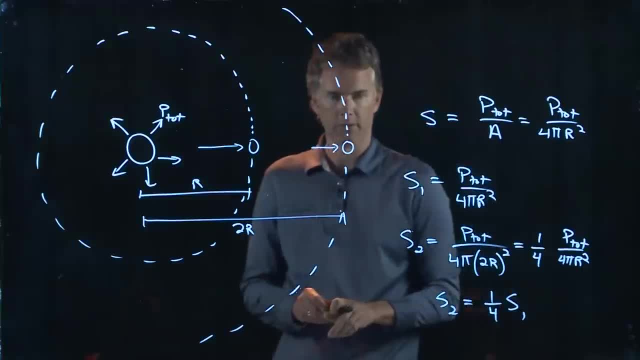 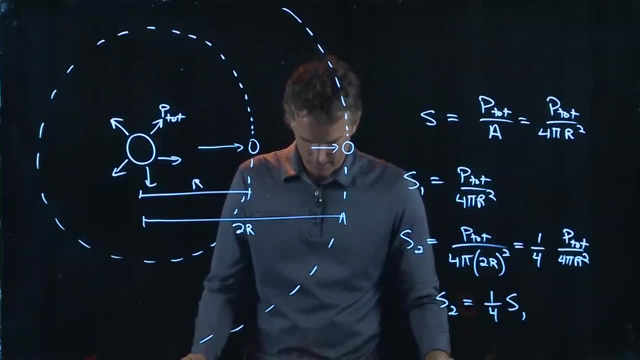 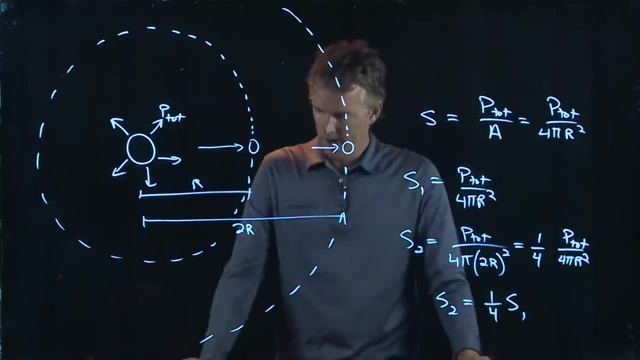 So S2 is a quarter of S1.. Double the distance It goes down by a factor of 4.. So let's try that one and click it in And it says: we're right, All right, Everybody feeling okay, Or at least completely overwhelmed. 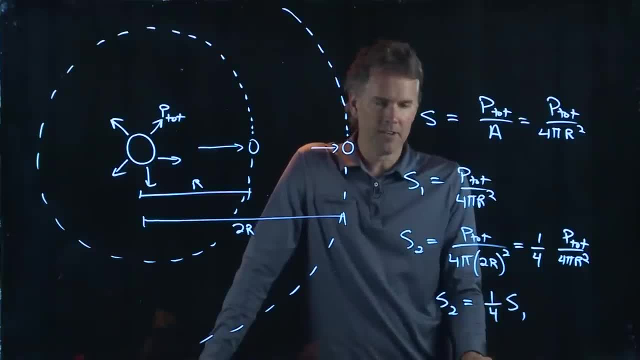 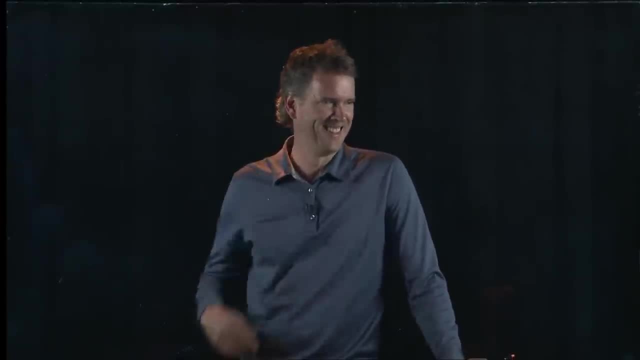 Okay, That's good. All right, Let's get out of here. I'll see you guys tomorrow. Cheers Hi class, Hi Hi class. How's everybody doing? Good, Good, We're going to continue talking about electromagnetic waves. 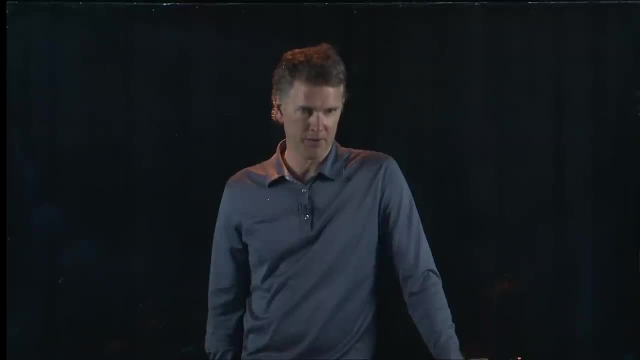 Did you guys get a chance to watch the videos from yesterday that introduced electromagnetic waves? Yes, Yeah, Even if you didn't just nod appreciatively. Yes, we did. Thank you very much, So let's continue that discussion. I thought maybe what we'd do first is take a look. 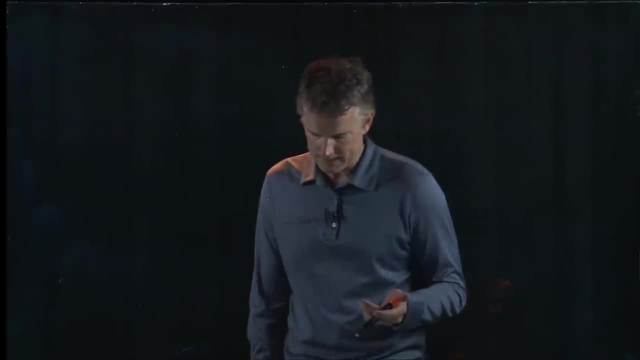 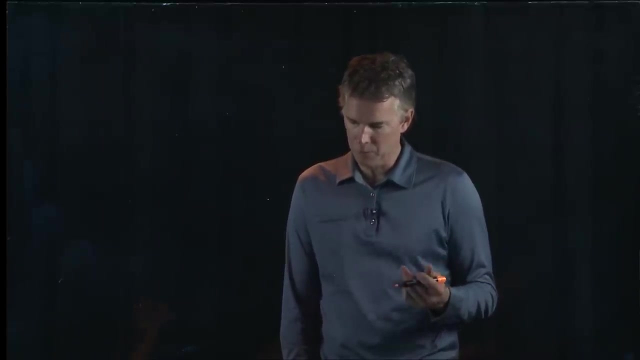 at one of the homework problems for Chapter 22,, which is one of the misconception questions, And it says the following. It says an electromagnetic wave is traveling straight down toward the center of the earth. At a certain moment in time, the electric field points west. 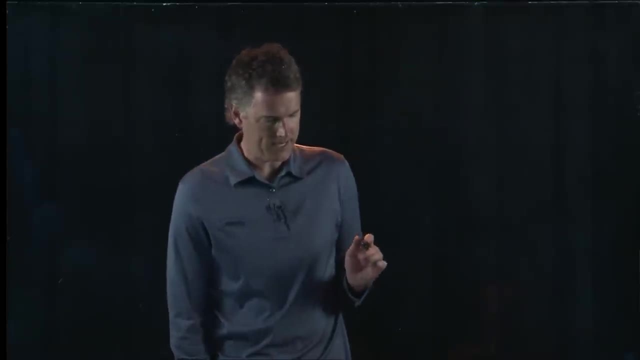 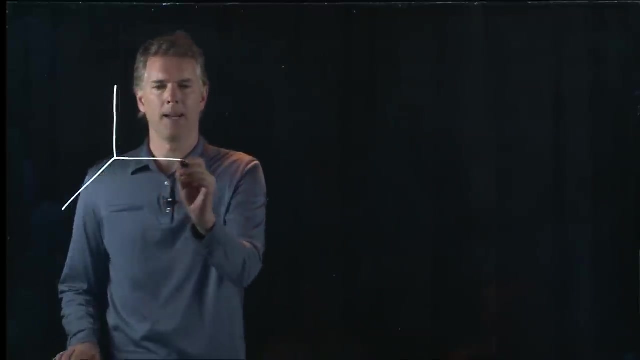 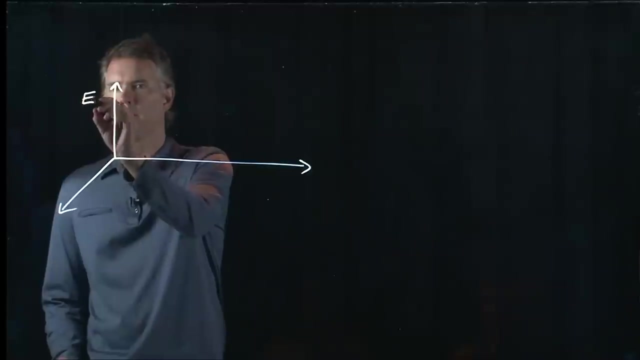 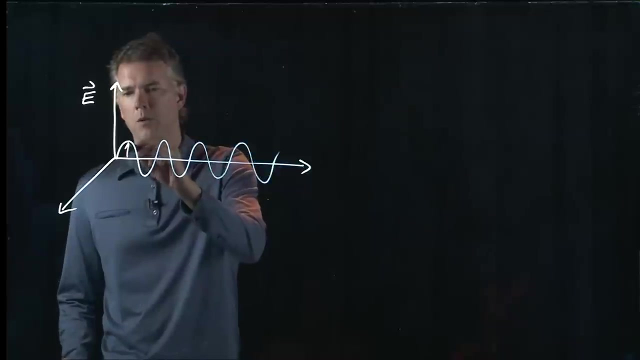 In which direction does the magnetic field point at this moment? So remember yesterday, when we drew electric and magnetic fields that combined to make a wave, we said the following: E let's let that oscillate up and down. Okay, And we know what that means. 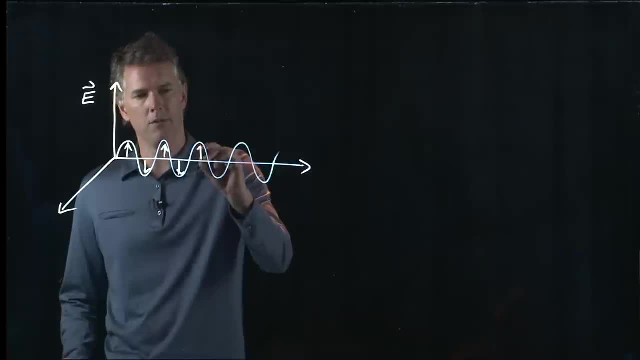 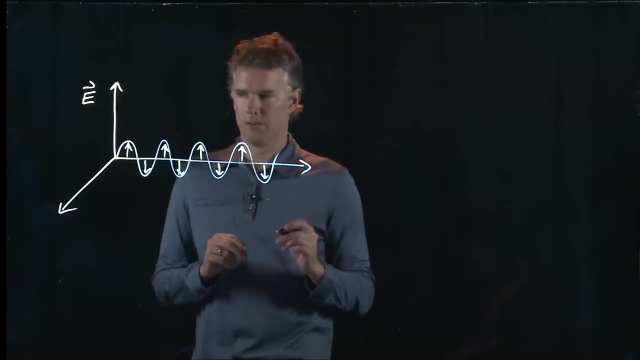 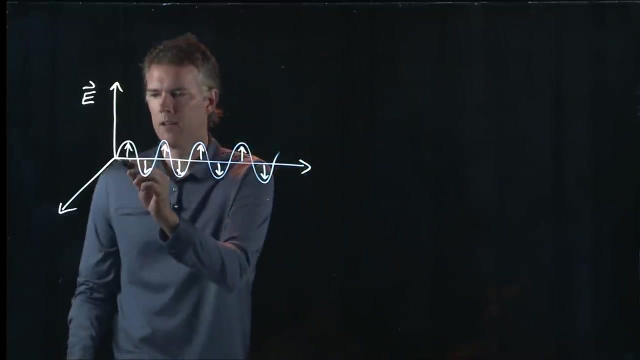 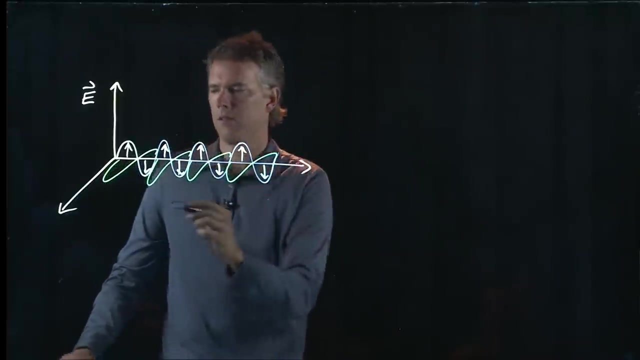 It's going up, then it's going down, up then down, and so forth. But the B field was at a right angle to that. So if we draw the B field, let's try it in green. The B field in fact comes into and out of the page. 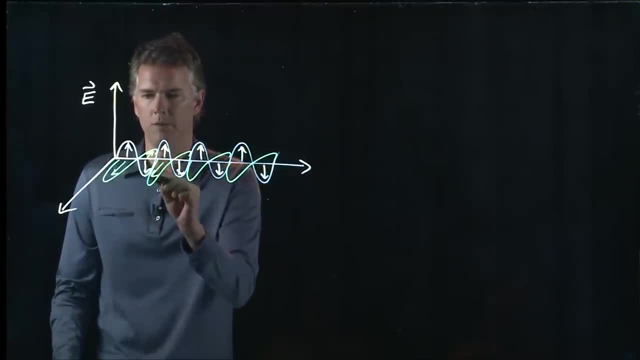 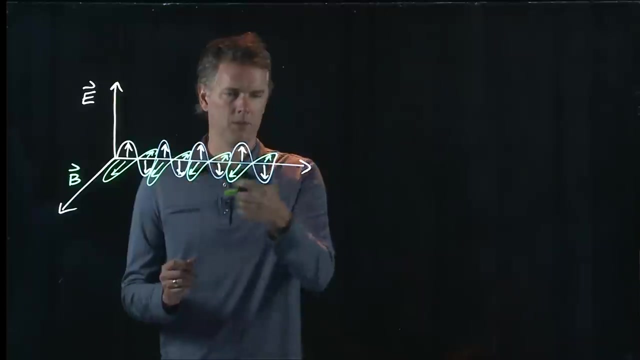 And so it's pointing out of the page and into the page over and over again. Both of these things are, of course, oscillating sinusoidally, And so this would be the direction of B. Now the whole wave propagates to the right. 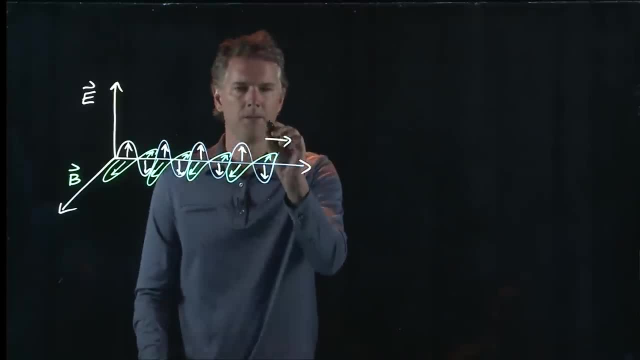 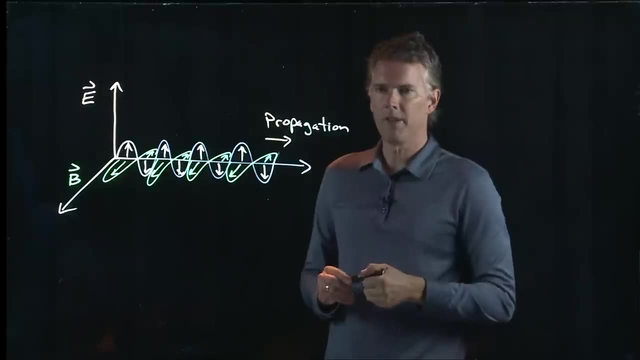 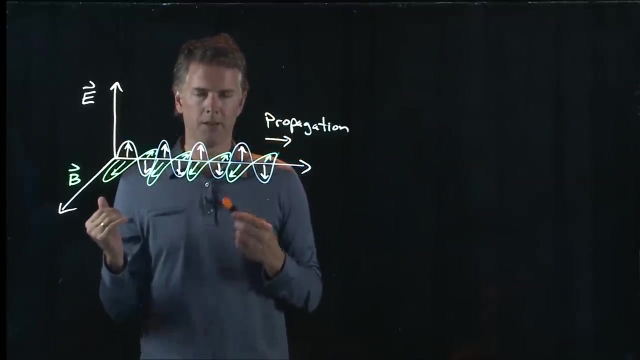 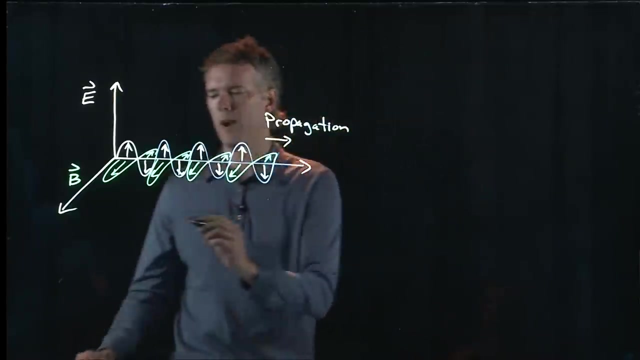 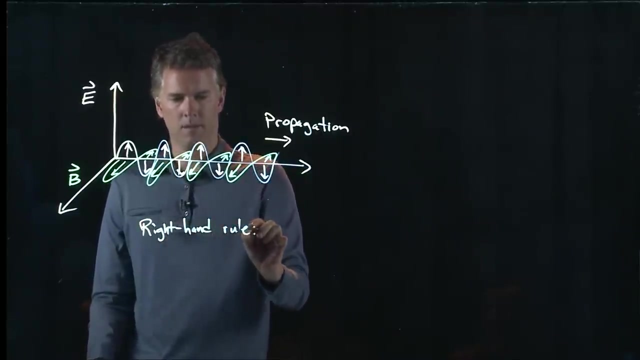 So the wave propagation direction is to the right, But there is a certain relationship between the E field and the B field. Okay, And to figure out how to calculate the propagation direction, we can again go back to our right-hand rule. Okay. 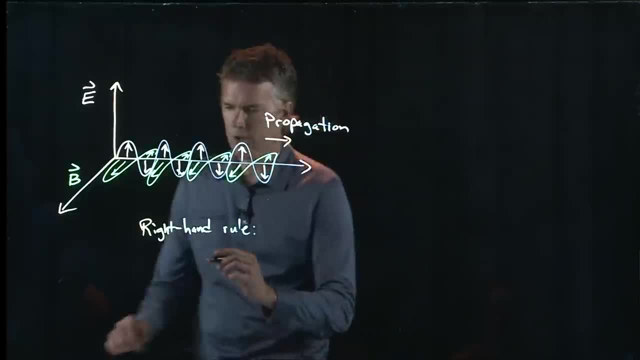 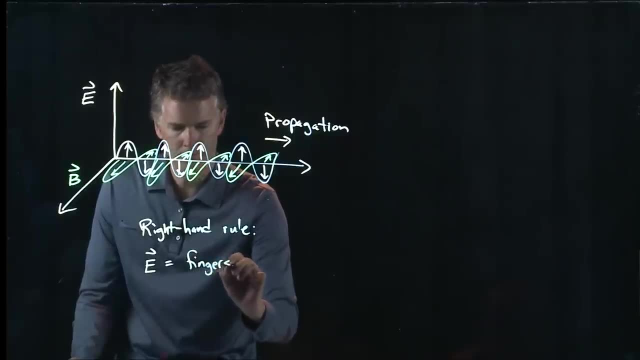 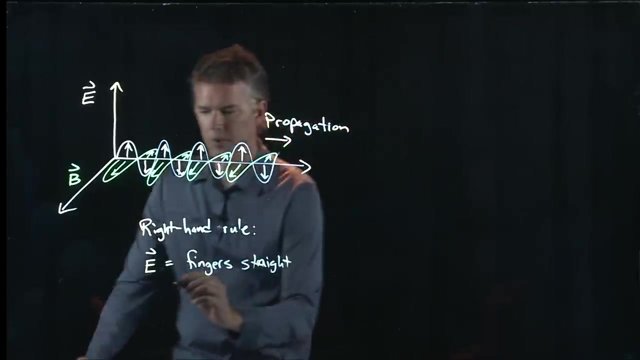 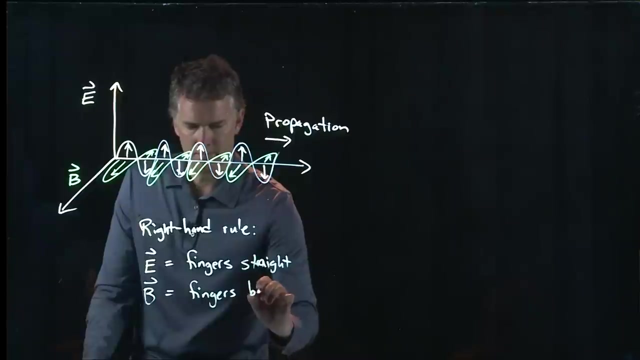 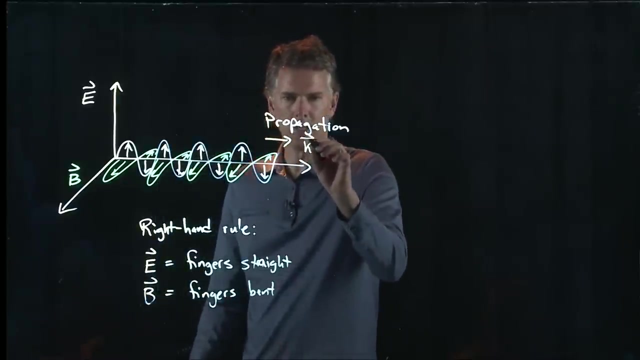 So the right-hand rule is the following: You put your fingers straight in the direction of E, You bend your fingers in the direction of B And then the propagation direction, which later on we're going to learn- is actually given with a, K. 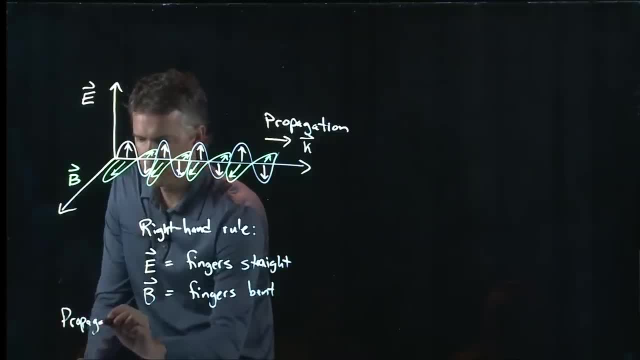 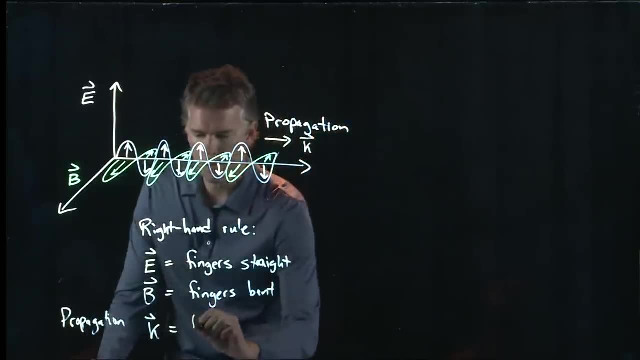 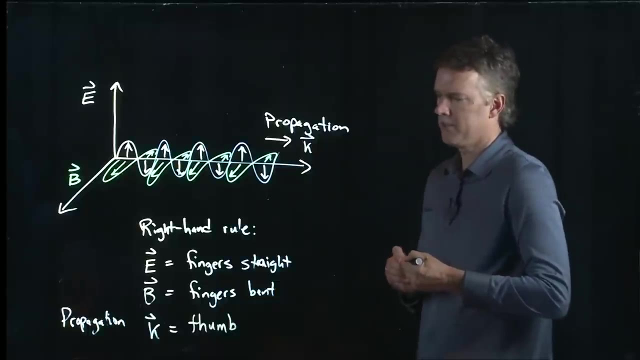 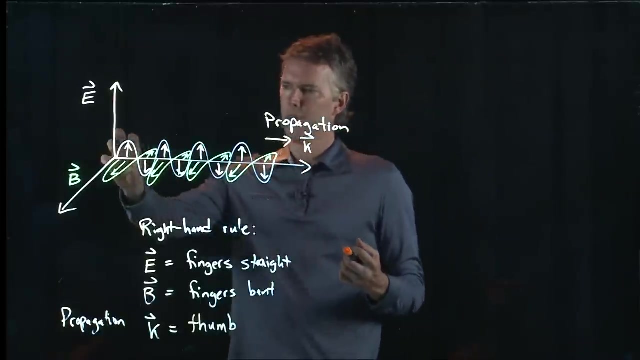 Propagation K is in fact the direction of your thumb. Okay, So let's try that with this picture and see if we can convince ourselves that it is true. And let's look at the first instant of time In the first section of this wave. 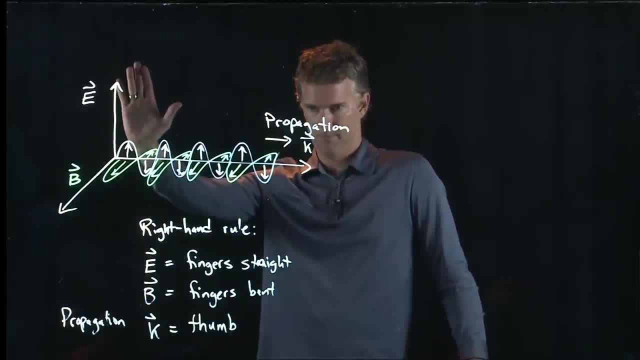 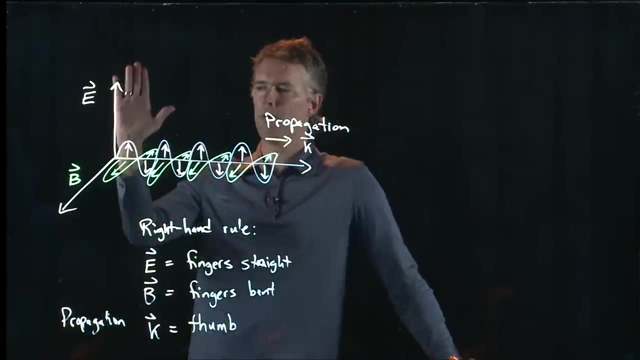 I have an E field that is pointing up, I have a B field that is coming out of the page And therefore my thumb gets me the direction of K. So everybody, look at the computer monitor, Hold up your right hand. Okay, And try that. 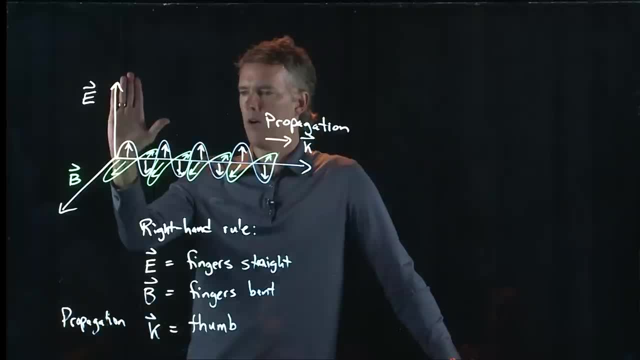 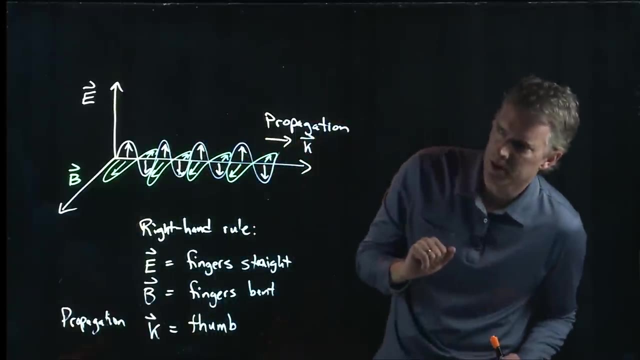 Put your fingers straight up in the direction of E And now bend your fingers in the direction of B. Your thumb should be pointing in the direction of K. Is that what everybody is seeing? No, Okay, We could have it flipped. Let me see if I can see what's going on. 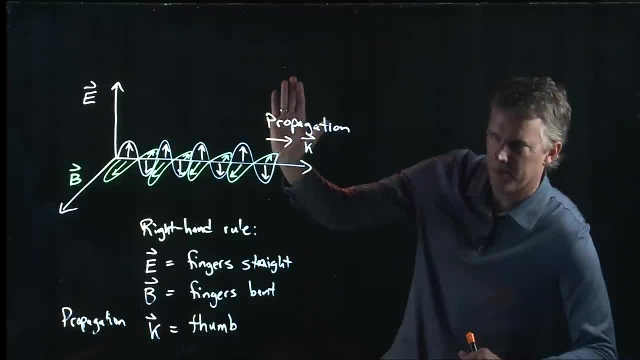 in the computer monitor. So we've got E going up And then B is coming out towards you guys. Is that right? Okay, And so you should get a thumb that's going to your right if you look in the computer monitor. Yeah, don't look at this. 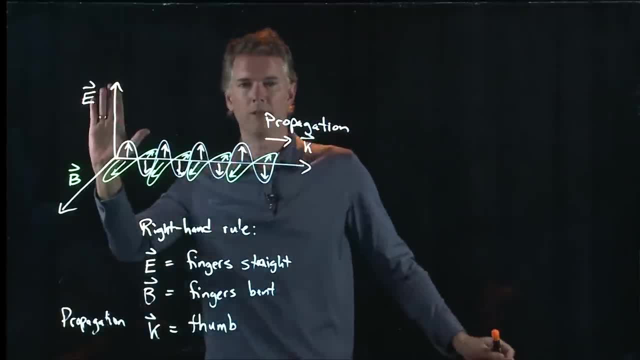 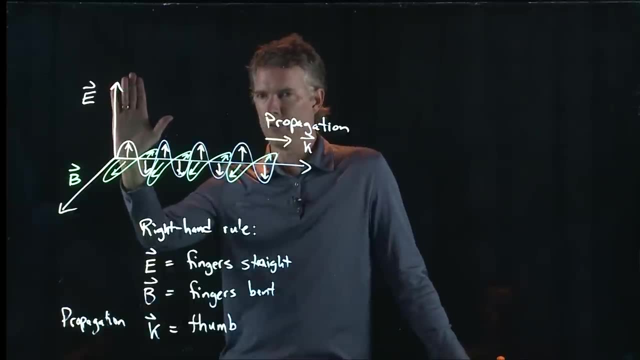 This is confusing, right? Look at that. Is that working over there? Does that look like my right hand in the computer monitor? Looks like my right hand right. My fingers are in the direction of E. yes, Now I'm in the direction of B. 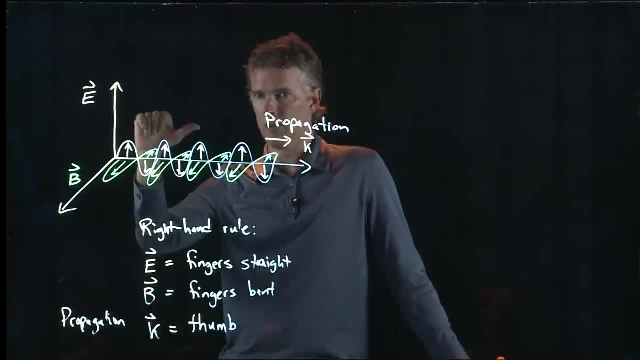 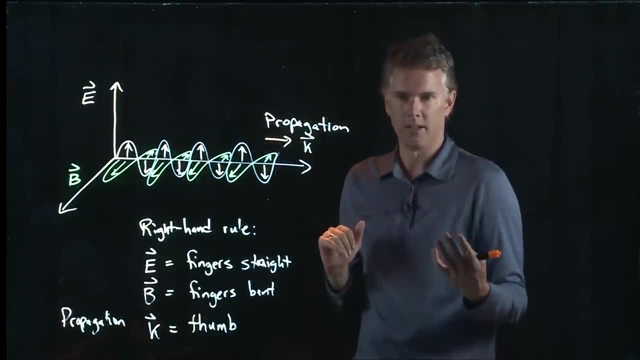 because it's coming out towards you, And now my thumb is going in the direction of K. Is that working? Yeah, It gets confusing when you're looking over here at the glass, because it's inverted on the screen and so we have to do a little clever trick there. 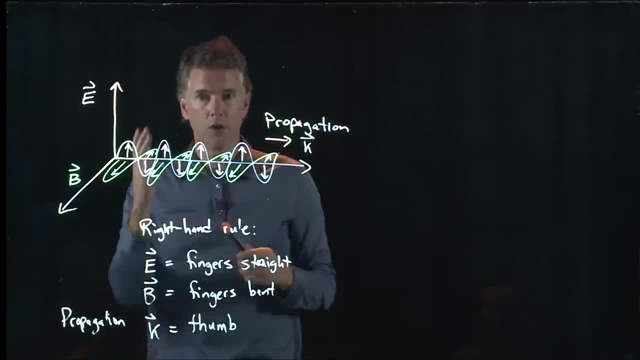 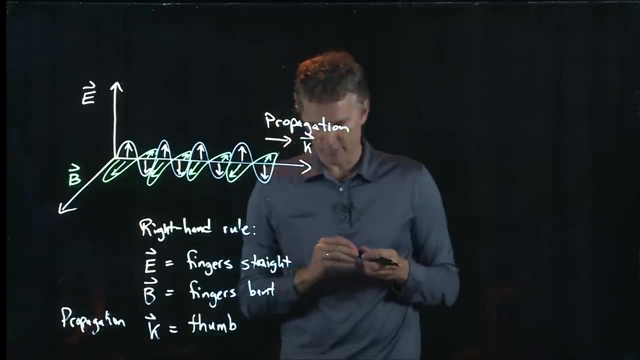 So the relationship between E and B. those two angles determine the direction of K. E is always orthogonal to B And if you use your right hand rule, it will tell you the direction of K. So let's go back to the question that they had for a second. 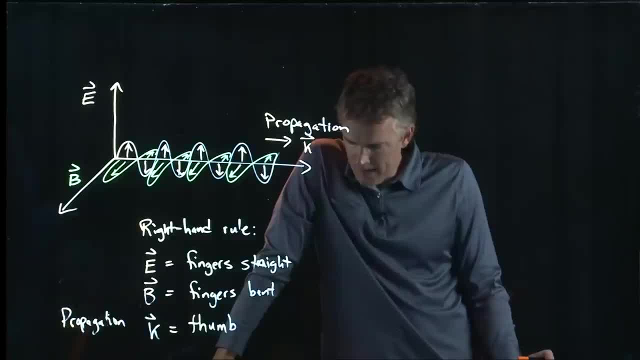 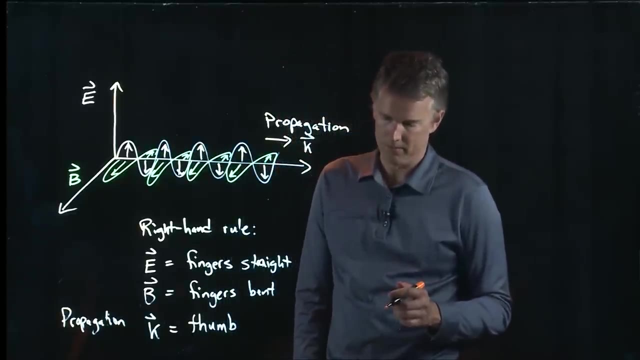 They said that an electromagnetic wave is traveling straight down towards the center of the Earth. At a certain moment in time, the electric field points west. Okay, In which direction does the magnetic field point at this moment? All right, Well, let's see if we can draw this picture. 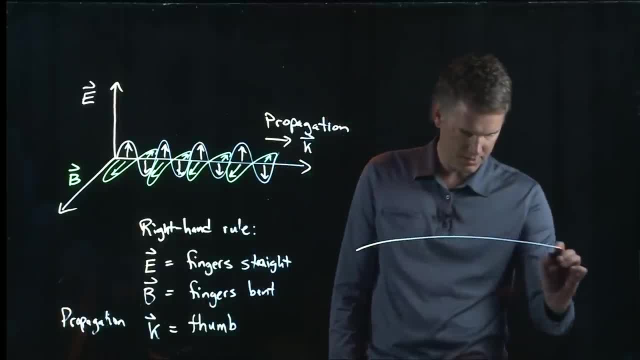 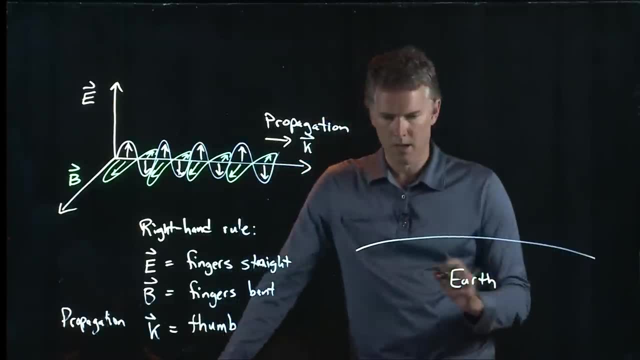 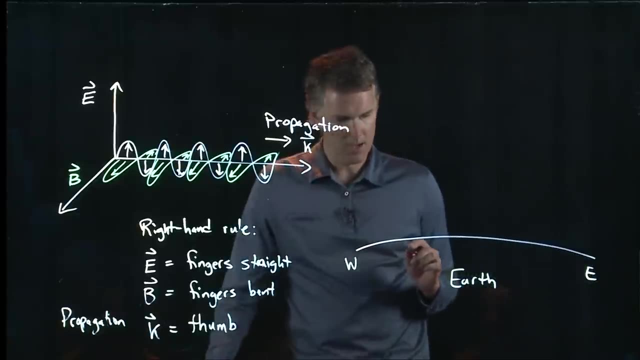 And it might be kind of tricky. It might be tricky to draw, but let's give it a shot. This is the Earth, Okay, And we're going to say that the west is to the left, The east is to the right. 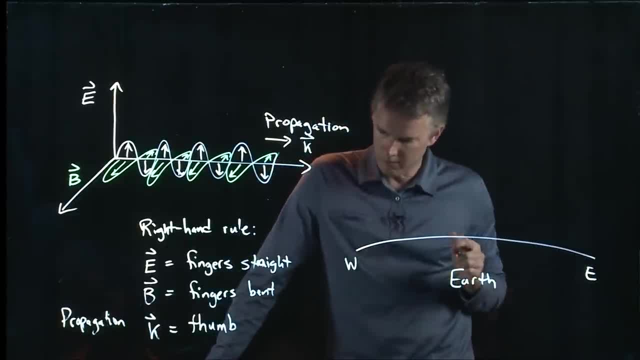 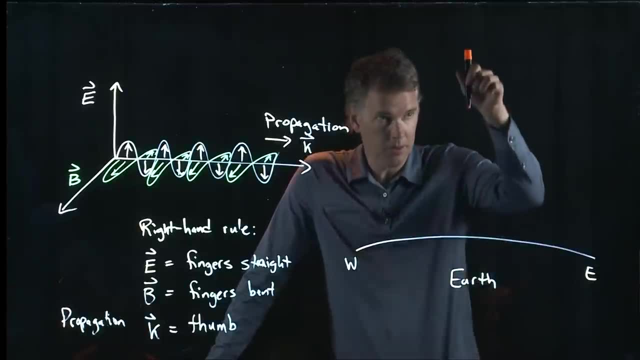 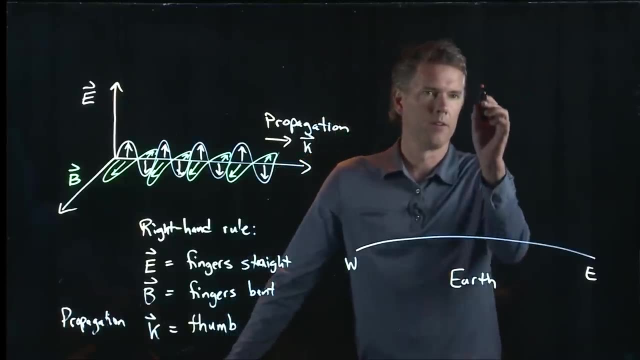 Okay, That means the north would be into the screen, The south would be out of the screen, And so if the wave is propagating down towards the center of the Earth, it's going to be coming down this way, And at a certain moment in time, the electric field points west. 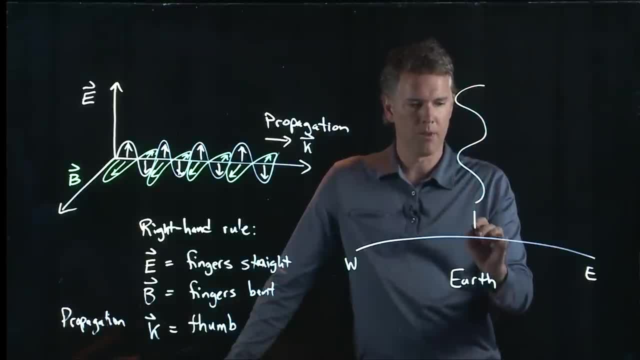 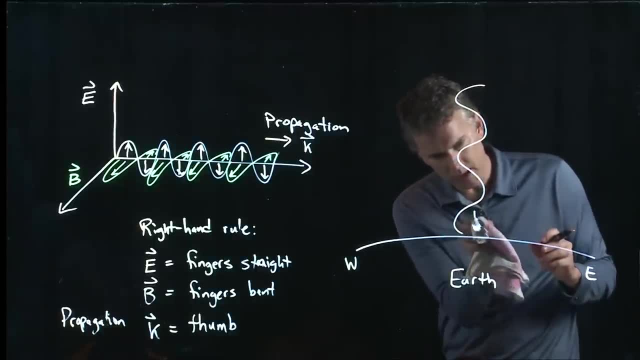 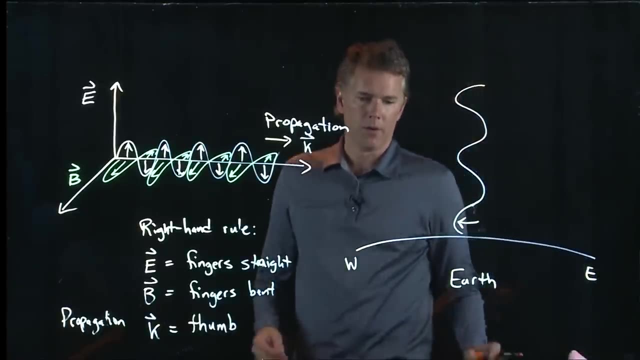 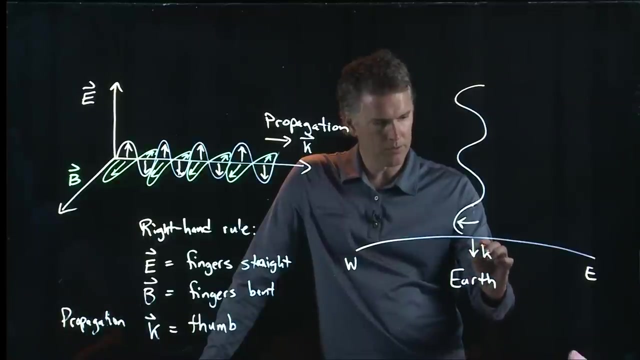 Okay, So here comes our wave. It is propagating this way And at this moment in time the electric field is pointing to the west. So there is our electric field. So if the electric field is pointing west and the wave is propagating towards the center of the Earth, 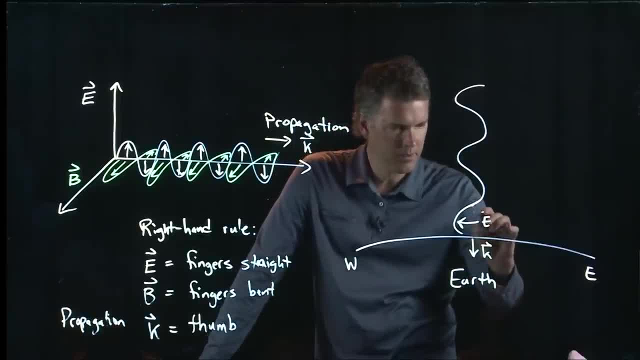 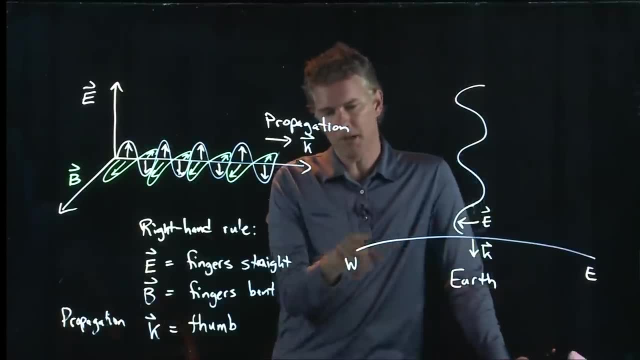 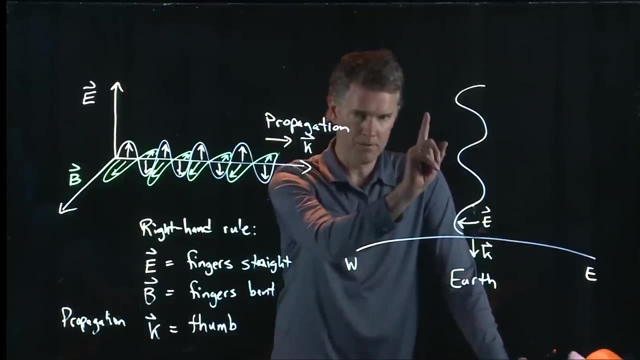 this is our E field. we know that the B field has to be at a right angle to the E field. Okay, So it can't be west and it can't be east. We also know that it can't be up and it can't be down. 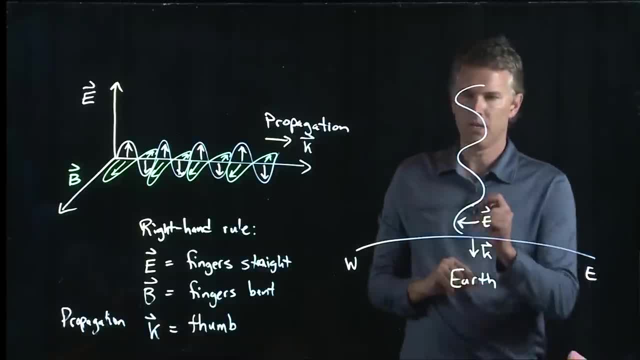 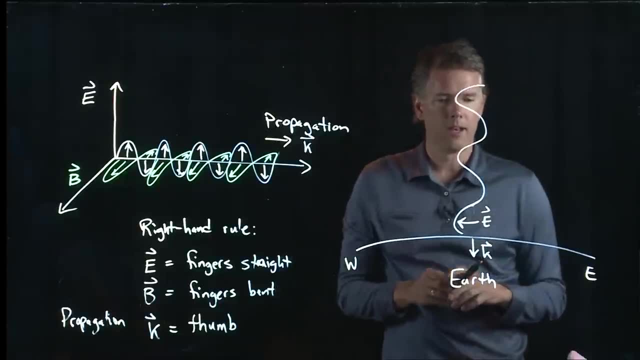 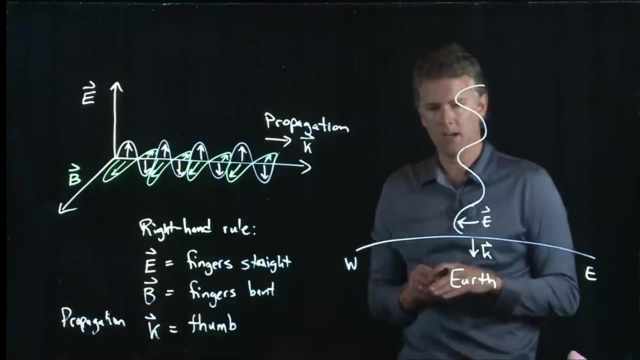 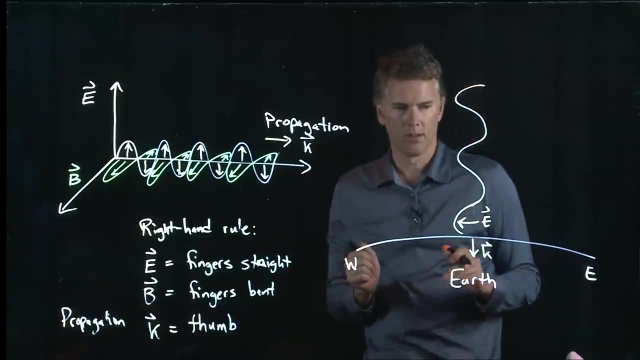 So the only option is into the screen or out of the screen. It's either north or south, And if north is into the screen, let's see what we would get. We would get E, cross B would get me a K. that is pointing. 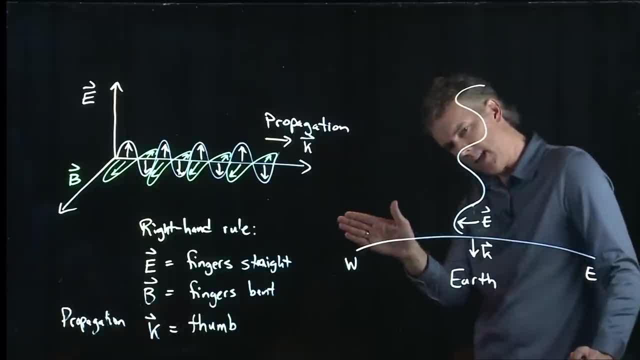 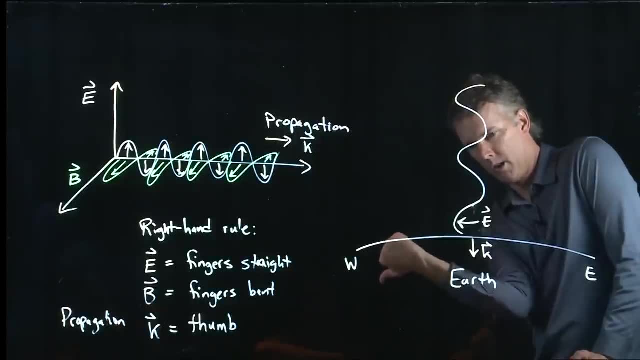 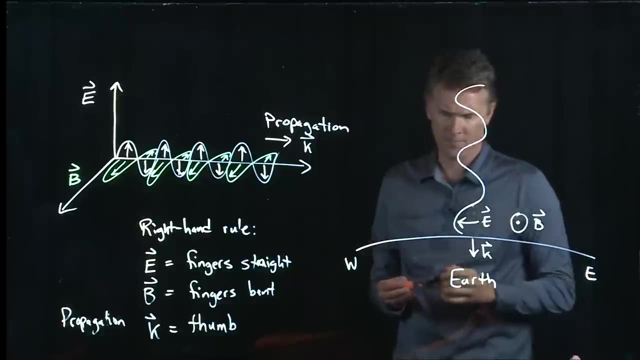 Well, let's see if we do this right. We've got an E And then if B was coming in, it would give me a K, like that. So it looks like we do want a B field. We've got a B field that is doing that. 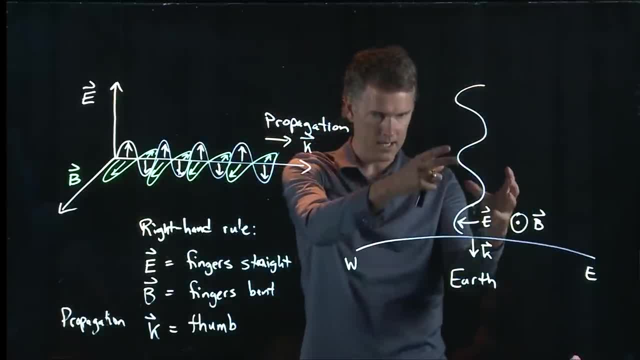 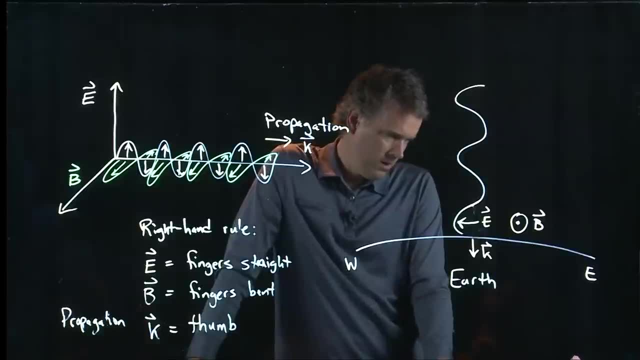 Okay, We've taken this picture and we've rotated it to this where the B is going into and out of the board. So I would say I would say that we need, is that right? Hmm, I think that's the wrong way. 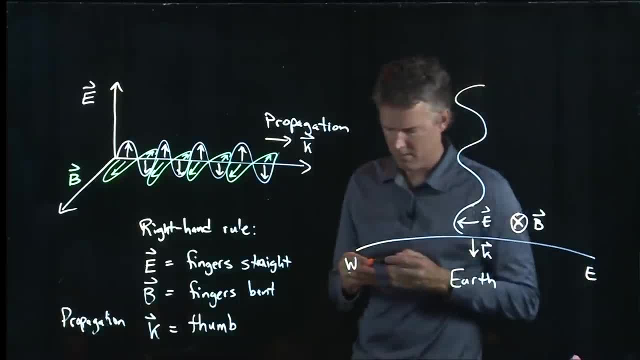 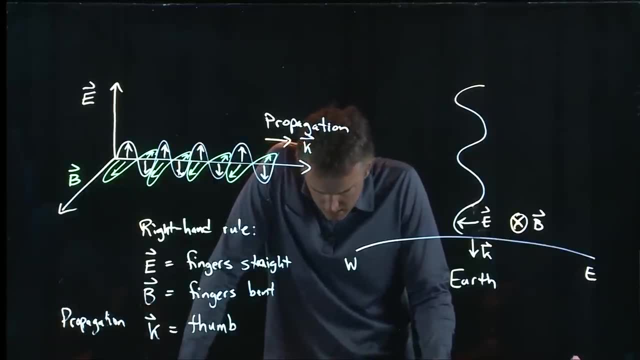 I think it's got to be this way. But you know what? Let's try it. So E going west means that the B field I'm going to say should be north. Let's just try it and see if we're right. 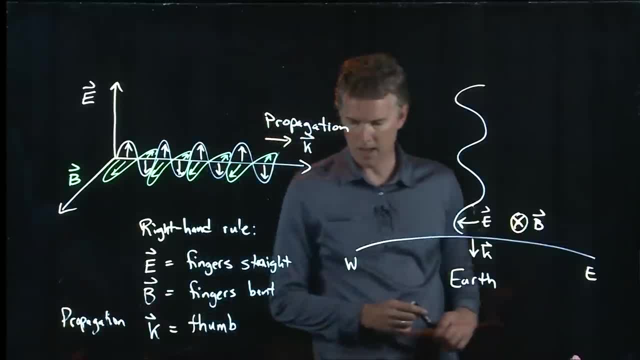 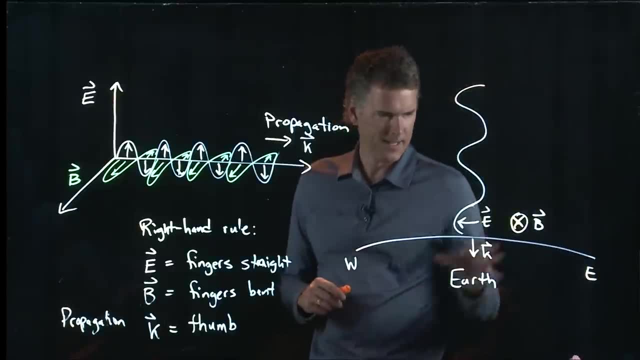 And if we're wrong, it's probably the opposite which is south, And it says we are correct. Okay, So B field is in fact in the north direction. I might have tweaked this up a little bit, But the important point is we can eliminate west and east up and down. 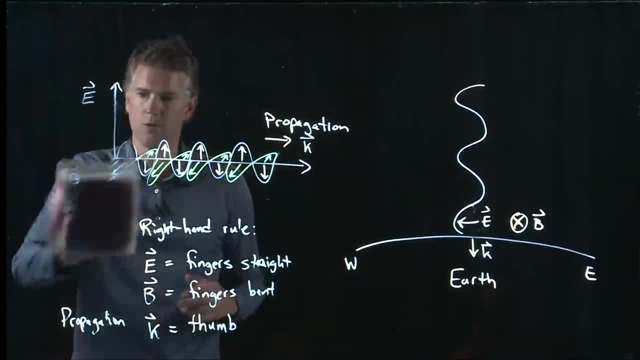 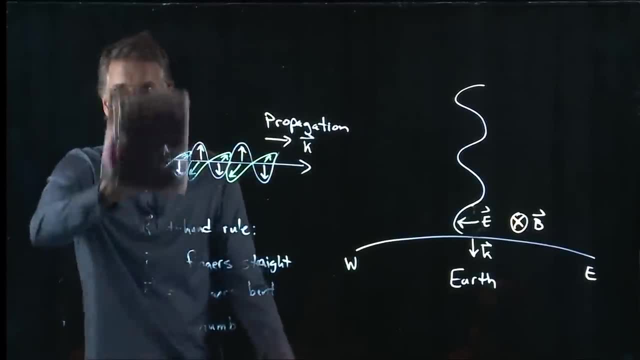 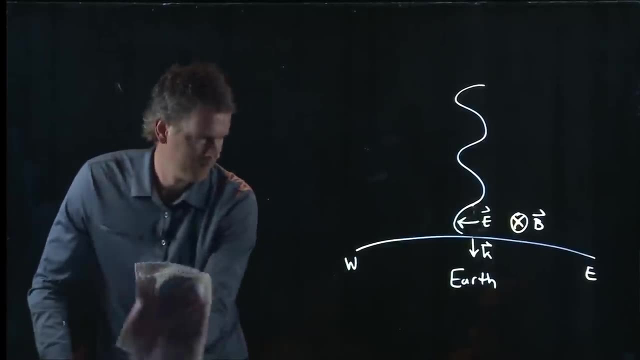 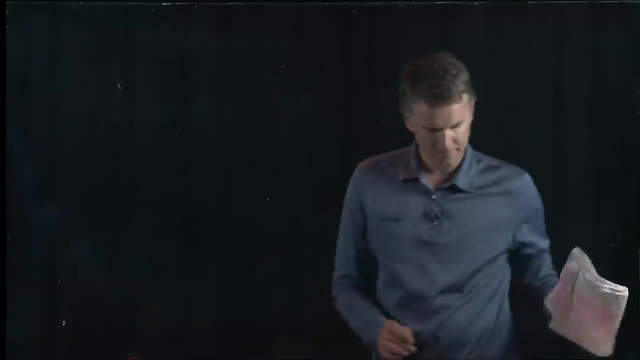 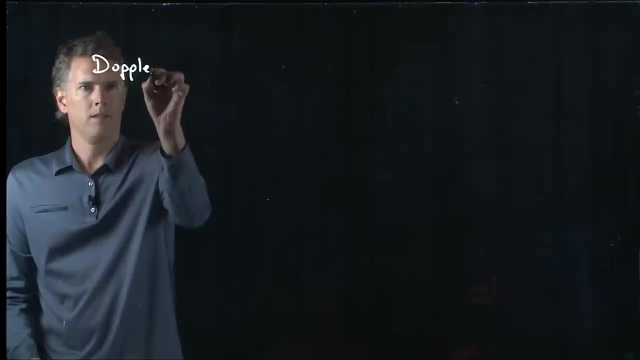 Okay, Let's go back to this idea of waves for a second and talk about something called the Doppler shift, because this is really interesting. So this is something that you guys have heard about, But let's talk a little bit about what's really going on. 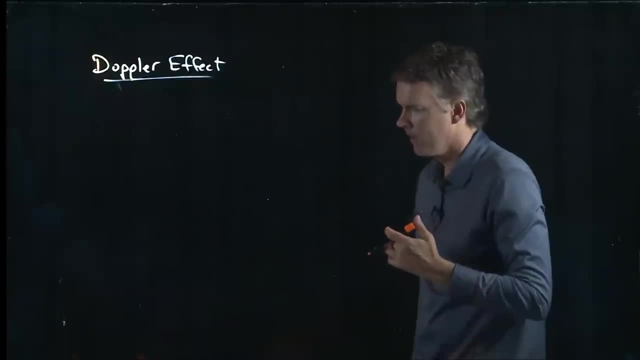 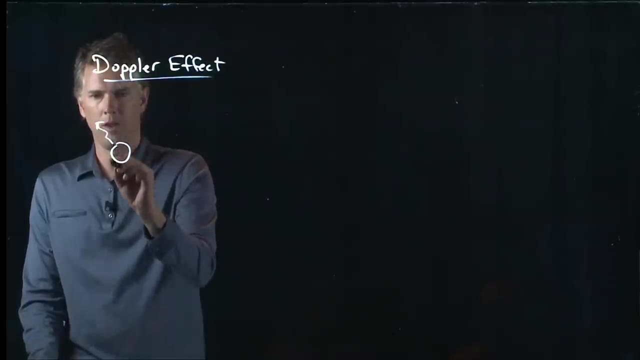 with something called the Doppler effect. Okay, And the Doppler effect is just this. Let's say I'm looking at a star And I know that that star is spitting out light in all directions, And let's say that it is stationary relative to me. 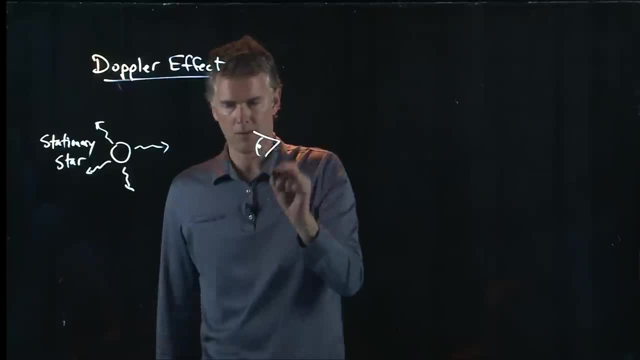 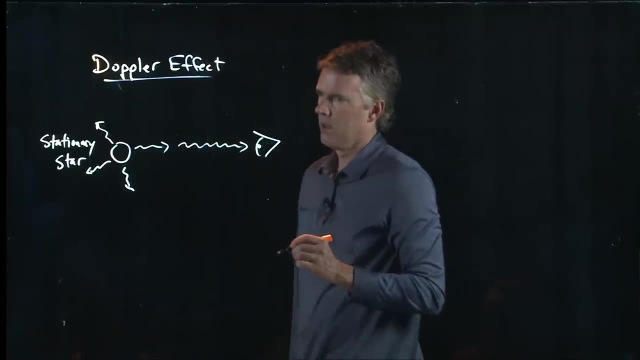 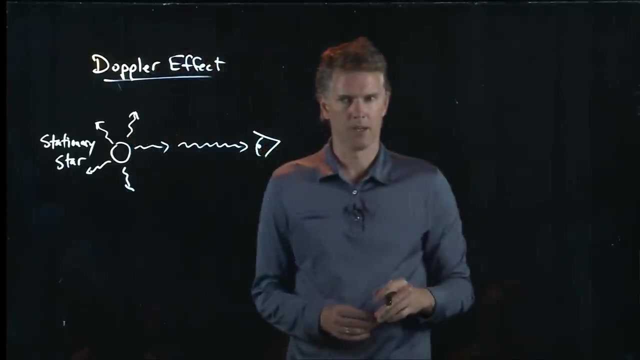 Okay, Here I am on the earth. I'm looking at the star with my eyeball. Some of that light comes all the way and gets to me. What do I observe? I observe some particular color that came out of this star. Okay, 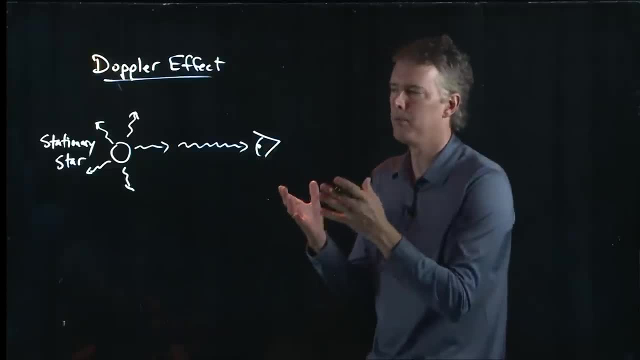 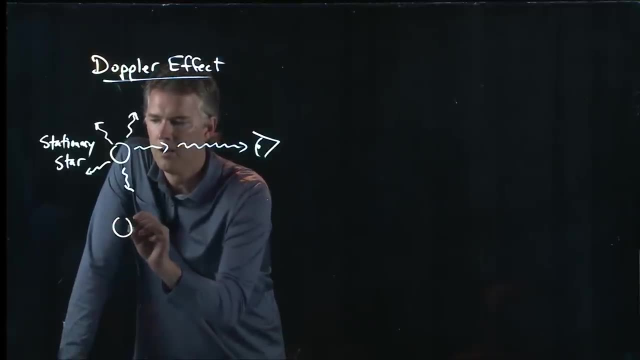 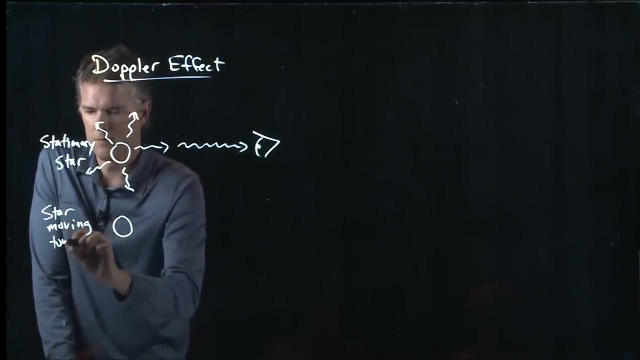 This is usually a whole spectrum of colors, of course, But I observe some particular colors that are coming out of this star. But let's say the following happens. Let's say the star starts moving towards us. Okay, The universe is a big, crazy, violent place. 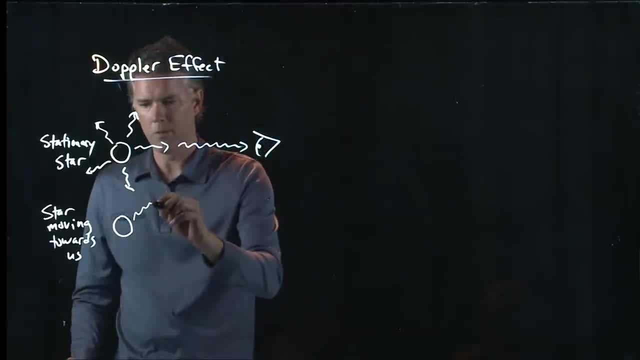 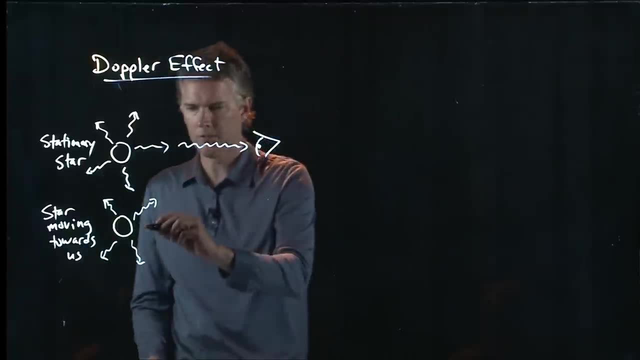 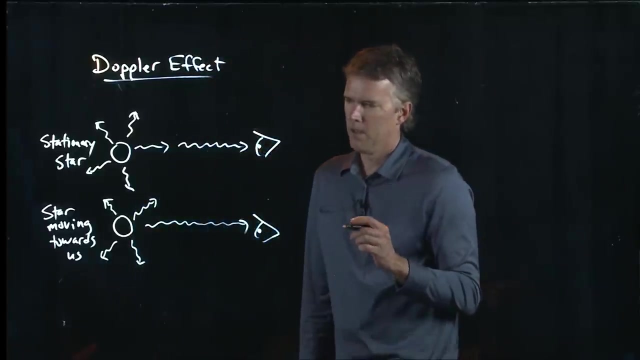 Stars are moving all over the place. Let's say we find one that it's moving towards us. Okay, It's still emitting light And some of that light gets all the way to us. When we look at that light, we can measure the frequency. 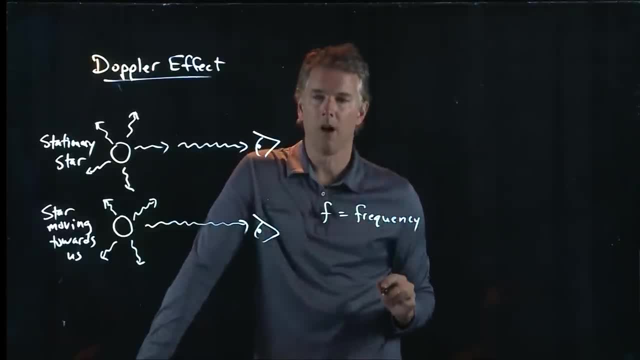 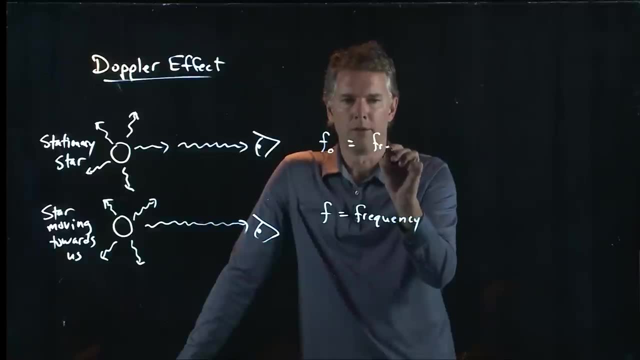 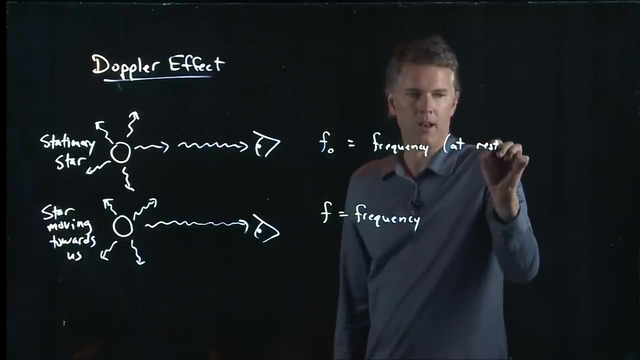 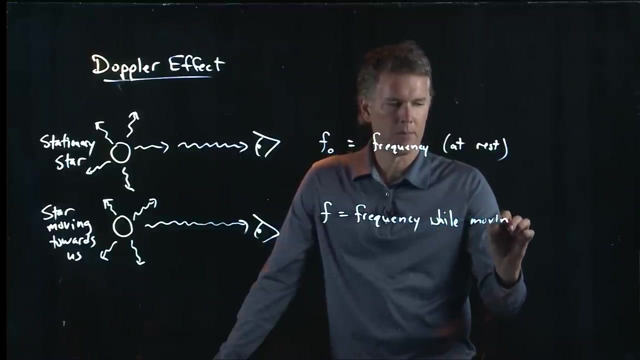 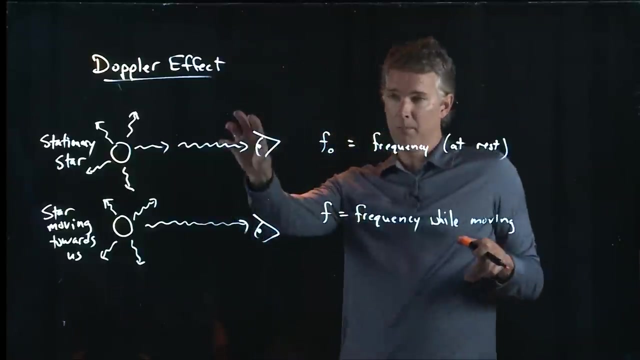 F is the frequency of that light. And let's say we did the measurement up here. We measured the frequency When it was at rest And we call that F naught. And let's measure this one and see how it compares With that star moving towards us. is this frequency the same as we measured before? 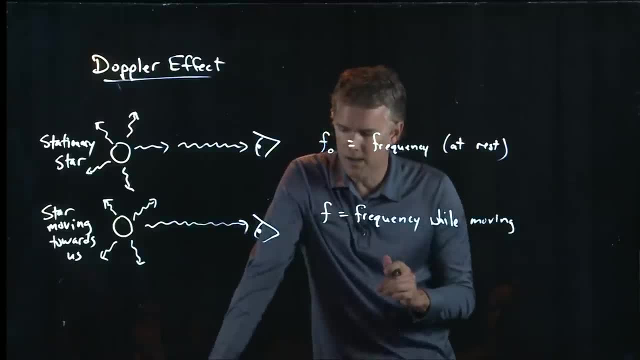 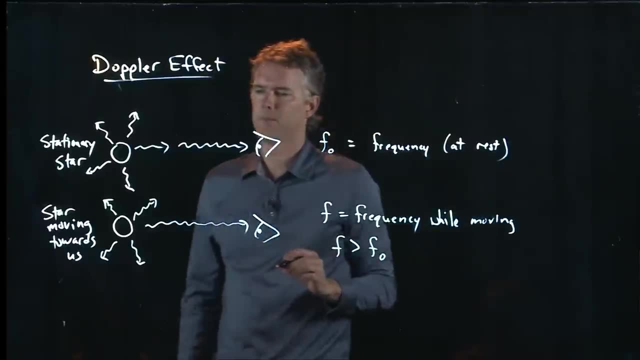 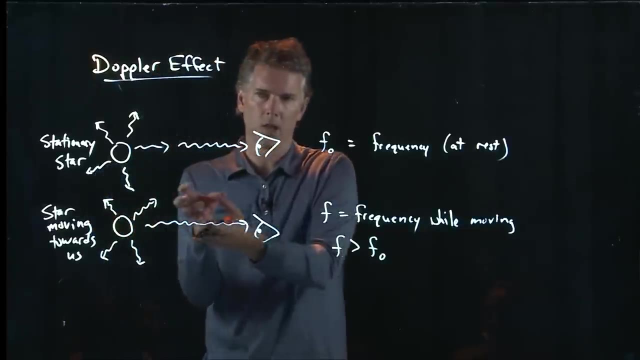 Or is it something totally different? Well, it turns out that the frequency is, in fact, bigger Than it was before, And one way to think about this is when you're exciting these waves And you're traveling along with the wave. 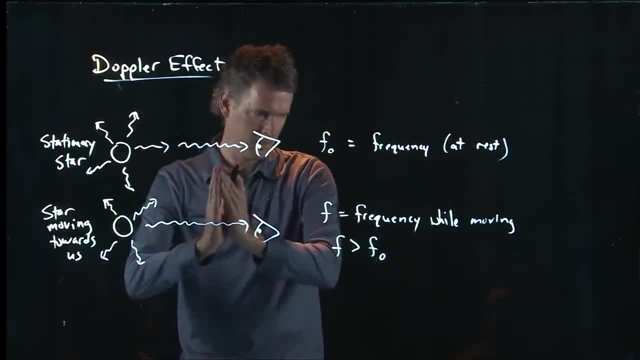 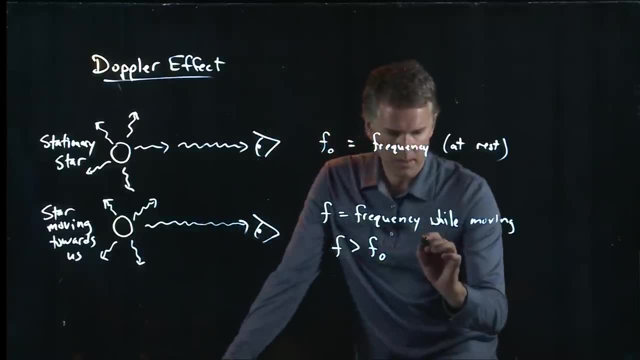 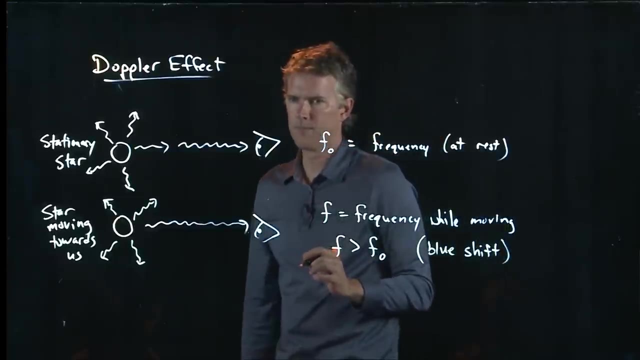 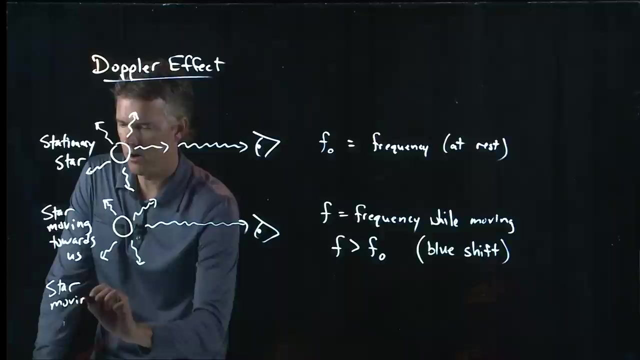 You kind of compress the wavelength. A shorter wavelength means it has to have a higher frequency. Okay, And this is something that you've heard of, It's called the blue shift. You've probably heard of the opposite, Which is when the star is moving away from us. 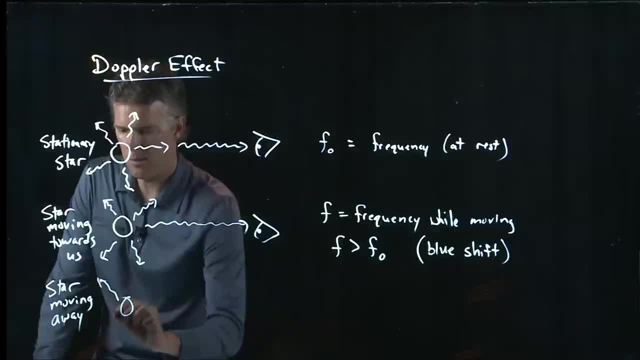 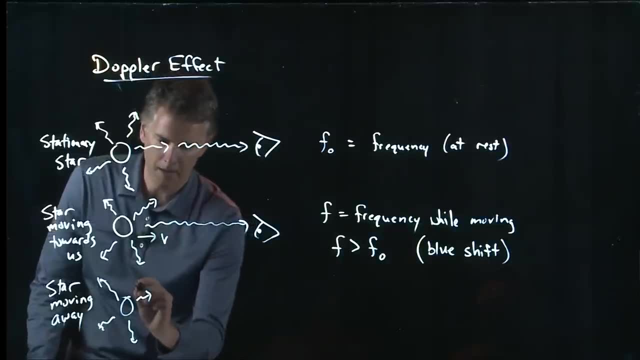 Okay. So now we're going to take that star And it's going to move away from us. In this one it was moving towards us with a speed v, And now it's going to move away from us with a speed v, And when that light gets to us, 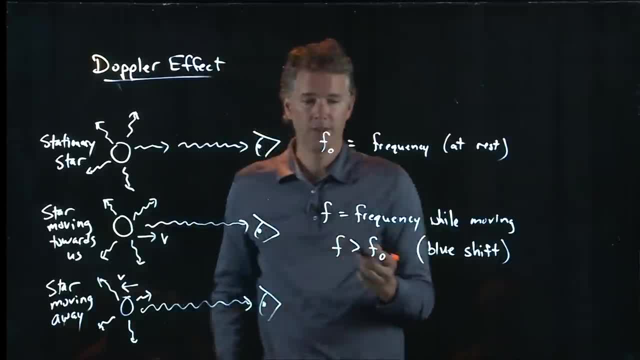 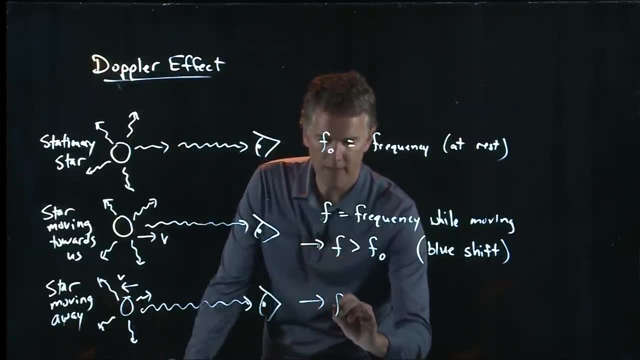 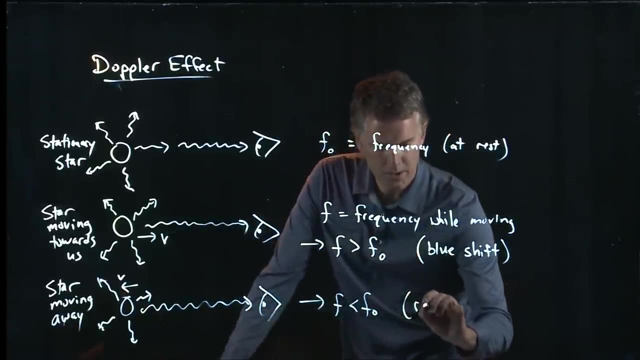 It, in fact, is shifted the other way In this case. So that was moving towards us, This is moving away. We have f is in fact less than f naught, And that's called a red shift. Okay. 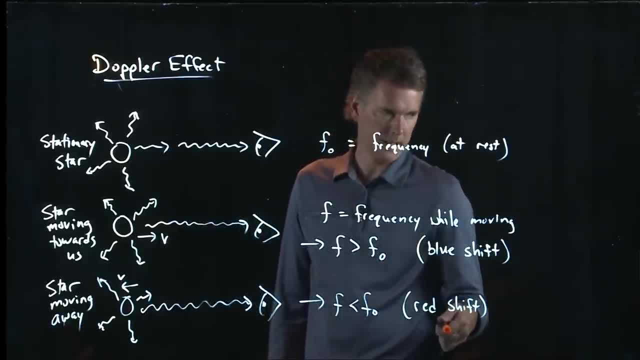 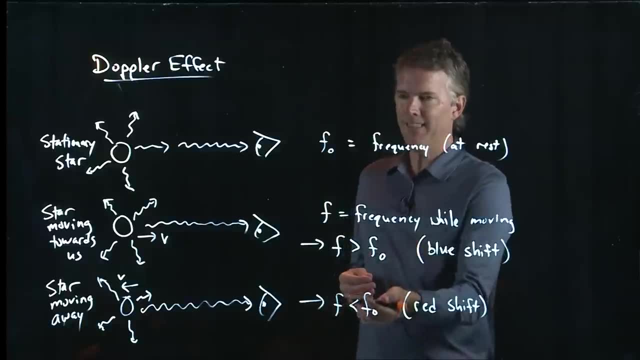 And this is probably something that you've heard about in astronomy classes. Right, We talk about the red shift of different stars out there, And what it means is the light that we observe has a different frequency than it should, Than it would if it was at rest. 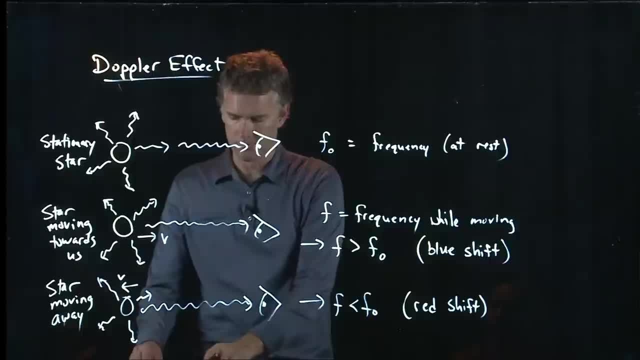 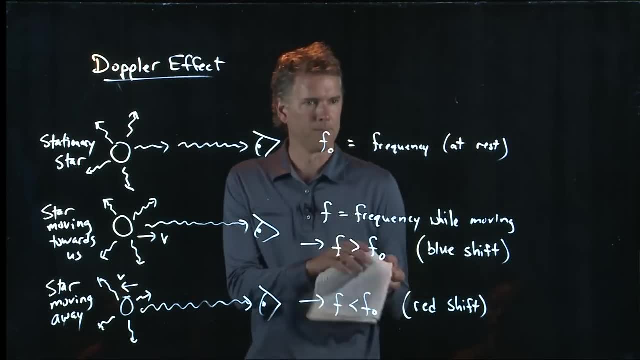 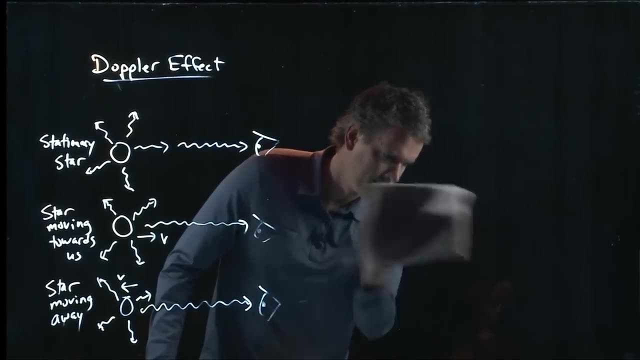 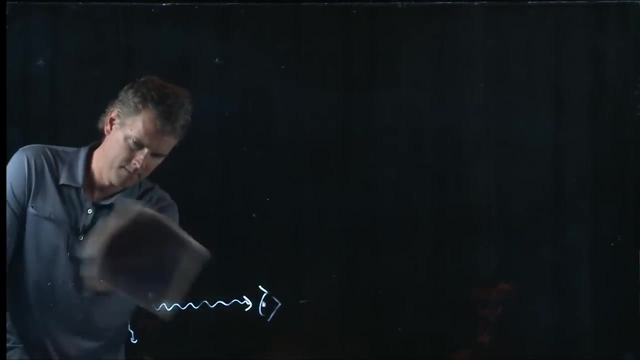 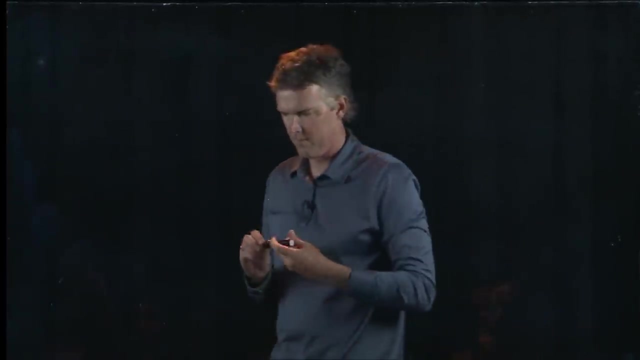 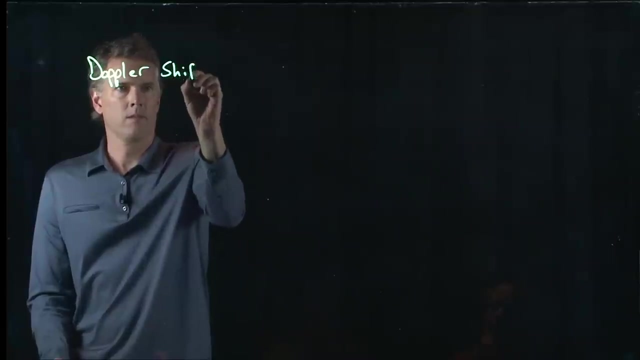 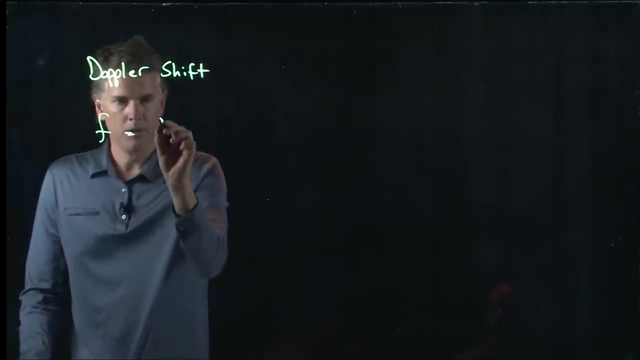 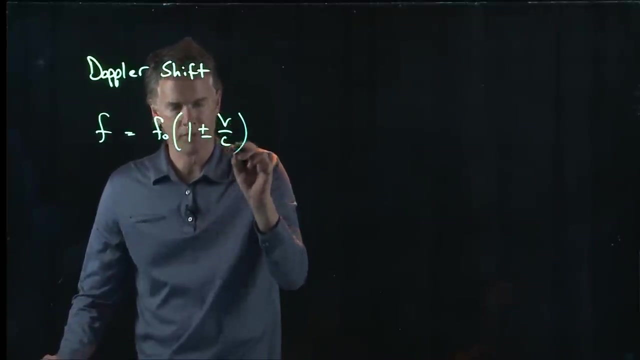 Okay, Now how does all this stuff tie together? How do we actually calculate the Doppler shift for different moving objects? So the equation that we need is the following: F is equal to f naught. F naught times 1. plus or minus v over c. 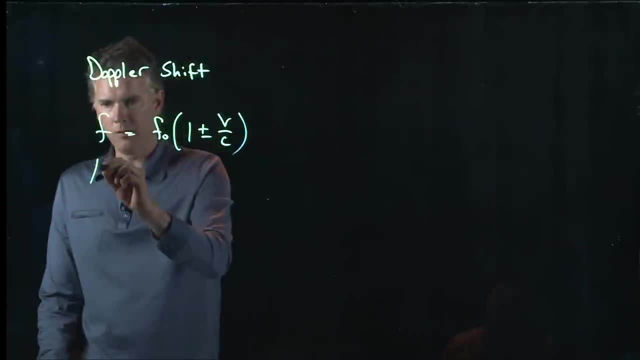 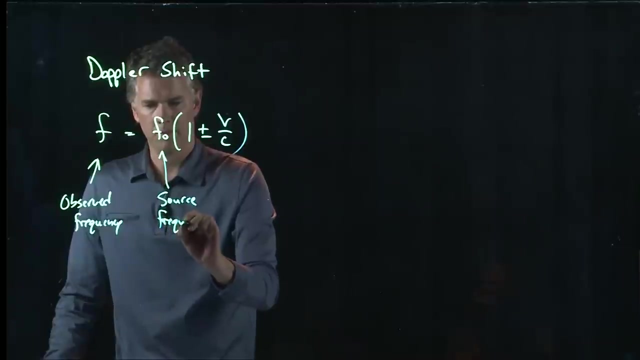 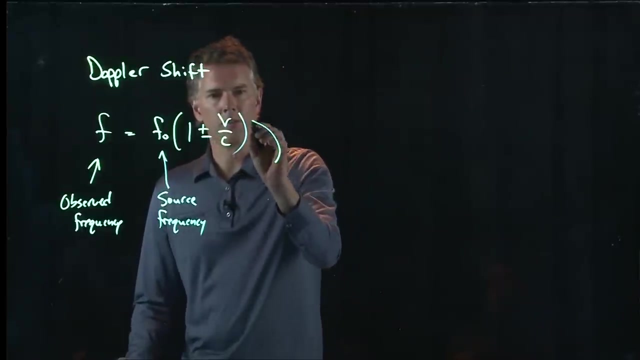 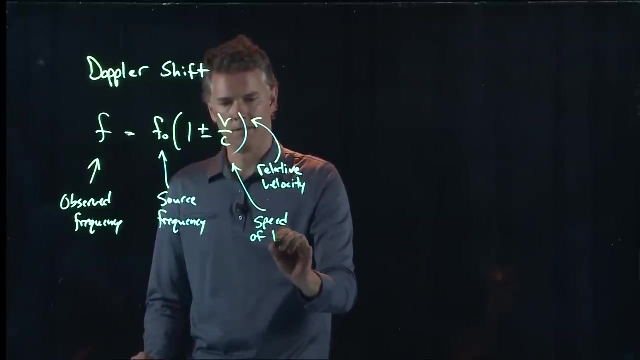 Okay, So this is the frequency that you measure, The observed frequency, This is the source frequency, That way that it's emitting. If it was all at rest, What would it be? V is, of course, the relative velocity, C is speed of light. 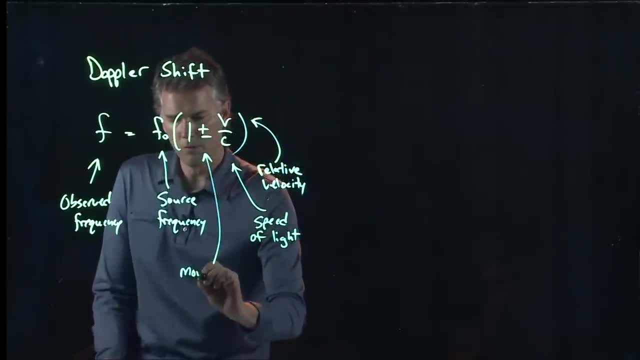 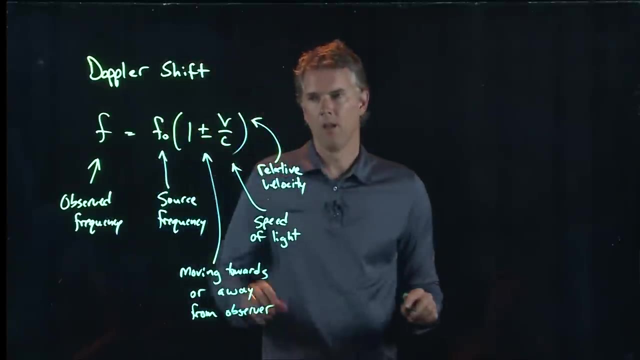 And this thing, the plus or minus, just means moving towards or away. Okay, So it's moving from the observer. Okay, Frequency can either go up if it's coming towards you Or it can go down if it's moving away from you. 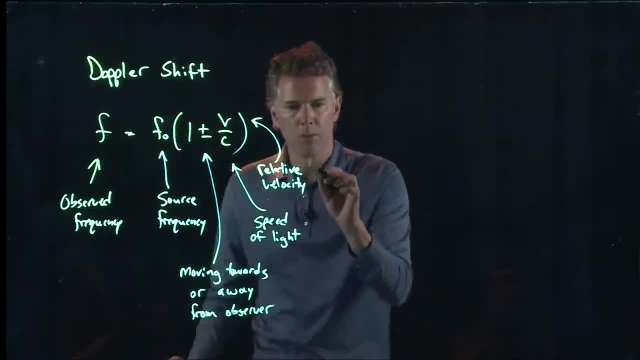 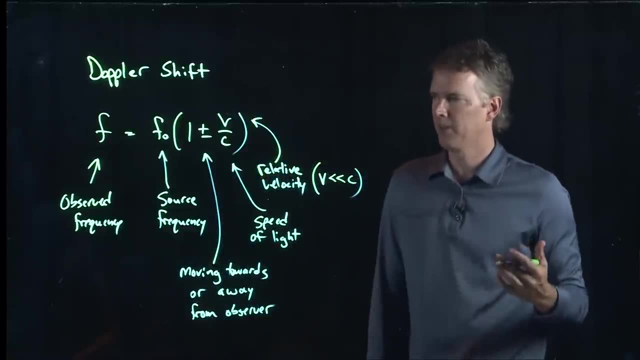 Now, this is true when the relative velocity v is much less than the speed of light. It gets a little more complicated once you get up to the observer. It gets a little more complicated once you get up to close to the speed of light. 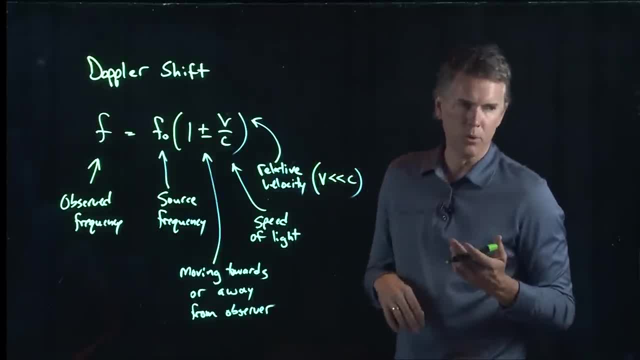 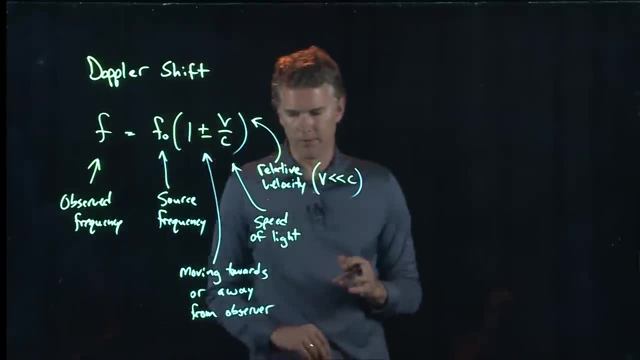 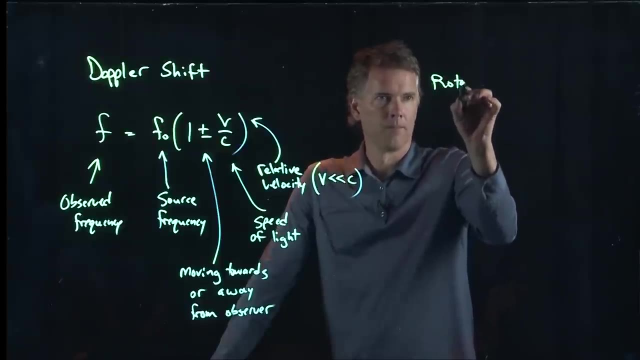 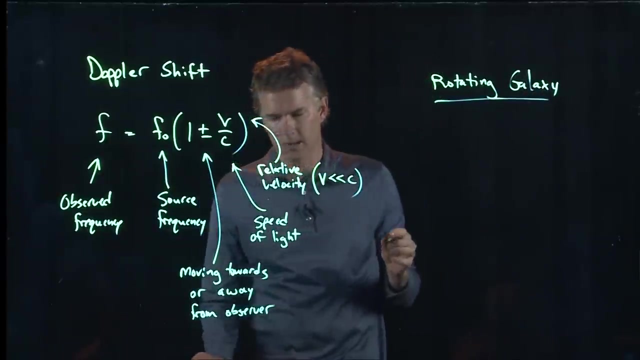 But for most objects that we're familiar with, the thing is not going to be moving anywhere near the speed of light. So let's take a look at an example of this, And let's look at a rotating galaxy. Okay, So a rotating galaxy looks sort of like this: 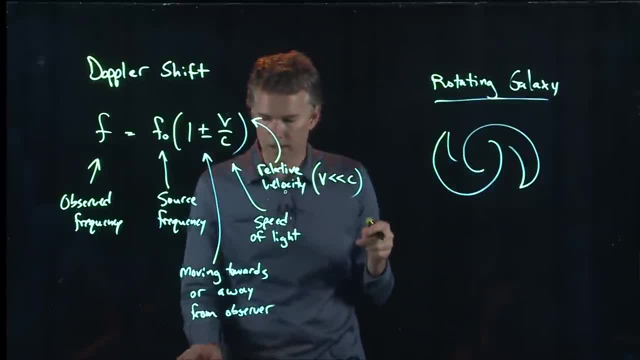 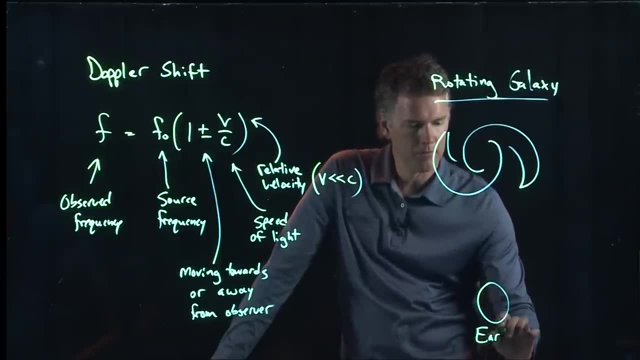 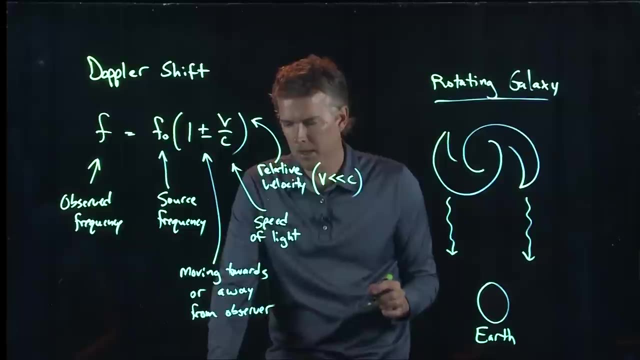 It's got these spiral arms on it And the whole thing is spinning And as it spins it emits light that we can observe down here on the Earth- not to scale, Okay- And the thing is spinning in this direction, So there is some point here which has some speed v. 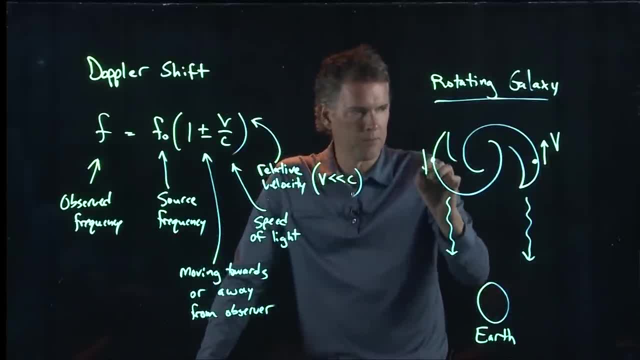 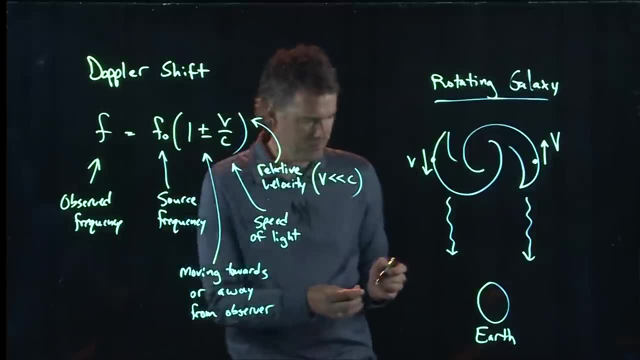 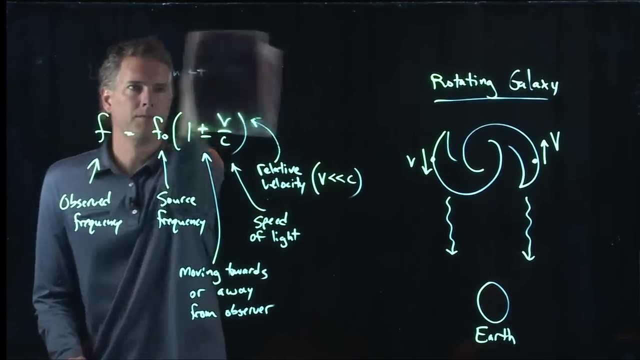 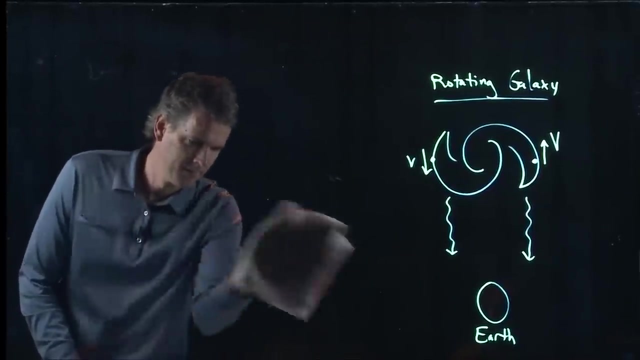 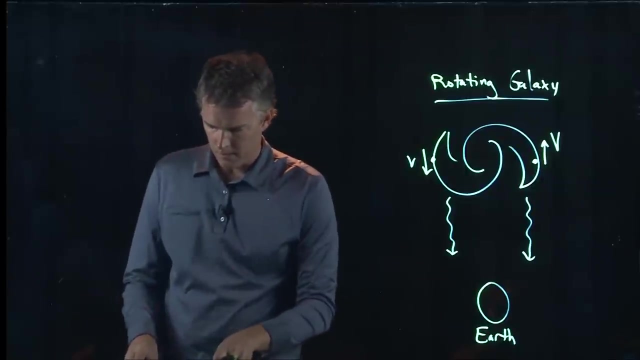 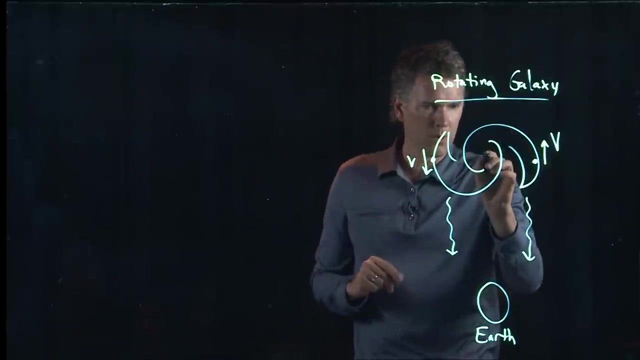 There's some point on the other side which has some speed v, And so the whole thing is spinning around like that. All right, Let's see if we can calculate some stuff about this galaxy using the Doppler shift. Okay, So we're going to say that not only is the whole thing spinning, but the whole thing is moving away from us. 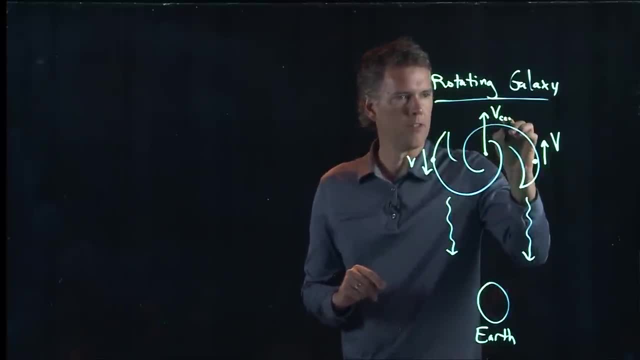 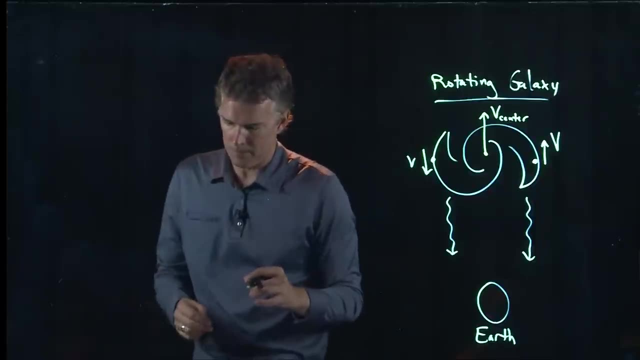 And we'll call that speed v of the center. Okay, It's moving away from us And it's rotating. So we have this complicated system And let's write down some givens. So the speed that it's moving away from us is: 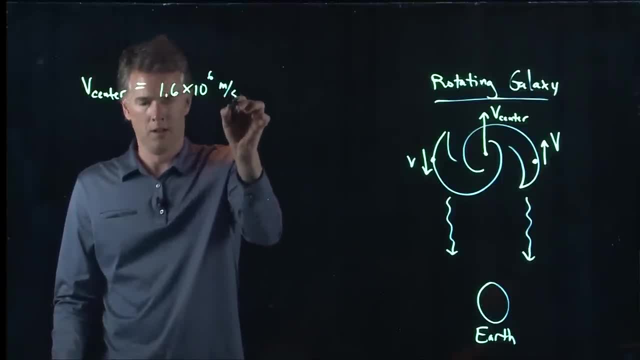 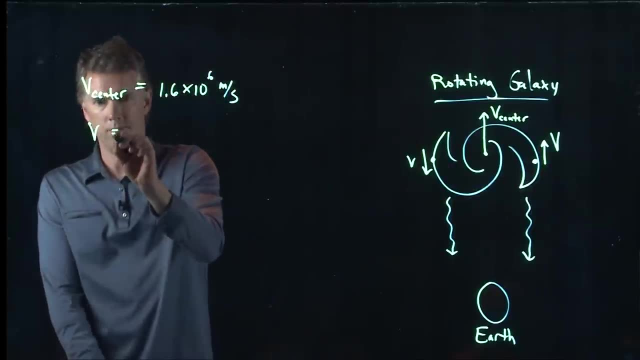 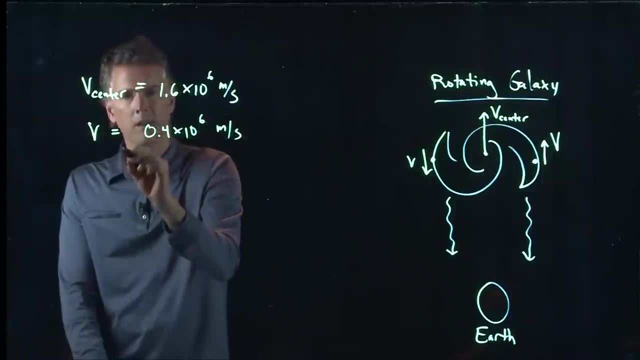 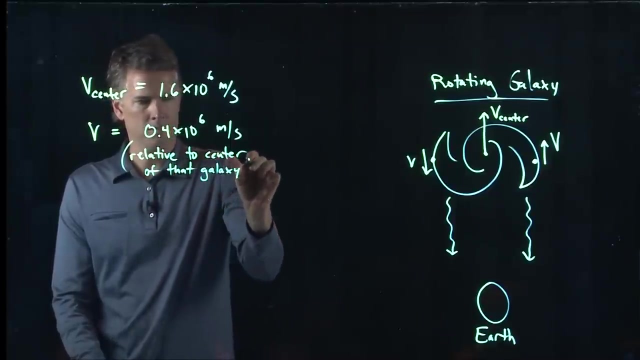 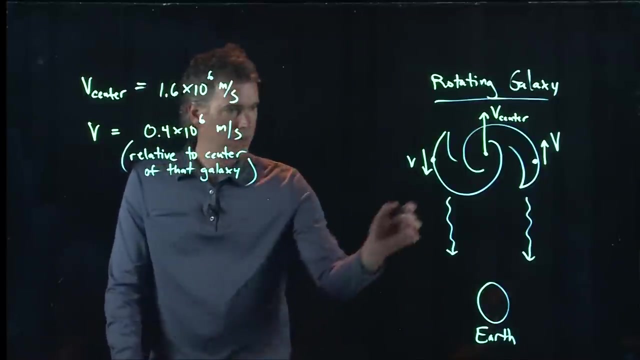 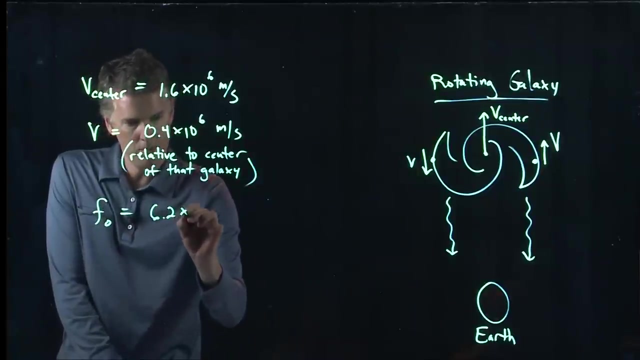 1.6 times 10 to the sixth meters per second. The speed here v is 0.4 times 10 to the sixth meters per second, But this is relative to the center of that galaxy. Okay, The source of the light has a frequency f-naught of 6.2 times 10 to the 14 hertz. 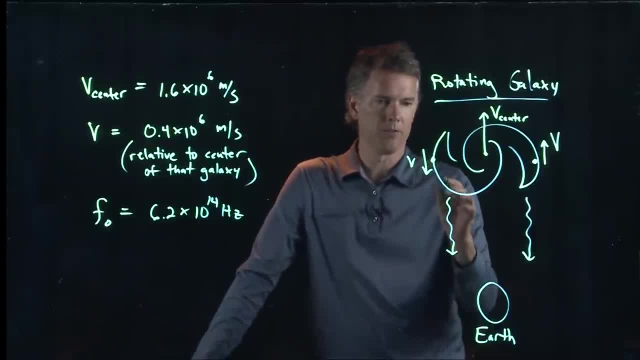 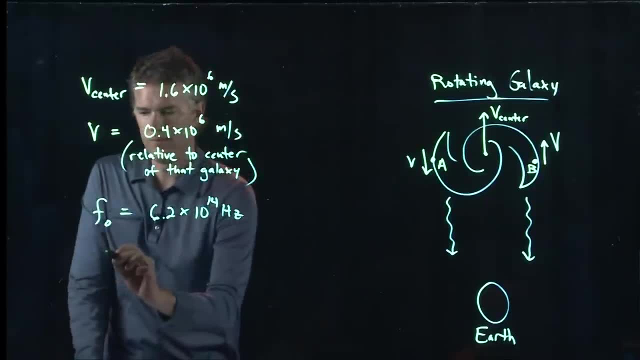 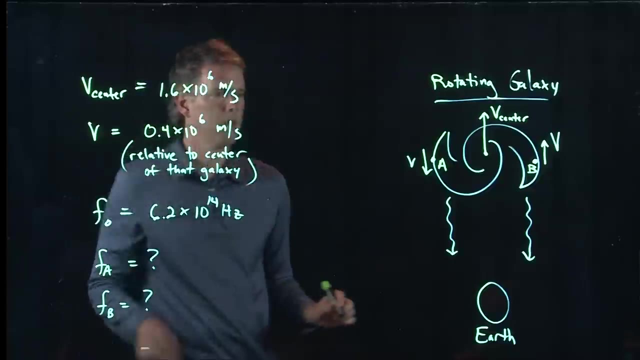 And now we want to find the following: We want to figure out what is the observed frequency from A And what is the observed frequency from B. Okay, You've got a star on this side that is emitting some light And we're going to collect it. 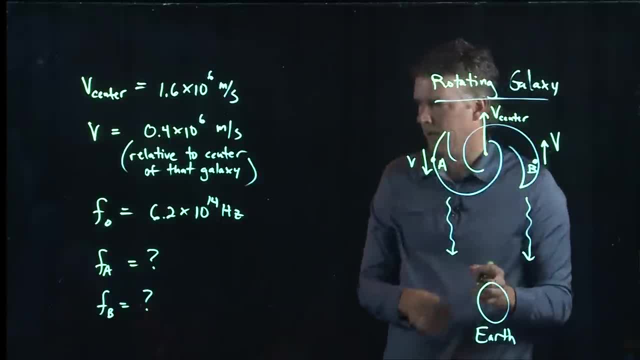 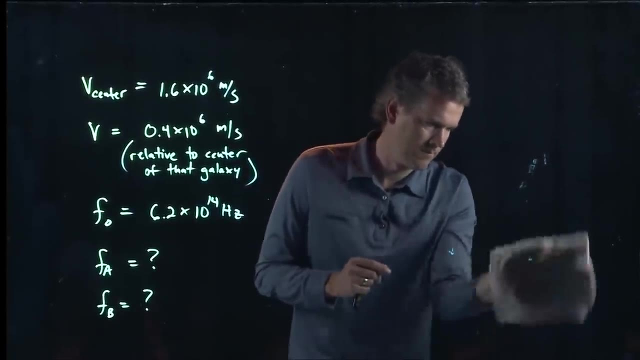 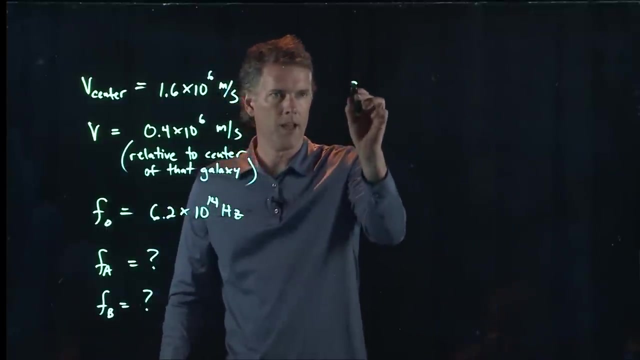 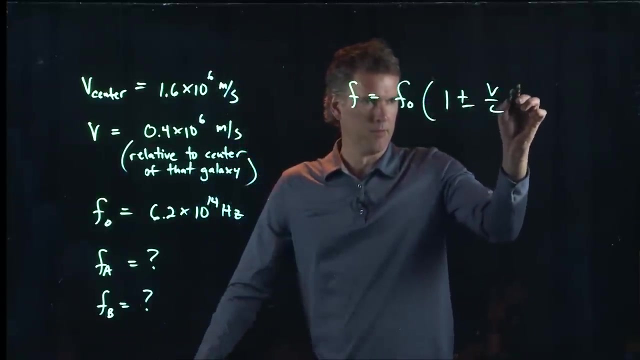 You've got a star on this side that is emitting some light And we're going to collect it And we want to figure out what those frequencies are. Okay, So we go back to the Doppler shift. So the Doppler shift we said was: f equals fo times 1 plus or minus v over c. 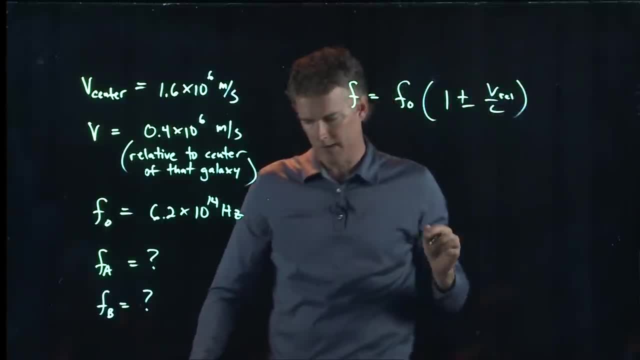 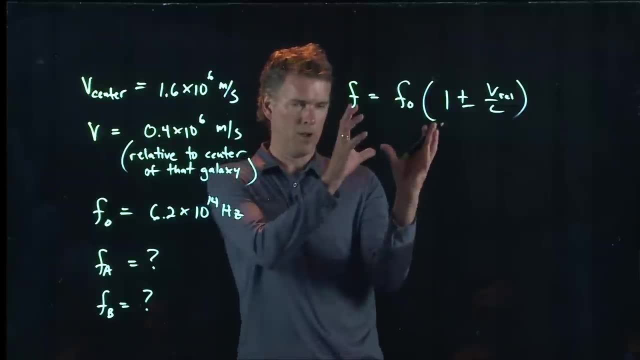 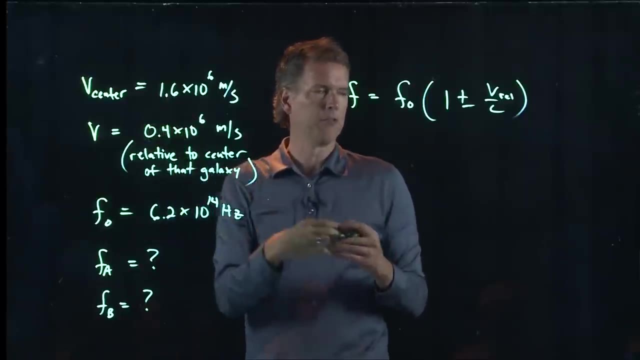 But remember, that is relative to us. Okay, So we're going to label that v relative. And the whole galaxy is moving away from us? Okay, And it's moving away from us faster than it's moving away from us. Okay, And it's spinning. 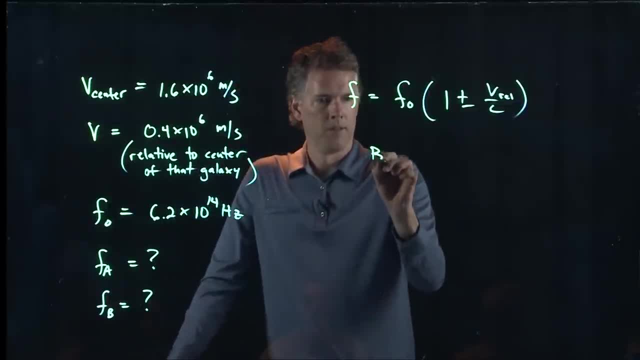 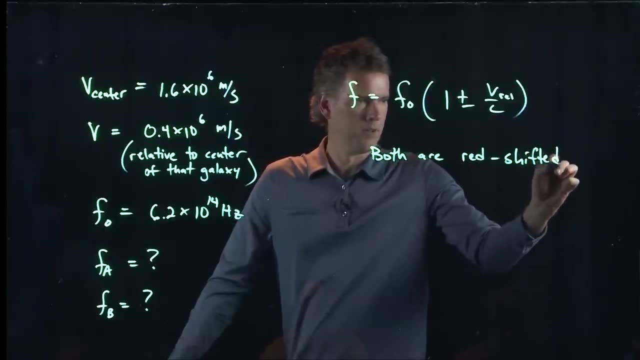 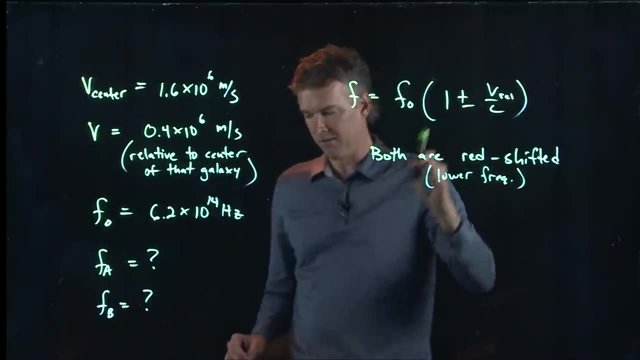 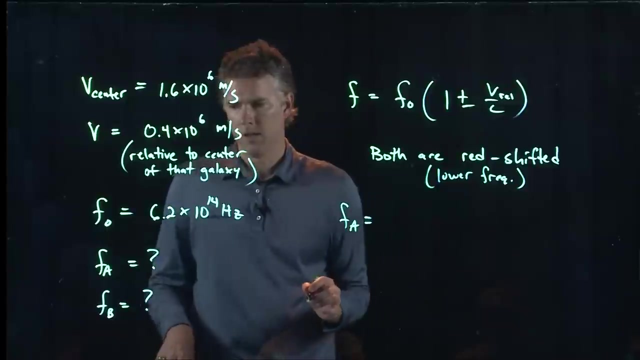 And so both of these are going to be redshift. Both signals are in fact redshifted, Which means lower frequency, And so we want to use the minus sign in our equation. Okay, So what is fa going to be? It is the natural frequency fo. 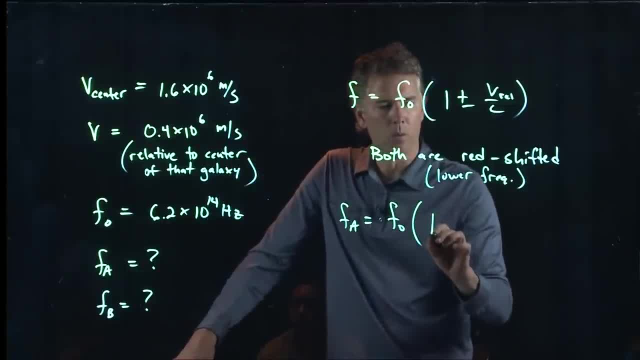 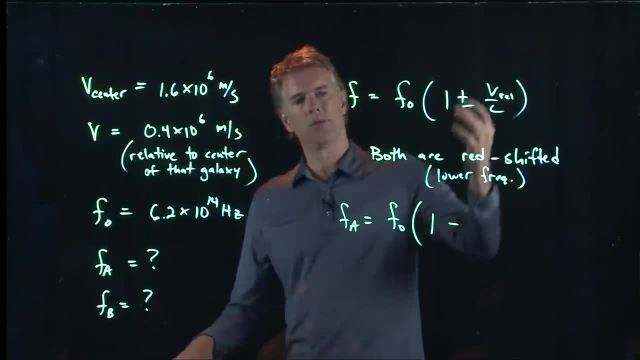 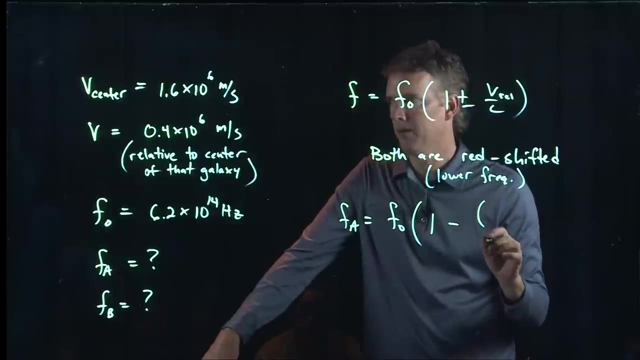 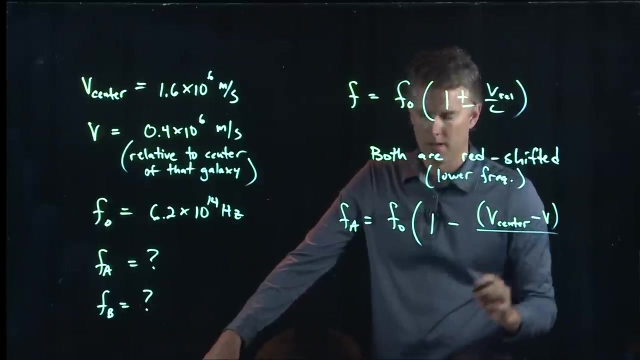 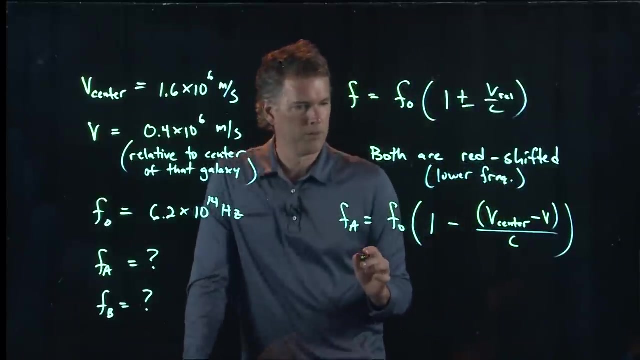 And then we have 1 minus v relative, Okay, But remember, the a side was coming towards us, as the galaxy was moving away from us, And so we in fact need to put up here v center minus v, all over c. Okay, And now we have all those numbers. 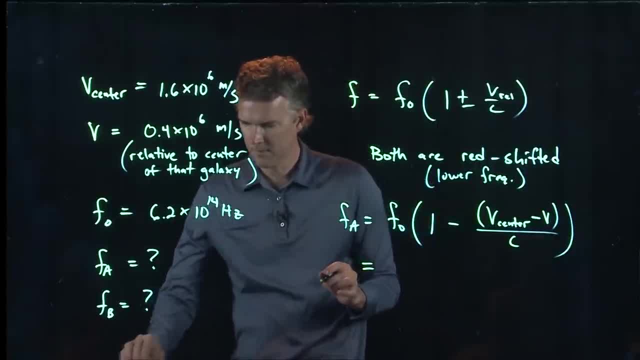 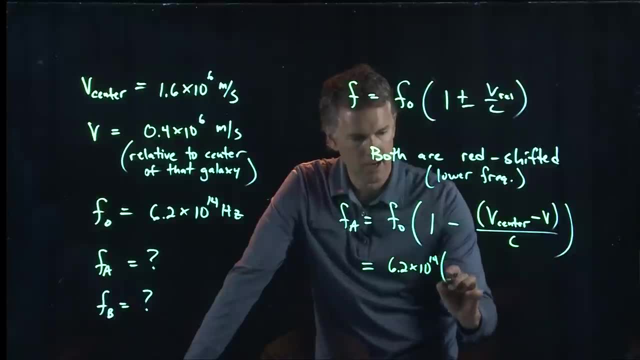 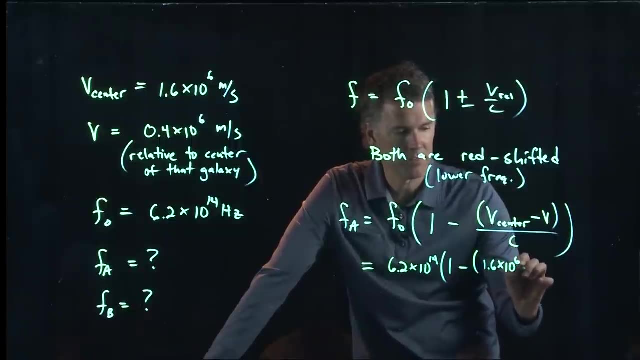 And so we can punch them in and try it out, And let's do that. We've got 6.2 times 10 to the 14. Out in front we have a 1 minus this thing, which is 1.6 times 10 to the 6.. 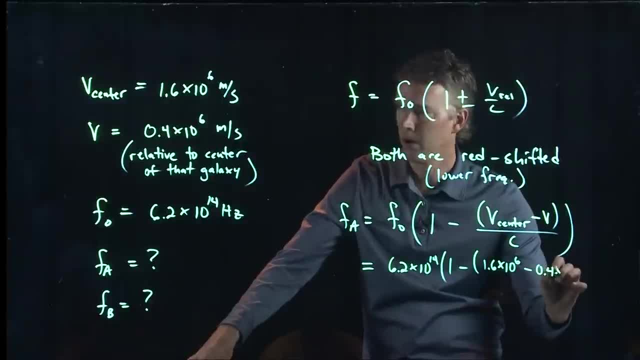 Minus the rotational speed, which is 0.4 times 10 to the 6.. And then that last bit is all over c, which we know is 3 times 10 to the 8 meters per second. Okay, We'll just keep SI units on everything. 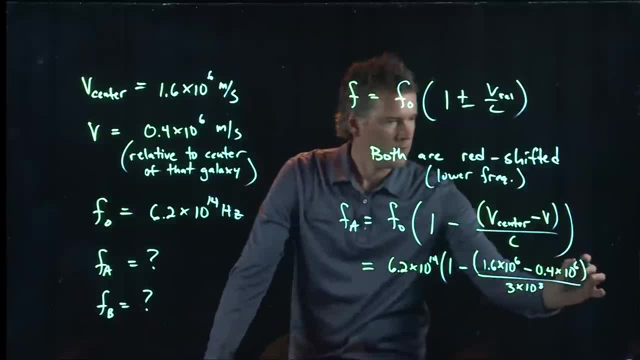 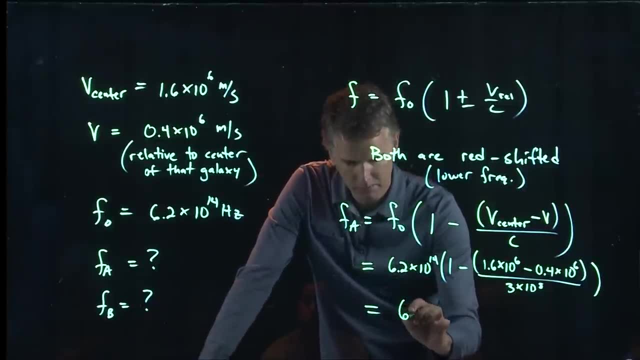 We don't have to write the units, Close the parentheses And if you do that you should get. you can double check my numbers. I got 6.1752 times 10 to the 14 hertz. Okay, And that was the frequency of a. 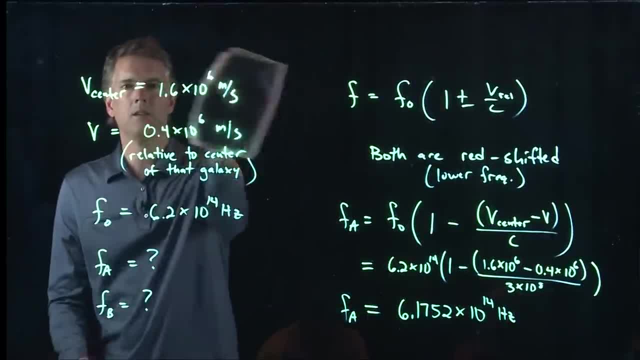 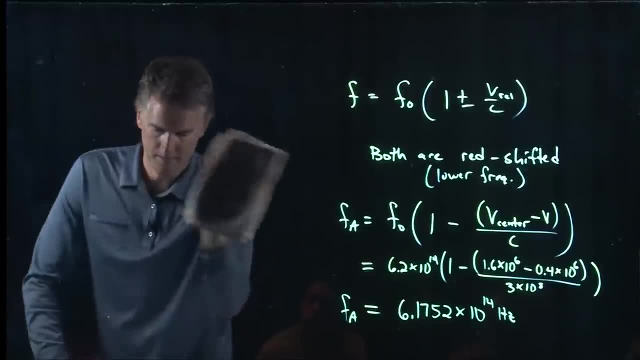 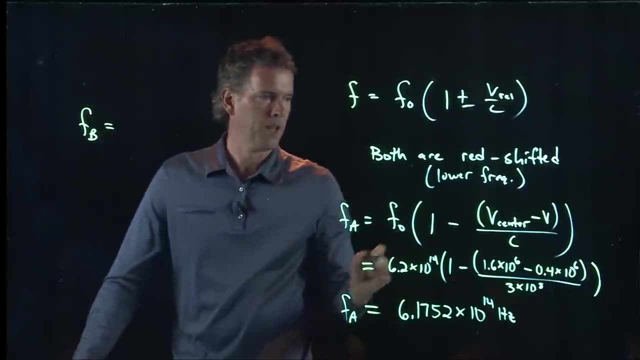 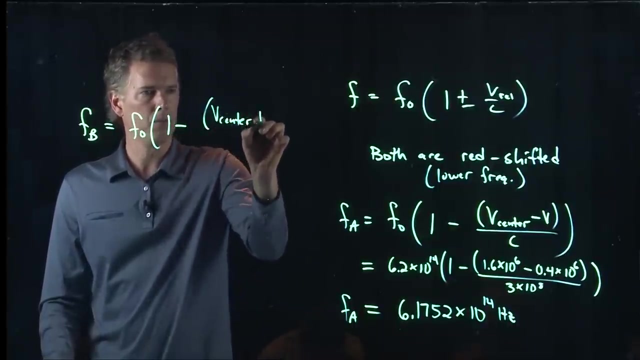 Now, if you do the other side, frequency b, what do you get? Frequency b is going to look very similar, except we're going to change one of these signs. So it's 1 minus v center plus 1.. v center plus v all over c. 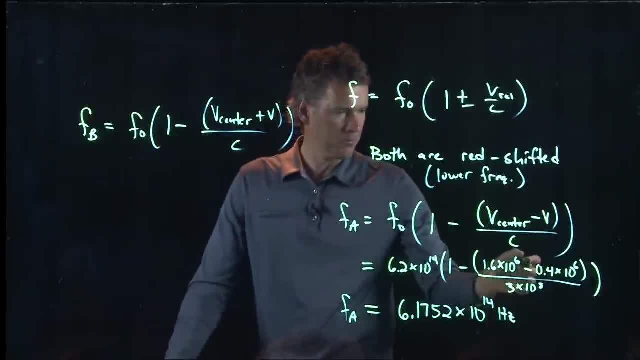 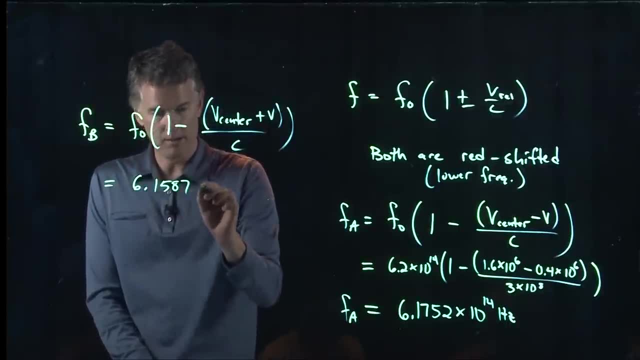 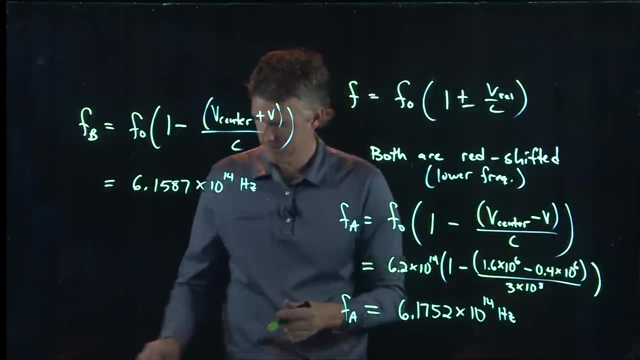 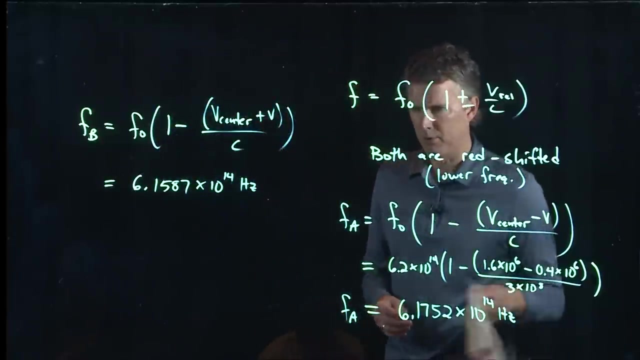 And now it's the same numbers You're going to plug in. You just put a positive sign right there, And if you do that, you should get 6.1587 times 10 to the 14 hertz. Okay, So this is the Doppler shift. 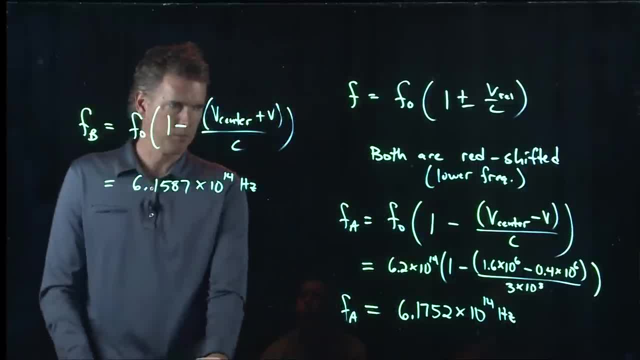 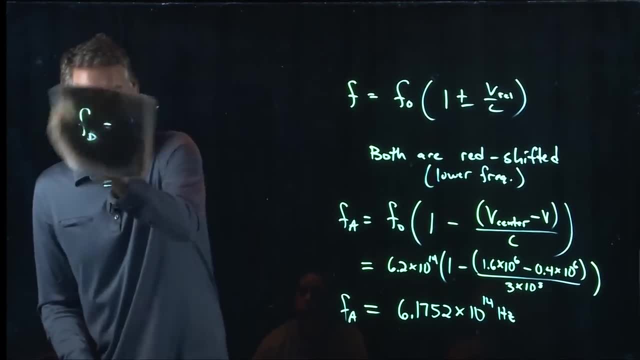 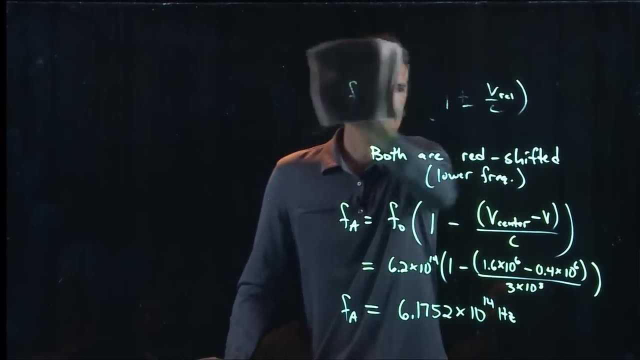 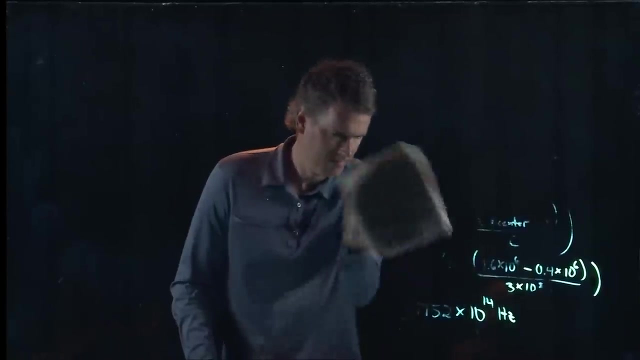 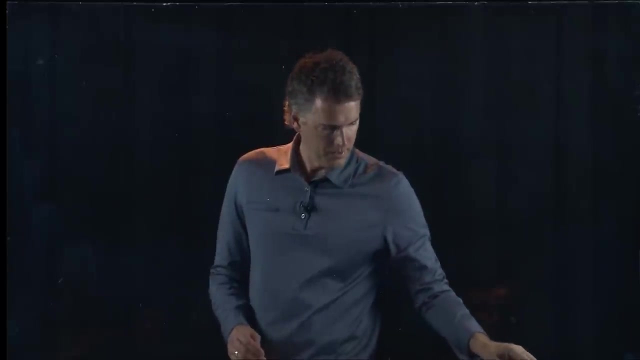 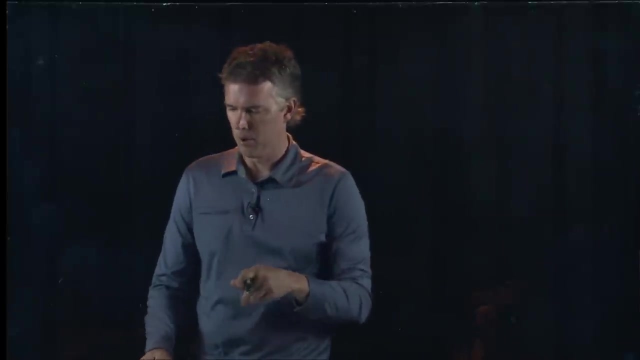 It's something that's not in your textbook chapter, But I think it's really important to understand what's happening in our universe, And especially since this has such an impact in astronomy. Okay, One thing that we need to talk about is this idea of polarization. 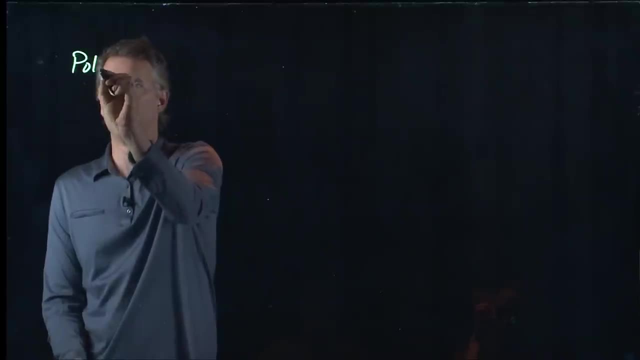 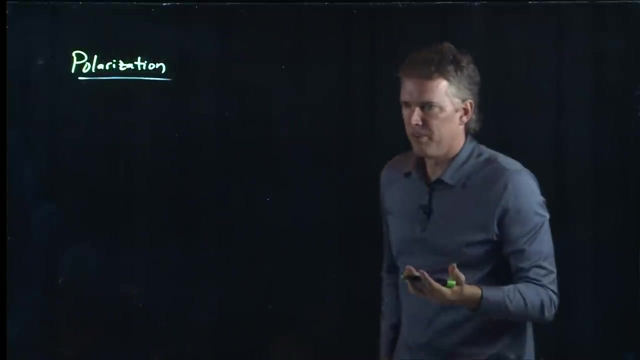 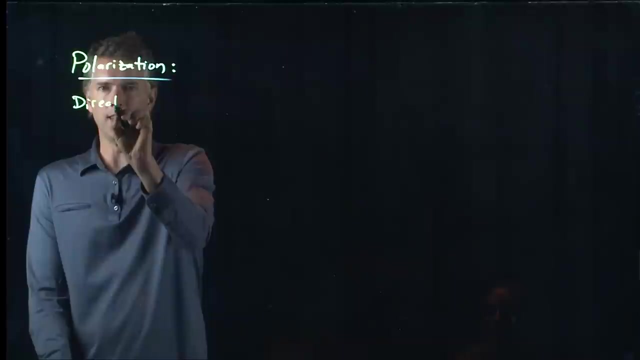 Okay, And this is going to come back again later on when we start talking a little bit more about optics. But when we say polarization, what do we mean? Polarization is the direction of the ephemeris, The direction of the e field. 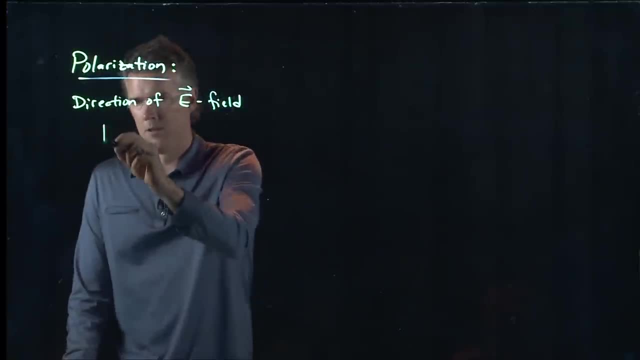 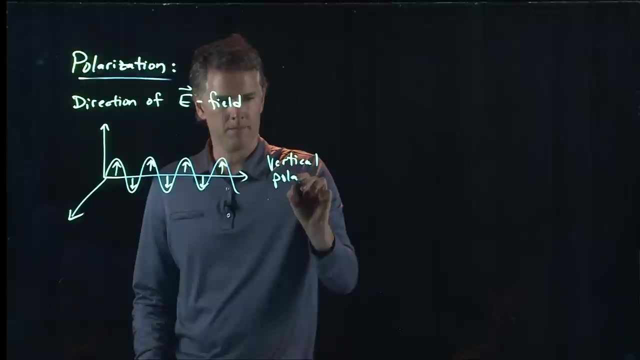 Okay, This is just how it's defined. So, for instance, if my wave has an e field that's going up and down, Then we say that it has vertical Polarization. Okay, We don't really care about what the b field is doing. 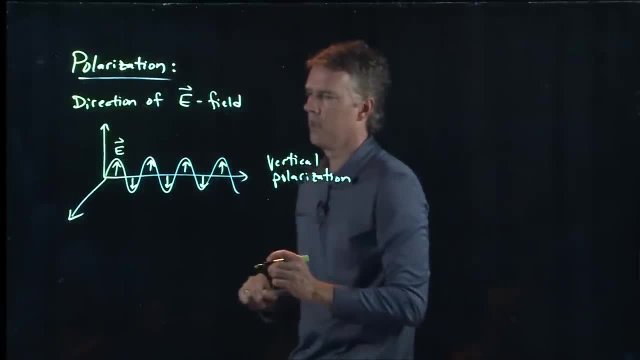 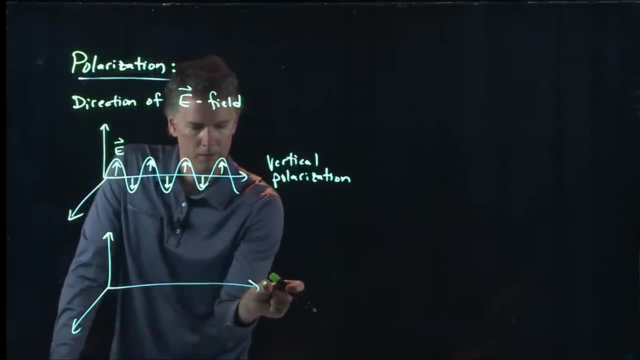 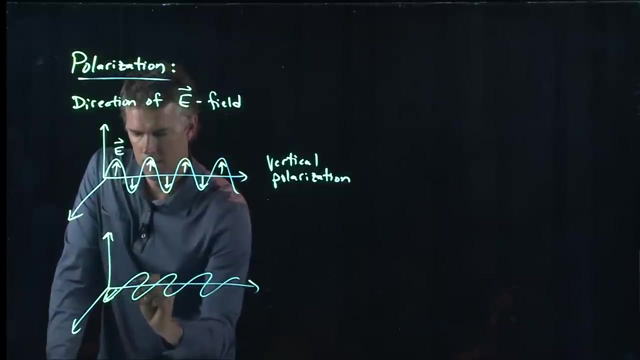 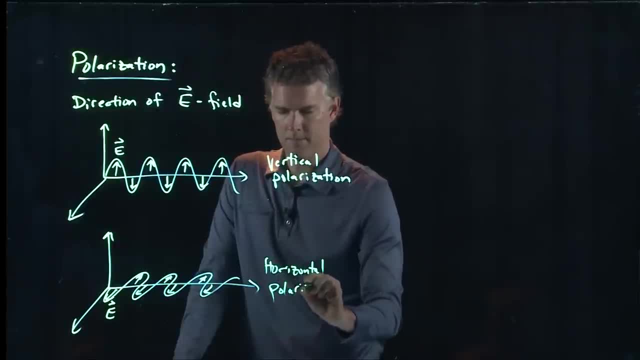 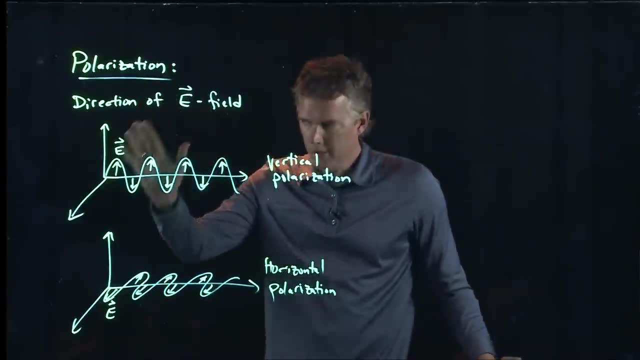 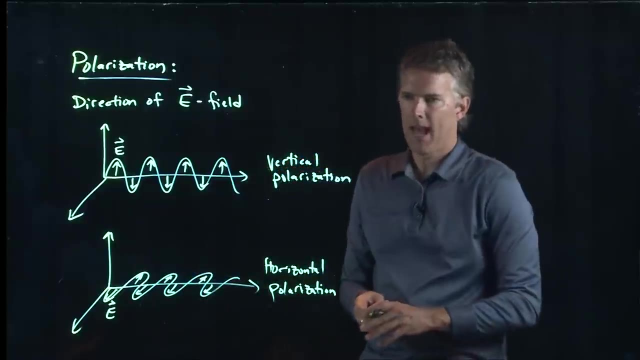 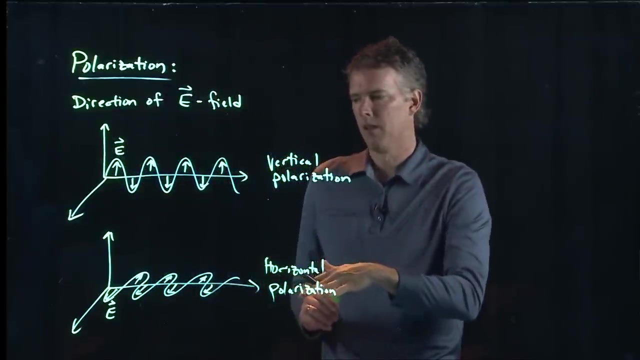 Then this is called horizontal polarization. Okay, So these are the two polarizations for an electromagnetic wave, Either horizontal or vertical. And things like lasers have a preferred orientation for their electric field. for their electric field They either come out vertical or horizontal. But things like 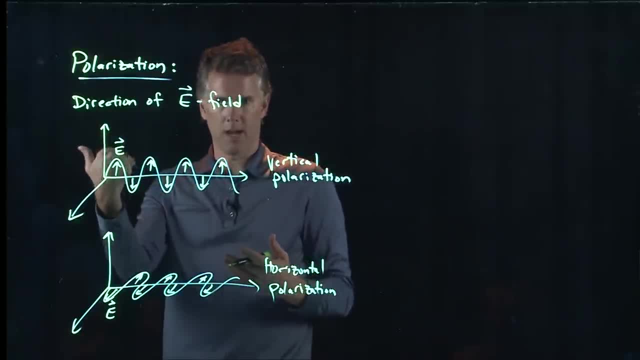 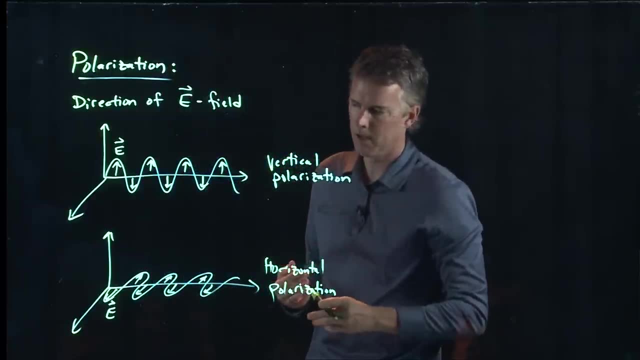 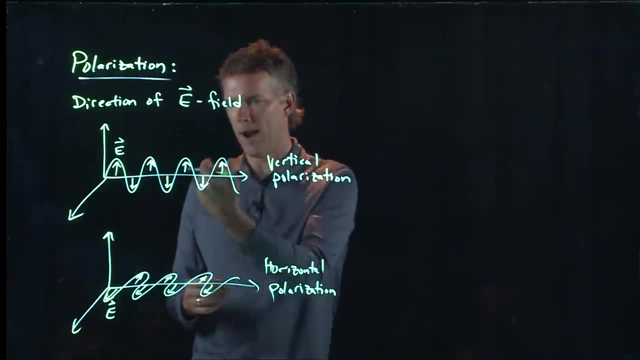 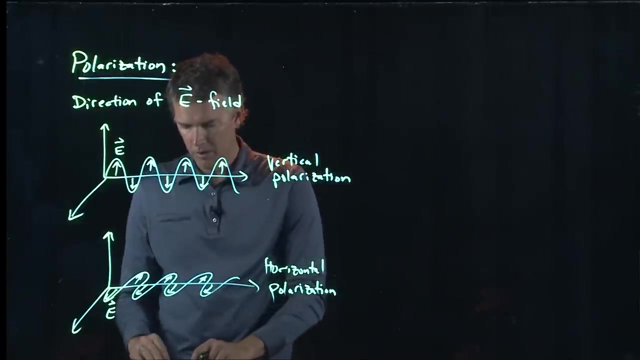 sunlight have all different polarizations. They have a vertical component, they have a horizontal component and then they have all the different angles in between. So incandescent sources, like sunlight, like a light bulb, those will have random polarization, whereas lasers will have defined polarization. So you're familiar with this because of two things. 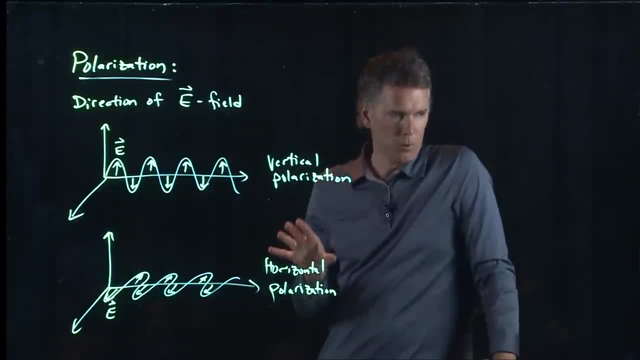 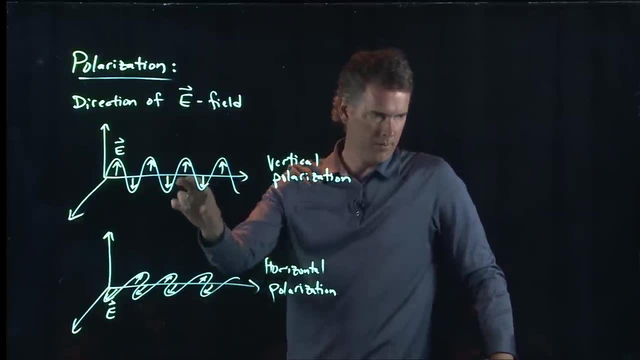 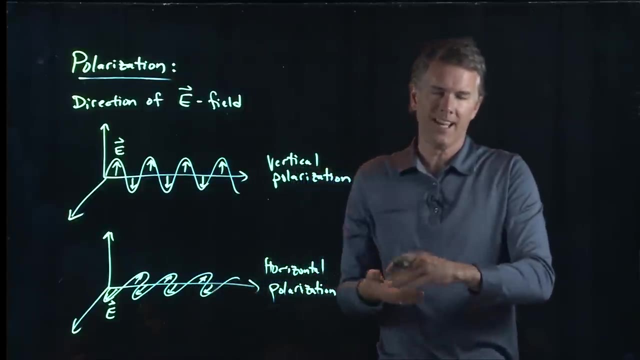 One is: you might have sunglasses that are polarized, And what polarized sunglasses mean is they block one of these polarizations. It turns out that the glare off the ocean or the glare off a wet street is dominantly polarized in one direction. 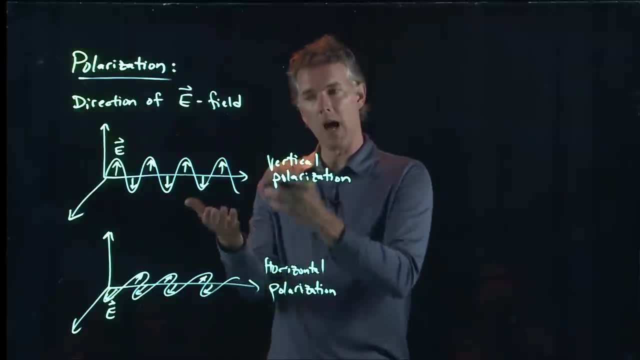 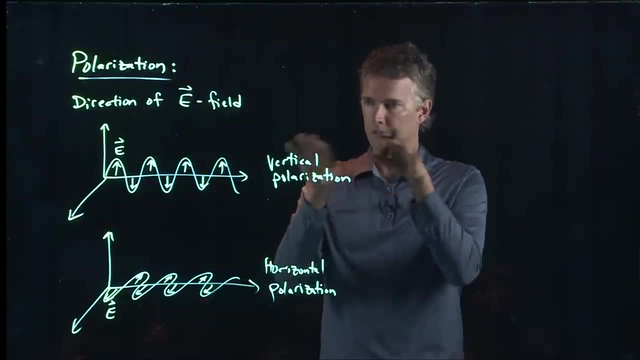 And so if you put on your sunglasses to just block that particular polarization, you essentially cut out the glare. Okay, So when you're looking at the ocean, you see a bunch of glare. Put on your polarized sunglasses, the glare goes away And that's because that glare is polarized. 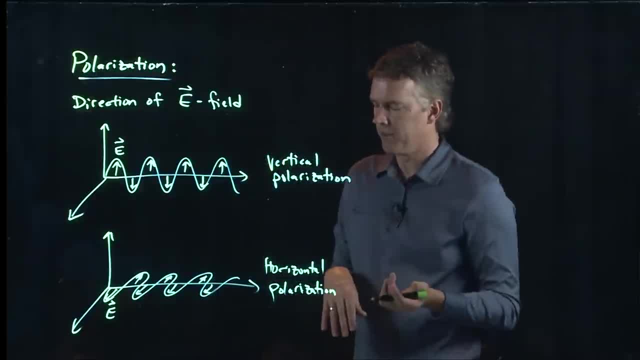 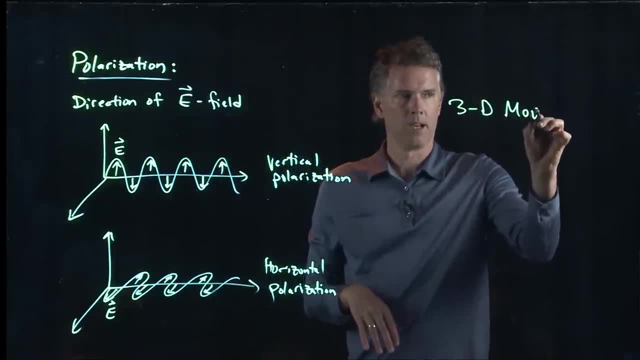 in one direction. your polarized sunglasses block it. But this is also used in things like 3D movies. Okay, 3D movies take it in a different direction. They're not just called 4D, They take it in this direction. 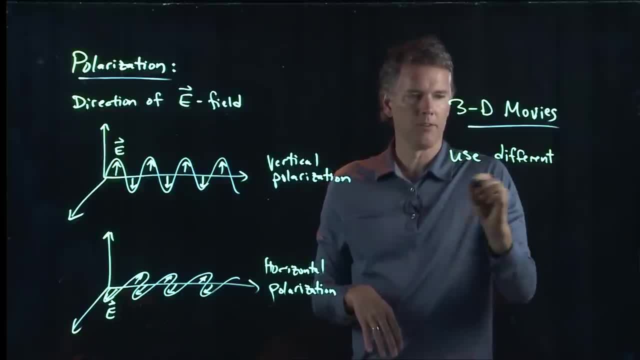 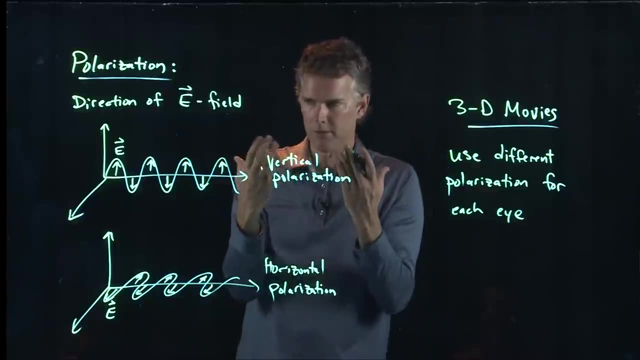 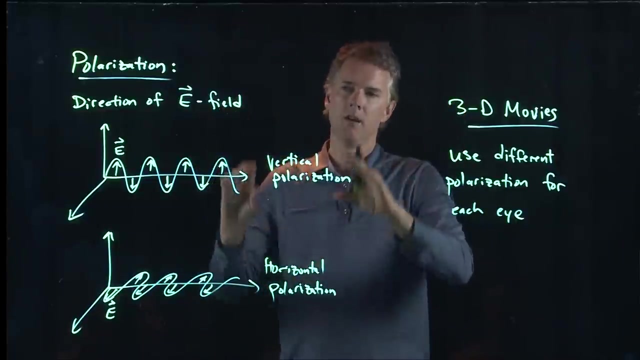 So that's the advantage of polarization, And basically they use a different polarizer for each eye. Okay, So if you go to a 3D movie and you get those glasses, what those glasses are doing is there is a different polarization on the left eye than on the right eye, And 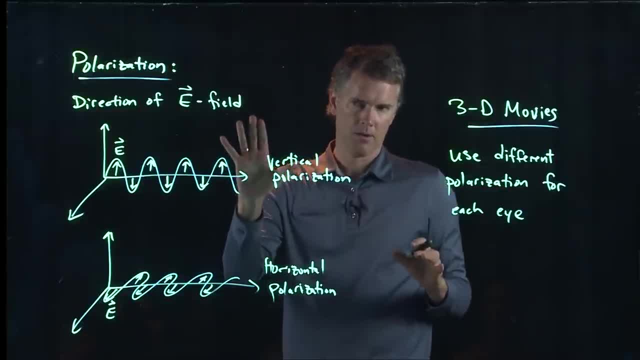 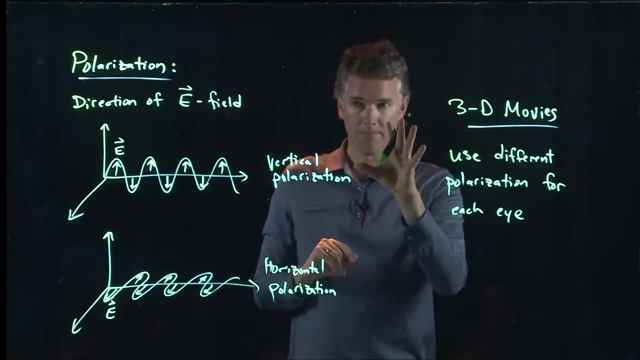 so when they project it on the screen with a certain polarization, they want to get those glaring glasses on the other side from the lamp and they use some polarizers to do it. they're creating a different image for your left eye than your right eye. so now, when you put them, 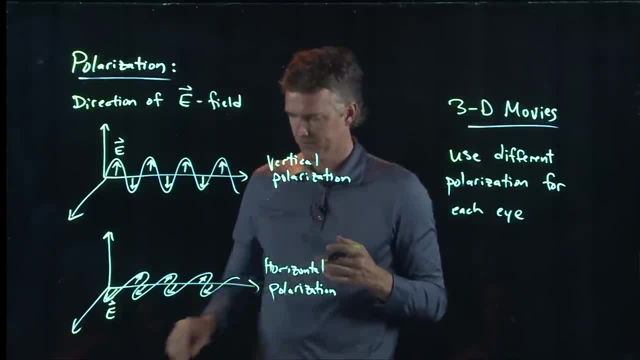 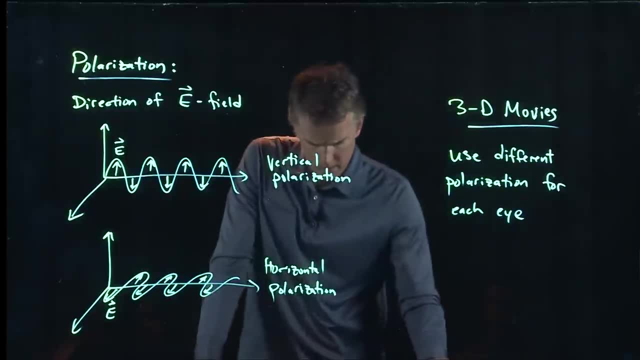 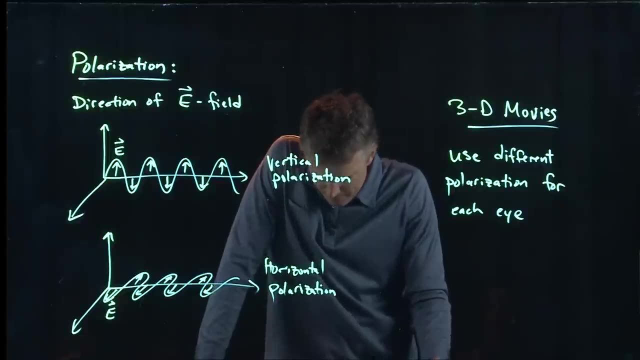 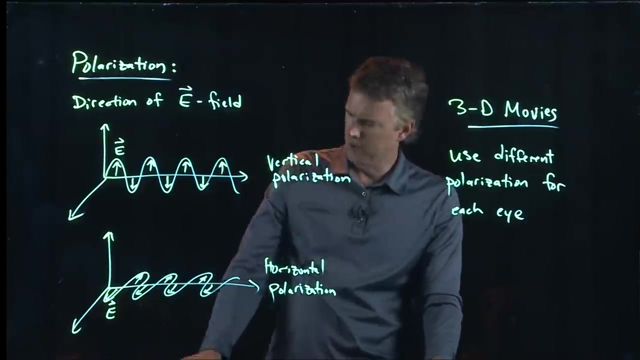 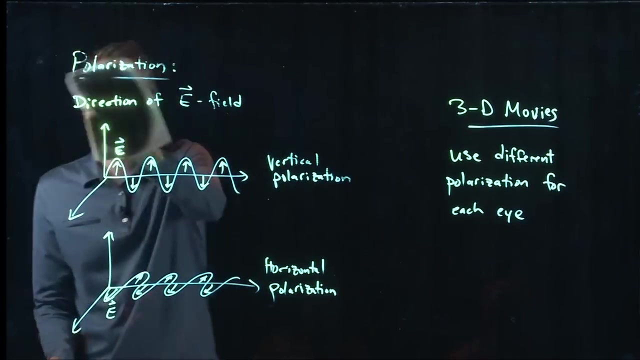 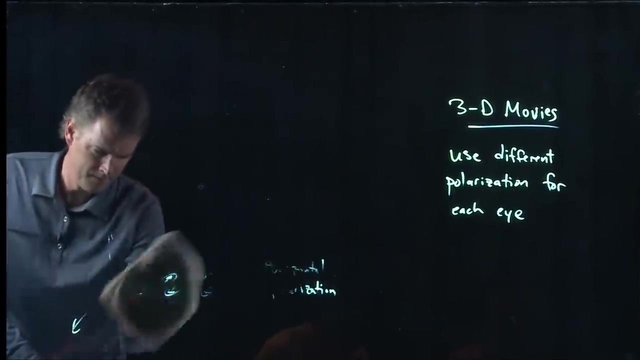 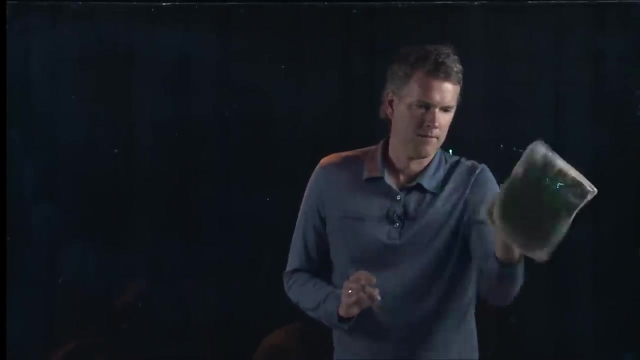 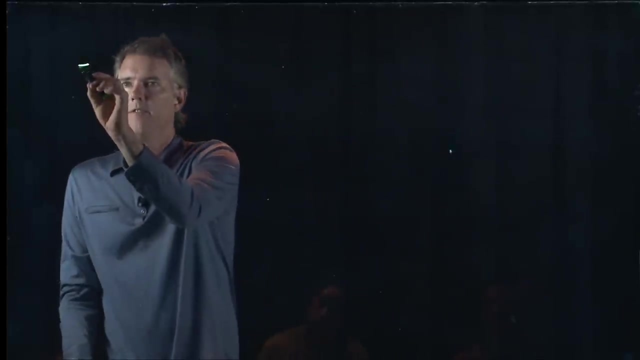 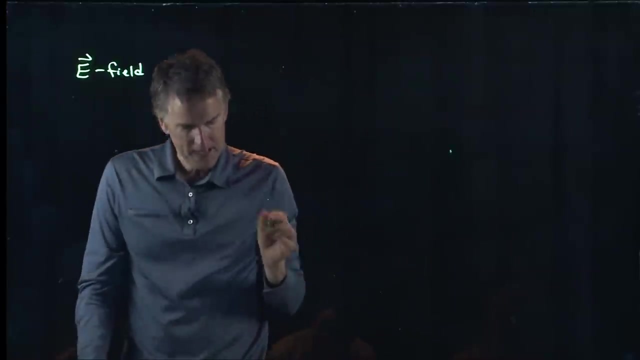 back together. it looks like a 3d picture to you. okay, let's take. take a look at one another, one of your homework problems. okay, so this relates to stuff that we talked about yesterday. let's look at 22.22. okay, so it says the following: the E field in an EM wave has a peak value. 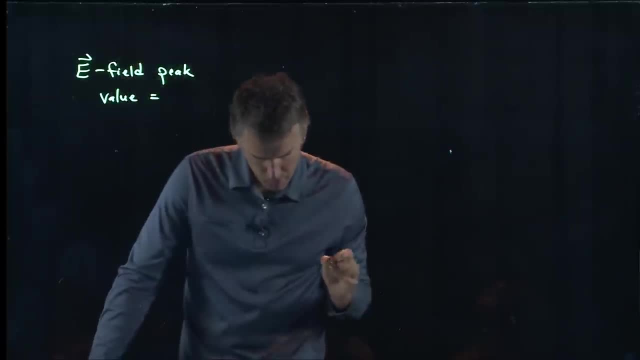 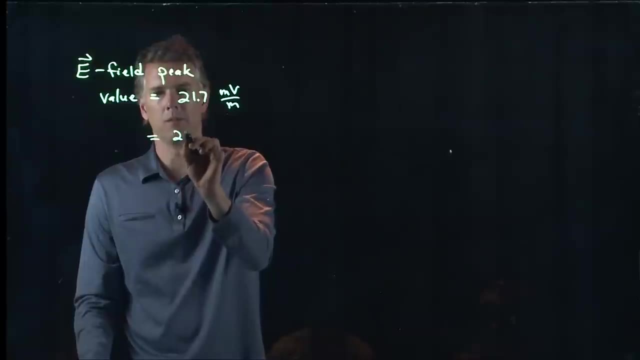 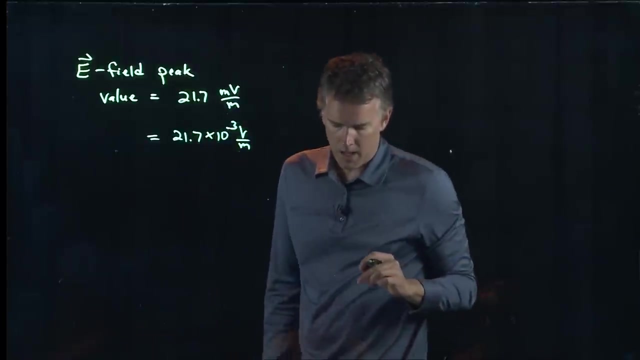 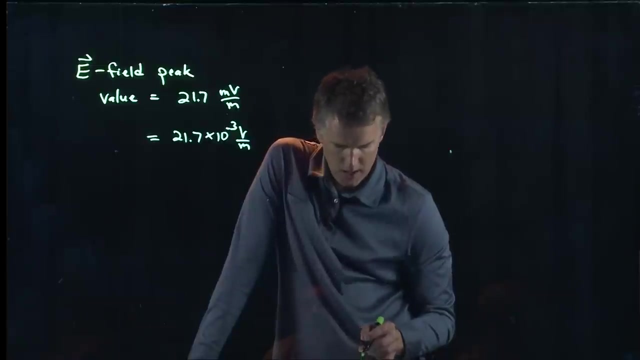 of the following: 21.7 millivolts per meter. okay, so that's 21.7 times 10 to the minus 3 volts per meter, and it wants to know what is the average rate at which this wave carries energy across unit area per unit time. so we have some. 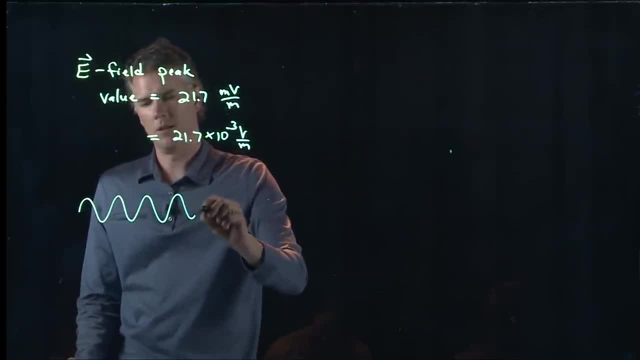 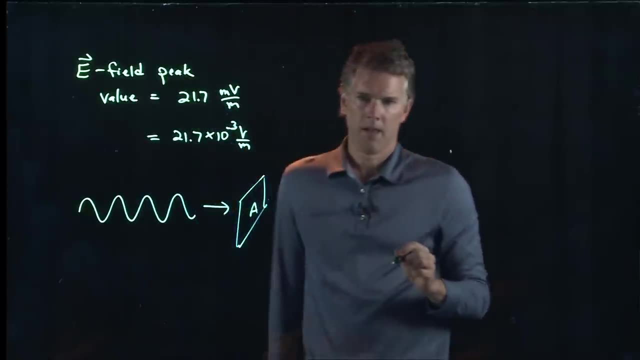 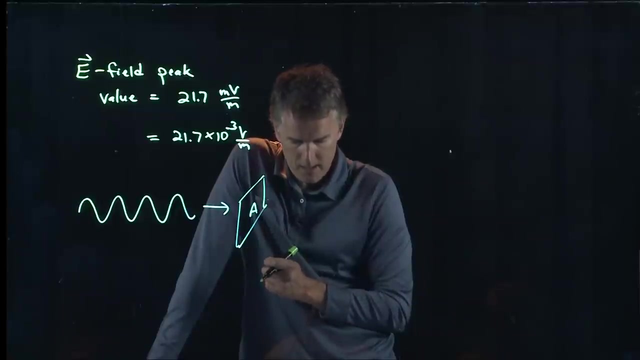 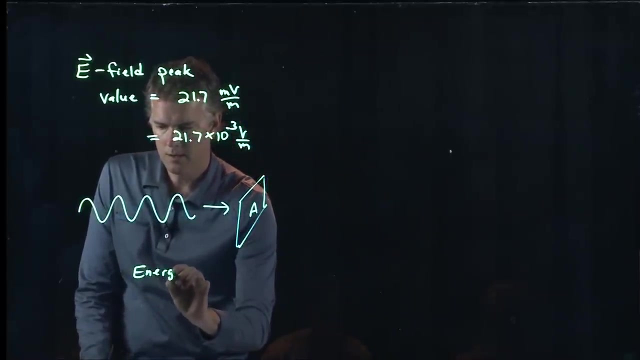 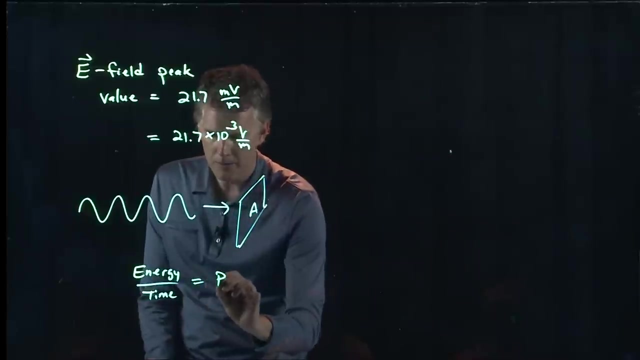 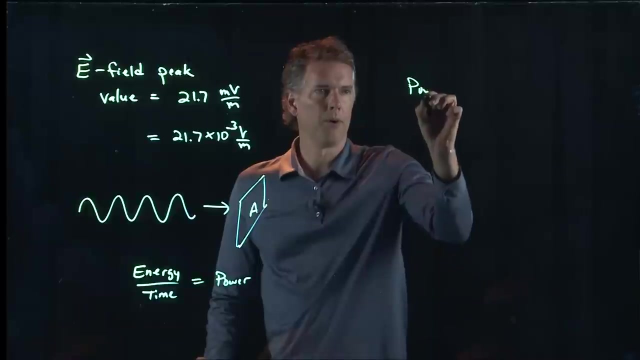 electromagnetic waves coming along and we need to define some area and figure out how much is coming across per unit area, per unit time. now, when we talked about energy per time, remember that was power, and when we talked about power per area, that was what we called intensity. 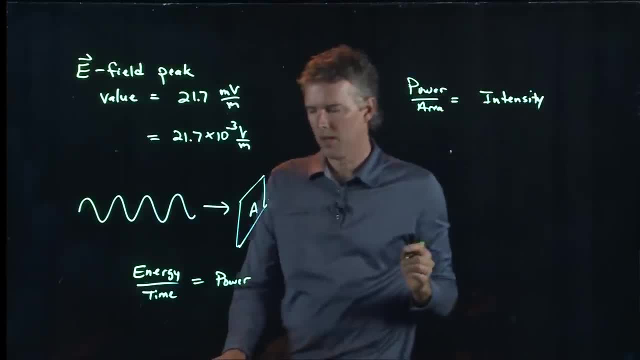 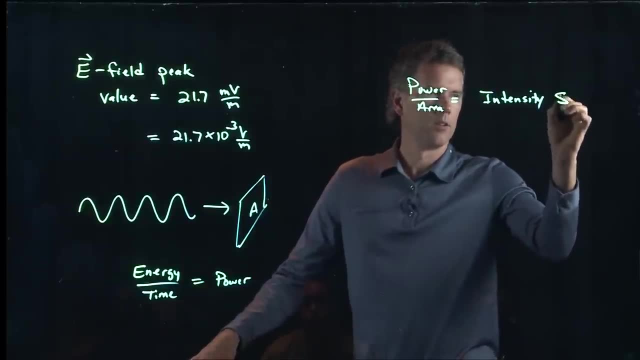 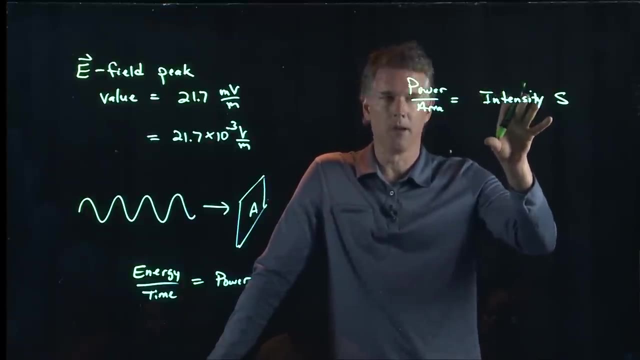 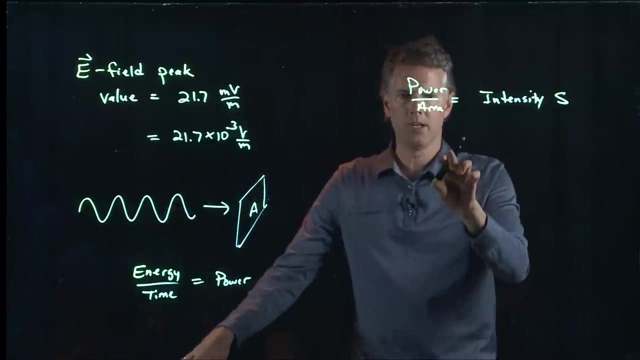 and now yesterday we were using intensity as s. in your book, I think they use intensity as I. All right, so just make sure that you're aware that where we're using S, they were using I. Okay, so it looks like energy per time is power. 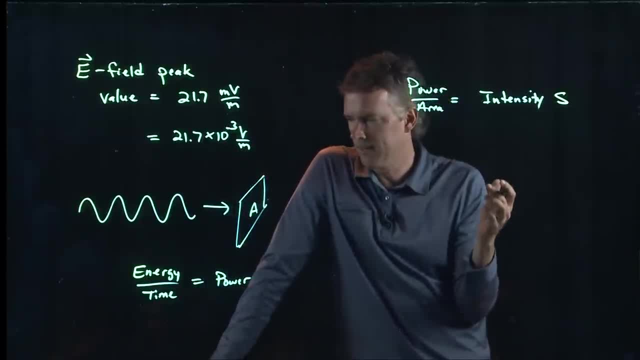 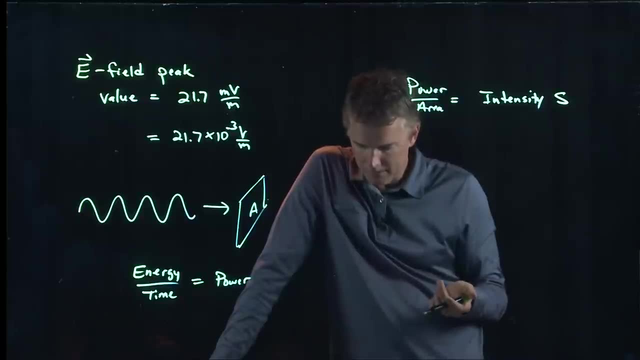 If I divide that by area, I just get intensity, And that's exactly what they're looking for in this problem. Okay, The average rate at which this wave carries energy across unit area per unit time. So we need to figure out what S is equal to. 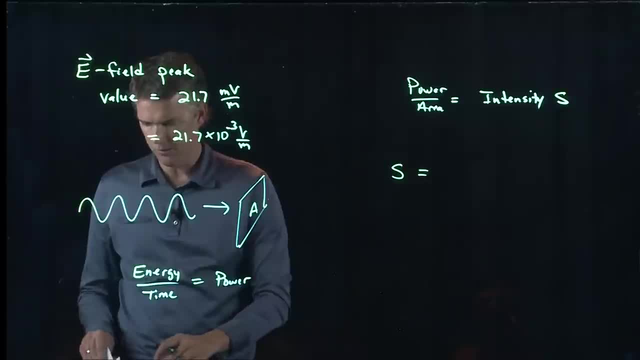 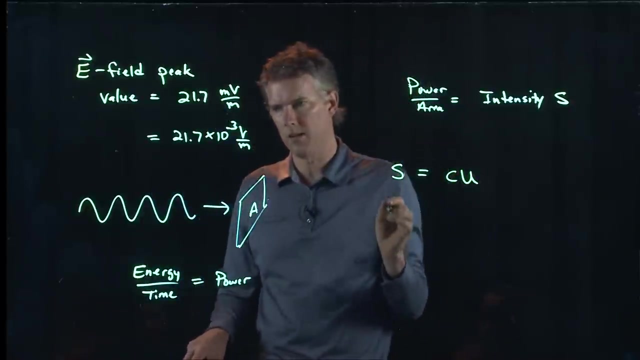 And if we back up a little bit in your notes or you click on the video from yesterday, we can go back to what we were talking about for S. Okay, and what we said was the following: S is, in fact, equal to C times U. C is the speed of light. 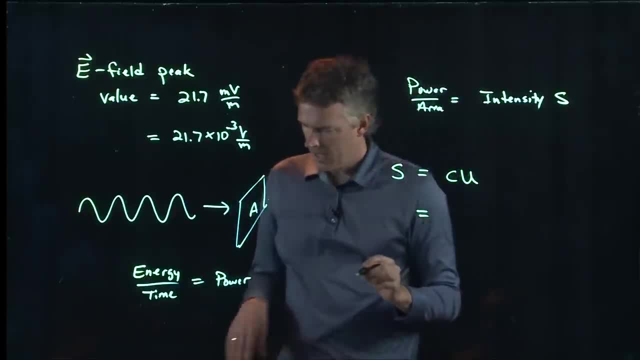 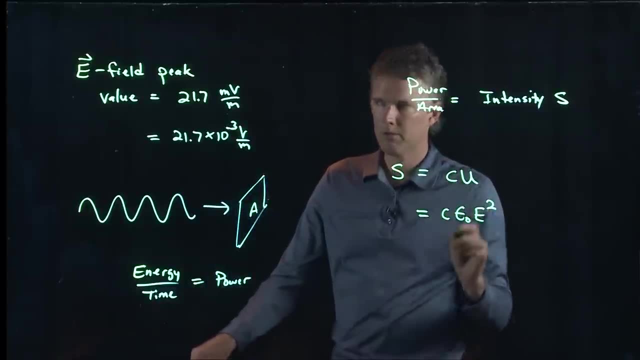 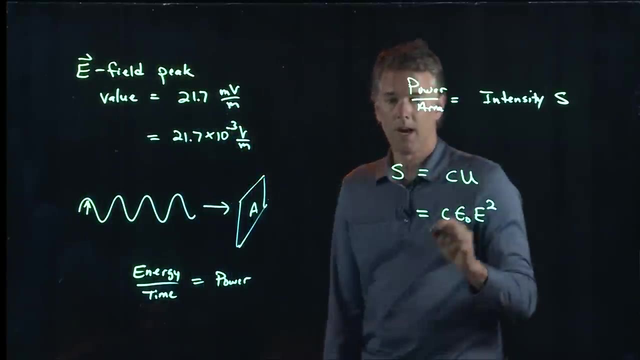 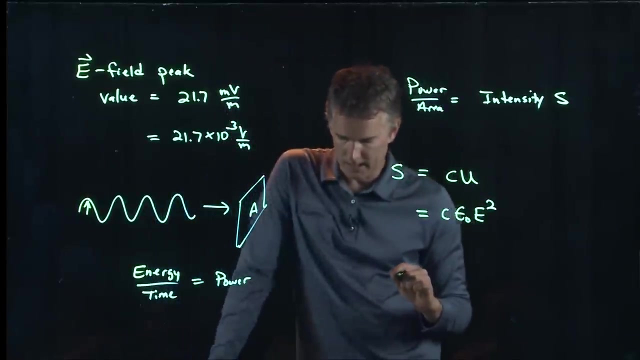 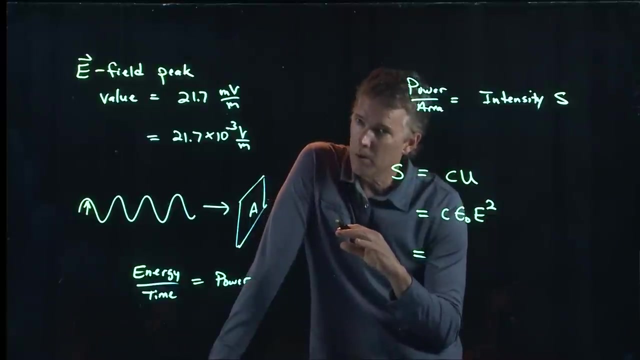 U is the energy density, And that is the same as C times epsilon naught E squared. So if I know E, I can in fact calculate this. Now we got to be perhaps slightly careful about this, because they tell us it's a peak value and so we have to be. 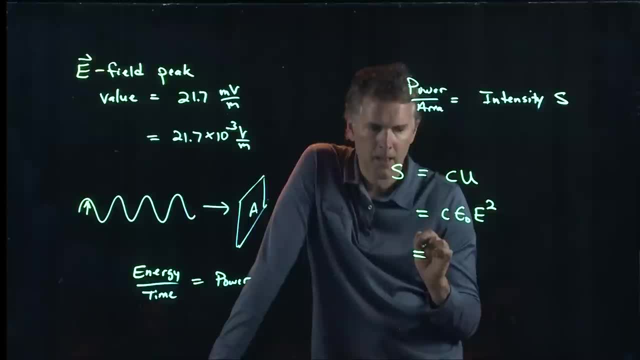 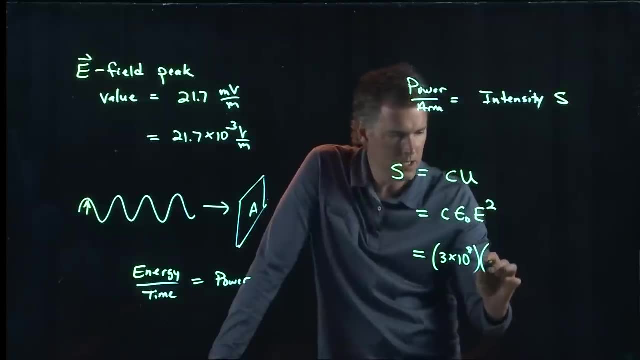 a little bit careful about what we're going to use in here, But let's try it and we'll see if it works out. Okay, so 3 times 10 to the 8th is C. Epsilon naught is 8.85. 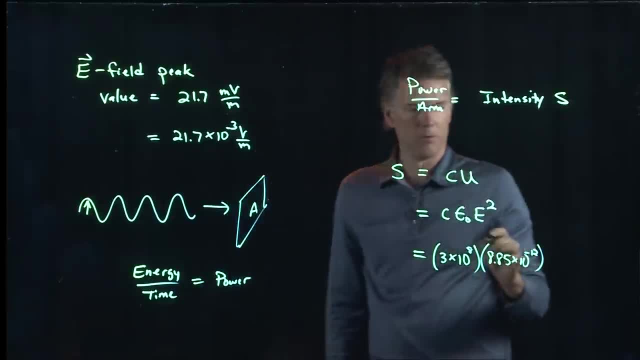 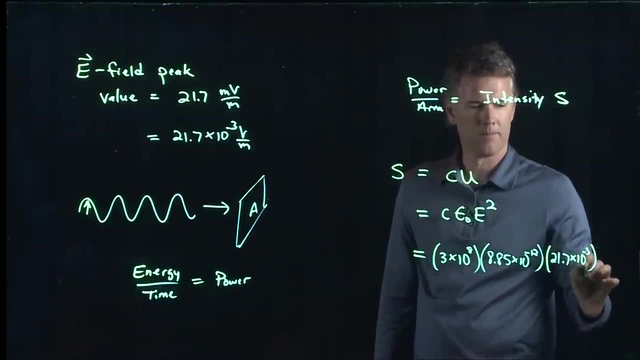 times 10 to the minus 12.. E we just said was this: 21.7 times 10 to the minus 3.. Okay, So that's the first one, So that's the second one, So that's the third one. 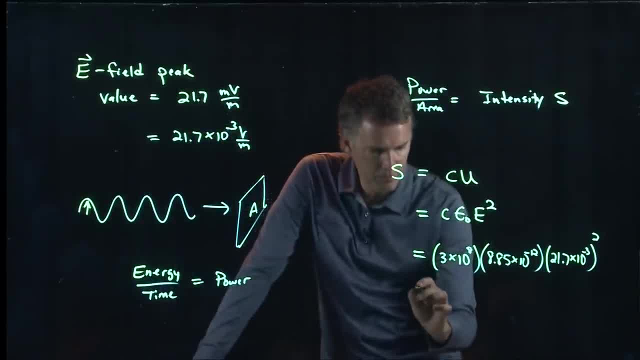 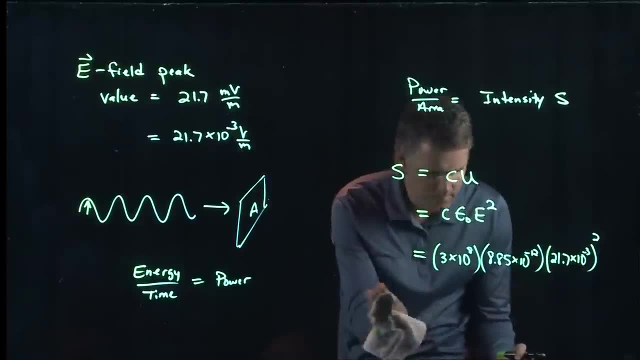 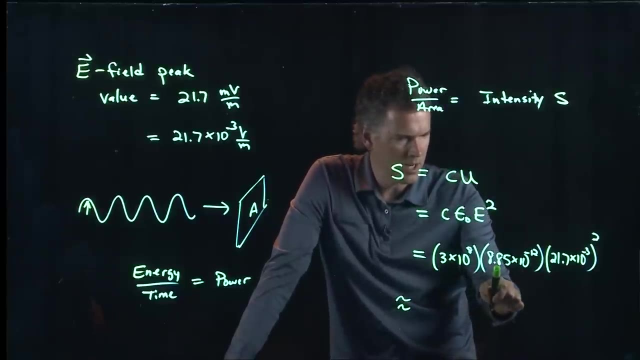 So that's the fourth one. So that's the fifth one. So that's the fifth one. Okay, So if you punch in all those numbers into your calculator, tell me what you get and I will approximate it right here. So we've got a 3 times a 9 times a 20.. 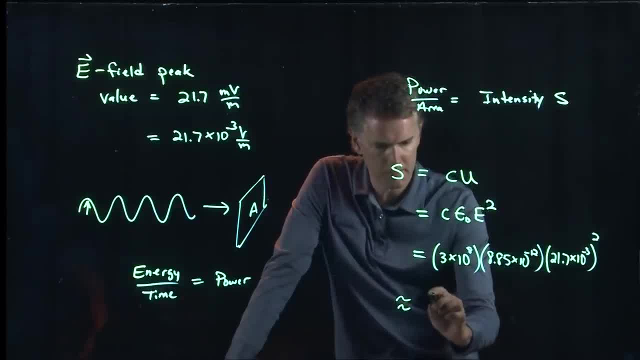 So that's a 60 times a 9.. 60 times 9 is 540.. And then we've got a 10 to the 8th, with a 10 to the minus 12. So that's a 10 to the minus 4.. 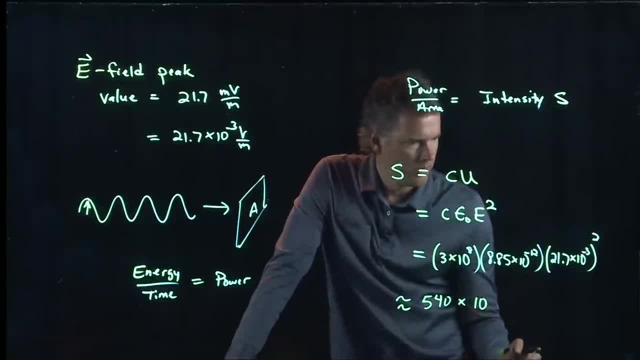 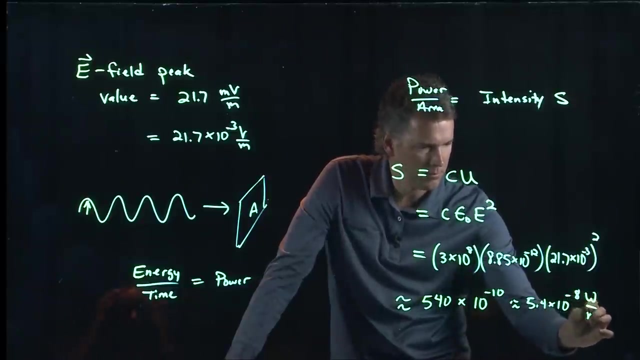 And then we've got a 10 to the minus 6.. So that becomes a 10 to the minus 10.. Okay, So this is 5.4 times 10 to the minus 8.. And the units are SI units. watts per square meter. 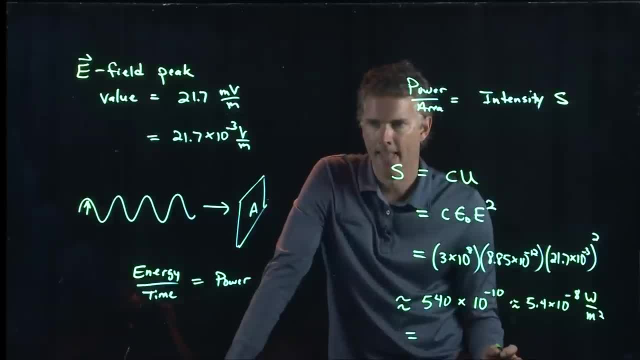 Did anybody punch this into your calculator? Did anybody punch this into your calculator and get a real answer? What did you get? 5.76 times 10 to the negative 5.. 5.76 times 10 to the negative 5?. 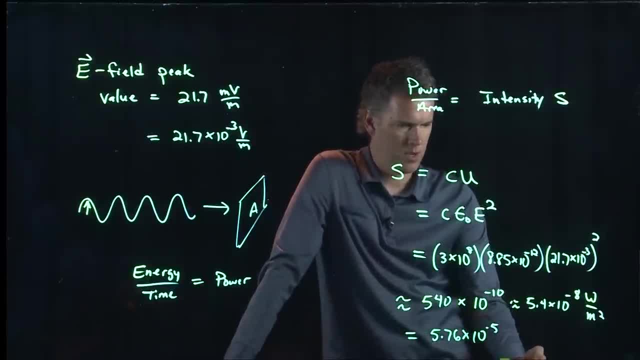 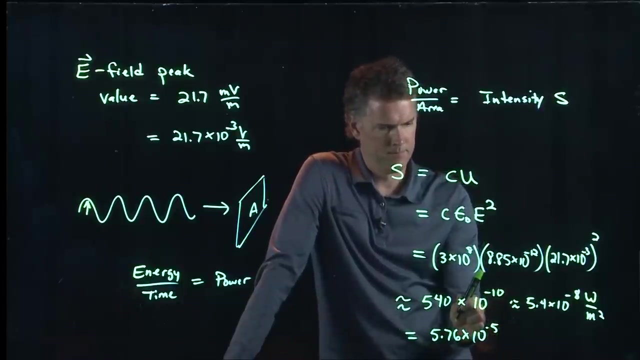 Okay, What did I do wrong? Anybody see where I went wrong here? Can anybody else confirm that number? I got 1.25 times 10 to the negative 6.. You got what? 1.25 times 10 to the negative 6.. 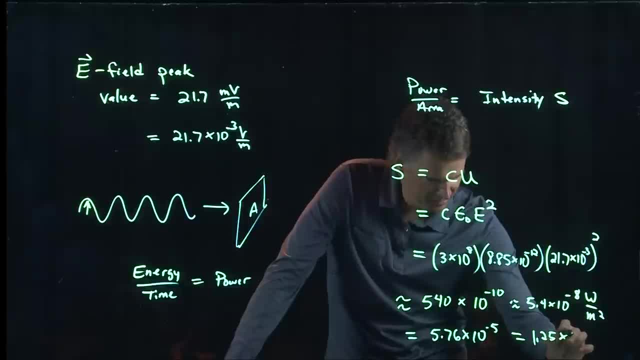 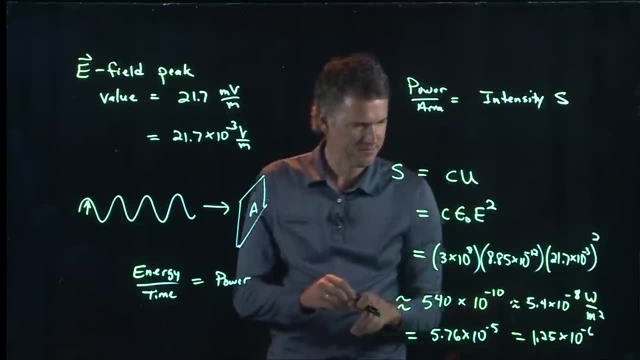 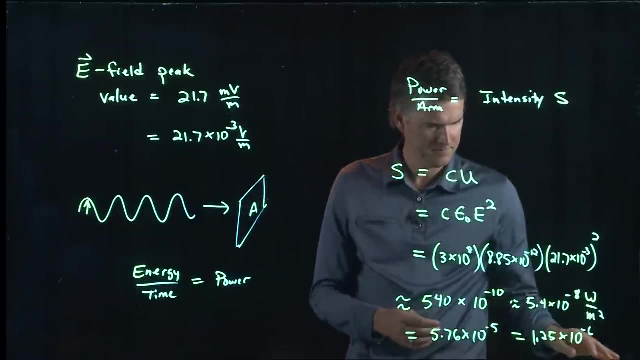 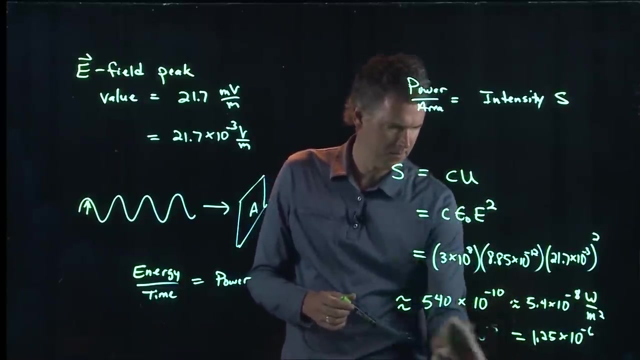 Okay, 1.25 times 10 to the negative 6.. All right, We've got three different answers so far. Should we get some more? This one's right. This one's right, Okay, So we'll erase that one. 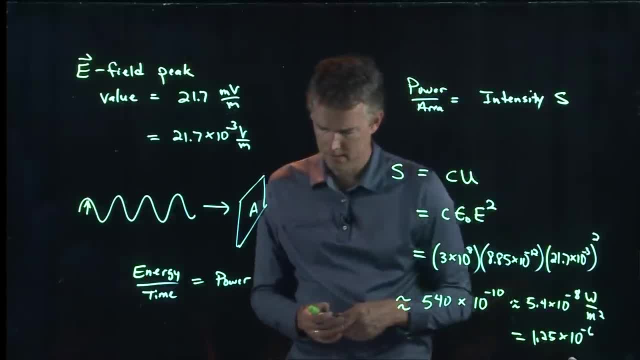 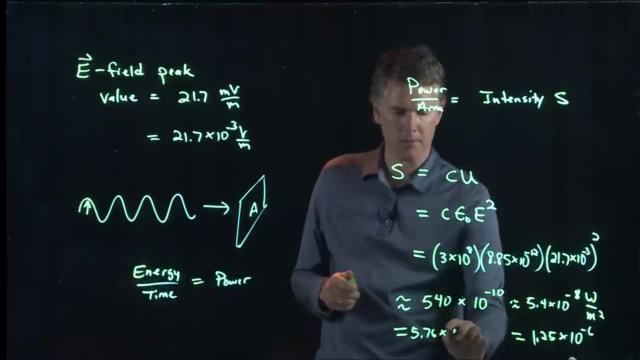 Is that one confirmed by anybody? Okay, 5.76 times 10 to the negative 8.. 5.76 times 10 to the negative 8?? All right, I'll tell you what we'll do. Why don't 1.25 times 10 to the negative 6?? 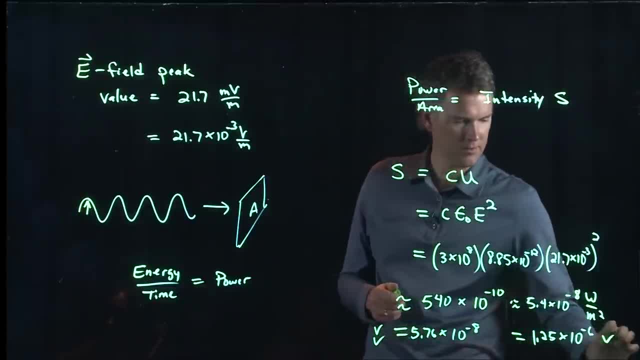 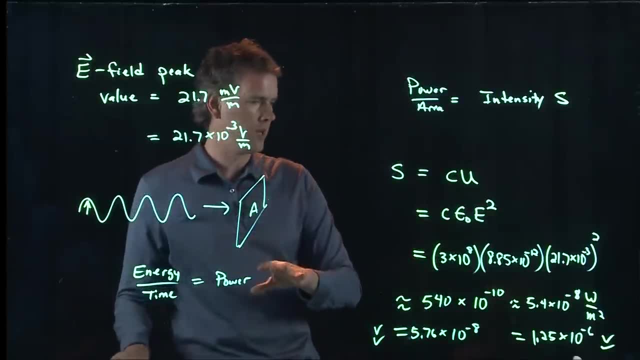 All right, We've got two votes here, Check, check. We've got two votes here, Check, check. Why don't we do this? We'll take a five-minute break, Okay, We'll work this out, And then we'll come back here and tell you what the answer is. 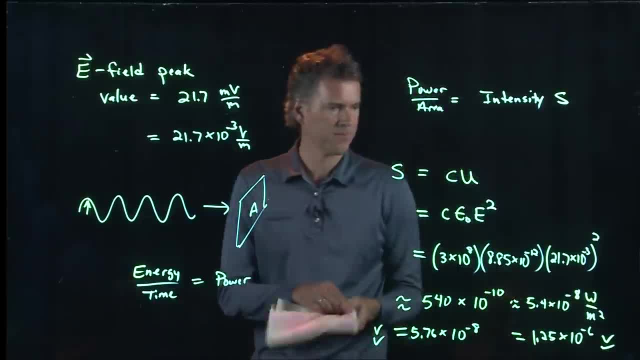 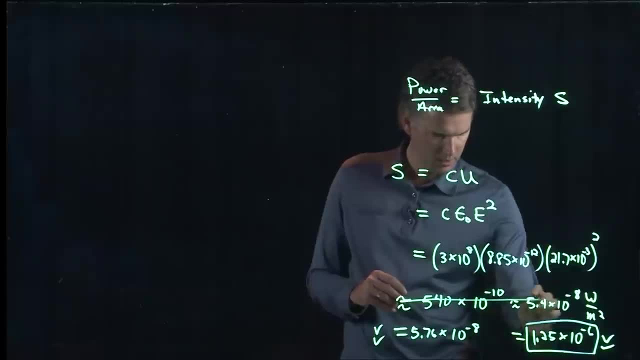 All right. So, Joe, why don't you take us out for five minutes? okay, All right, Welcome back. We figured out where we went wrong. My approximation was no good because we forgot to square the 20.. Okay, So that was no good. 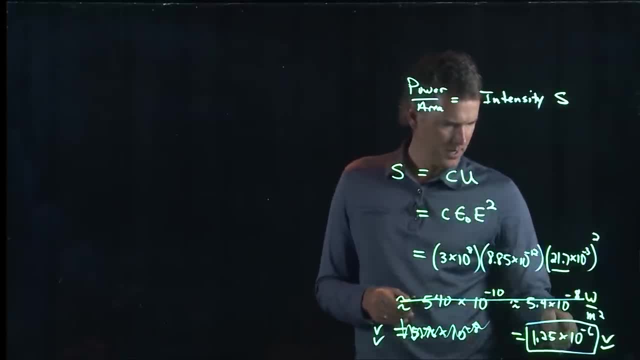 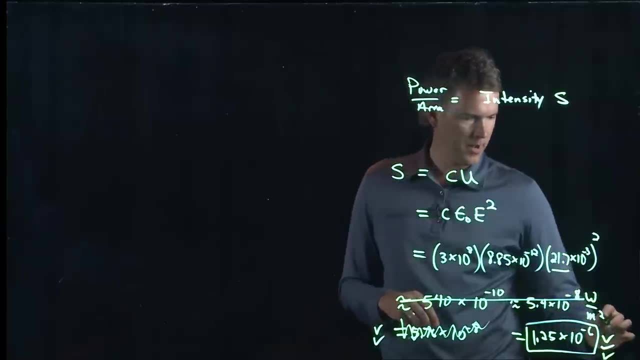 And in fact I disagree with that answer right there. So somebody chimed in from home and confirmed that that is indeed what they got as well, And I just chimed in. I just checked on Wolfram Alpha. If you guys have never used Wolfram Alpha, it's a great website. 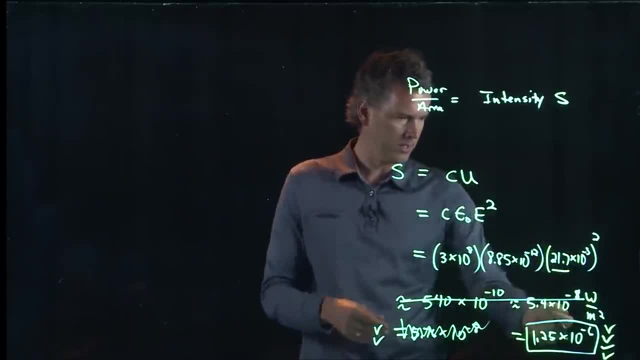 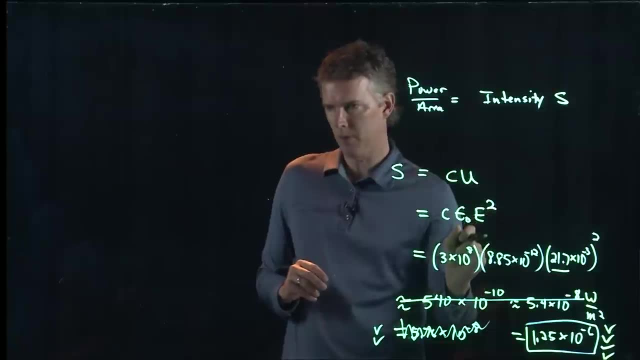 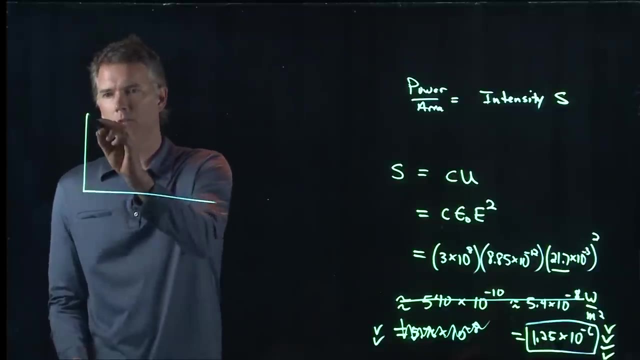 Just go to Wolfram Alpha and you can type in whatever you want. So I just typed in this and it told me that. Okay, So this is the value of C. epsilon naught E squared. But we have to be a little bit careful, because when we think about E squared, what's it going to look like? 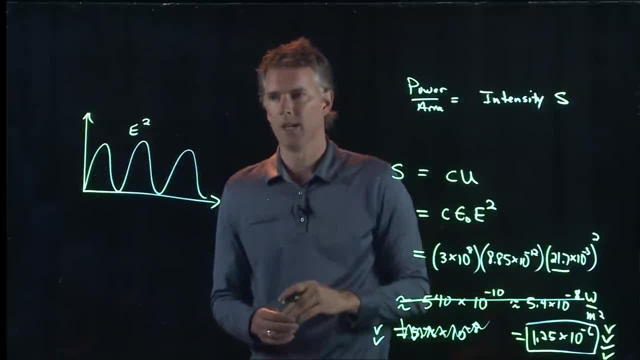 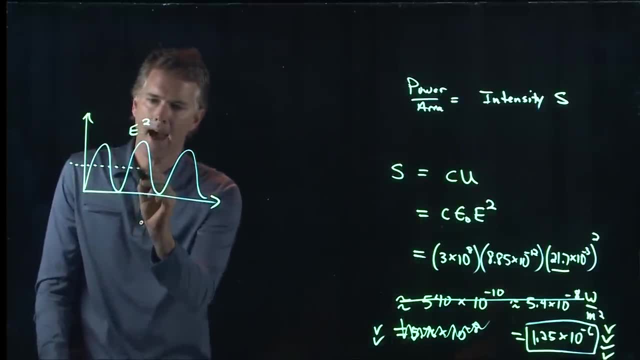 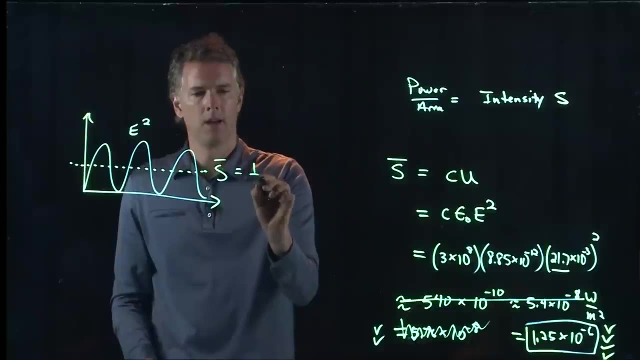 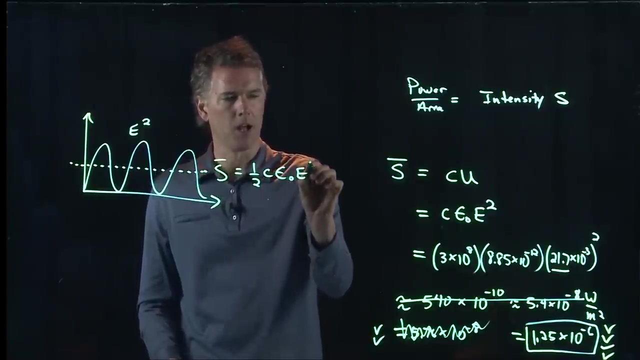 in fact going to look like that. right, It's a positive number, It's going to go up this high, And so when we are calculating the average S bar, we need to calculate a half of the maximum. So it's going to be one half C epsilon E squared. if this was the maximum value. okay. 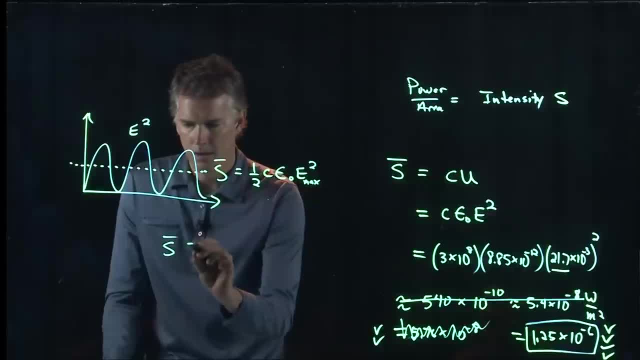 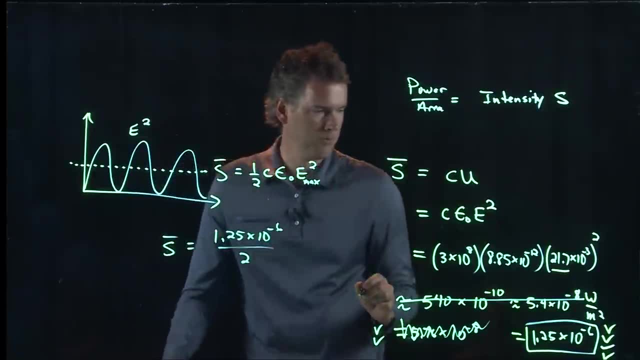 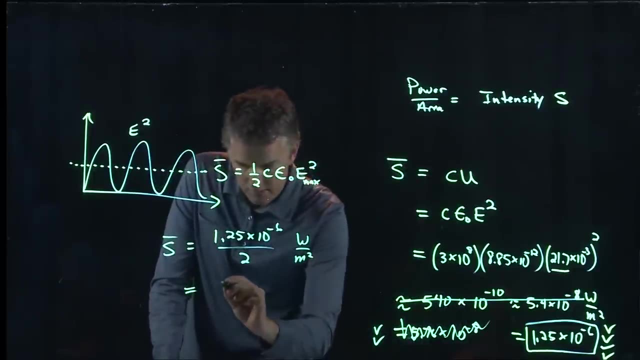 which is what we put in there. So what's the answer to our question? It is going to be 1.25 times 10 to the minus 6, divided by 2 watts per square meter, And if you divide that by 2, you should get 6.25 times 10 to the minus 7.. Okay, and I plugged that in on. 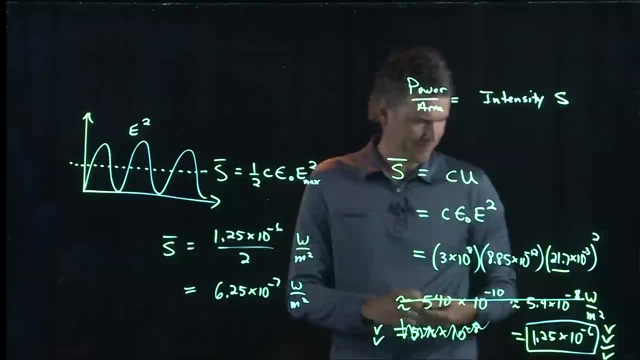 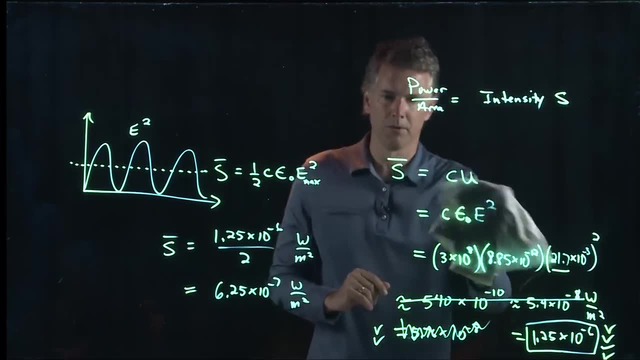 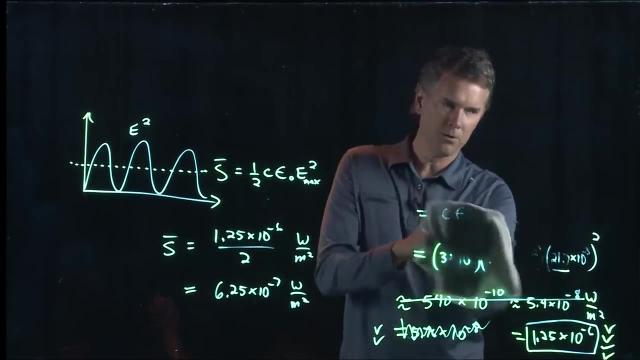 my mastering and it told me I was indeed correct. All right, I like this physics by democracy approach that we're taking here. This is good. I should take advantage of you guys more often. I got all these brains in the room- these. 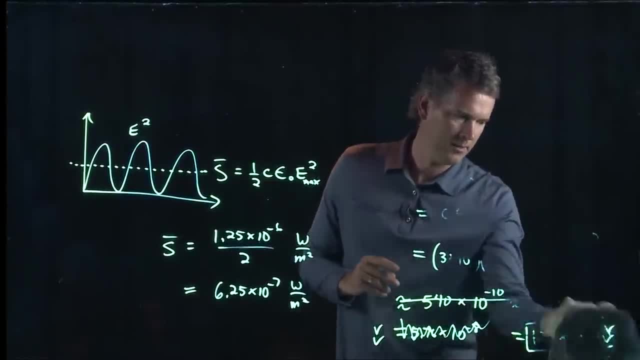 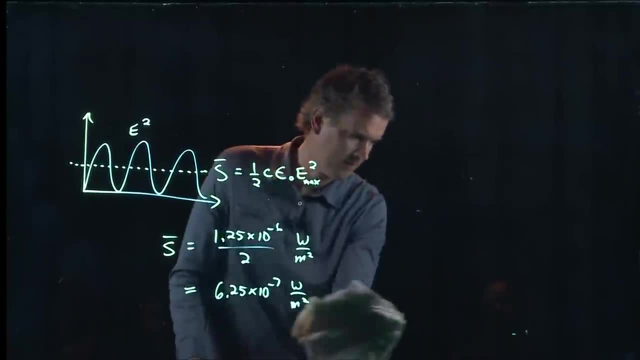 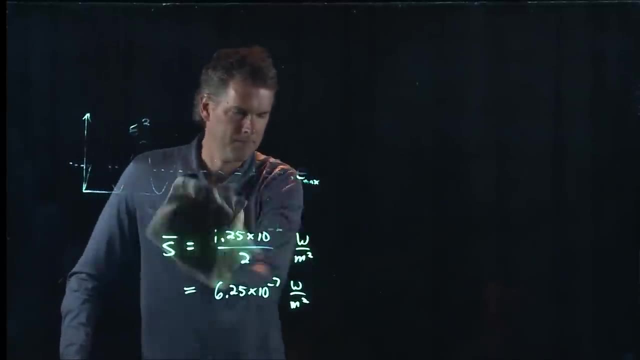 brains at home. all sorts of calculators everywhere Got to take advantage of that, Okay, and I'm going to take advantage of you guys more often. I got all these brains in this environment. Do you have questions about that problem? Are they any questions about that problem? 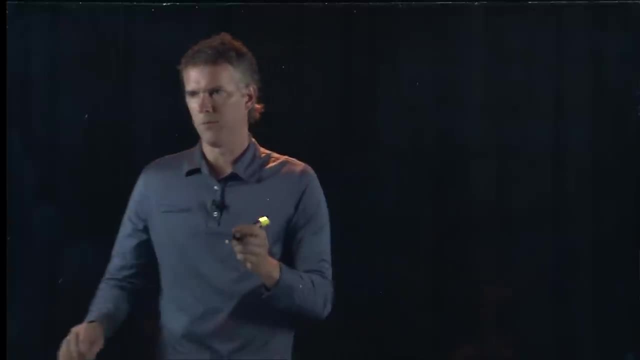 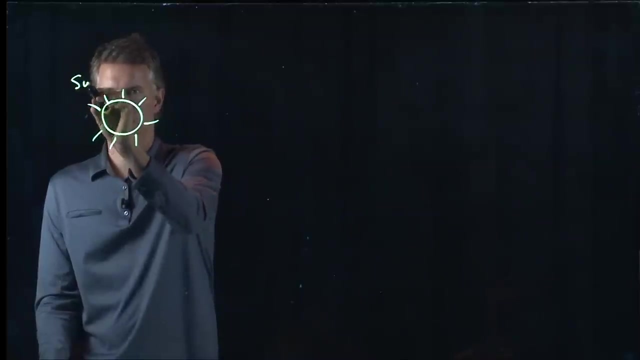 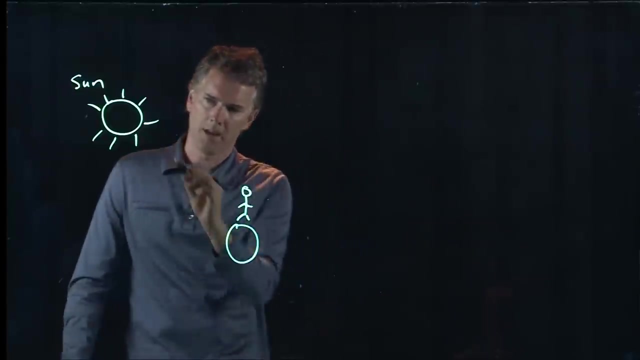 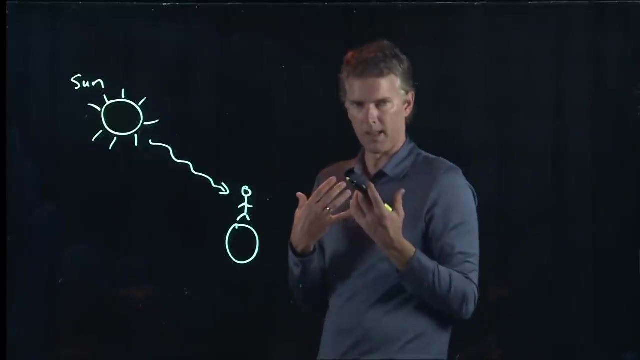 All right, Let's talk about something else. Here's the sun. Okay, Here you are, standing on the Earth. Subtitles by the Amaraorg community is going to come and hit you right. You're outside, you're absorbing sunlight. 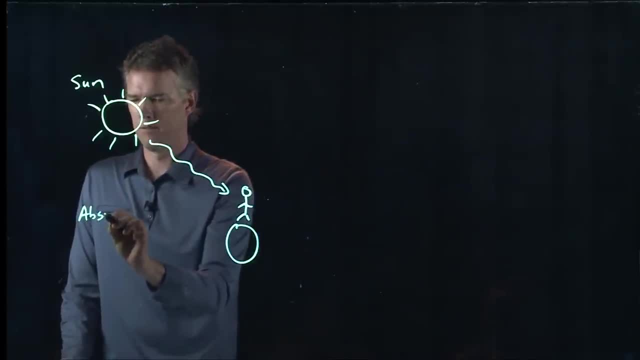 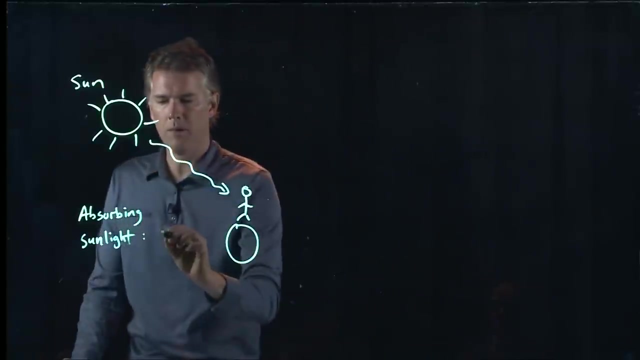 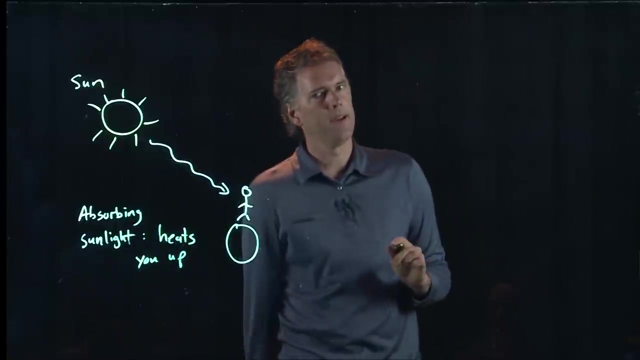 When you absorb sunlight, what happens to you? You guys have all done this experiment. You sit out in the sun. What happens? You get hot, right, You get warm. It heats you up. But let's ask a follow-up question. 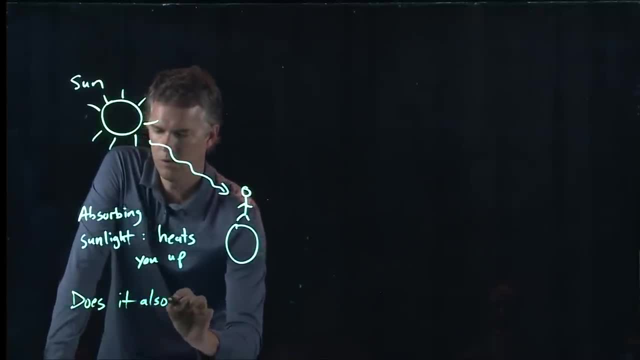 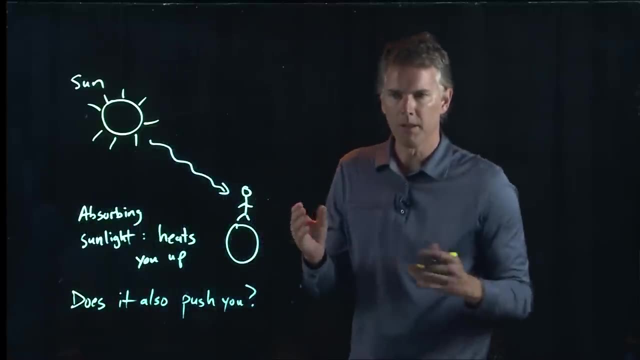 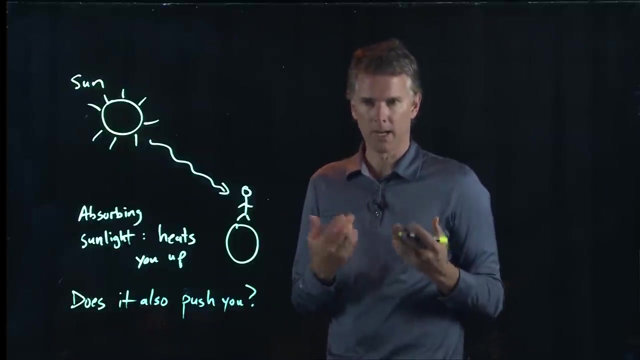 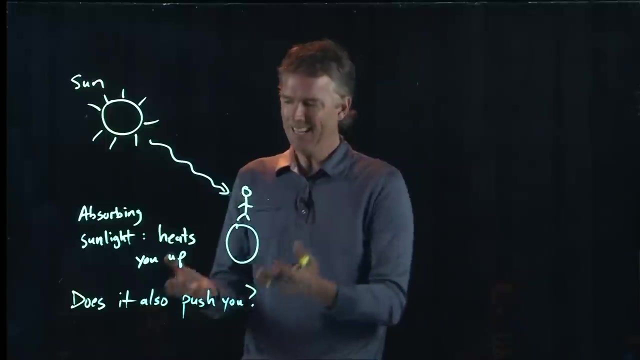 Does it also push you? We know it heats you up, but does it also push on you? Well, it doesn't seem like it. I go out in the sunshine. I don't get pushed over by the sunshine, right, But in fact it is pushing on you. 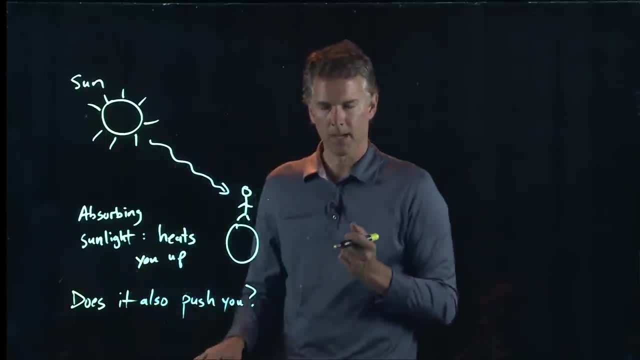 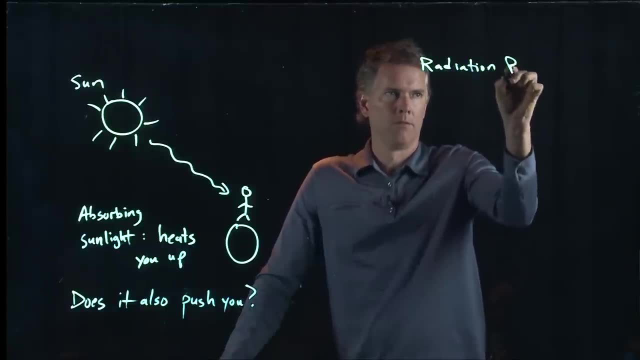 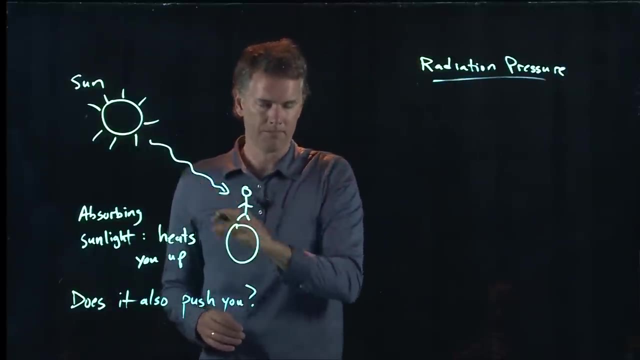 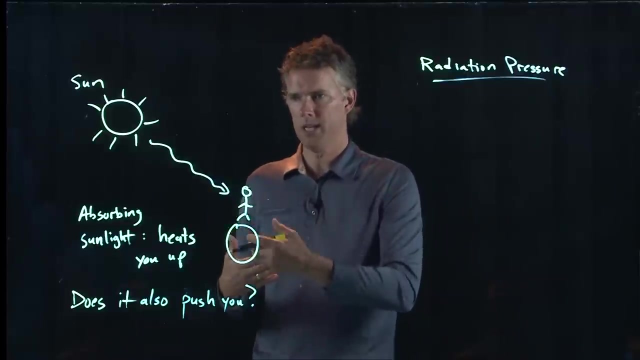 Not very much, but a little bit. And so there's this idea which we call radiation pressure. Radiation just refers to electromagnetic waves, And those waves, when they hit something, not only do they transfer energy to it and heat it up, but they also push on it. 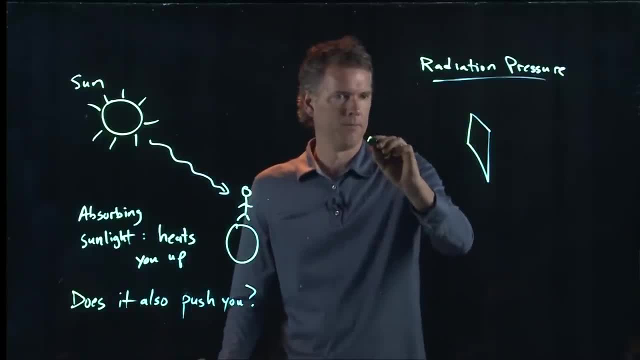 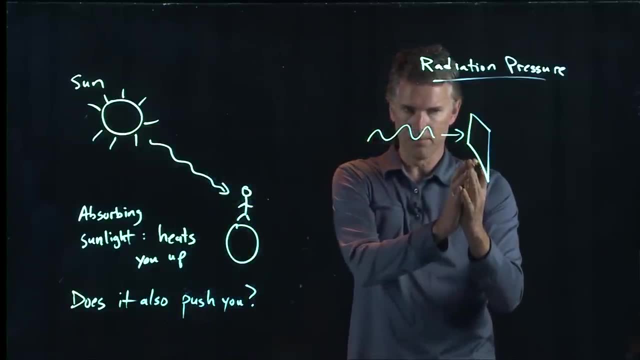 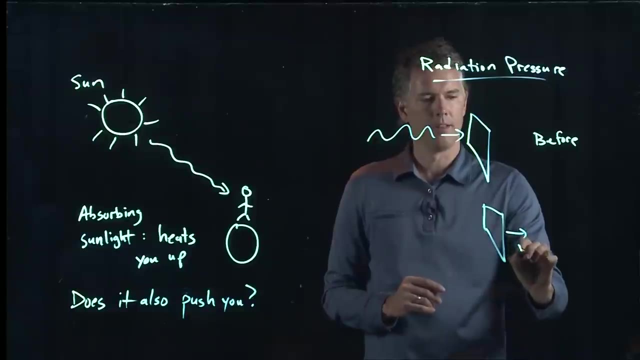 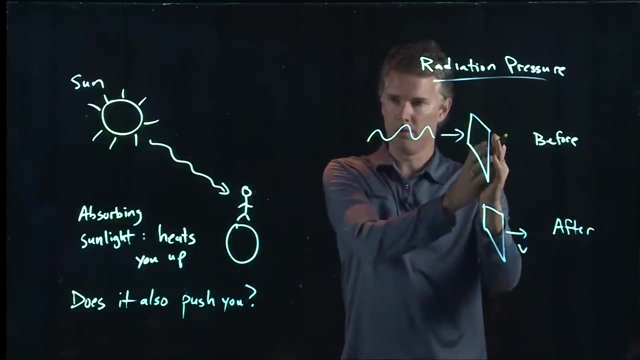 So if I think about an absorber and here comes a wave and it hits the absorber and it gets absorbed in the material, if this is the before picture, then after this thing starts moving, The wave is gone, It got absorbed. 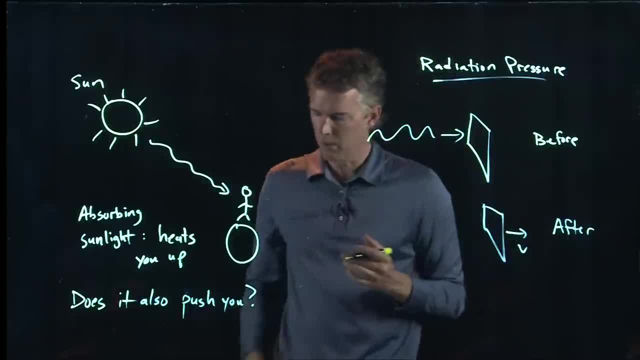 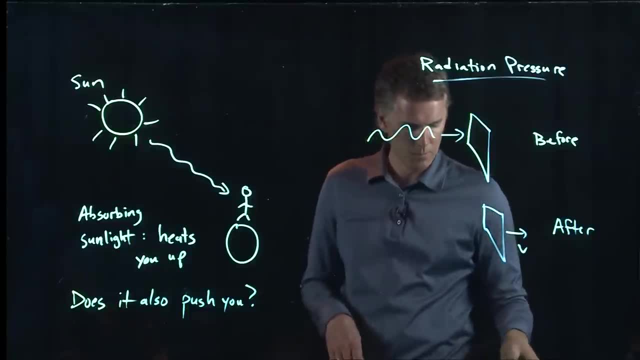 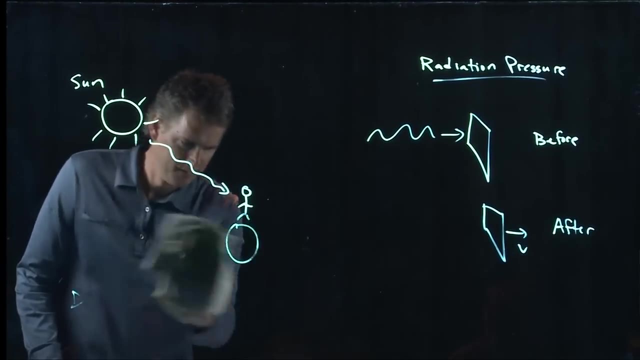 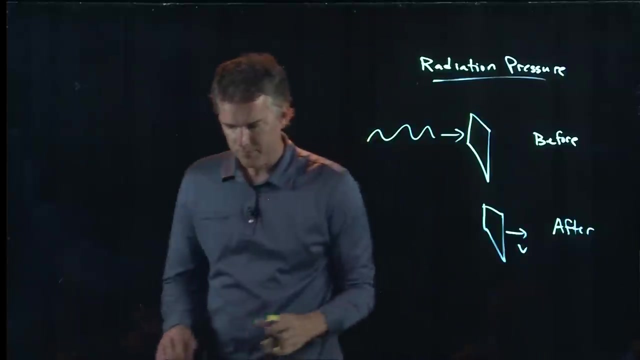 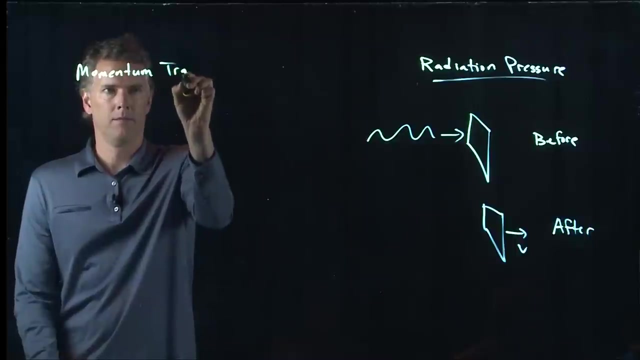 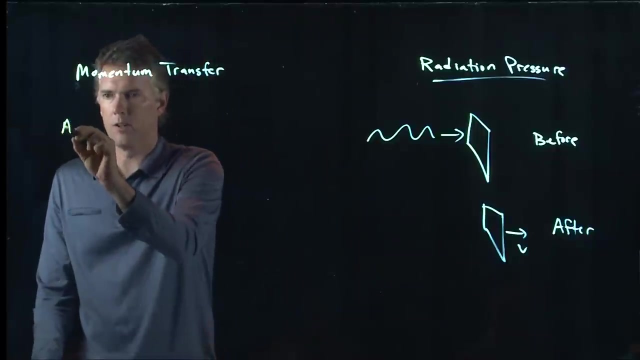 The object now is moving, It gets pushed away, So there is a momentum transfer between these two And we need to understand exactly how that works. So for an absorber, the momentum transfer from the wave to the absorber looks like the following: 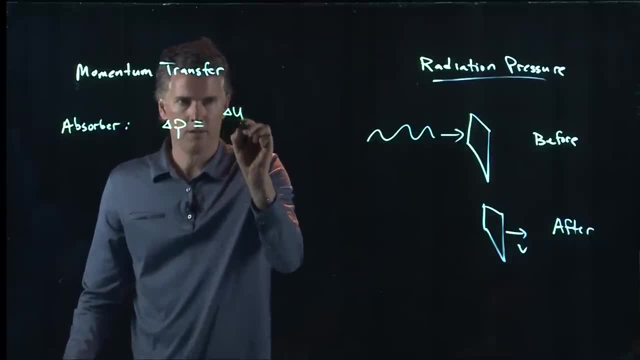 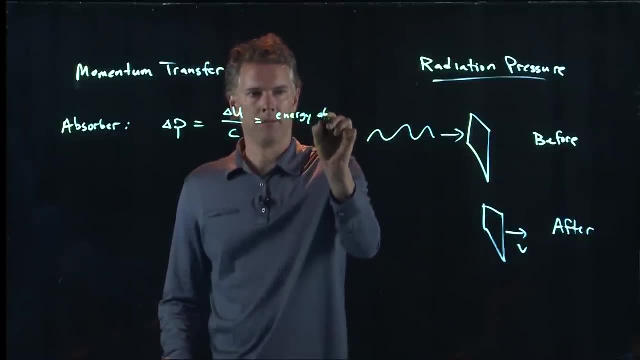 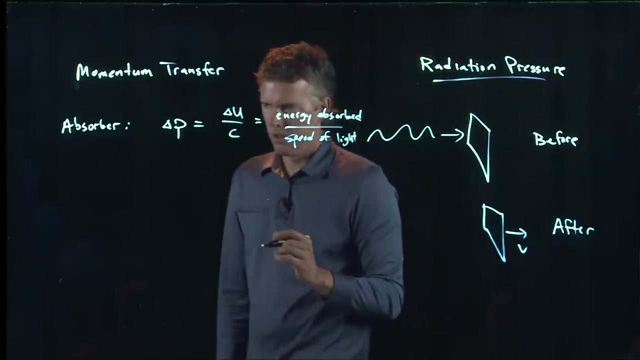 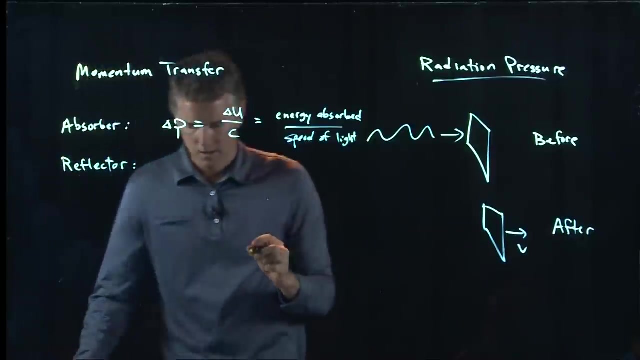 Delta P is delta U over C. How much energy was absorbed Divided by how fast it was going- Speed of light- And this is the delta P that is picked up by that absorber. If it's reflected, then that wave doesn't just get absorbed in the material. 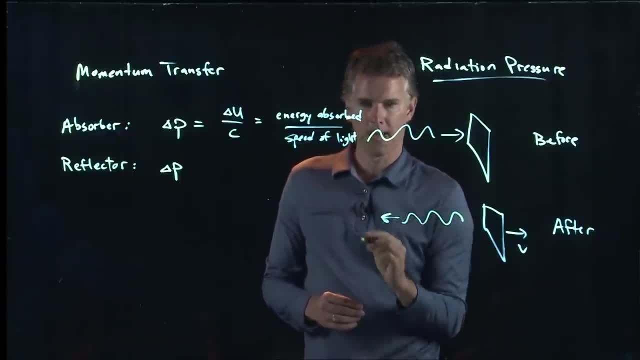 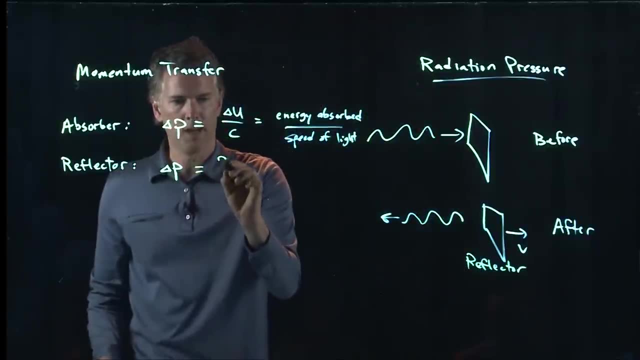 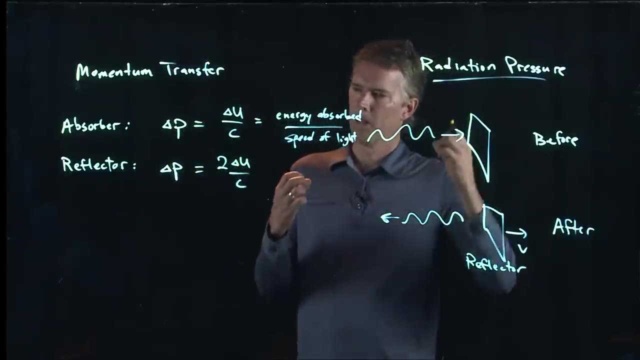 it actually bounces off and goes back the way it came. And if it's a reflector now the delta P is twice what it is in the absorbing case. This is kind of like when we talked about throwing the Superball at the wall. 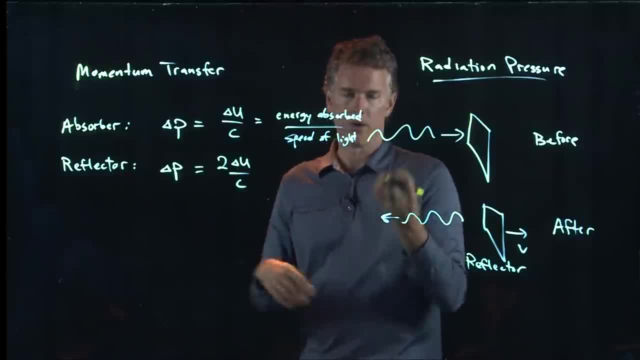 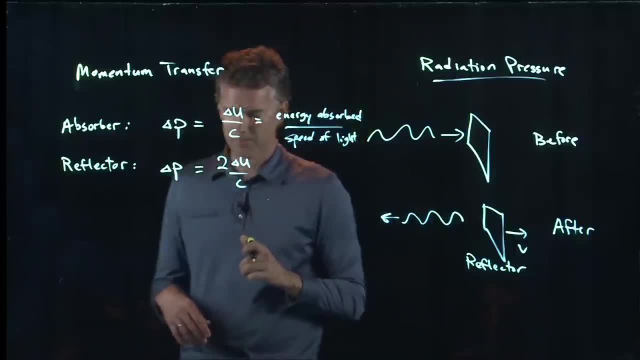 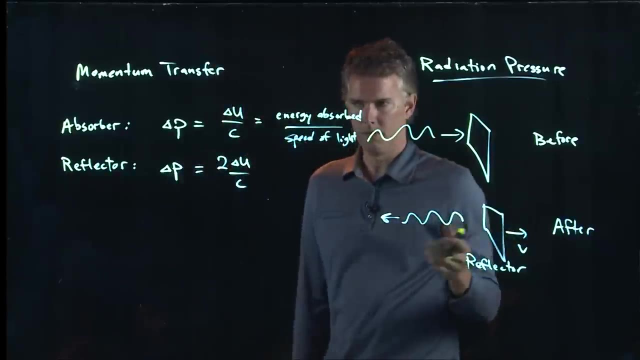 It transfers twice its momentum to the wall, Whereas when you throw the sticky wad of clay at the wall it just transfers one of its MV to the wall. Okay, But if we have a delta P here, we have some change in the momentum. 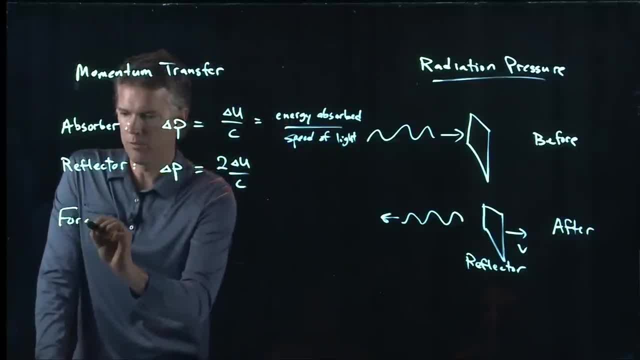 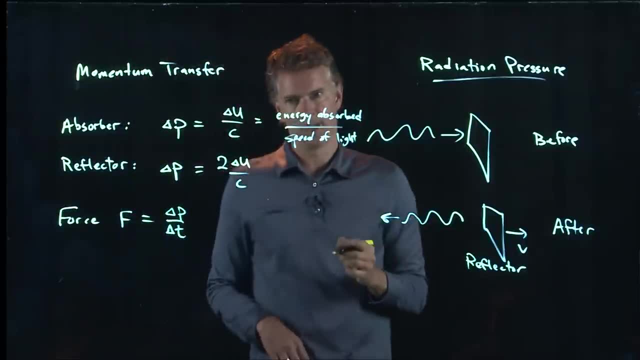 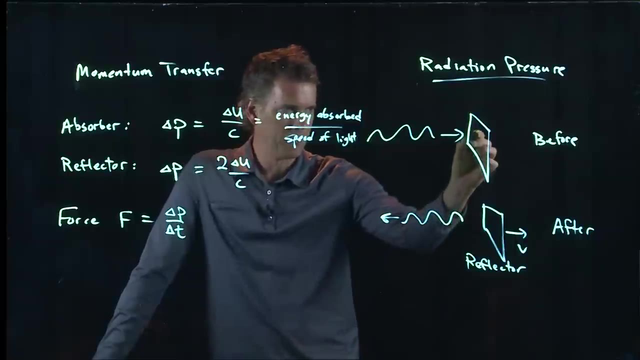 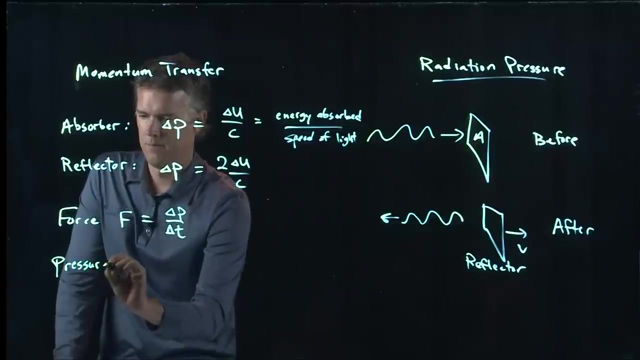 then we have to have a force, because we know that force F is related to momentum. It's delta P over delta T. All right, If I have a force and I have some area, then I have to have a pressure And pressure. 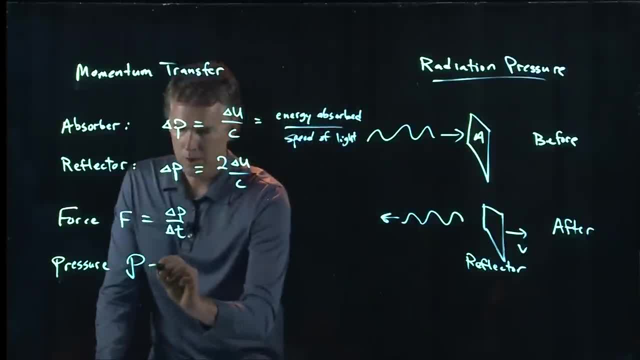 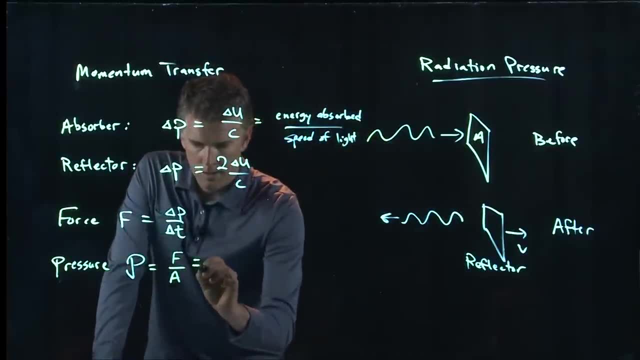 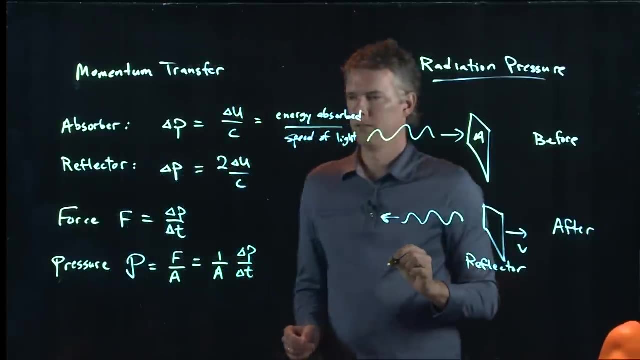 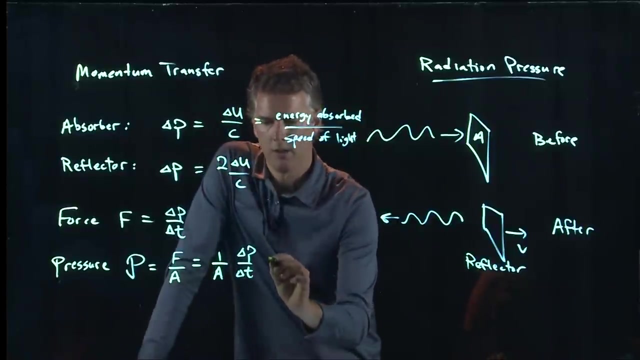 right with this sort of capital P looking thing. pressure is just force divided by area. Force we just said was delta P over delta T. But I know what delta P is. Delta P in the absorber case is just delta U over C. 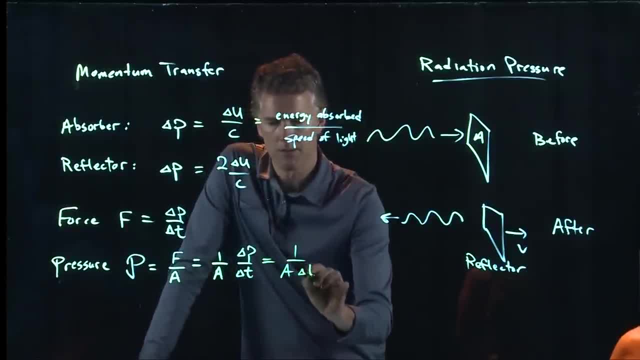 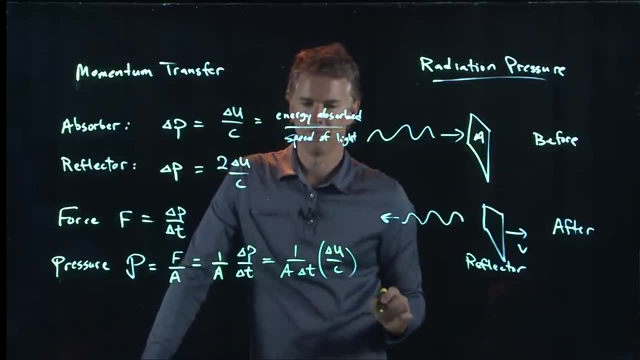 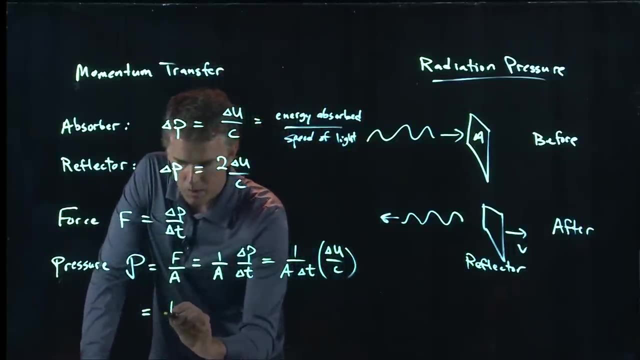 So this becomes one over A delta T. And then I have delta P, which is delta U over C. And now let's rearrange this a little bit And we can write it as the following: One over C times delta U over A delta T. 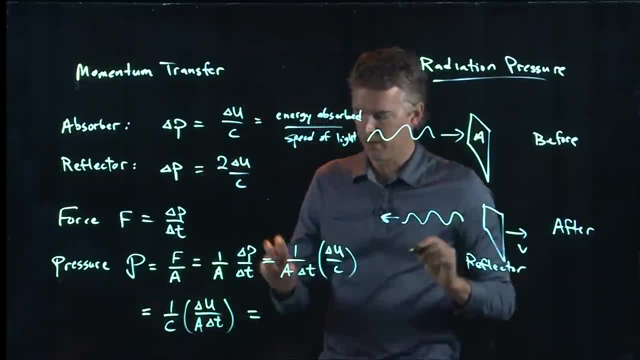 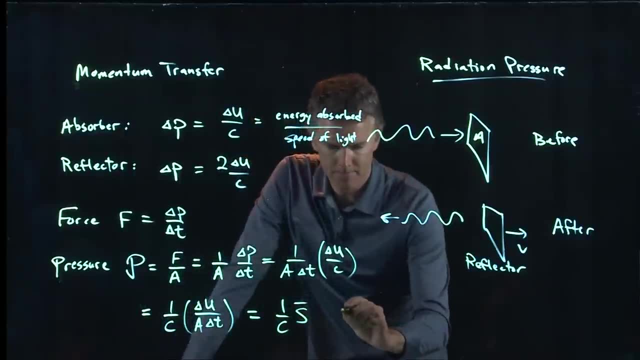 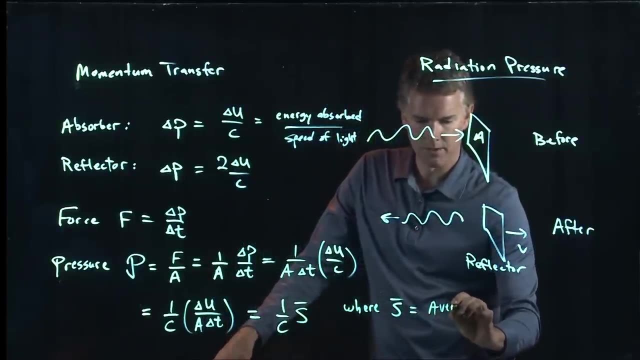 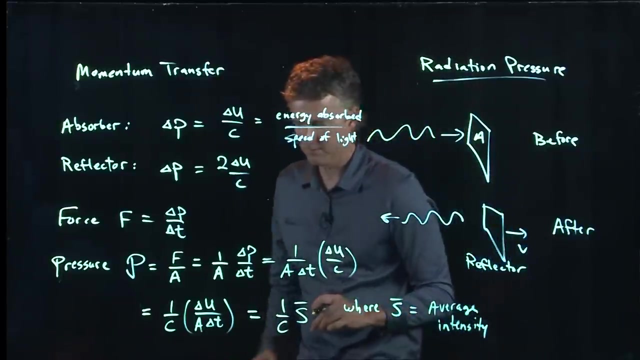 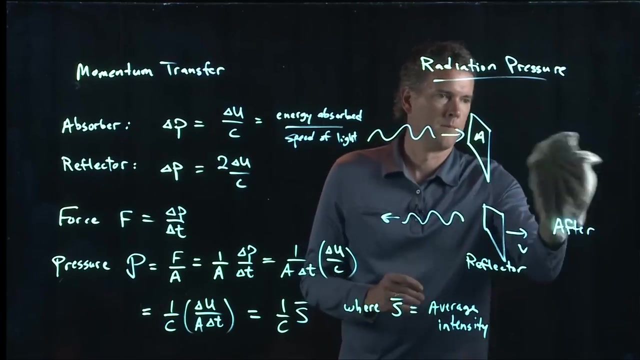 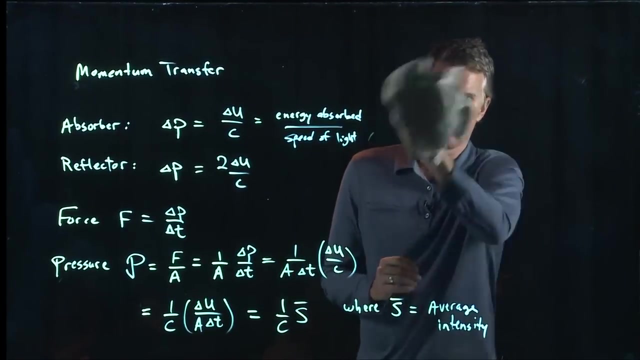 But we know exactly what this stuff is. This is our good old intensity, And so this whole thing simplifies to that Where S bar is our average intensity And then it's equal to: This is our average intensity And we've got the following: 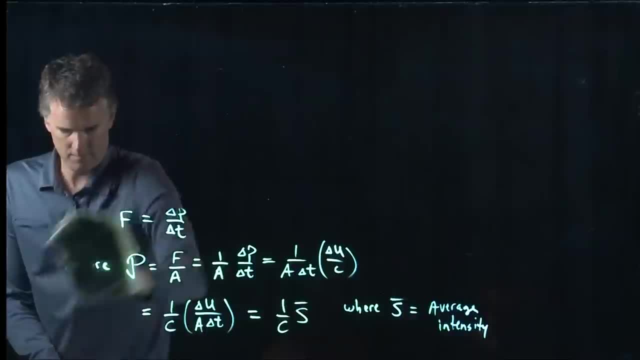 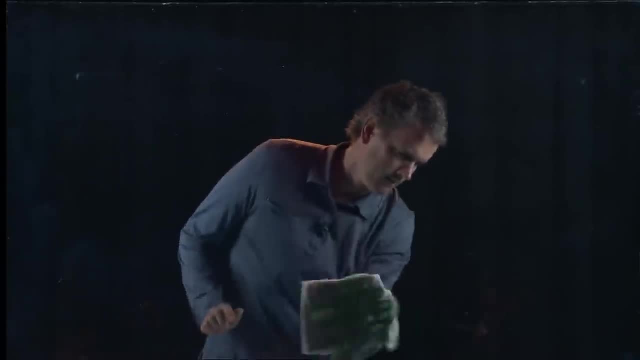 Okay. So when we know this graph is something that's 2 over 2, we've got to get the root of the equation in terms of this part. So what's the right answer? And what's the right answer? All right here. 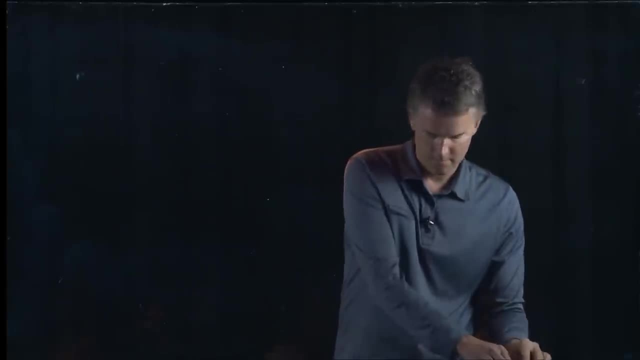 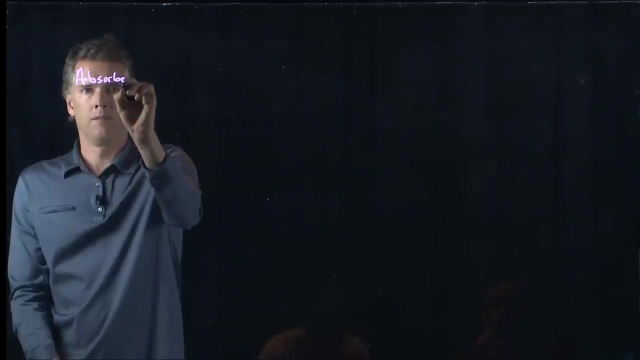 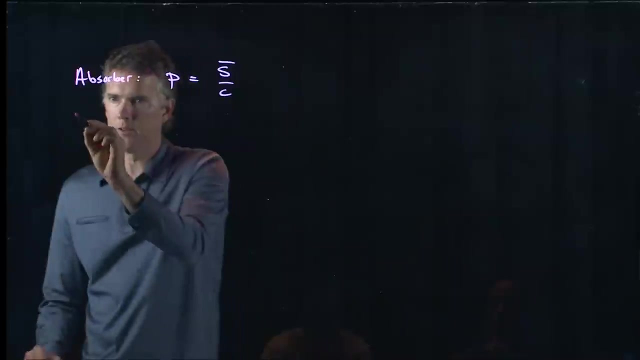 Now let me go back and take a look at this and see where I've got the right answer in terms of what I've got. So let's go back here. For an absorber, P is just S-bar over C. For a reflector- and this is supposed to be capital P right pressure is 2 S-bar over C. 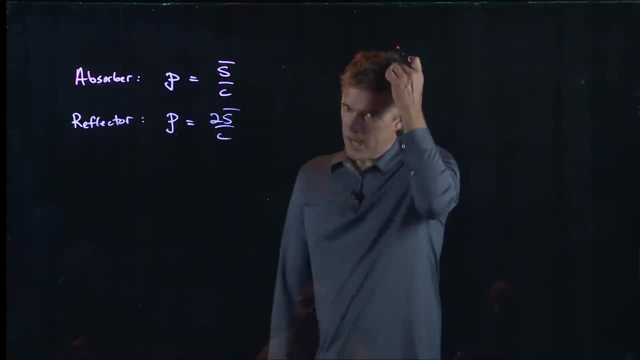 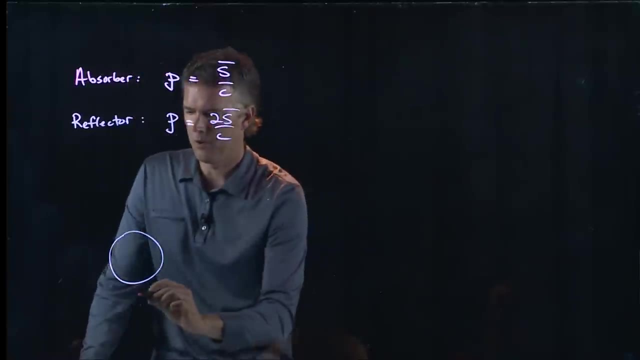 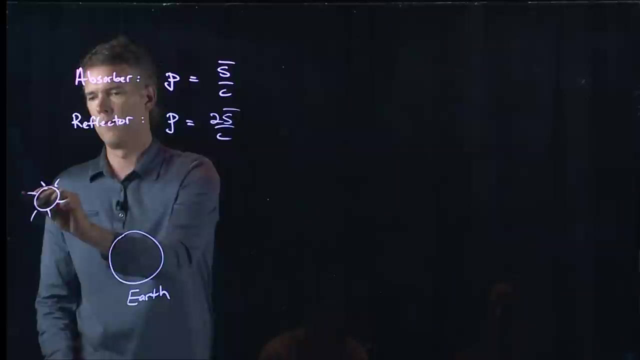 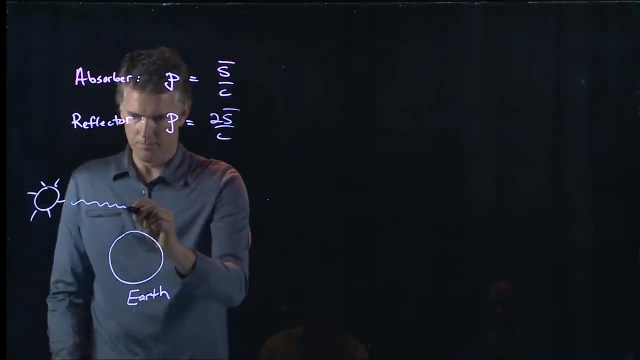 Let's take a look at an example, and this is something that people have actually undertaken. Here's the Earth. Here's the sun. way over here, The sun is spitting out sunlight in all directions. Some of that sunlight is skimming past our atmosphere. 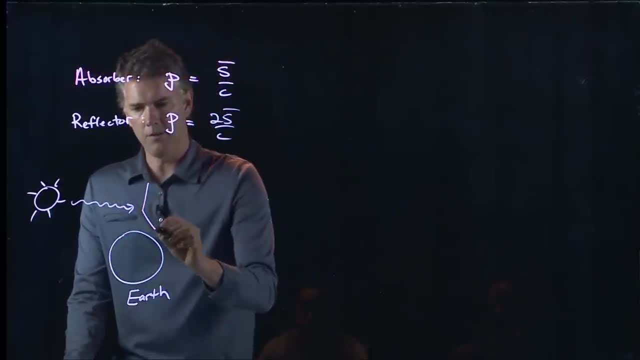 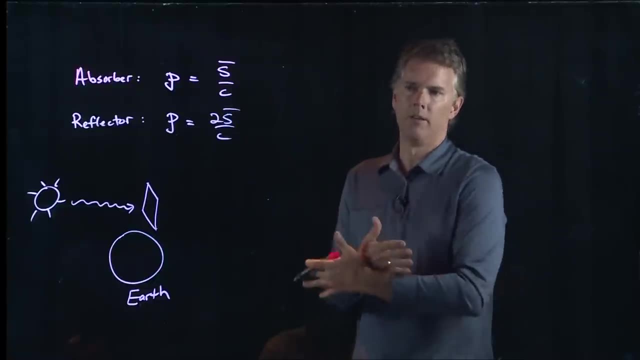 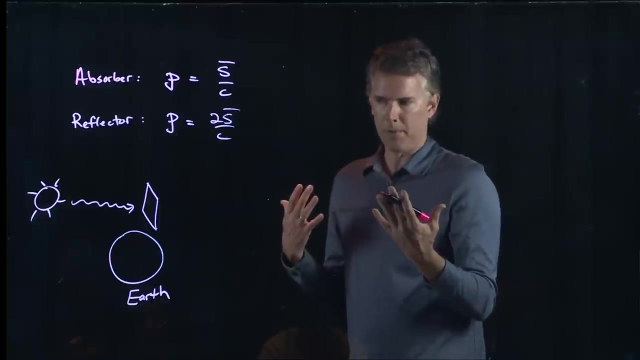 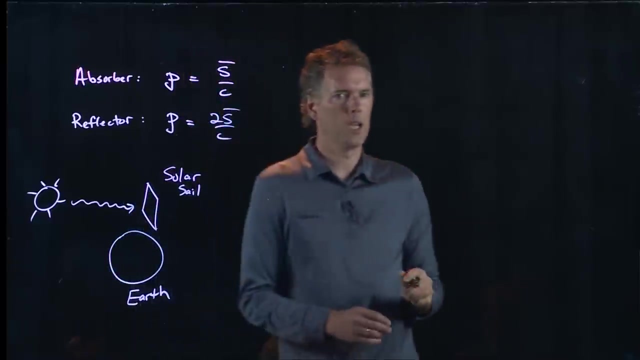 Let's take a spaceship, send it up into outer space and inside that spaceship let's include a sheet of Teflon, foil or mylar that expands when it gets into outer space. This is something called a solar sail. Mylar is like a big reflector. 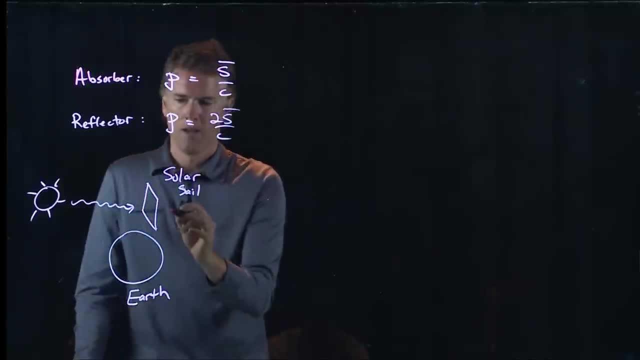 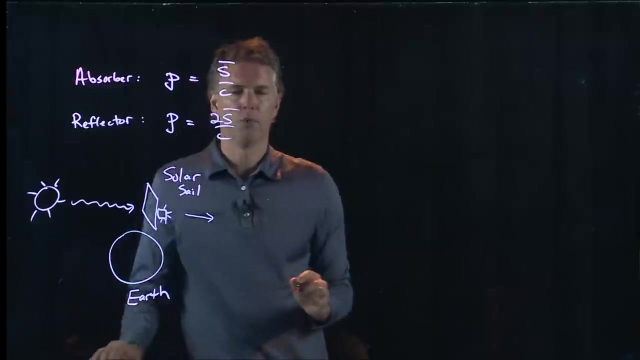 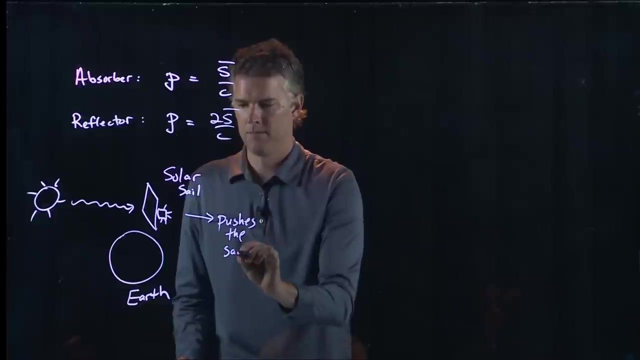 Okay, With that little spaceship. it has a big sail on it and we'll attach it to our little spaceship. put some antennas on it. The sunlight that's going to come in hits the solar sail and pushes the spacecraft. Okay, And this is a real project that humans have undertaken, right, this idea of a solar sail? 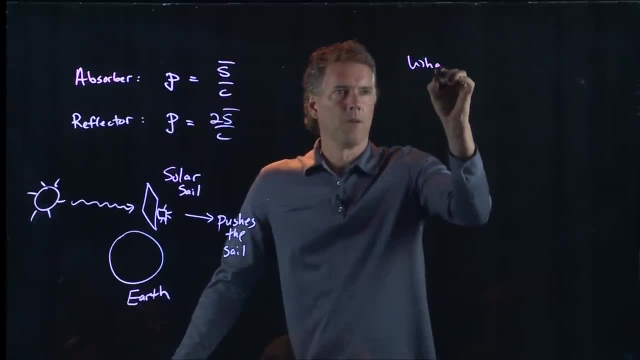 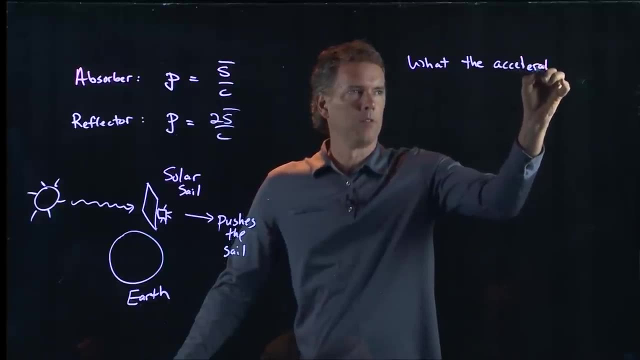 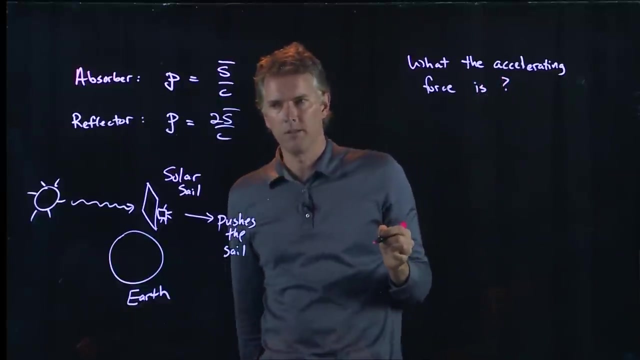 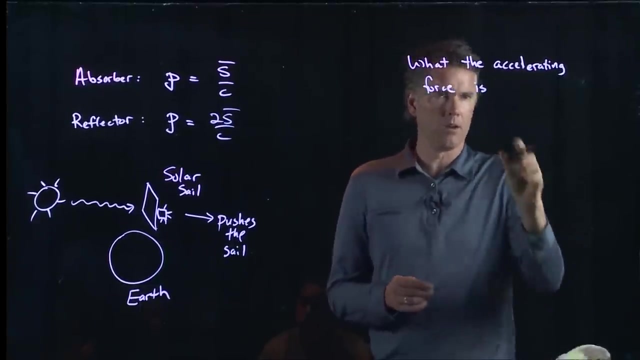 So let's see if we can calculate what the accelerating force is. Okay, Let's see if we can calculate that. Well, we know we've got pressure right. We just talked about pressure right here. for a reflector, Pressure is equal to. 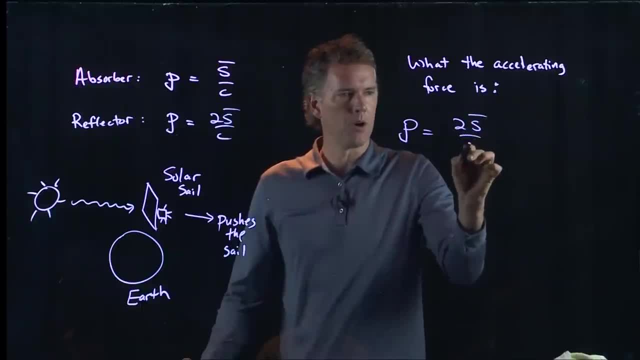 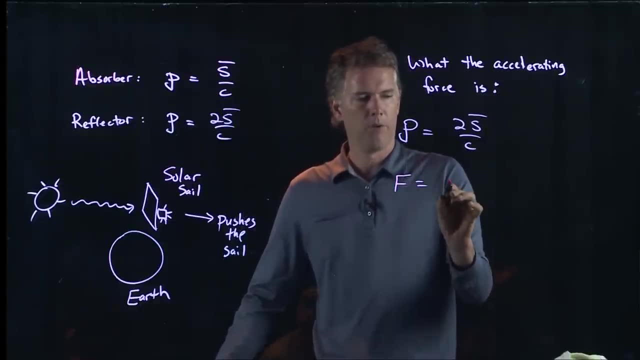 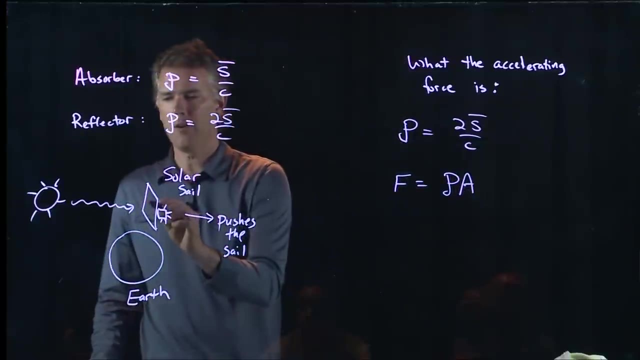 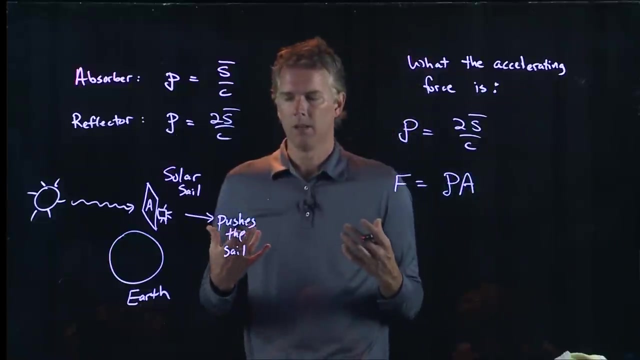 2s-bar over c If I want to calculate the force, force is just pressure times area, And so I need to know the area of this solar sail, And they actually make these things big, right, These solar sails can be 50 meters. 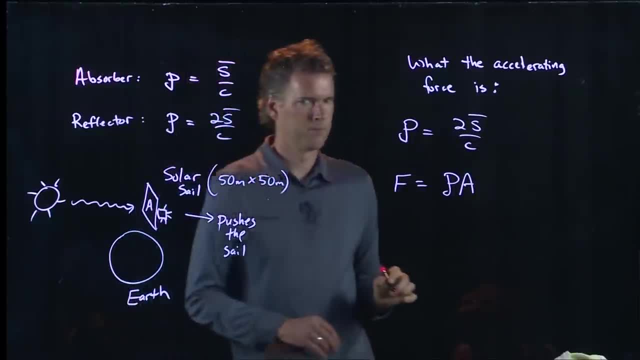 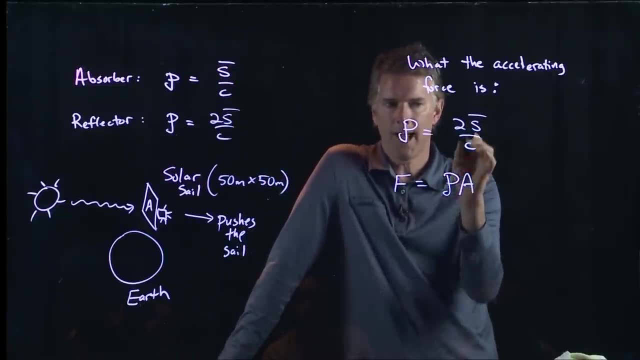 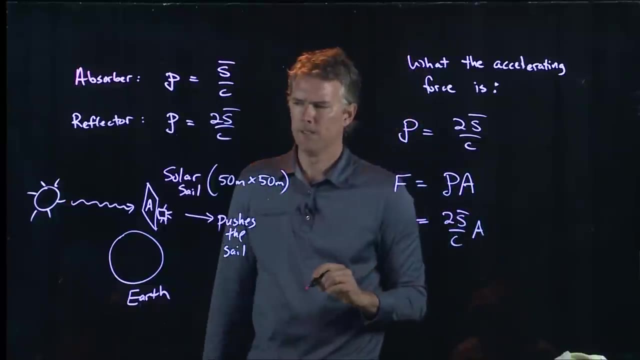 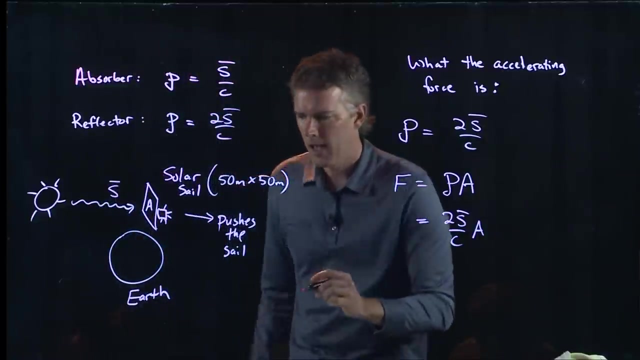 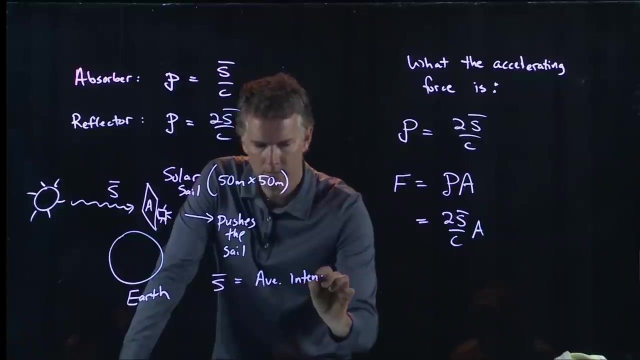 Okay, By 50 meters, and you want a big sail. Do we know what s-bar is? Well, s-bar is related to this electromagnetic wave that's coming in, And so s-bar is the average intensity, That's a trace elevator. 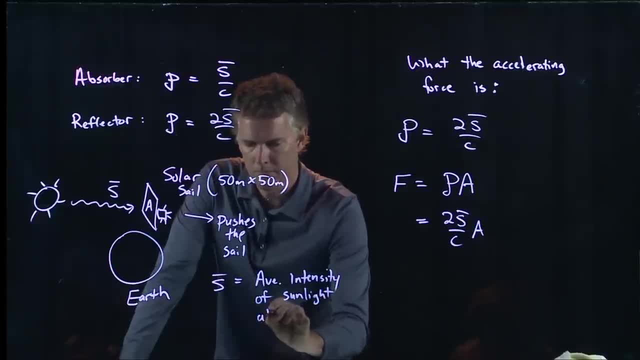 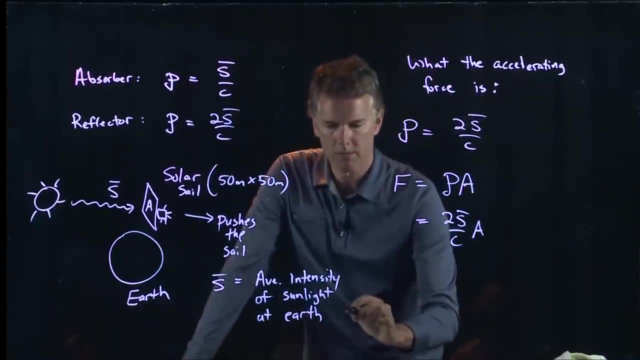 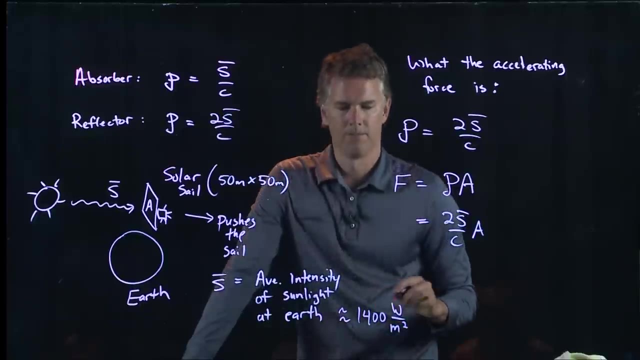 So s-bar is located at a place It has empresas in the whole world right And it's probably going to come in at the lowest pressure of directolla right. The airway of your� diminished And so it's able to do that stuff. 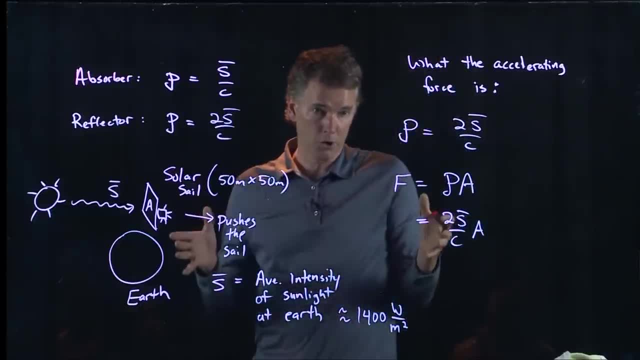 This is a test on actual energy. Hello, Hi, Hi, Hello. It's still small. Samsung It is, but it's places where our sun lies and where the Universe lies. car in the sunshine you leave all the windows rolled up. it gets really hot in there because 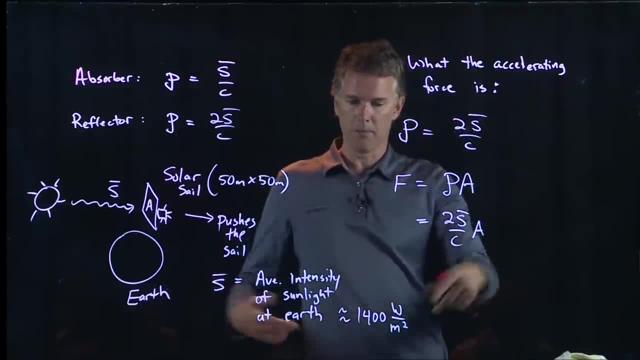 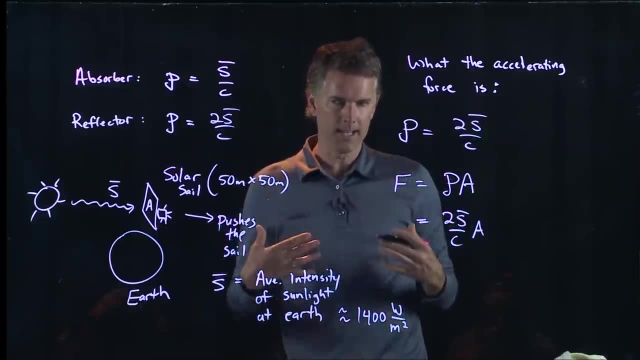 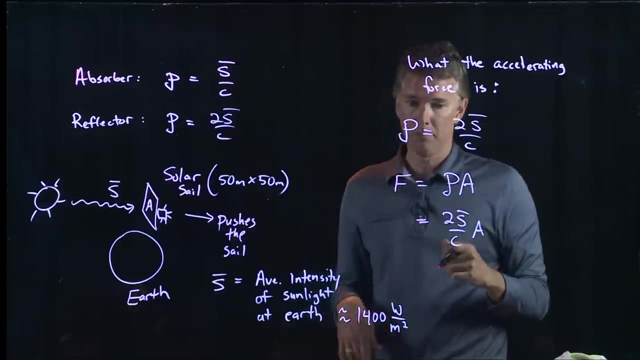 your windows have an area of like one square meter, And so they're letting in 1,400 watts of sunlight into your car. That's like you put the hairdryer on full blast and left it in your car. It would heat up in there quite a bit, Okay. so let's see if we can calculate this now. 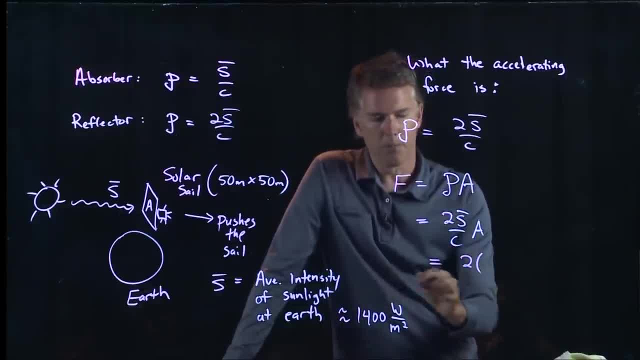 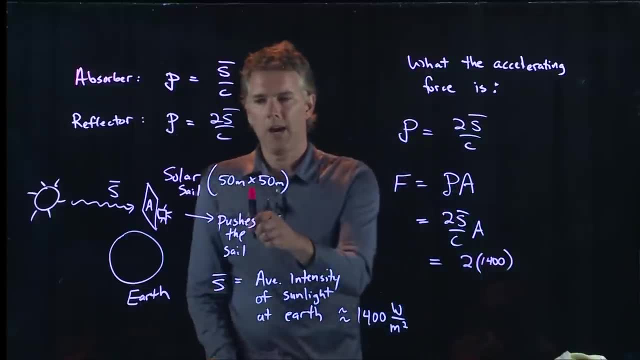 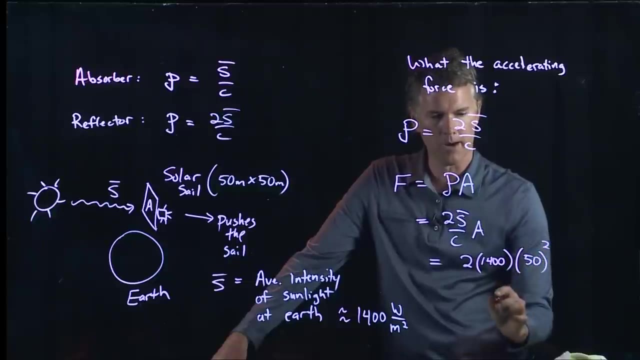 We've got 2 times s bar, which we just said is about 1,400 watts per square meter. We've got the area of the solar sail, which is 50 meters squared, And then we're going to divide by the speed of. 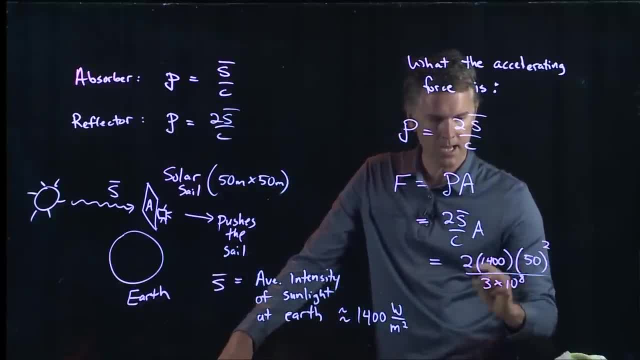 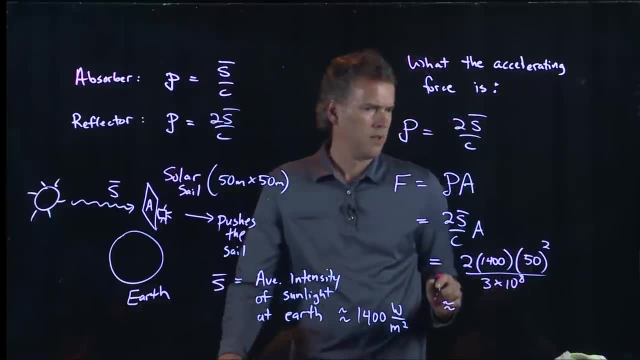 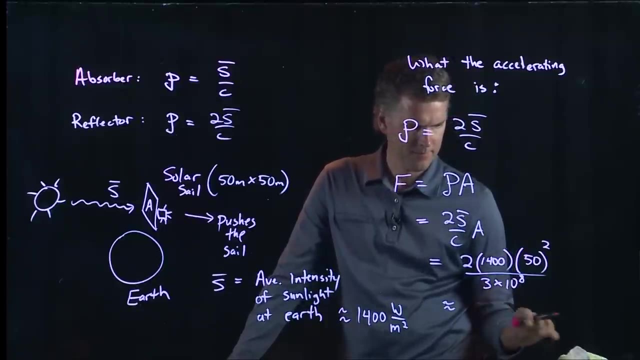 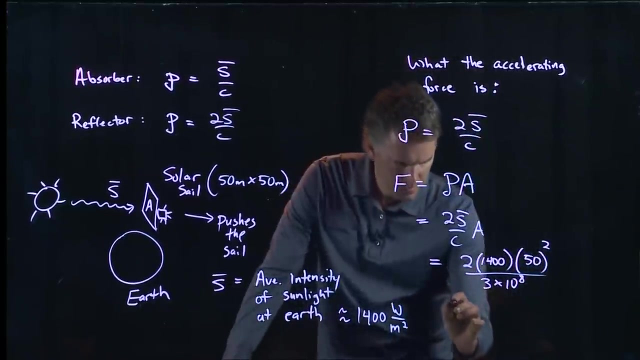 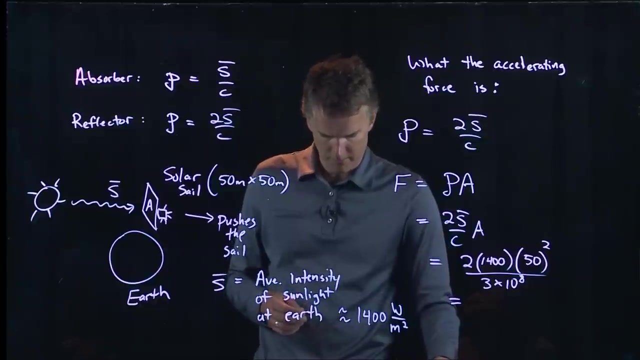 light 3 times 10 to the 8 meters per second. So if somebody punched that into your calculator, tell me what you think. I'll just let you guys do that. While you do that, I'll check Wolfram Alpha, If you're at home and you want to take a look. 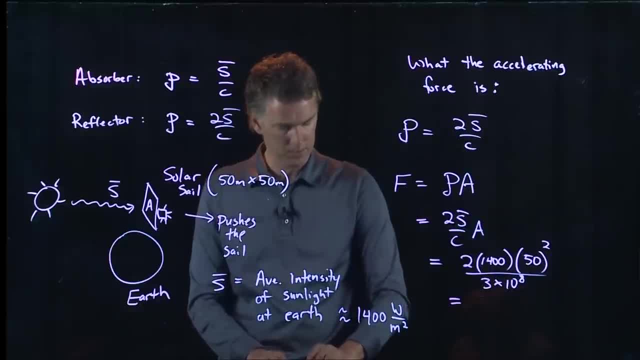 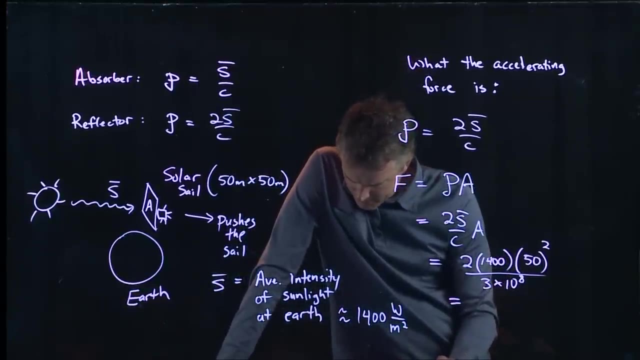 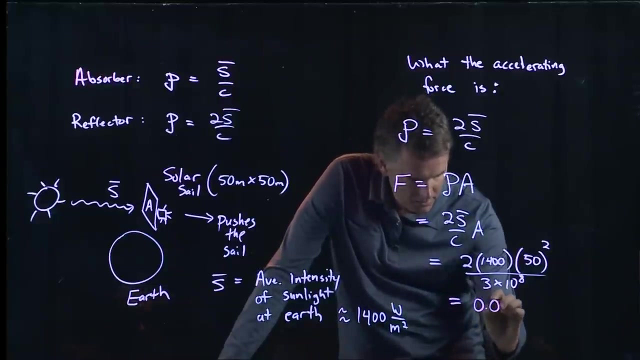 Wolfram Alpha is a great place to go. 2 times 1,400 times 3 times 50, squared all over 3 times 10 to the 8.. And I got 0.023.. Is that what you guys got? So 0.023.. And that 3 continues. but that's fine. 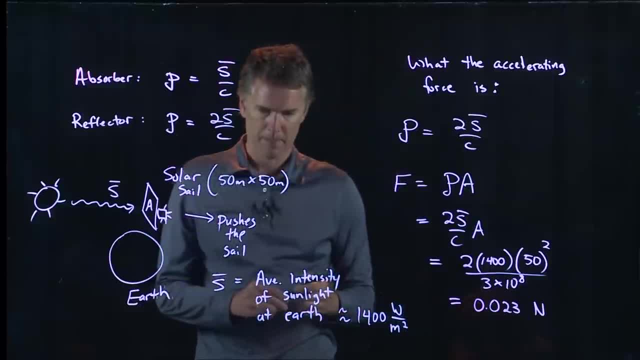 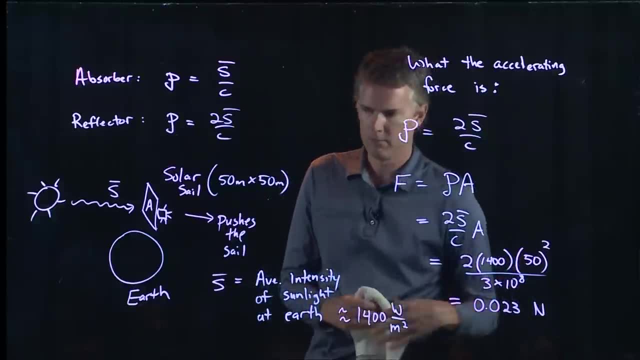 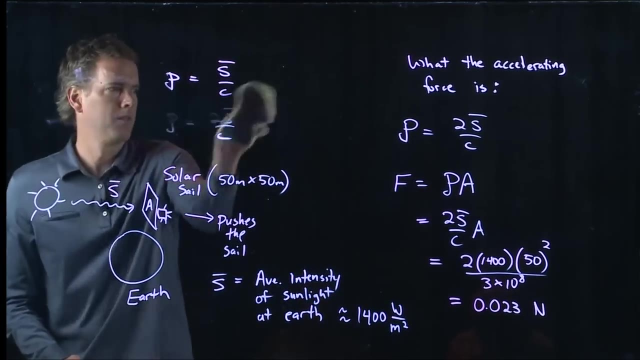 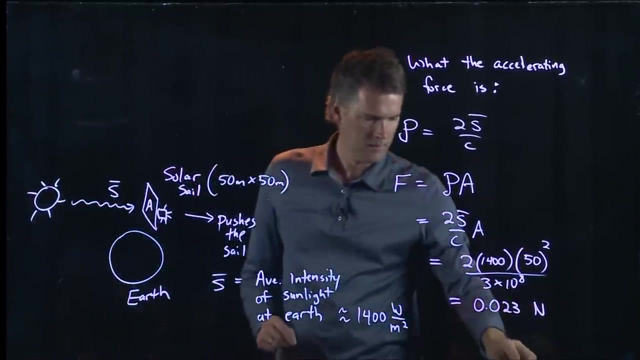 And the units are Newtons. So we need to work on that. So that's the force on this sail. It doesn't seem like a lot of force, right? That seems like a pretty small number. Let's put this in the comparison of something we know. 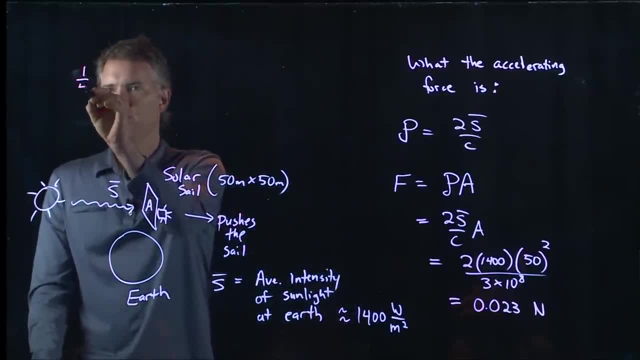 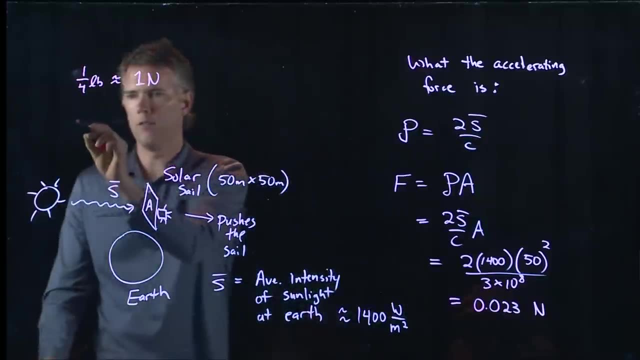 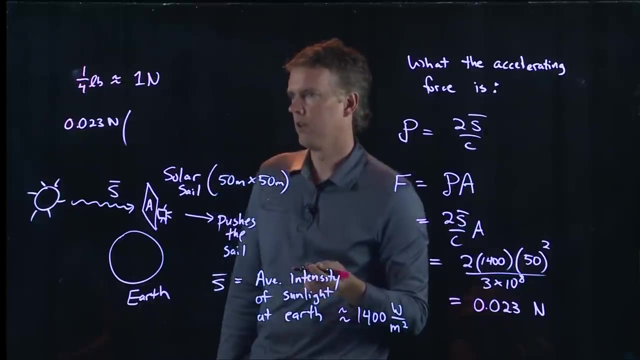 What we know is that a quarter pound is about one and a half miles. What we know is that a quarter pound is about one and a half miles Newton. So if I have 0.023 Newtons and I want to convert that to pounds, all I have to do. 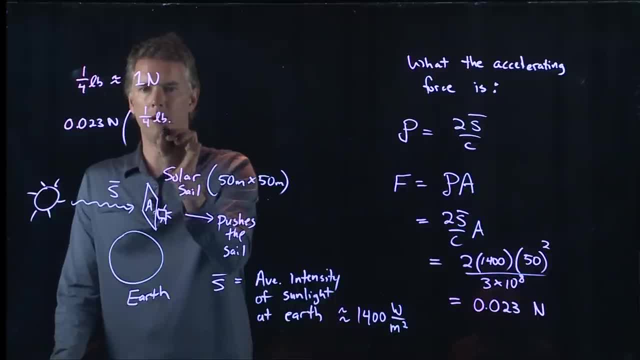 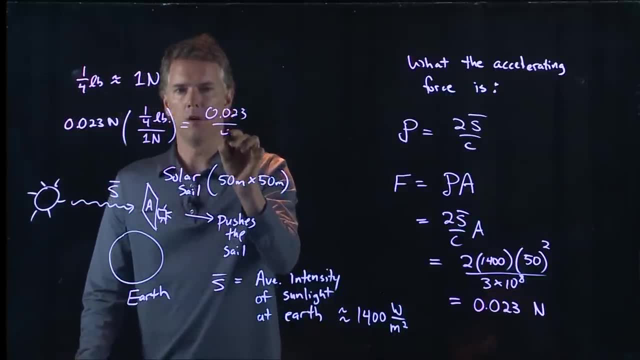 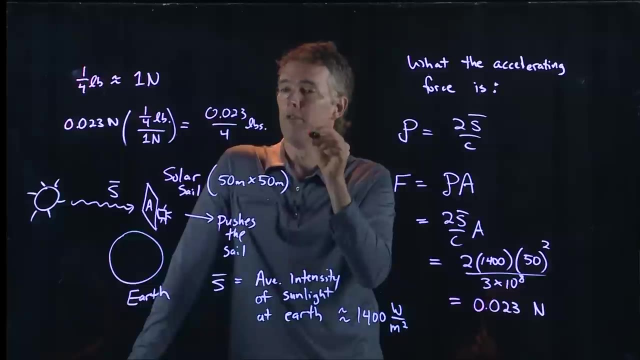 is multiply by 1. So it's a quarter pound over 1 Newton, And so I get 0.023 over 4 pounds. And 0.023 over 4 is what? Well, it's about 0.005 pounds. 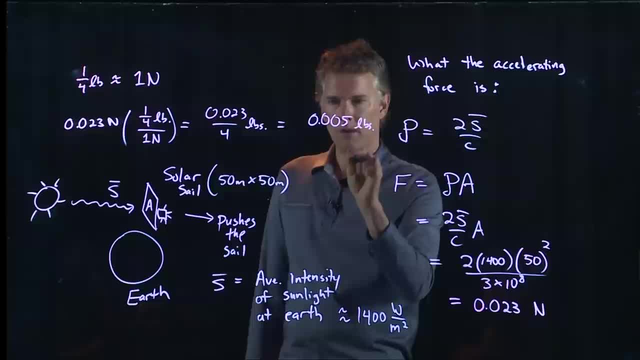 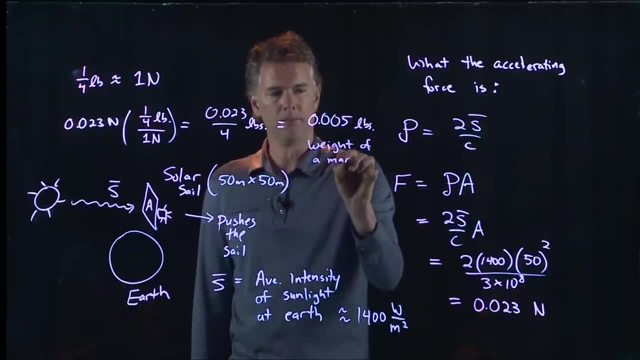 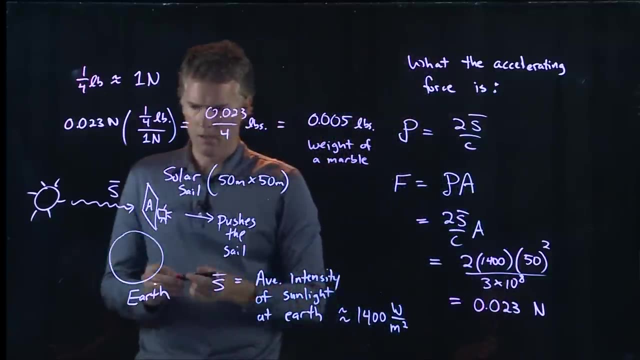 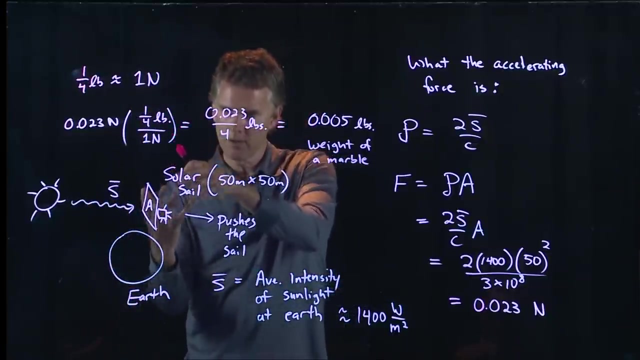 It's something really very small. This is about the weight of a marble. Okay, very small. This small marble has this much weight, So why would you do this right? If you're pushing on this giant spacecraft with the weight of a marble, who cares right? 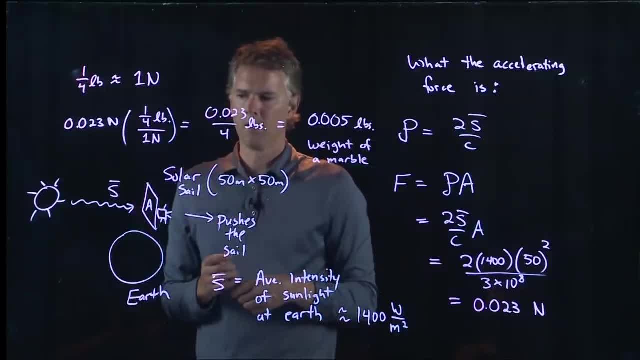 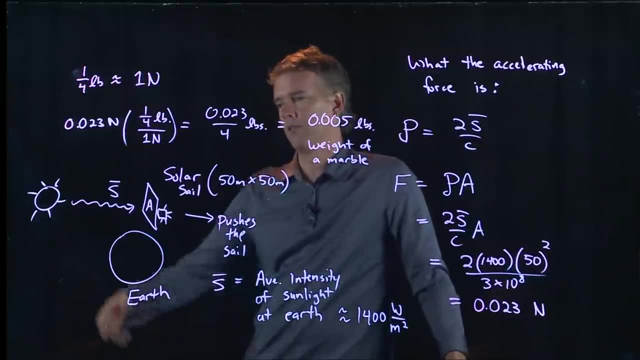 The acceleration of that thing is going to be really, really slow. Why would you even do this experiment? Because sunlight is free. You don't have to send it, You don't have to send any fuel with the rocket. It's continuous, It's on all the time. 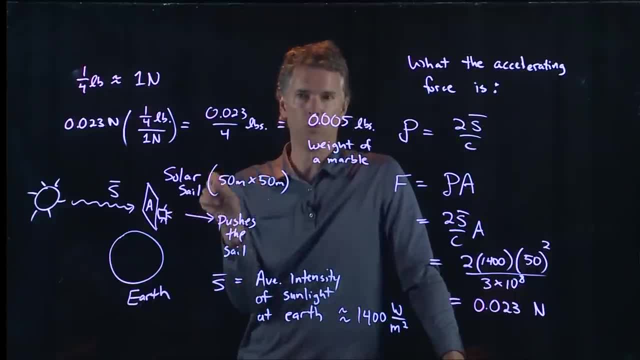 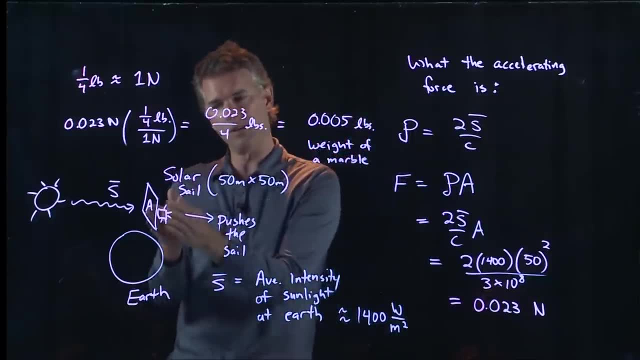 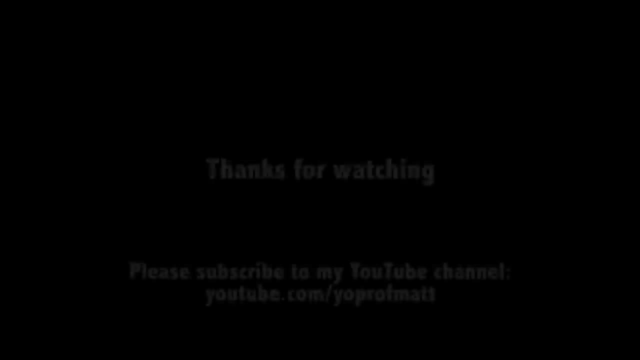 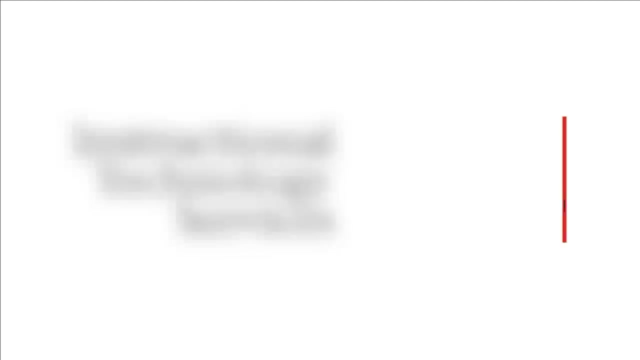 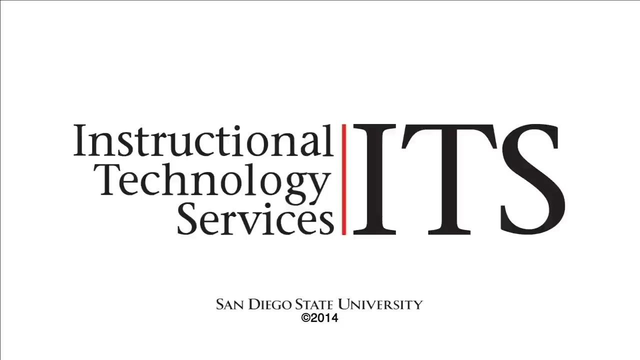 And in outer space there's essentially no resistance. There's nothing slowing you down. So even though this force is very small, which means the acceleration is going to be pretty small, it keeps accelerating forever. okay, until it leaves. So it's going to keep accelerating forever. okay, until it leaves. So it's going to keep accelerating forever? okay, until it leaves.